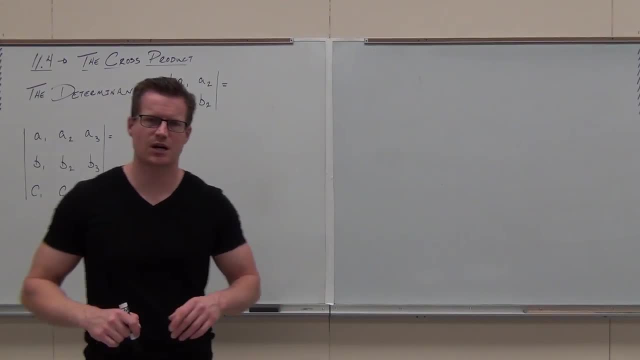 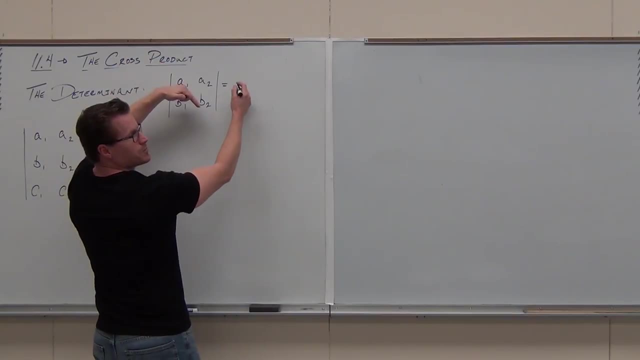 How do we find the determinant of a matrix? Someone out there who knows, tell me how you would do it This first. So we do a diagonal multiply- hey, that's where you get the product. Diagonal multiply, And then plus, minus, which one? 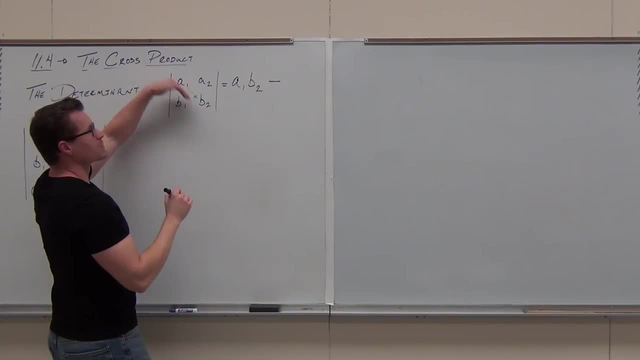 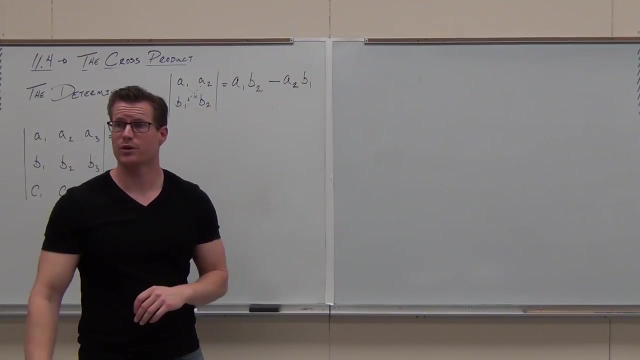 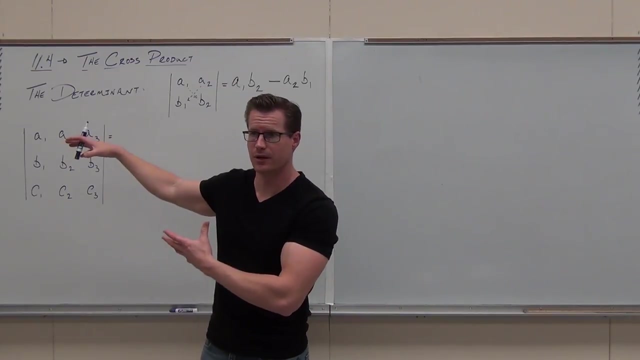 This way, This, no, I'm telling you. I'm telling you this time, This way, And then a minus sign, and then this way. That's how a determinant works for a two by two matrix. Now, when we start the three by three matrix, which is where we're going to live in this class, there's a variety of ways to do it. 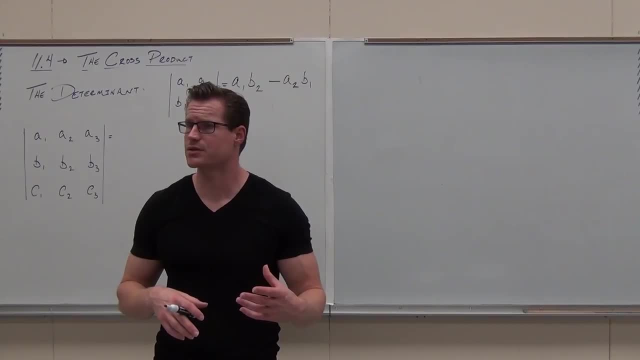 I'm going to give you the best way to do it for working with vectors, right? So there's a couple ways you can do it. This one's going to work really, really nice for the stuff that we're going to use. Does that make sense to you? 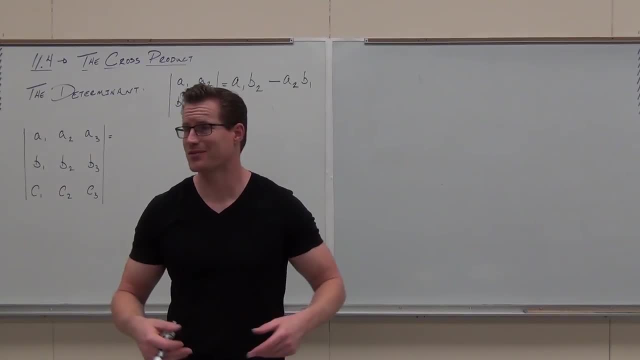 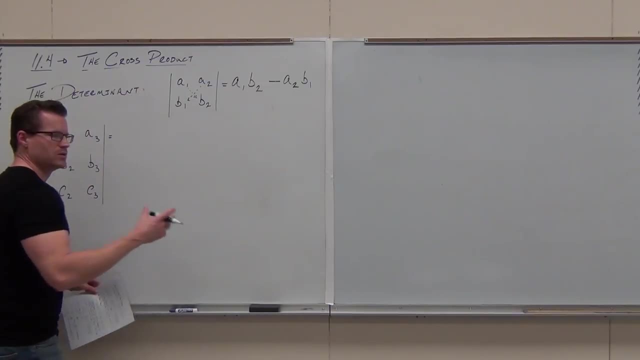 So you're like. I know a different way to multiply: a determinant. That's great for you, That's awesome. Use this way and you'll see why. as soon as we start figuring out what the cross product is, okay, There's a really unique thing that we can do. If you have a three by three matrix, we can actually take three two by two matrices, find the determinant of those and multiply it by those terms, those components, and get a determinant of a three by three matrix. I'm going to show you how it works. 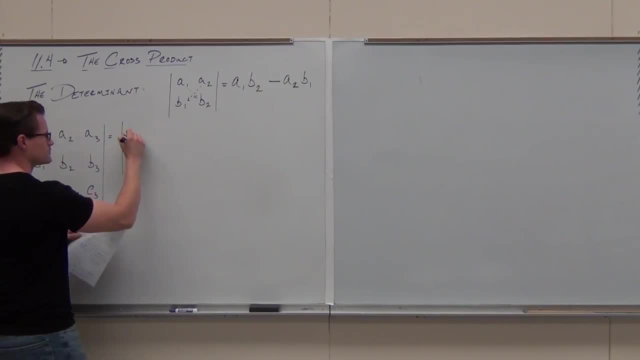 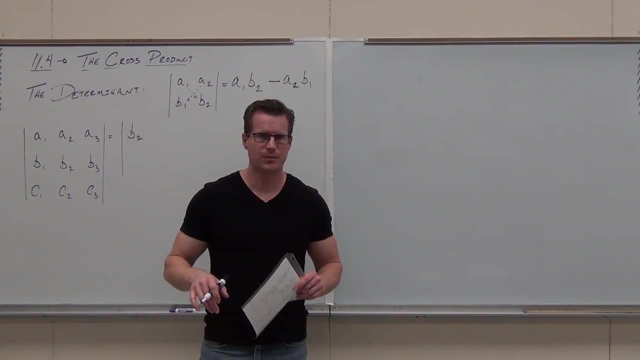 So if we do this, this is all going to look very confusing right now because there's going to be lots of numbers and letters floating around. It's honestly really really easy to do, So. don't let all the numbers and stuff confuse you yet. all right, 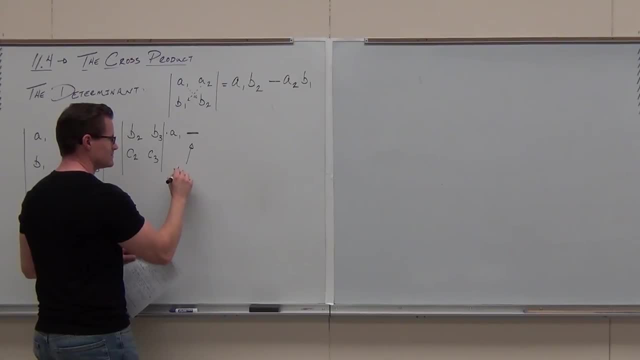 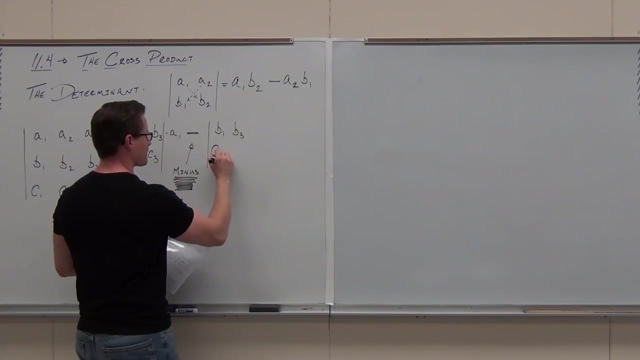 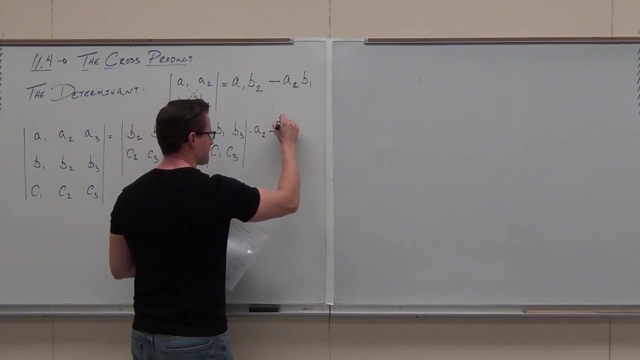 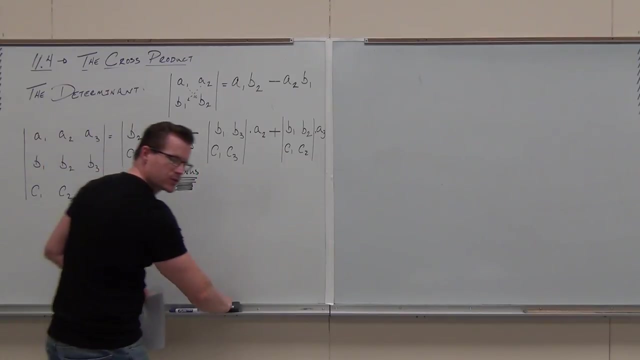 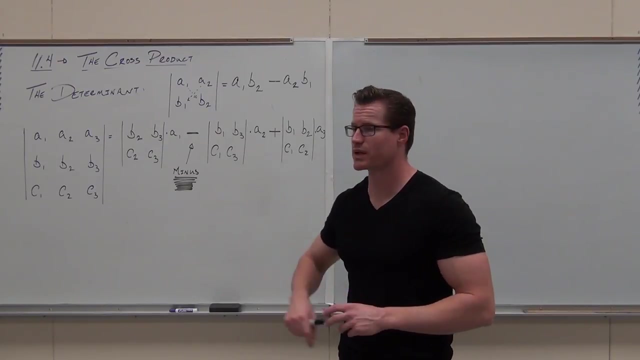 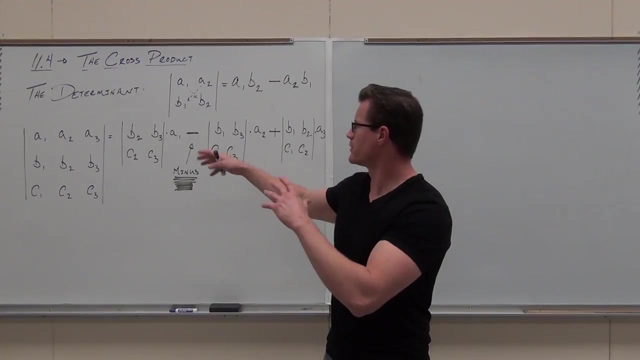 What sign is that? For real, all right. 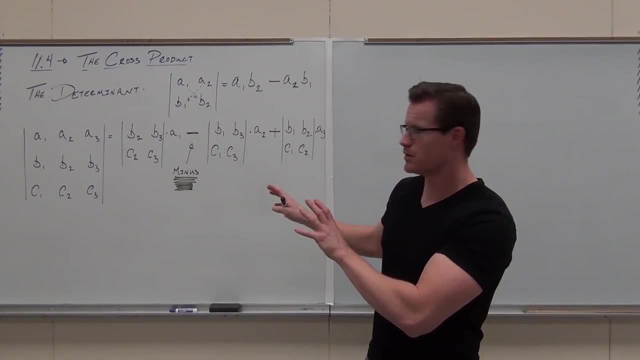 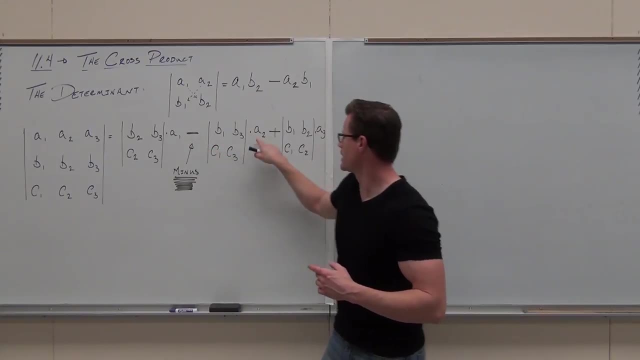 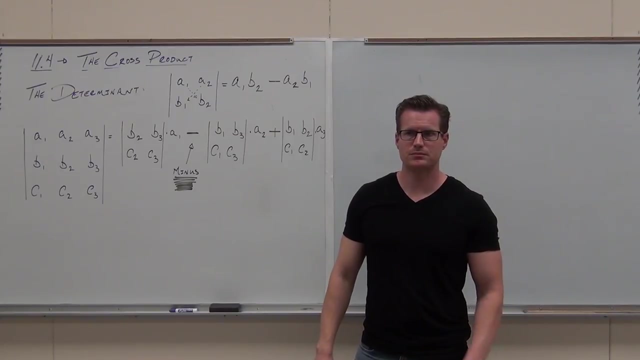 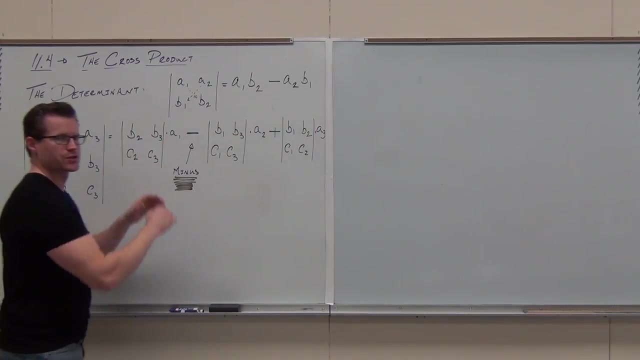 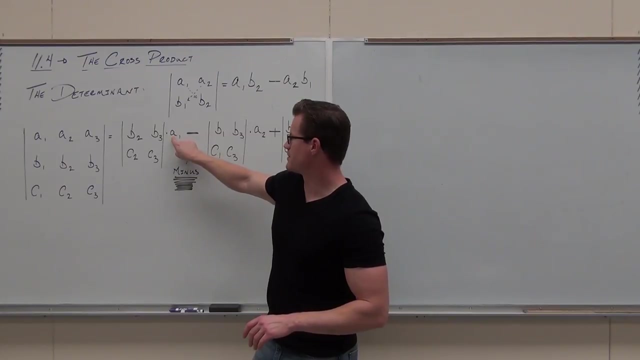 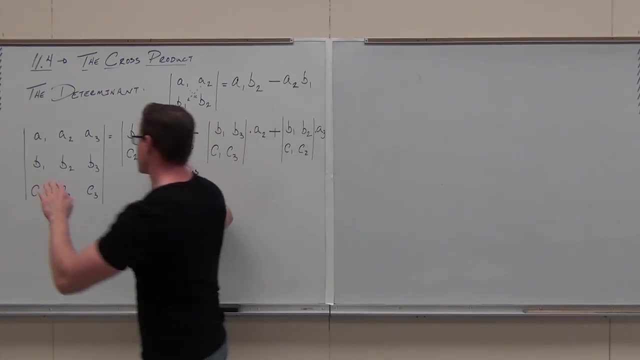 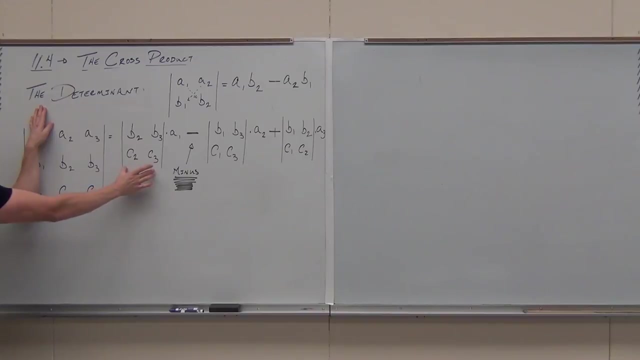 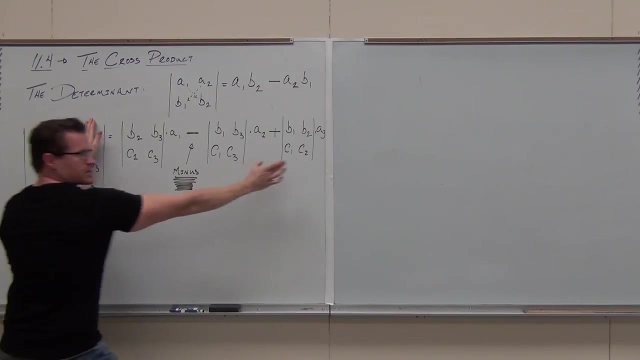 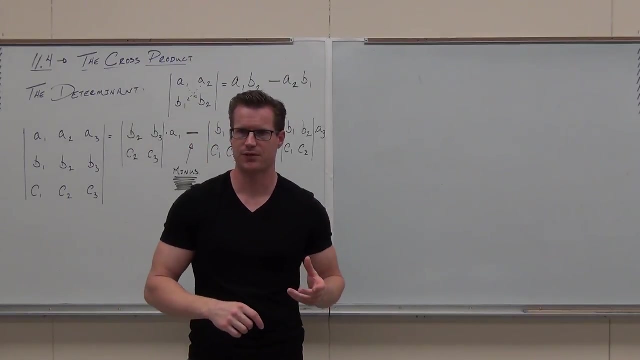 A very fast way to find the determinant of a 3 by 3 matrix. 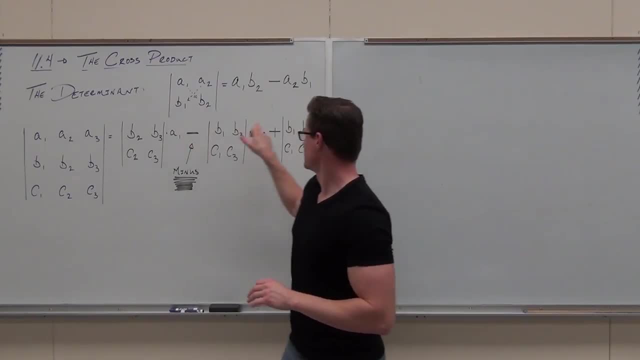 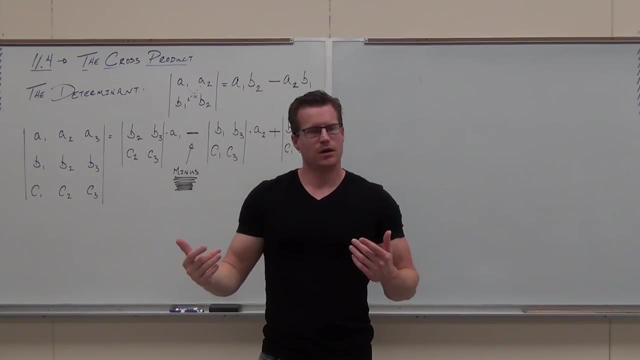 Very, very fast. The only thing you've got to worry about is minus plus. that's a big deal. So if you're okay with the idea, We're going to practice it. It goes very fast. I will warn you and it's going to happen to you. 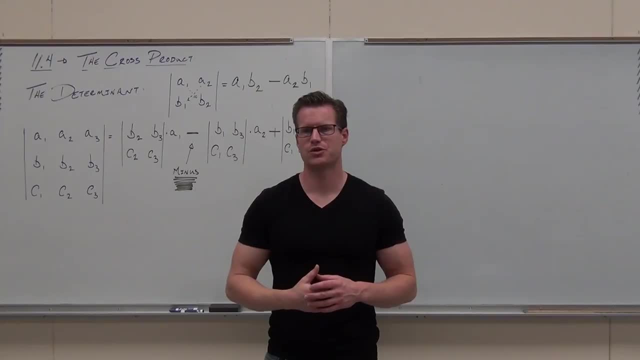 Because it happens to me too, The biggest mistakes you're going to make. what do you think? Signers Happen all the time, Especially when you've got positives and negatives floating around. You're subtracting negatives. It happens all the time. 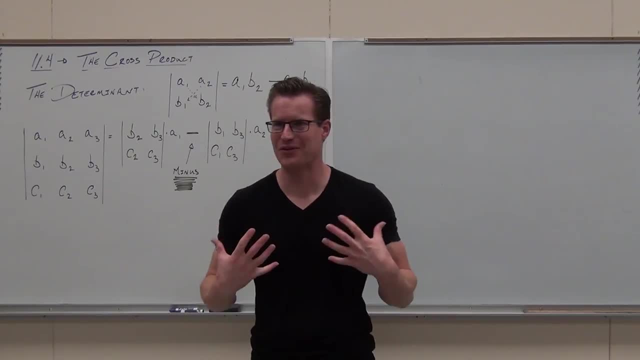 Now we're ready, Get the chills a little bit. Did you feel that We're ready for something cool? That's what I meant. That's why I get the chills, because it's so cool, You just get the chills. 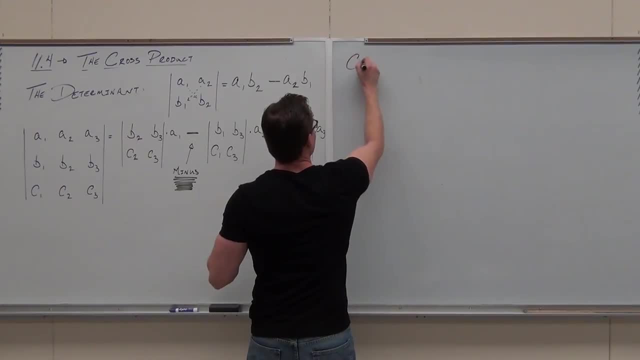 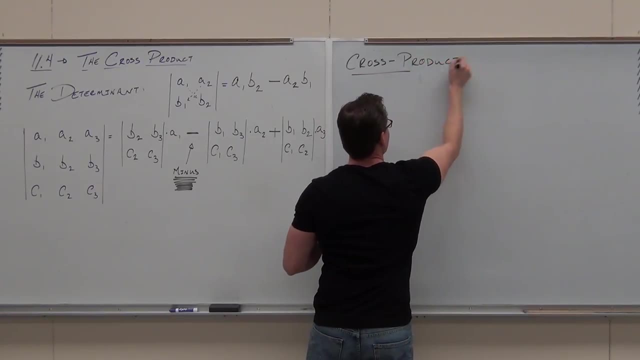 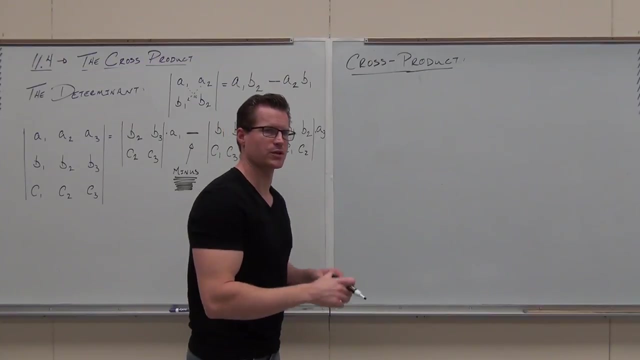 We're going to talk about what the cross product is now. With any two vectors, we could do a dot product. We can also now do a cross Cross product, And here's what it looks like. Since it's still a product, it's got to have a symbol for multiplication, but we already 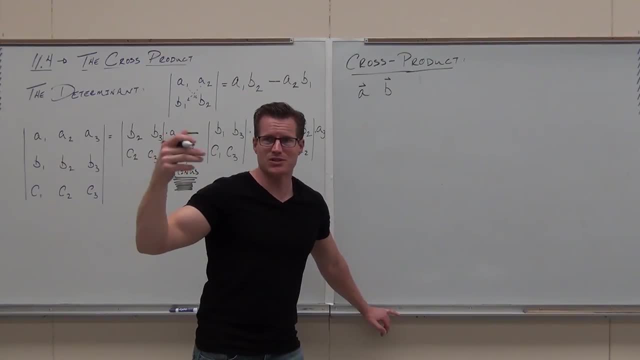 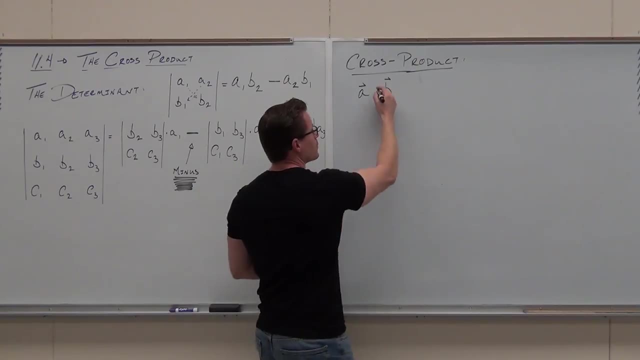 used up the little dot because that was called dot product. But then we had this old symbol going way back. What's the other one that we use for multiplication Cross? Yeah, That's that little dot And that's called a cross product. 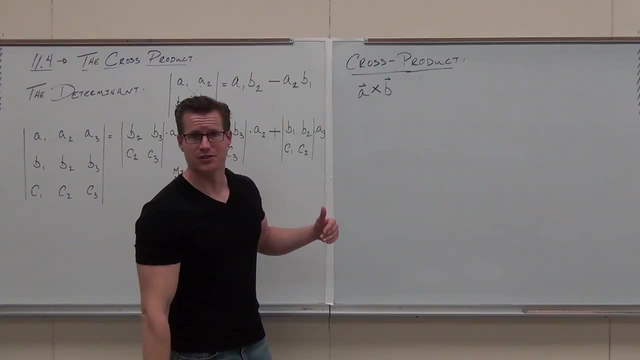 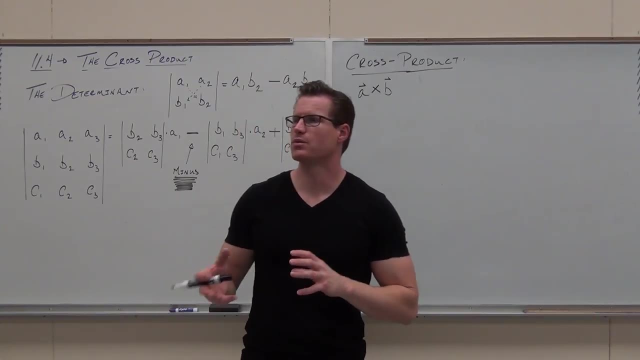 What's really kind of convenient. not, mathy, is the way you find a determinant here is going across the determinant which is kind of convenient. So cross product, cross. the determinant Works for me. That's the way that we write the cross product. 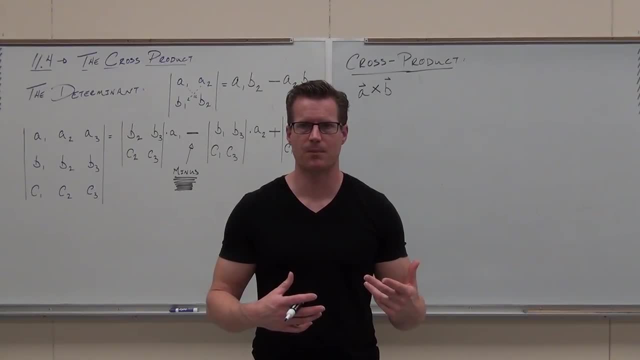 So whenever you see that we're talking about a cross product, Are you with me on what I'm talking about? I'm going to give you the definition of what the cross product actually is. I'm going to show you why in the world we have this thing. because, like what? 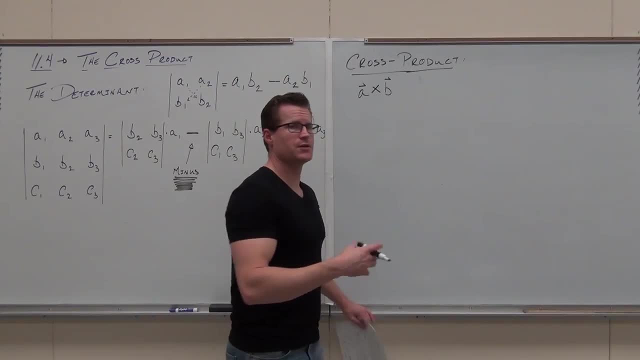 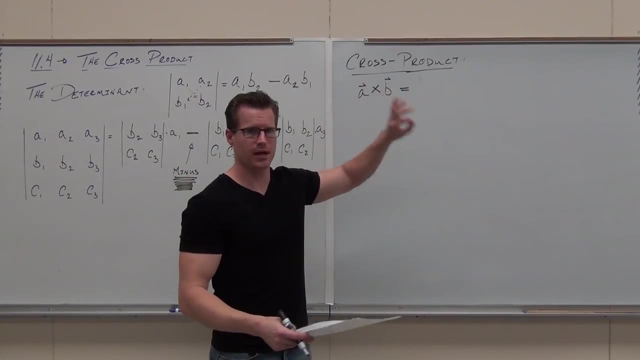 Why, And I'm going to put them together for you. Here's the definition of what a cross product actually does. So, provided we have these two vectors- A1, A2, A3, and then B1, B2, B3,- here's what the 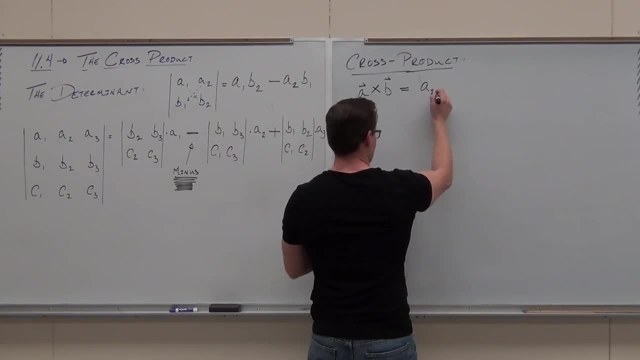 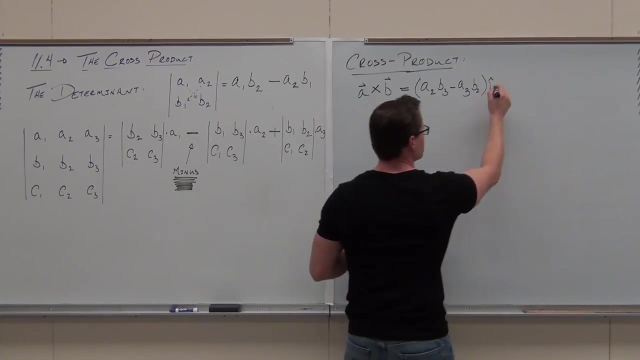 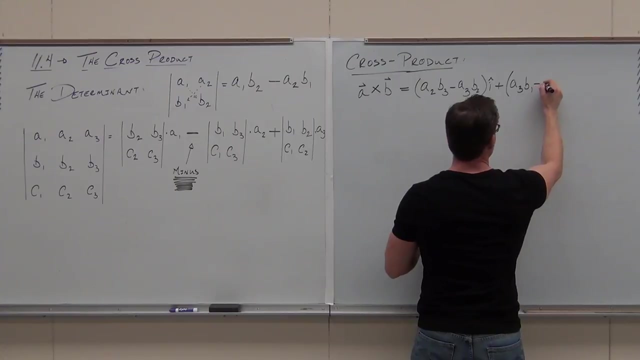 cross product does? It? takes A2, B3, minus A3, B2, and puts an I after them, A3, B1, minus A1, B3, and then puts a J after them. Okay, All right. 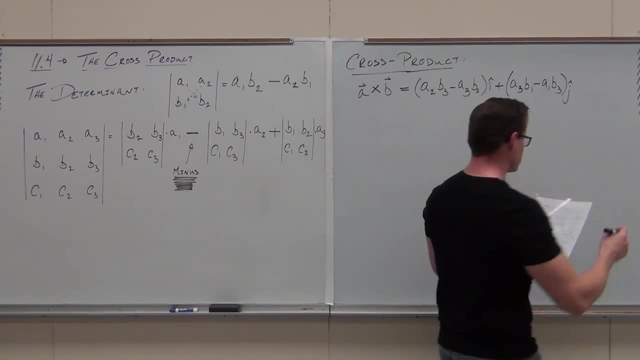 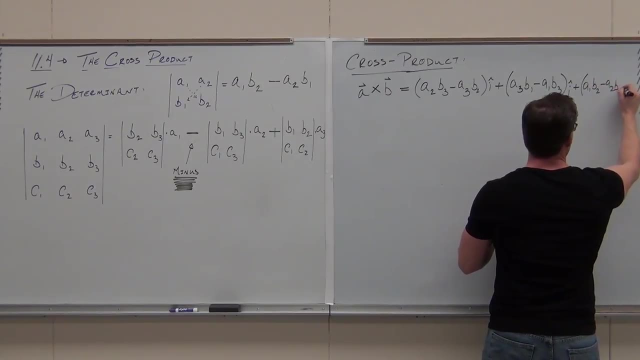 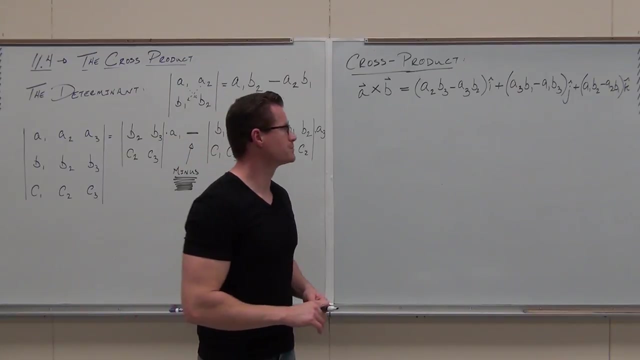 And then A1, B2,, A2, B1, and puts a K after them. Here's my first question to you. When you did the dot product, what did it give you Scalar? When you do a cross product, what's it going to give you? 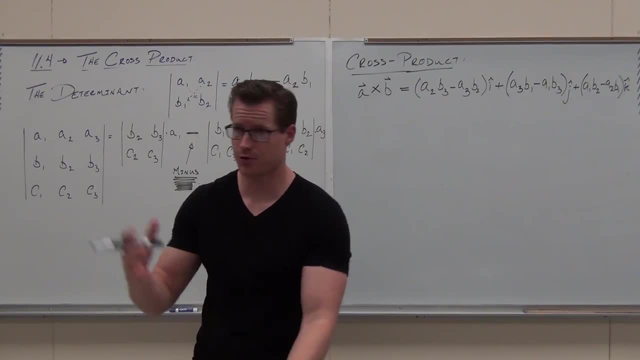 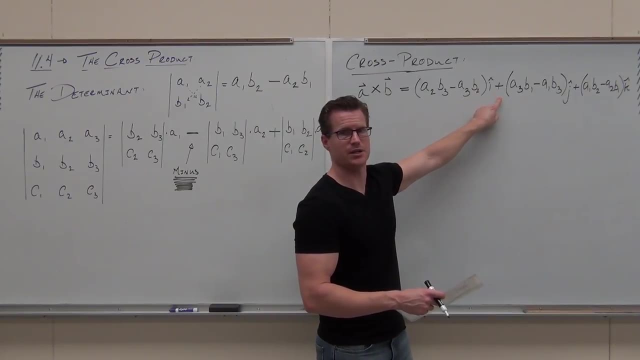 A vector. A vector, That's a different result. So this thing that we're getting first thing, the cross product, gives you a vector. By the way, did you make sure to put a plus there? I'm not making a mistake. 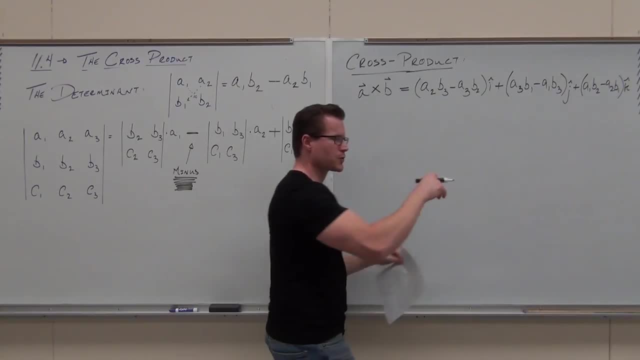 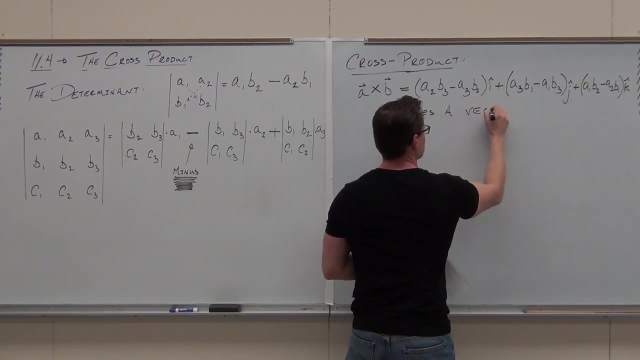 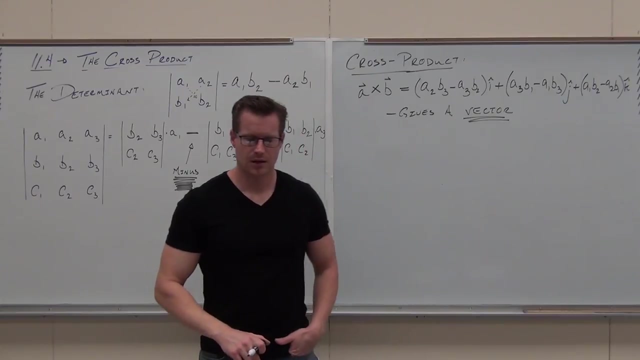 Okay, Put a plus there. I'll talk about why in a second. So first note: you've got to know this thing gives you a vector, Not a scalar. Let's even write that down because a lot of people go: oh, dot product, cross product. 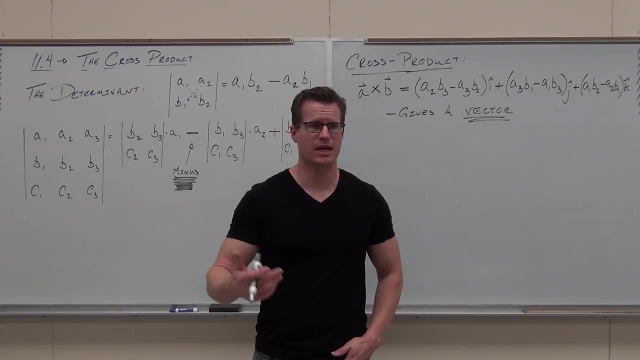 what's the difference? Well, there's a big difference, but there's a huge difference between them. One of them is a scalar. We learned how to use it a lot last section. This section goes: okay, we're getting a vector. 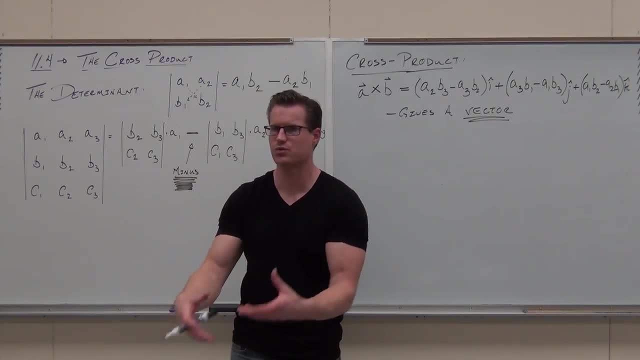 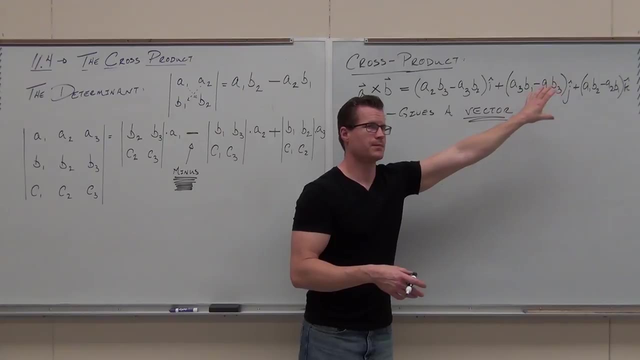 What's that vector do? That's the whole subject matter of this next section. okay, is what we're going to learn is what it does. The main things you need to know right now is, firstly, how you do it this way. 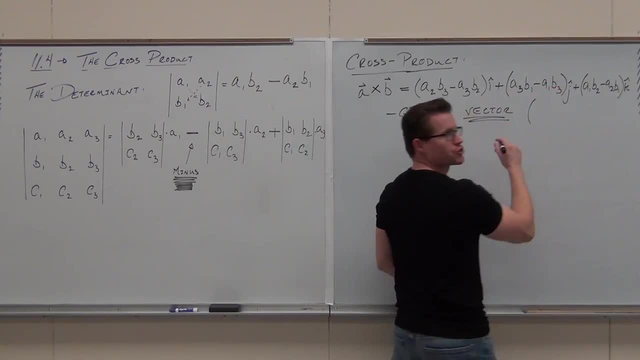 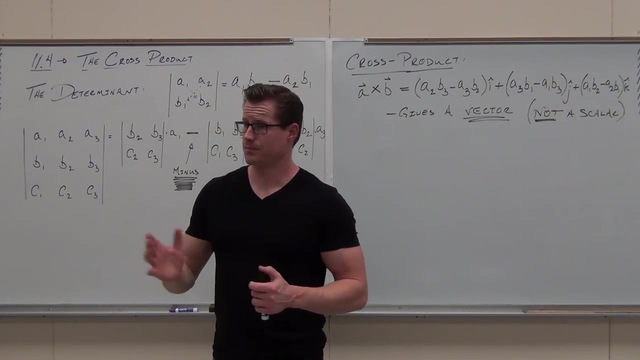 Secondly, what it is. It's a vector, It's for sure, not a scalar. Now the other thing why we even did this: look: you can do this for the cross product every single time. A lot of teachers teach it that way. 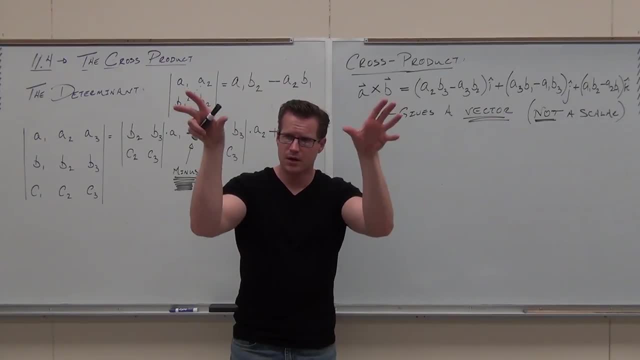 Oh, that's how you do the cross product. You just take your vectors and you do the A2 with the B3 minus the A3 with the B2, and then you keep going And you do all that And that's fine. 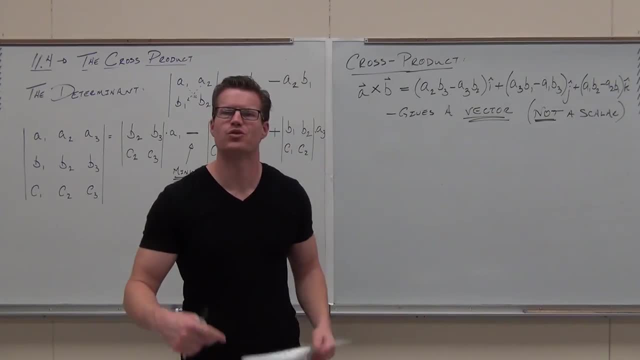 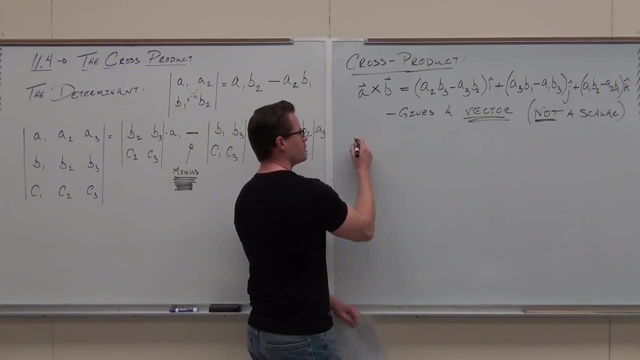 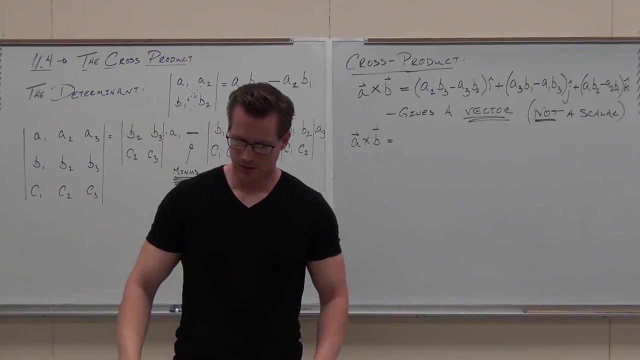 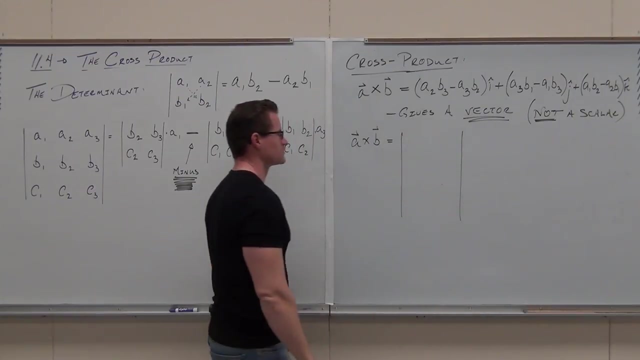 It works every time. However, there's a really really much more better way to do this. Let me show you that. So if I wanted to find another way to do this, check this out. This is pretty cool If we take the components of our vectors. 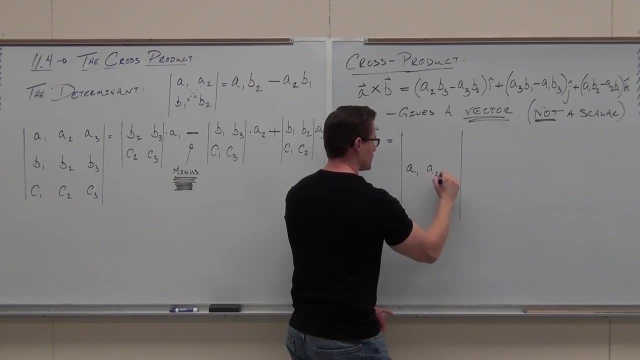 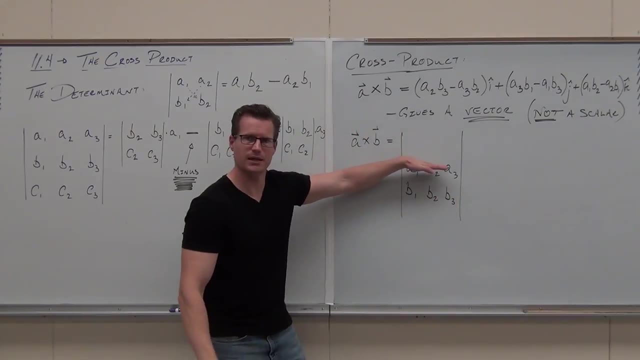 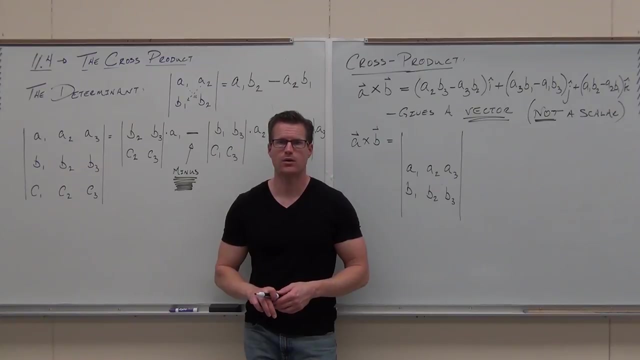 Like that, And we put them on the second and third row respectively. And you're going to ask me this later: Does the order matter? We're going to determine that. okay, Right now, put them in the order that I'm telling you and we're going to say we're. 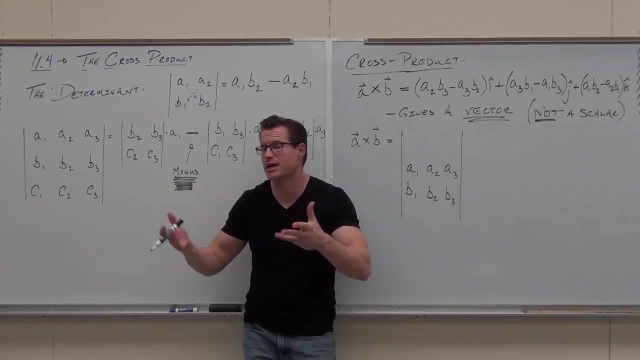 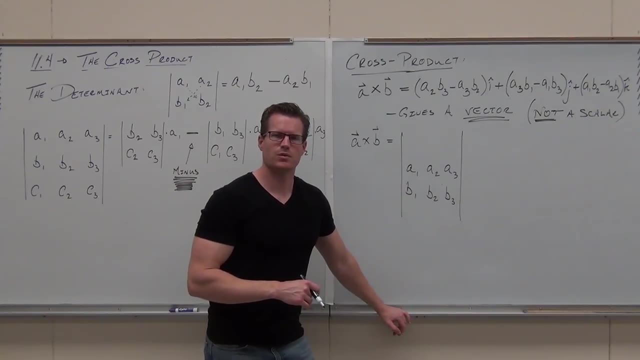 going to see later. does the order matter? What does the order mean? What's the interpretation of that? Just hang on for a second on that one. Up here we go. yes, let's kind of do something really cool. Let's dot or let's not dot this. 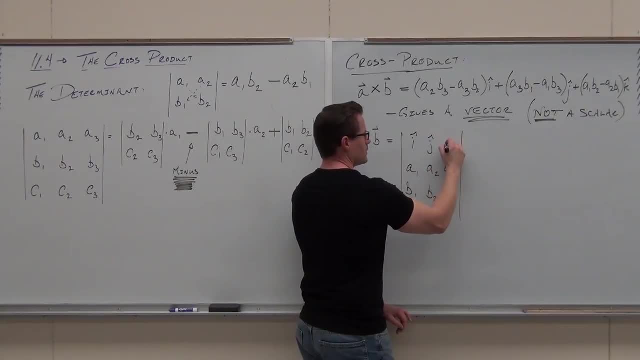 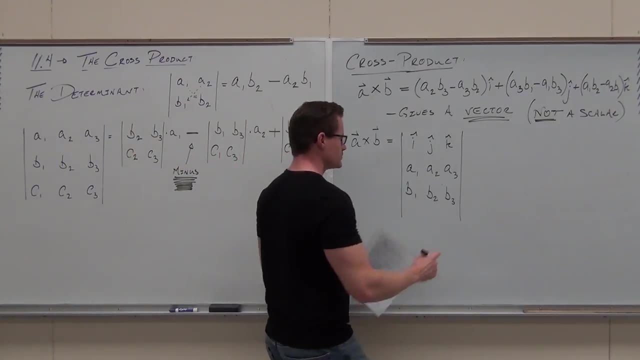 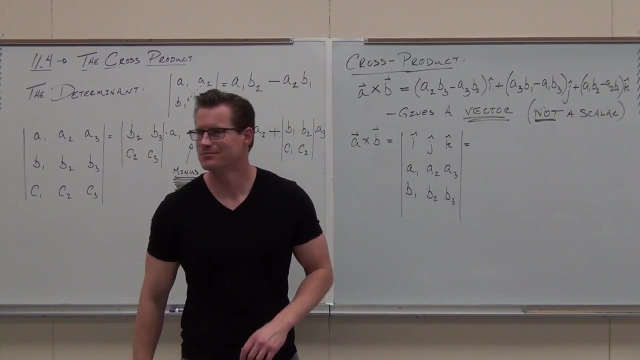 Let's put another vector- i, j and k- and let's see what happens If we do it. bless you, I'm going to have to bless you. I'm going to have to bless you all. Now it's my turn. 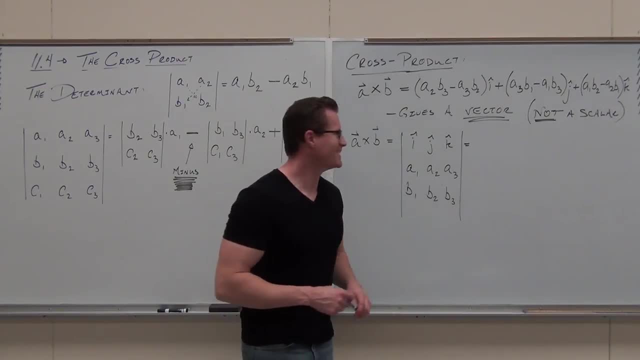 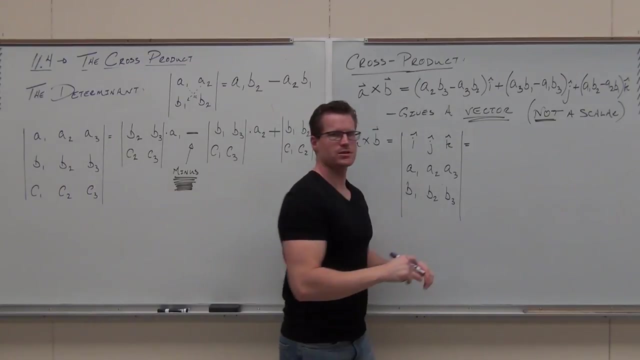 You have to bless me, Bless you, Bless you, Thank you. Let's now take this junk, apply it to this thing and let's see what happens with it. OK, So check this out. If I do this to this, what's the first thing I would do? 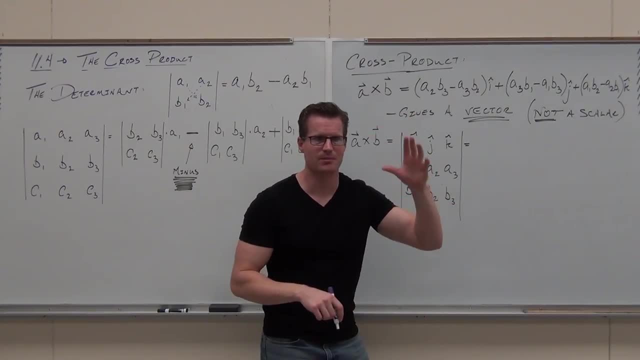 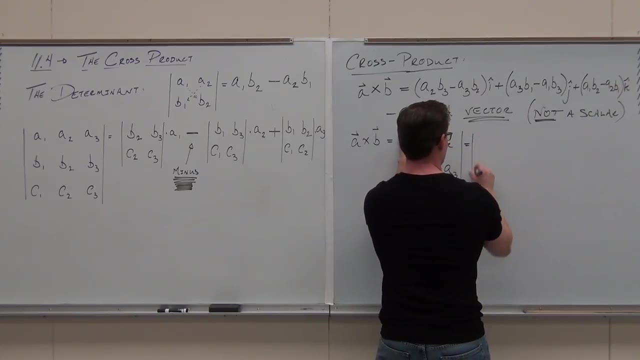 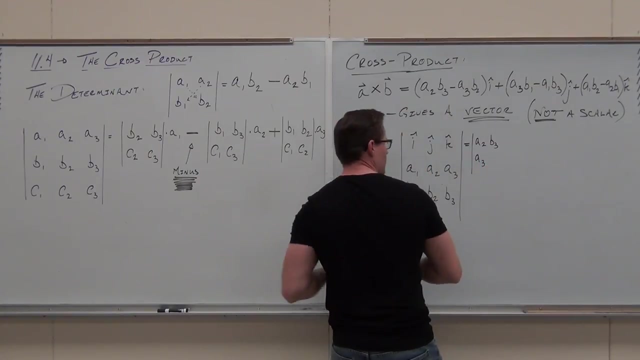 This guy remember covering it up. I literally have to cover it up, otherwise I get my numbers mixed up for real. So I cover it up and I go: OK, It's this, This, This is a square matrix. Sorry, I'm doing the multiplication in my head right now. 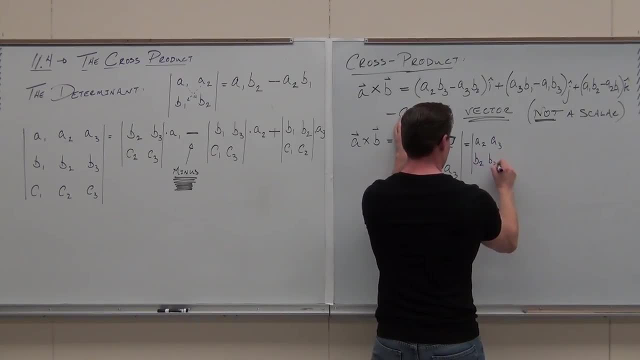 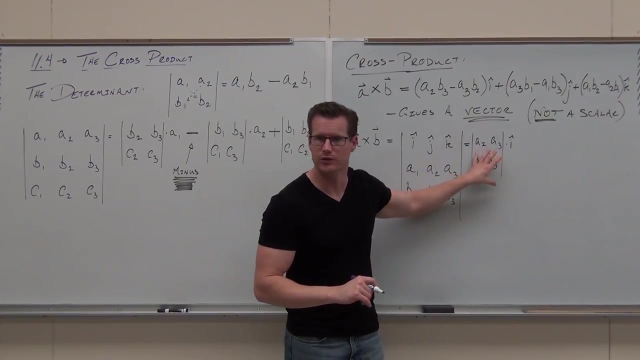 Now here's the magic. What goes there? i, i, i, i, i. Is it OK to multiply a? that's going to be a scalar, because these are all numbers. so is it OK to multiply a scalar by a vector? 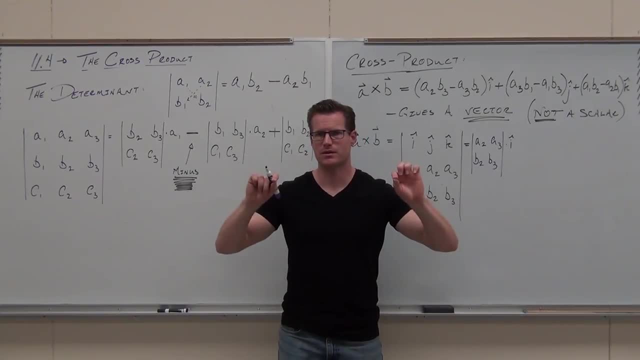 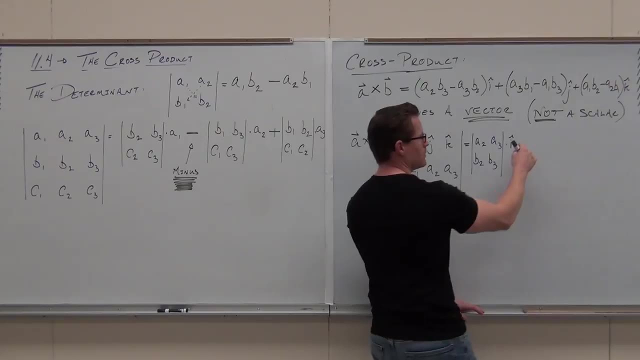 Yes, Yes, Absolutely. You're growing the i unit. That's what's happening. It's a unit vector. You multiply by numbers. It's growing in that direction. That's all that's happening. Hey, big one Minus. 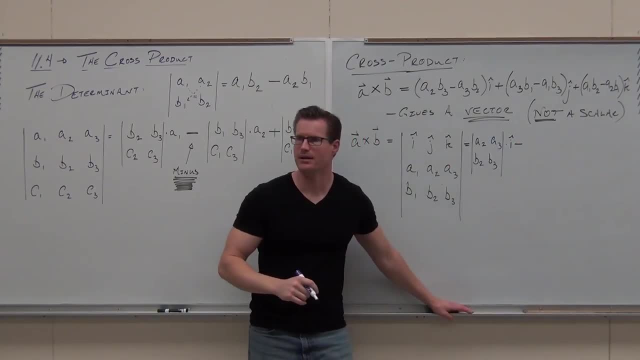 It's a minus. Now, this is where you're going to be lost for just half a second. Wait a minute, I Just wait, You'll see. Trust the Leonard, Trust the Leonard. Just on this, though: None of this. 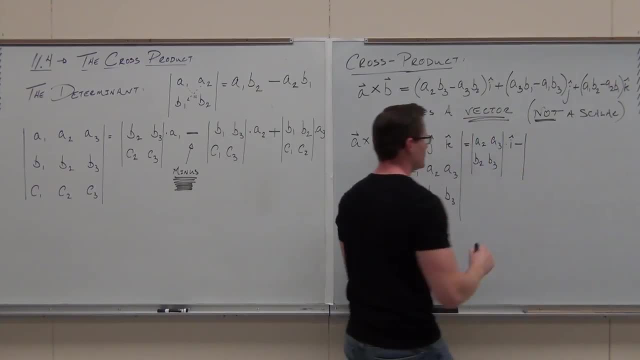 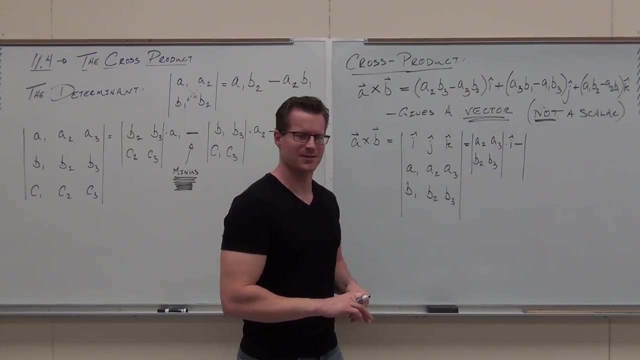 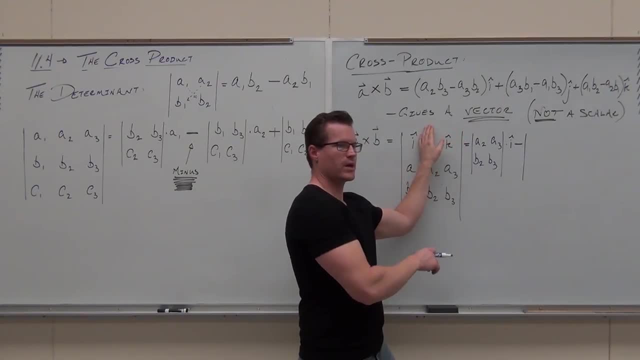 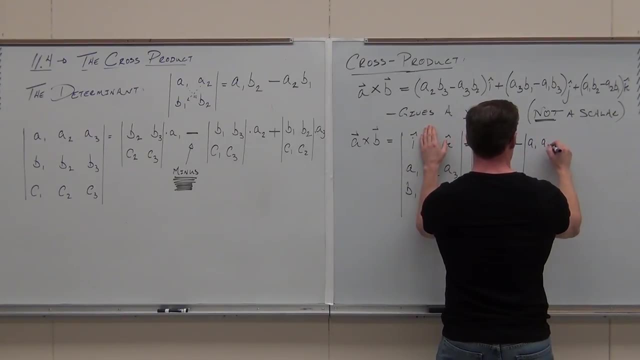 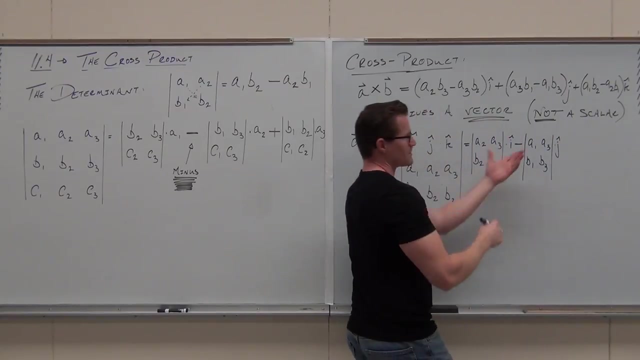 We go: i j k, That's what we do. We're going to cover up that one. We have another square matrix. We have this, that Again, scalar vector. We're cool. Plus sign, Plus sign, Just like we had. 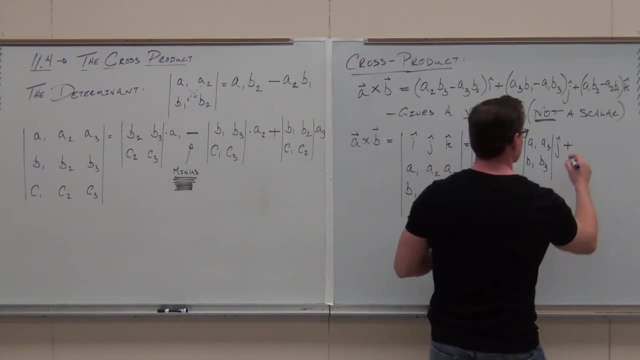 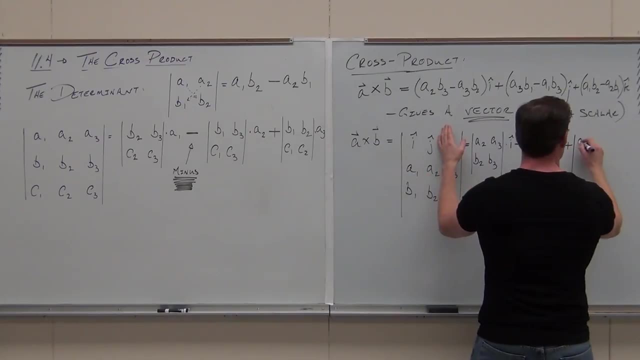 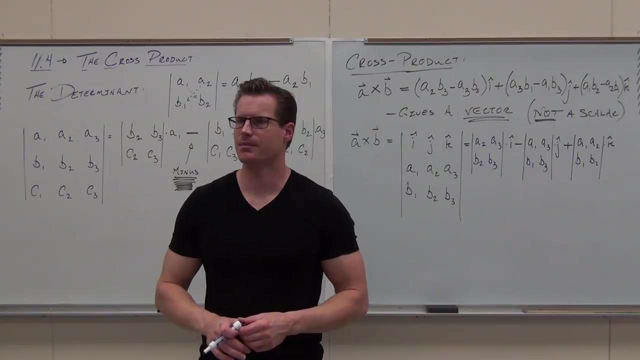 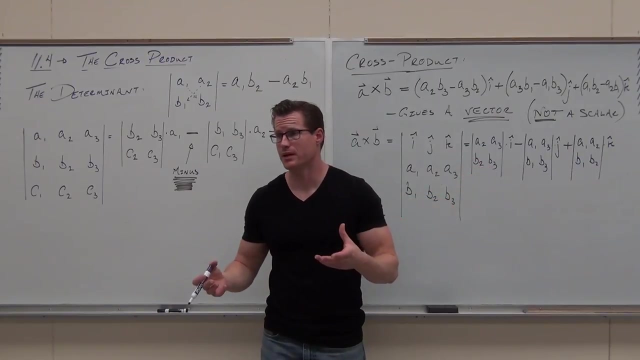 And if we cover up that last column, we've got our last little square matrix here, And all I want to do right now let's just verify they're the same. All right, This is no better or no worse What this does. it gives you a way to remember it so that you don't have to memorize that. 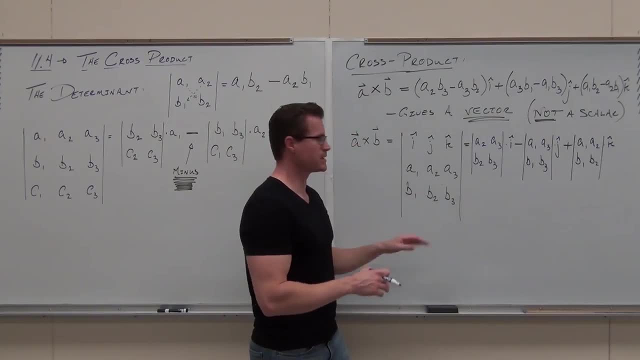 Because that's a bunch of junk, man, That's hard to memorize. But memorizing this determinant, this determinant, this determinant, that's pretty easy, as long as you know about the minus. Now let's see if that actually works. 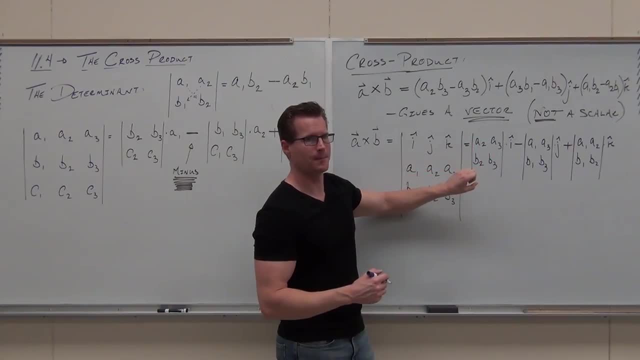 If you did the determinant, come on, stick with me here. What numbers would you multiply? A2, A3.. Minus, Minus A2, A3.. Boom, boom, i Done Done. Now wait a second. 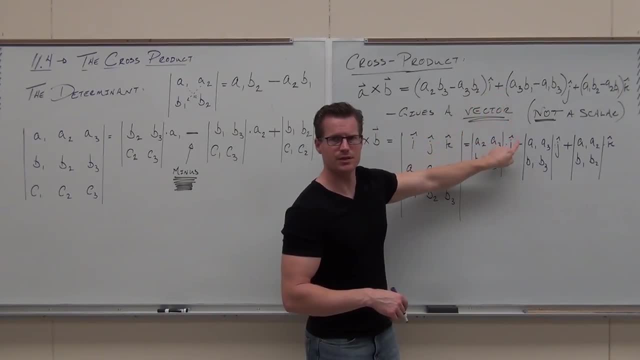 Why this difference? Let's do it: If we multiply, what would you multiply here? A1, B3.. Minus, That's there. Minus A3, B1.. That's there. They're out of order. That's the reason why we have the minus. 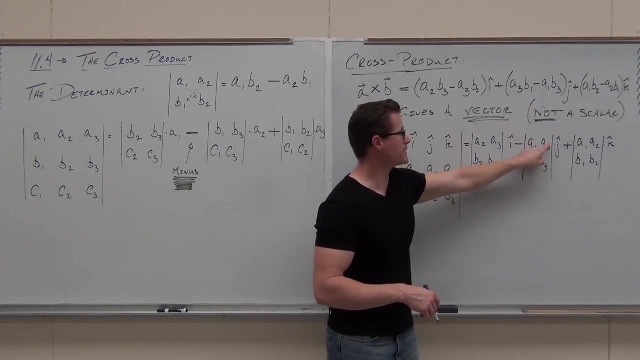 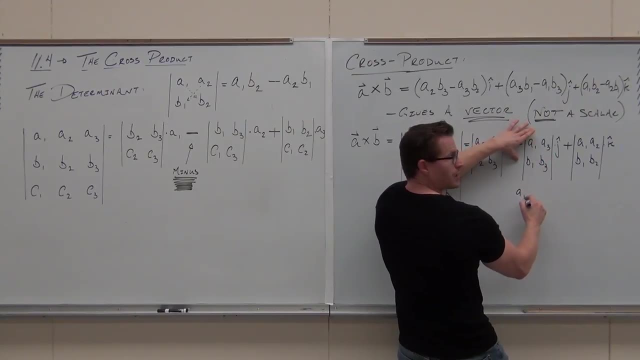 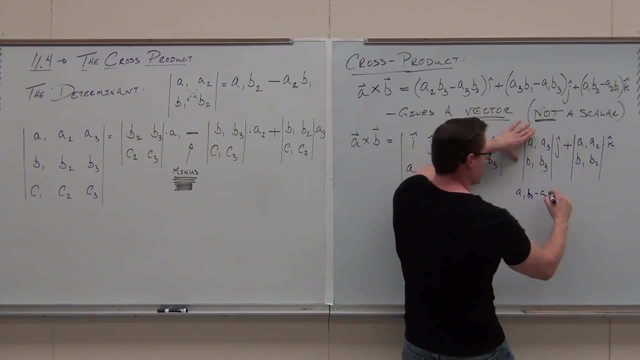 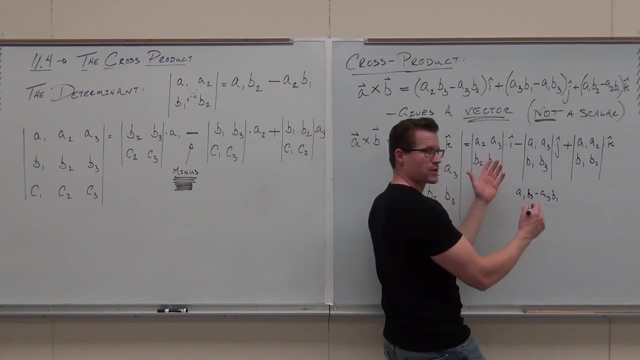 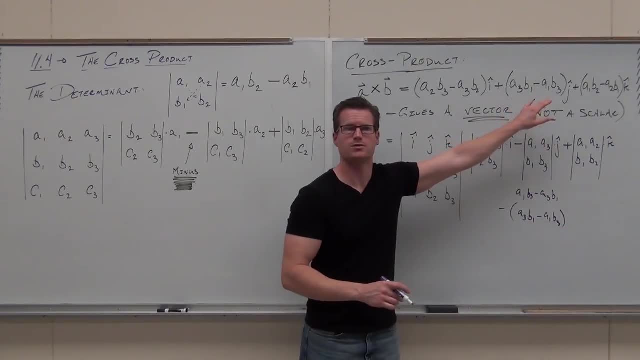 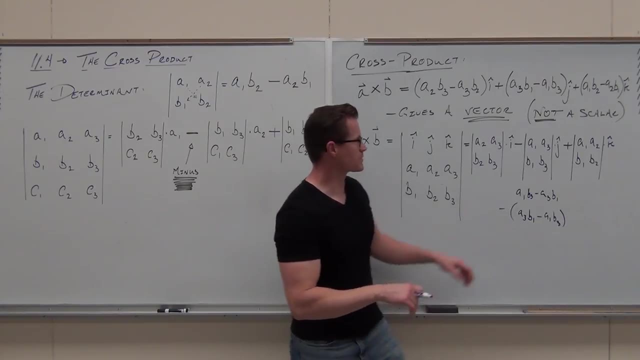 then I get what I want, and that's why we change the plus to a minus, because they're out of order, because the determinant puts them out of order. That's why Does that make sense? Last one's pretty easy. Last one says, yeah, hey, A1, B2, Minus A2, B1, K, and that one works just fine. 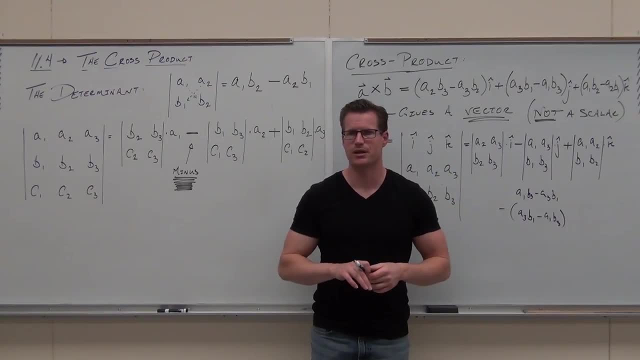 So that's why we get that minus right there is because the nature of that determinant. I'm sure Vince will be okay with the idea behind it. When you're factoring those for negative, you still have a negative on the inside, Just like we had there. 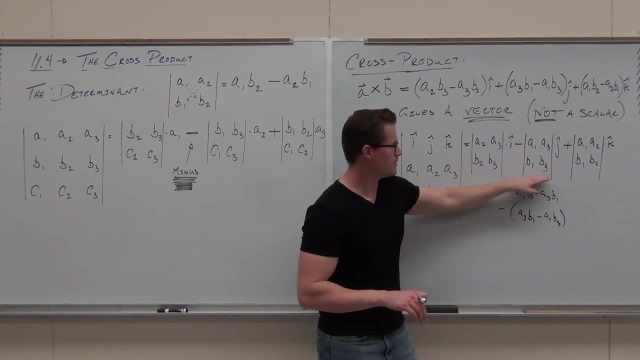 We're trying to make the determinant. this match up with that one. To make it match, you have to factor out that negative, And when you do that, that plus becomes that minus. That's what we have, And how do you match it? 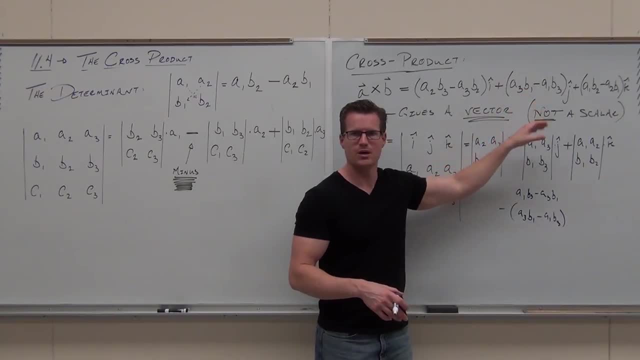 No, you don't have to do anything. What I'm telling you is that these things are equivalent, because when we put the minus there, it automatically makes the reverse order fit. You don't have to do anything, Don't factor nothing. I'm proving it for you. 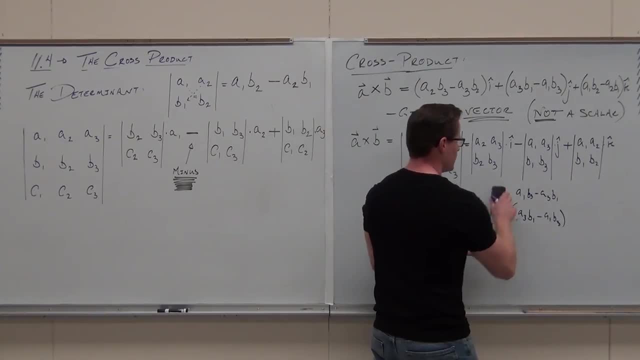 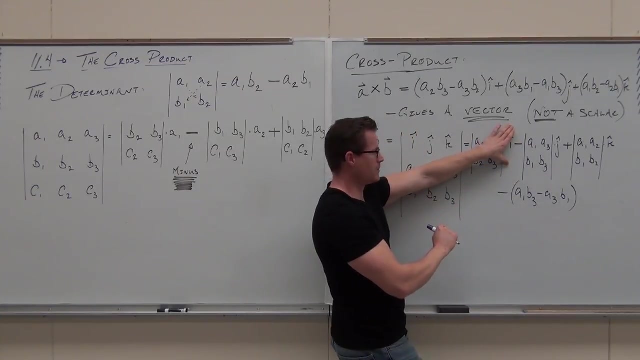 I didn't make it make sense. I can tell by the looks on your faces. Okay, so you go. okay, watch, I'm going to spring on the minus. okay, I'm going to do the determinant. That's literally what we have right now. right, 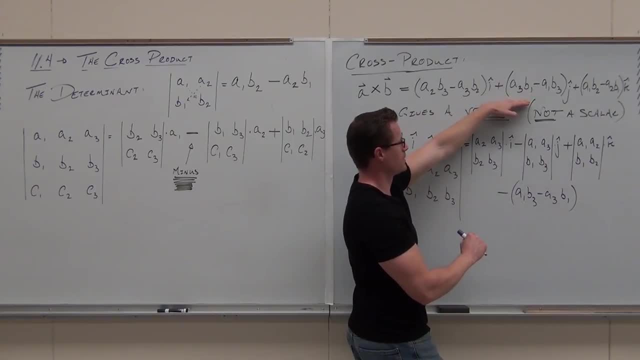 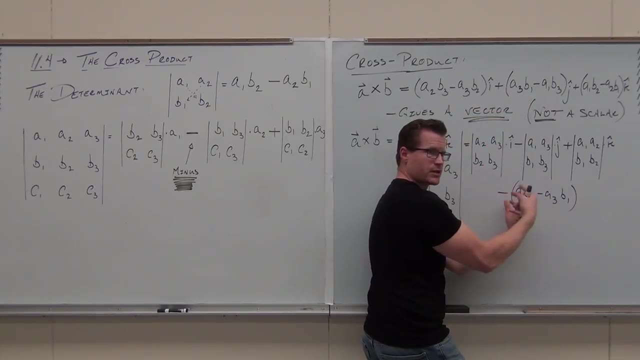 But you go, wait a minute. Is this the same as this? The answer is well yes, And I can prove it by doing this: If I reverse the order and factor a negative, here's still the minus, Here's the factored negative. 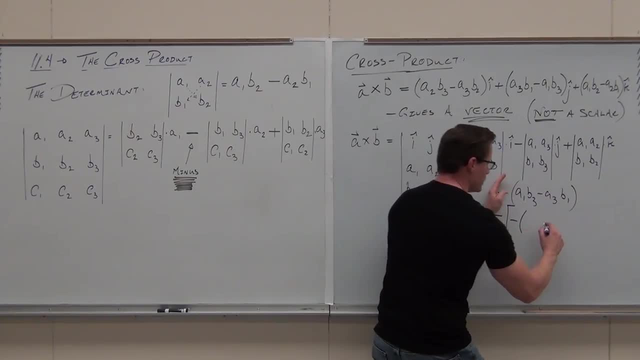 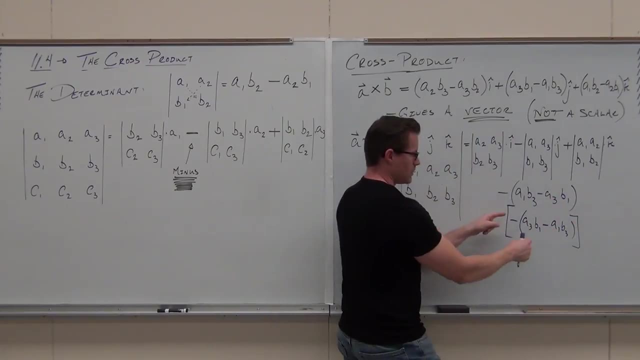 This would change to a. let's see, that would change to a negative. This would change to a positive. If you want to just distribute this, am I confusing the heck out of you? No, I don't know. Yeah, It's the same. 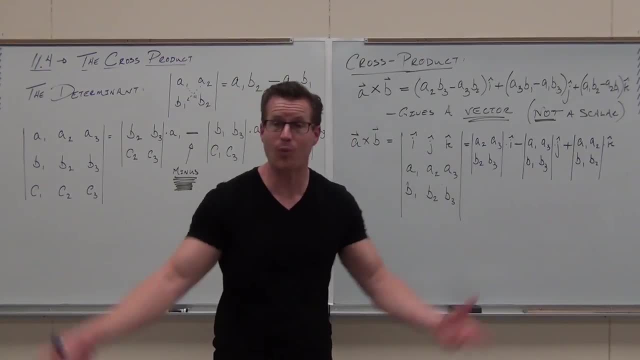 Got it, But what is it? What is this? What is that? A vector? Yeah, it's a vector, That's great. What does that vector look? Well, okay, let's you know what. Let's write them all down. 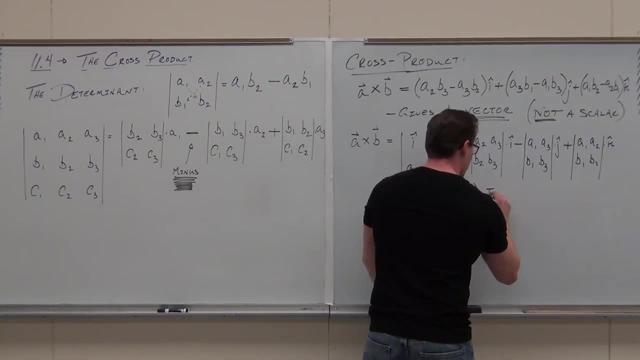 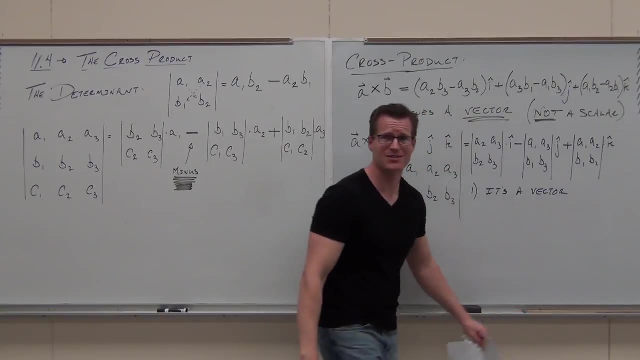 So what is this number one? It's a vector. Hey, that's a big deal. You're getting a vector out of this. It's not a scalar, It's a vector. Okay, What's the vector do? This is the important part. 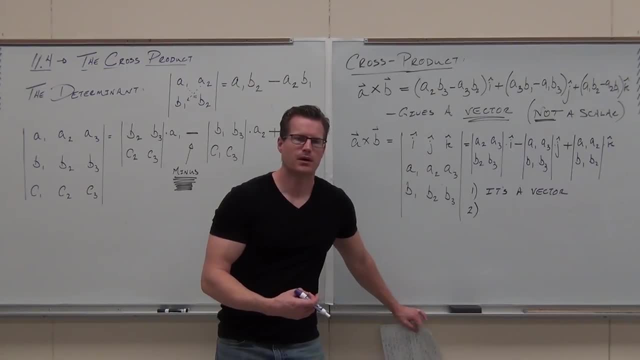 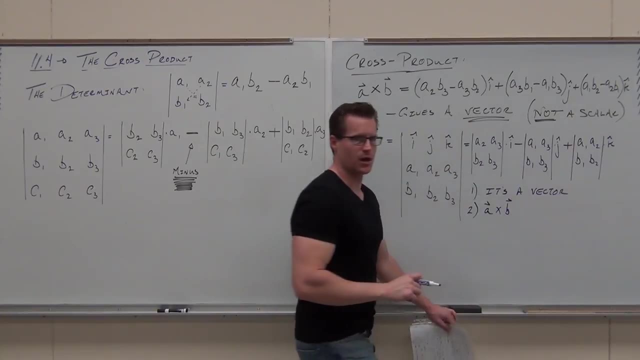 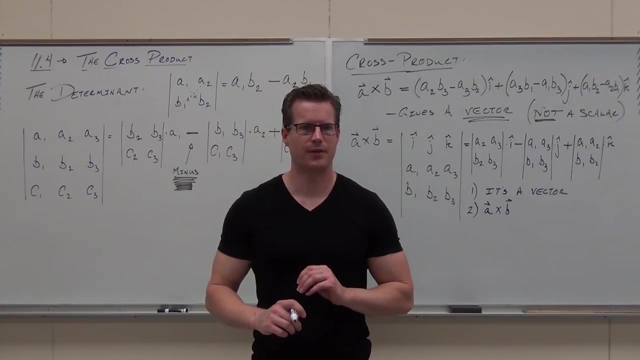 What this creates. this is the awesome part: A cross B. That's how you say it. by the way, A cross B, It's obviously a vector. It's a vector that is orthogonal to both A and B. That's what this vector does. 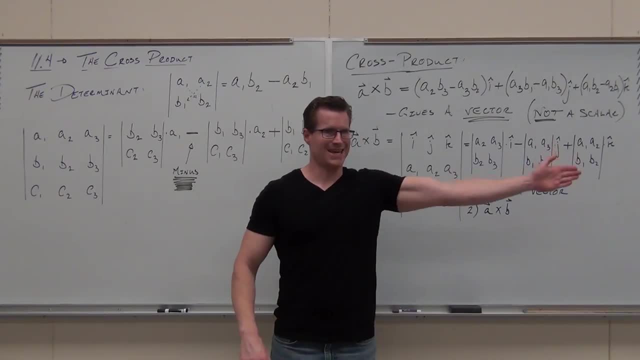 So if you have a vector A and you have a vector B, we have a vector that's orthogonal to both. Where they meet goes right through my head. My neck bone is connected to the shoulder bones at a point like this, right, If I think of a vector that's orthogonal to both. 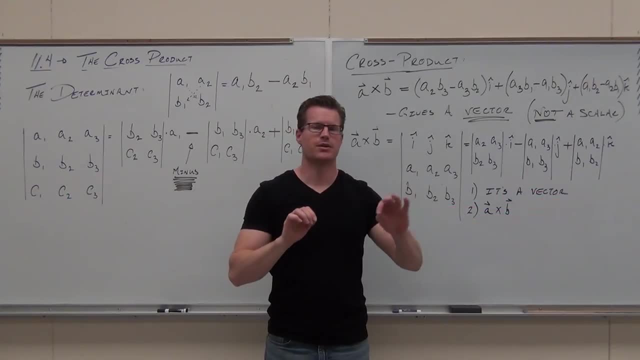 of these guys. it would go right this way. How about this? The Z axis is orthogonal to both the X and the Y axis, correct? If you cross I and J, you're going to get K. I cross J is going to give you a K, the vector that's orthogonal to both. 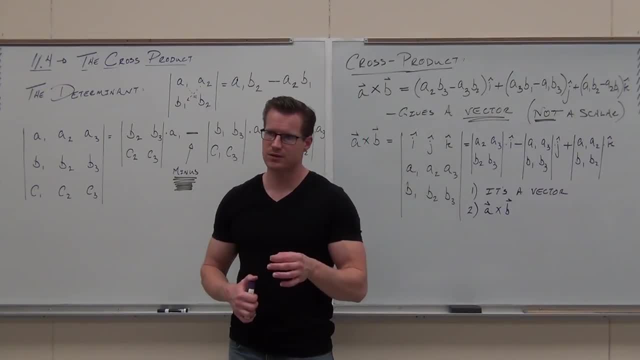 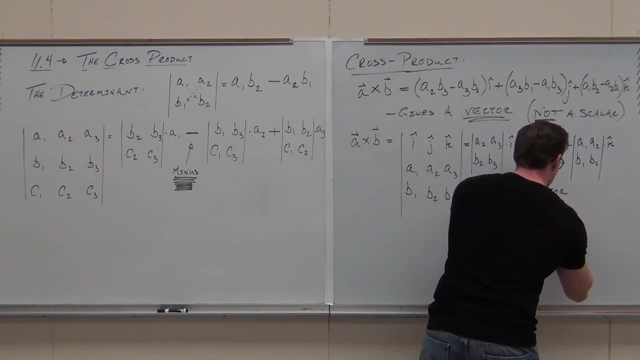 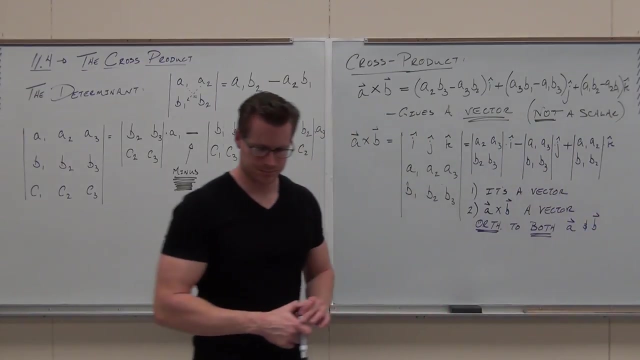 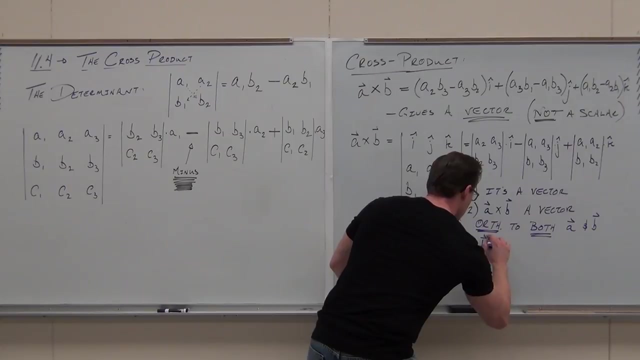 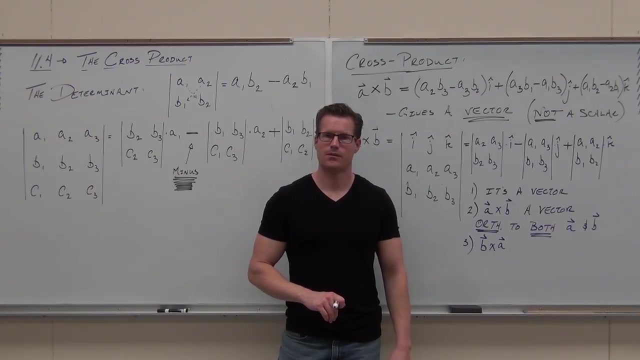 That is going to happen. So A cross B is a vector that is orthogonal to both A and B. But wait a minute. What would B cross A? be Same or different? what do you think Is it still going to give you? well, 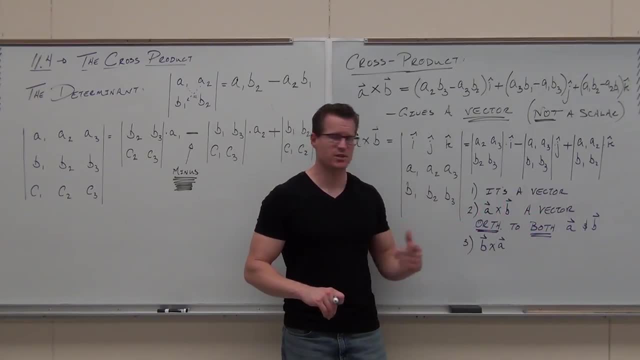 we have a definition right here. I'm going to prove it in just a bit: A cross B, it's a vector, It's orthogonal to both of them, right? So, which means A, I and J gives you K. That's if we went. 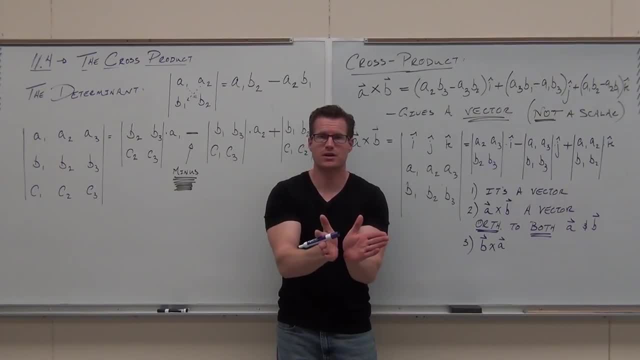 from I to J. What if we go J and I? Is it still going to give you K Yes and no? Does it still have to be a vector that's orthogonal to both of them? It does, because that's what a cross product gives you. 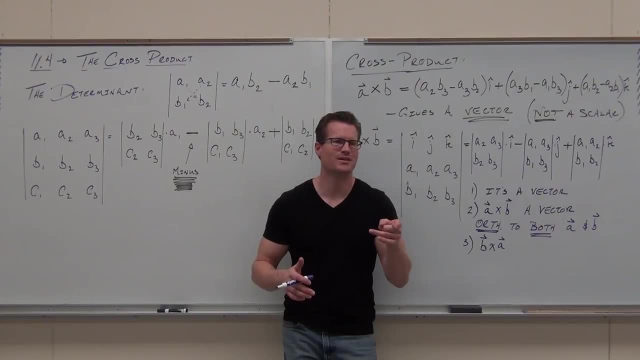 Is it in the same direction? No, That's what it does. So if I reverse the order, it's no longer positive K, It's just negative K. It still has to give you a vector orthogonal to both, but it's in the opposite direction. 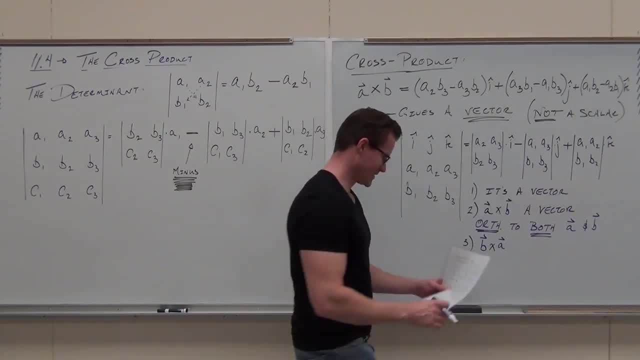 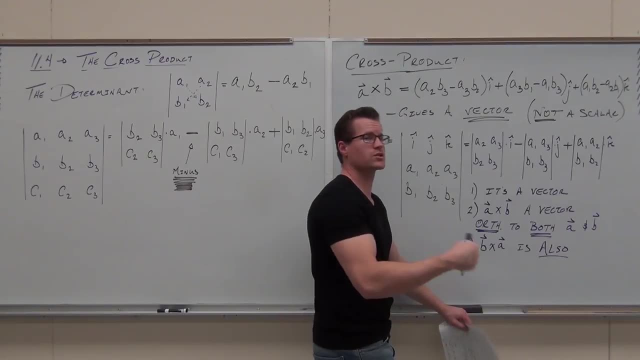 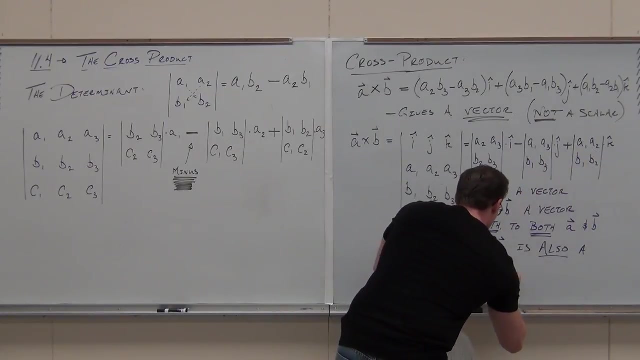 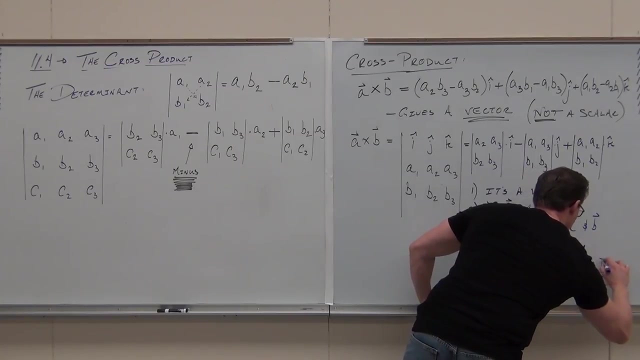 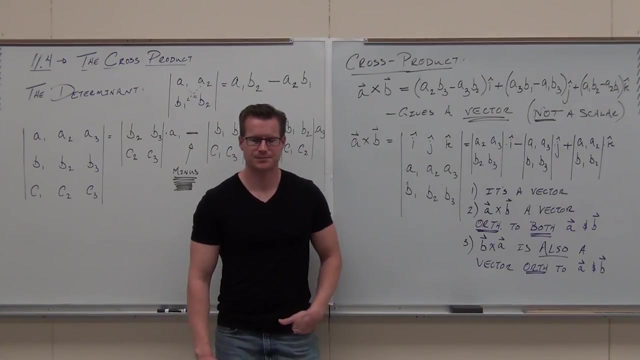 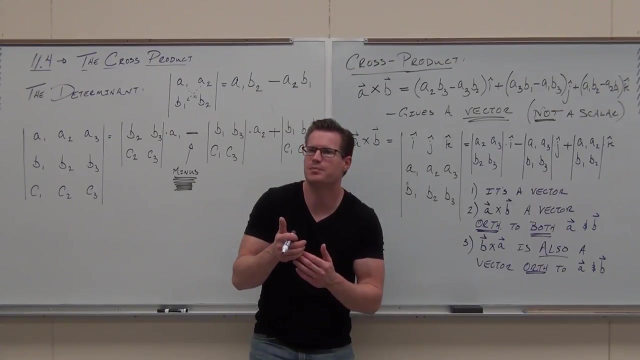 Does that make sense? That's kind of cool. This is also a vector orthogonal to both A and B. If they're the same, if they're both orthogonal but they're not the same. you can't be like both be orthogonal to the same two vectors and not be going in the same direction. 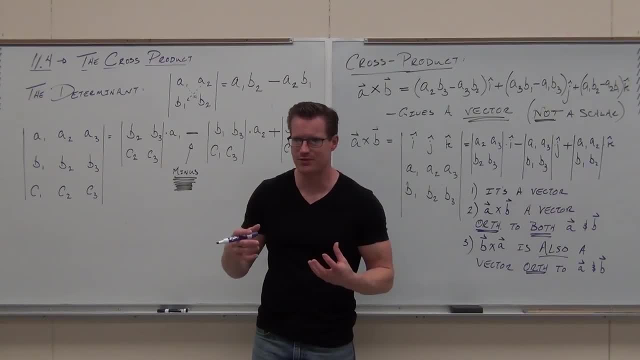 not have the same unit vector. So they're the same size vector. even They're the same vector but in opposite directions. So they're not the same vector, But one is just negative of the other. That's what happens, And that's the last thing we're going to write. 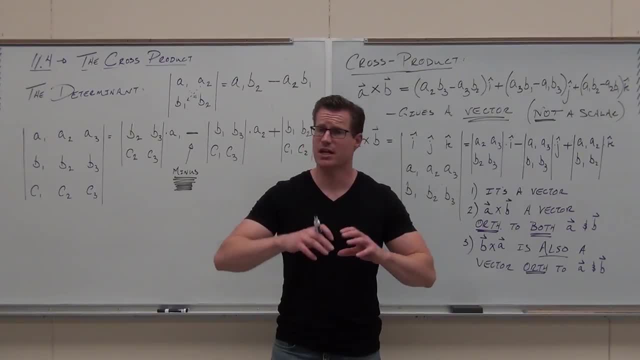 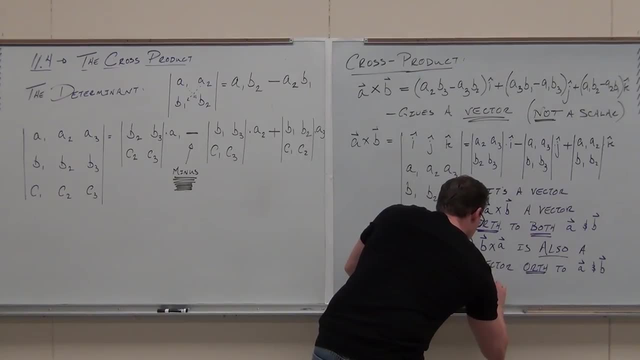 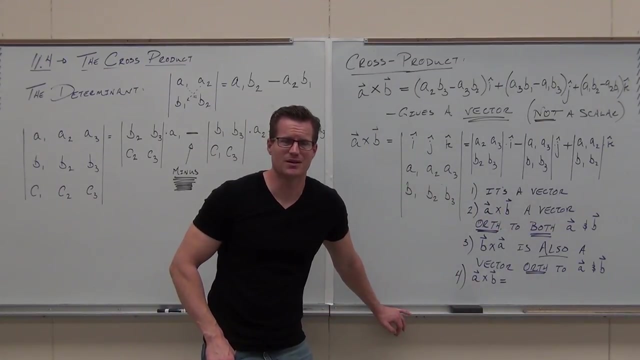 So A cross B and B cross A. they're the same size vector, but they're in opposite directions. I'm going to say it this way because I'm saying the same thing. Here you go. Hopefully you see this. Here you go. 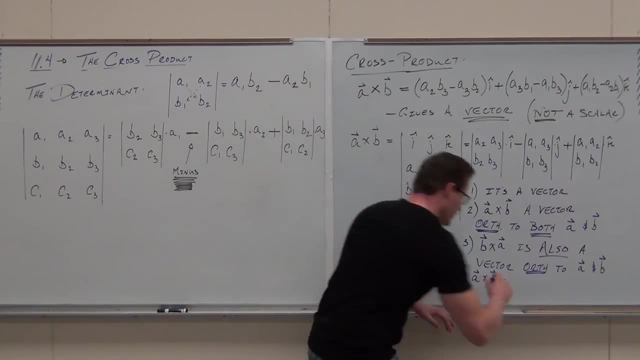 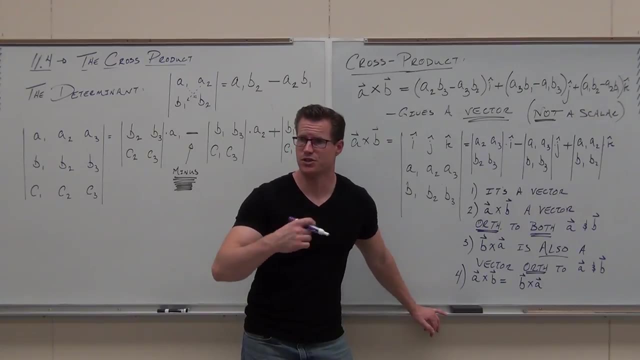 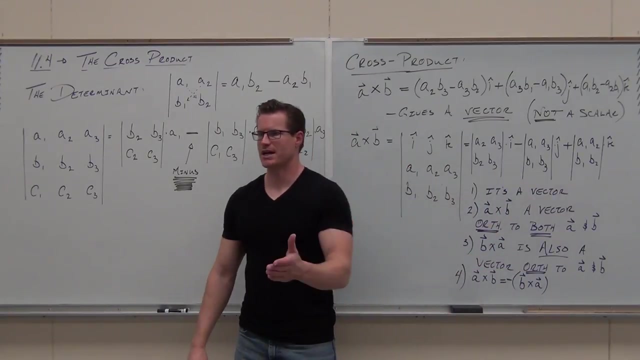 This is the same thing. I said that A cross B and B cross A are the same size vector, but they're just in opposite directions in mathy ways. We say that like that One is just negative of the other, because all that does is flips the direction. 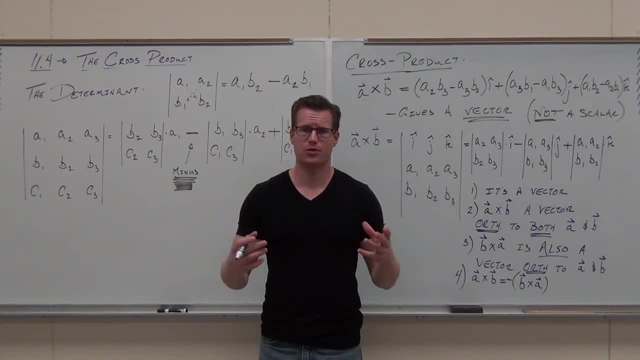 It doesn't change the magnitude, It doesn't change the fact that they're both orthogonal. So if you're okay with the idea, I'd like to draw you a picture to make sure that you really, really do get it. I'm going to do it right here. 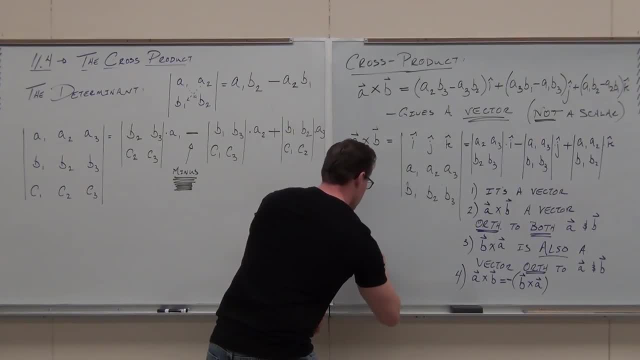 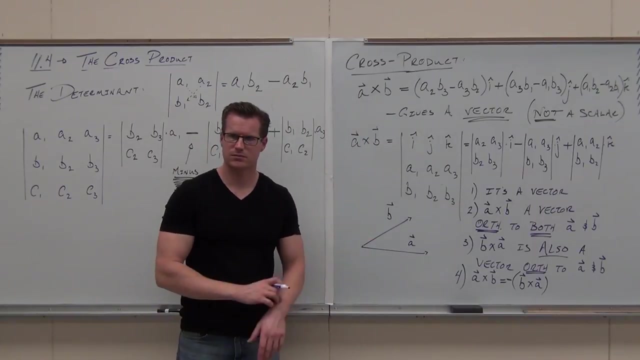 I'll show you. So let's say that's vector A and that's vector B and there's obviously an angle between those vectors. We'll make a little attribute. So A cross, A cross and A cross. Here's a couple things I need you to know. 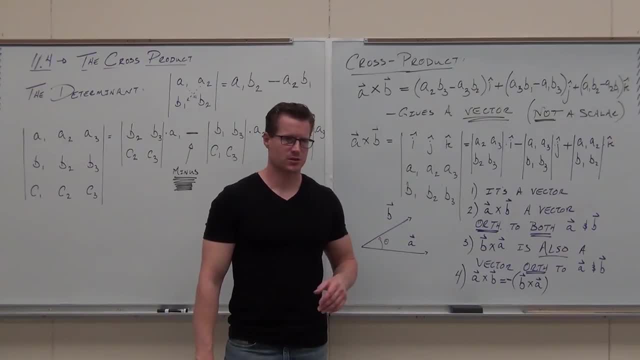 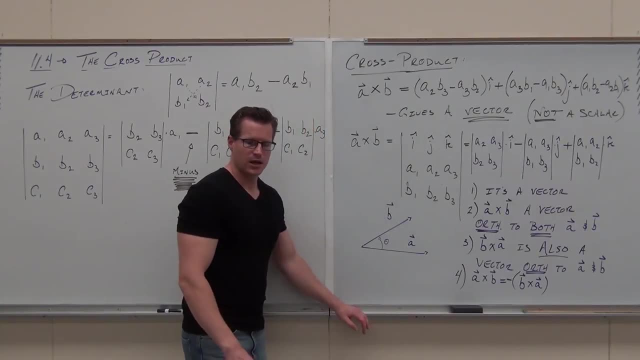 Firstly, the representation of what A cross B and B cross A means What I want you to do. just imagine this right now. I'm going to actually do it. If we are talking about A cross B, what that means is we're going. 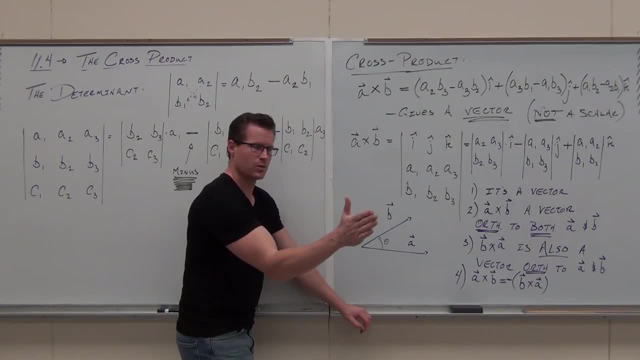 to put our hand. we're going to put our hand with the palm side towards the vector we're crossing, So put your hand like it's on A, with your palm side open towards the B. Does that make sense? Seriously, do it? 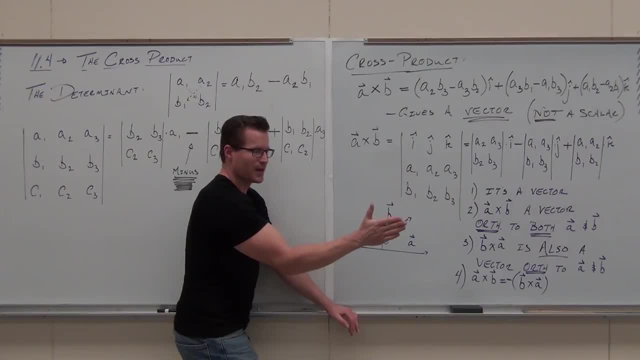 You're looking at me like I'm an idiot right now, Seriously, try So. it's like this: Now close so you don't have a thumb right now. all right, Close your hand so that A starts going towards B Does. 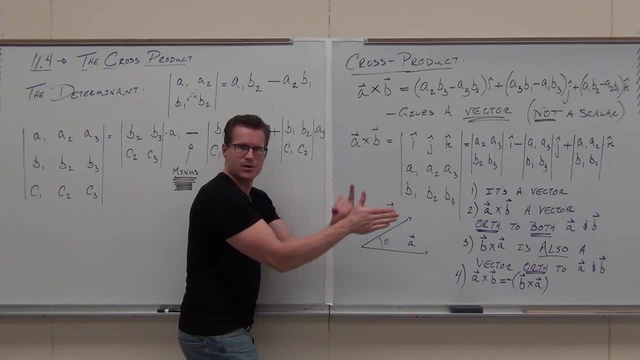 that make sense. If you do that, your thumb is pointing up. Do you see what I'm talking about? Where your thumb is pointing is where that cross product vector goes. It's called the right hand rule. So if we put our hand on A palm open, 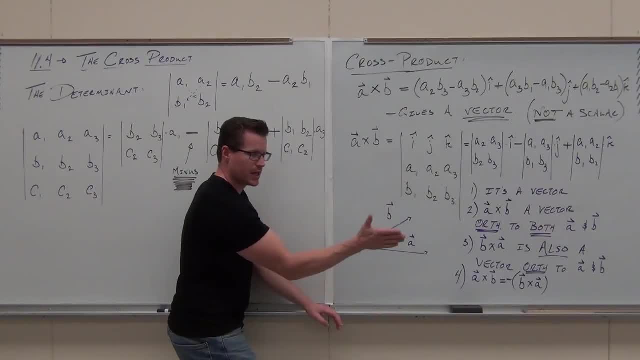 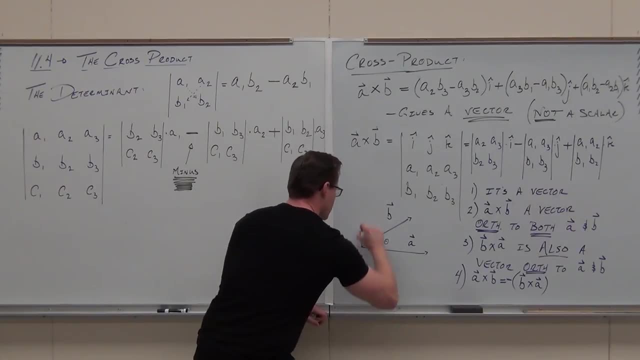 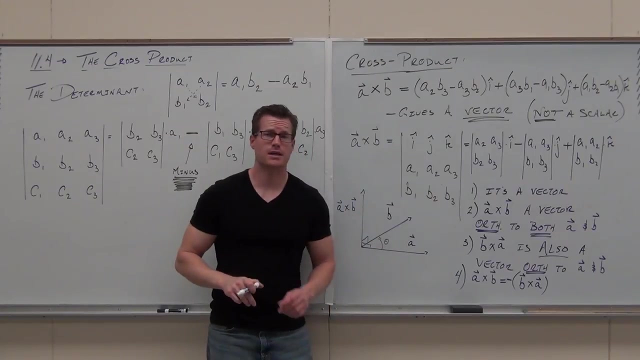 to the vector we're crossing. So A to B, A to B. My thumb is pointing upward, My thumb is pointing this way: right now. This is perpendicular to both A and B. That is, A cross B. Now you're like: well, wait a minute. 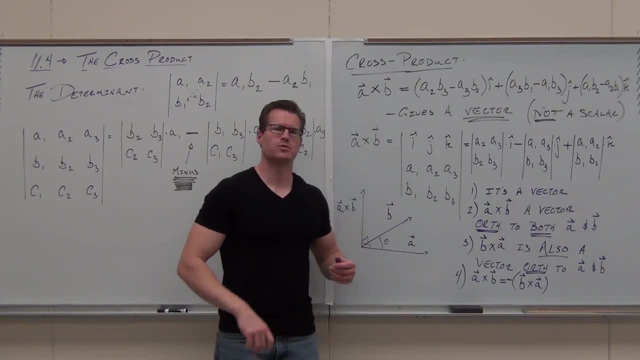 How is B cross A any different? Well, do you guys have flexible shoulders? That's what I need to know right now. I don't. So here's how you have to do B cross A. You have to put your hand on B with your palm open towards A. Eh, 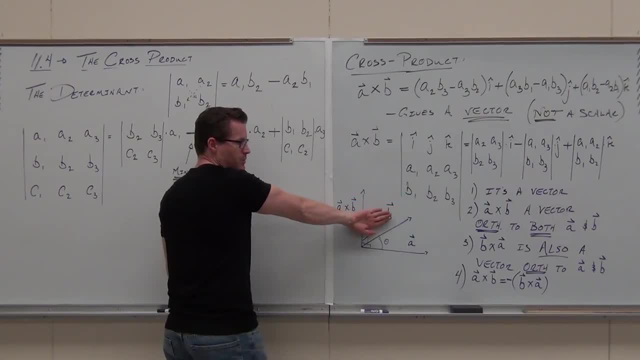 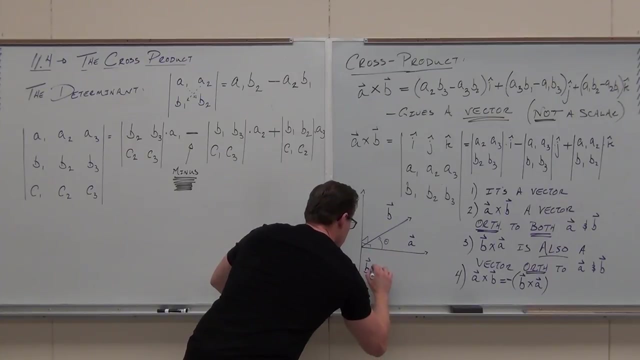 No, Eh Yes. This is on B. palm opens towards A. When I close that from B to A, my thumb is pointing downwards. That's where B cross A points. Hold on a second. One more thing, One more thing. 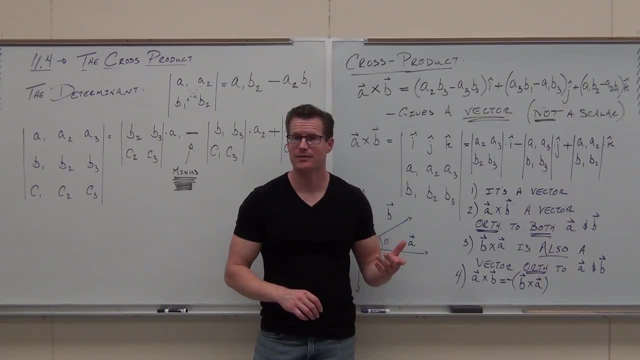 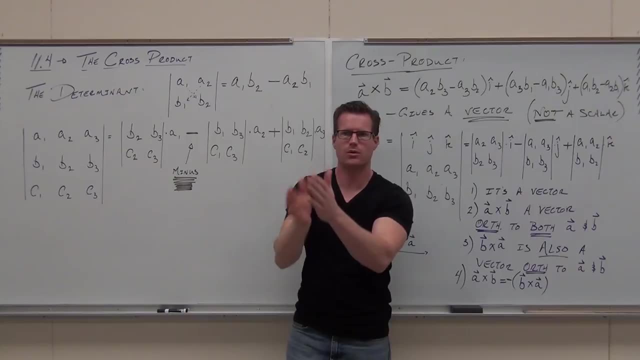 The angle here. you can't go any past pi, Your finger doesn't go, you can't close your hand past pi. Okay, So because you get there the other way, You don't want to go past pi because it would be easier. 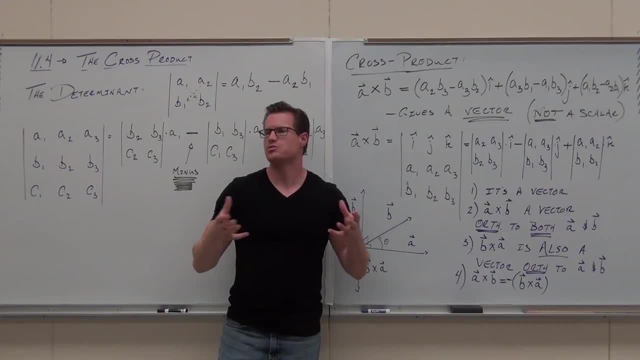 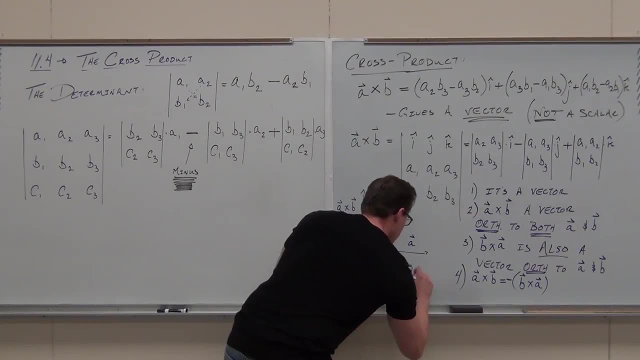 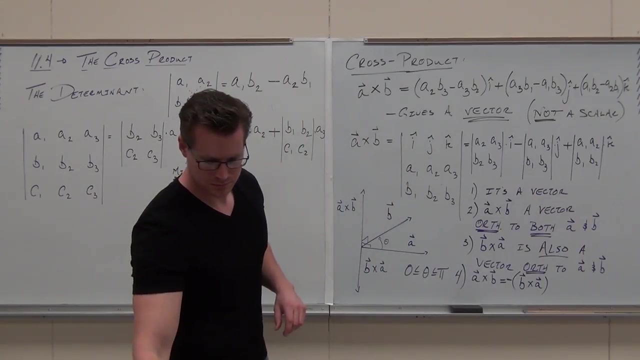 to cross product across the smaller angle. Does that make sense to you? So So we're never going to go past 180, never go past 5.. So this is defined for that. I really want to know if I've explained this well enough for you guys. 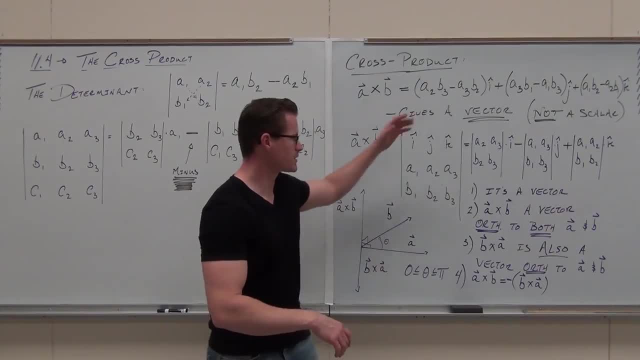 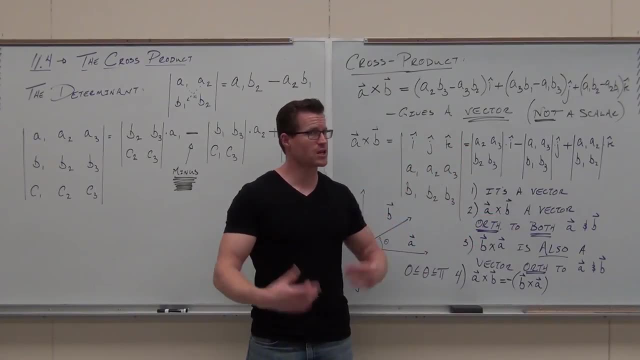 to understand the concept behind it. There was a lot behind it. I could have just given this and said that's cross-product, But we talked about this. We talked about what determinants are. We have not done one yet. I understand, like if you're seeing this for the first time. 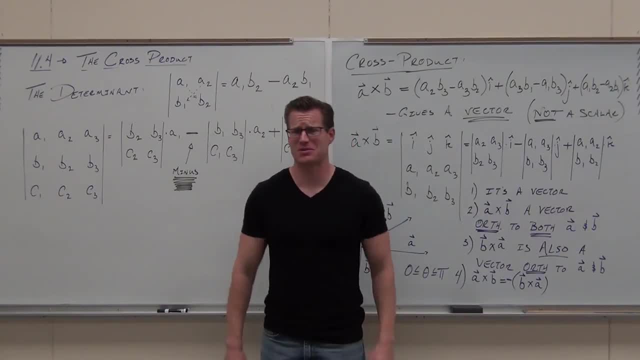 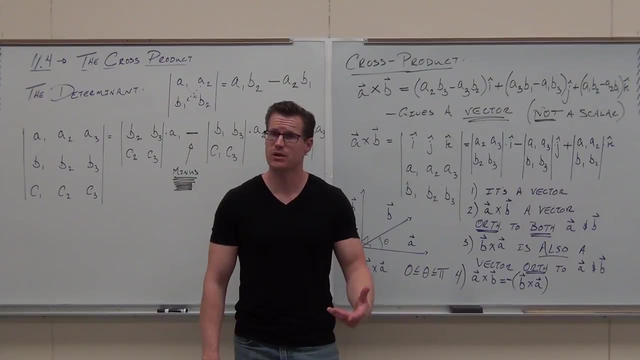 and you're going. that looks like a whole lot of work. Please just let it stick with the dot product man. That's easy. This is just as easy. I promise It's not hard. We're going to do a couple examples in just a little bit. 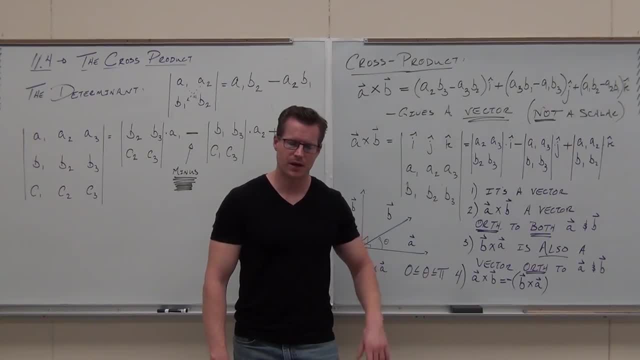 Do you want to see the proof of? you know what I'm going to hold off on the proof. If you want the proof that this vector and this vector are perpendicular to both, I'm going to do that when we finish our examples. 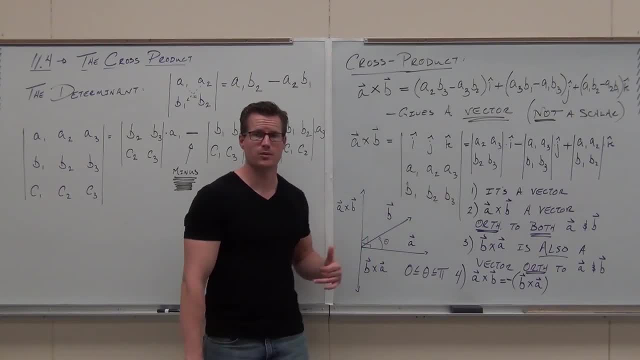 Right now I want to get to our examples. Does that make sense? So we're going to do this proof a little bit later. I won't leave you. You hang in. We're going to do that in well, like two hours. 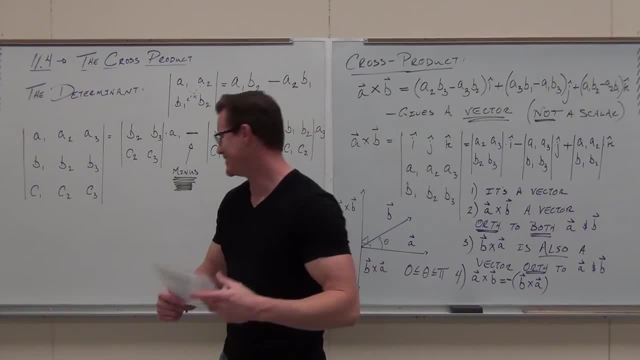 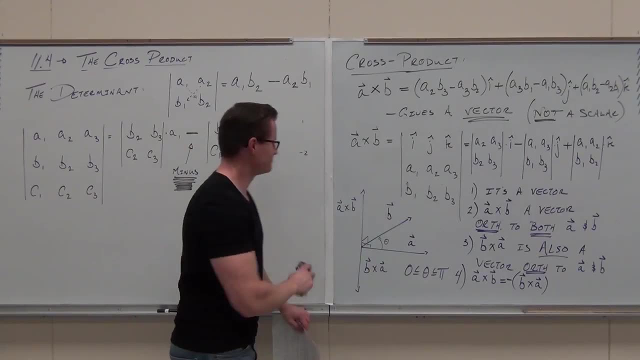 But it will be on there. So you're going to have to look for it later And you can remind me, because I'm going to forget. You're not going to remind me, are you? No? Thanks guys. Thanks a lot. 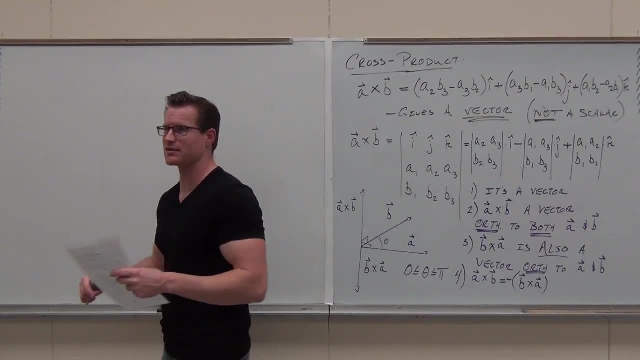 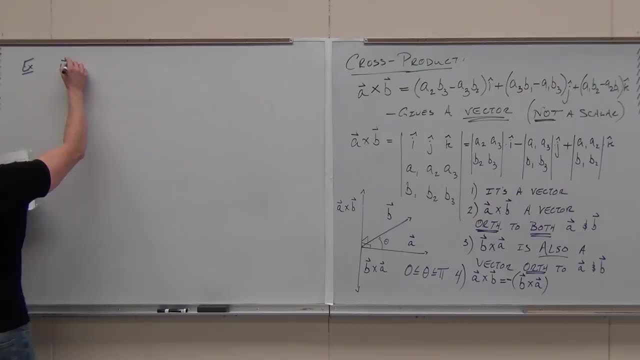 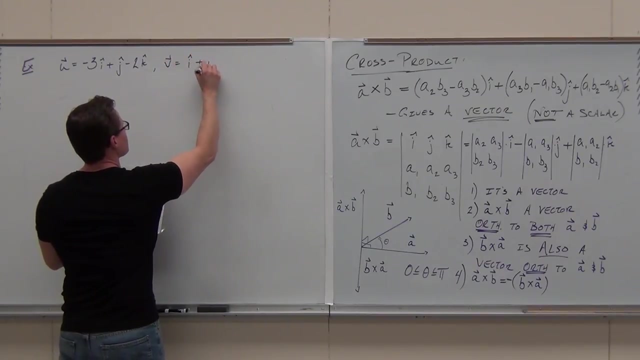 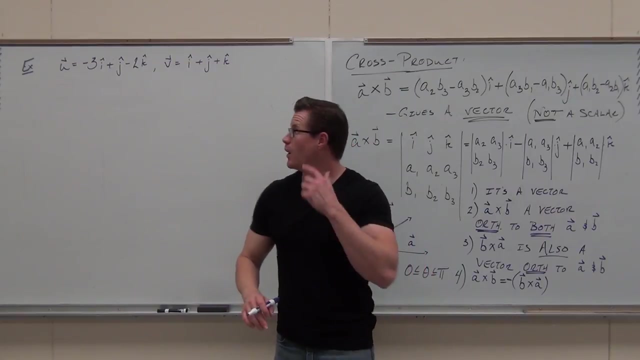 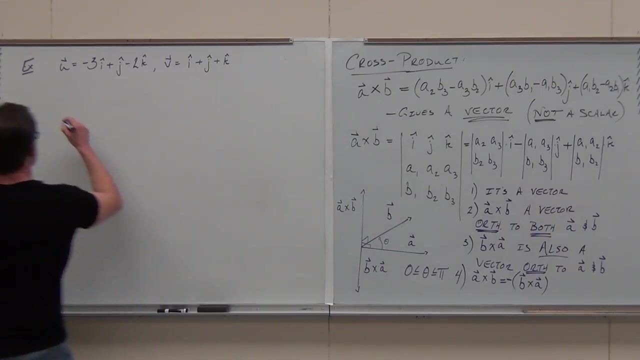 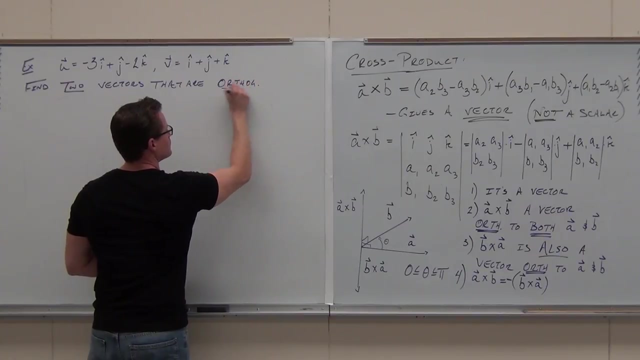 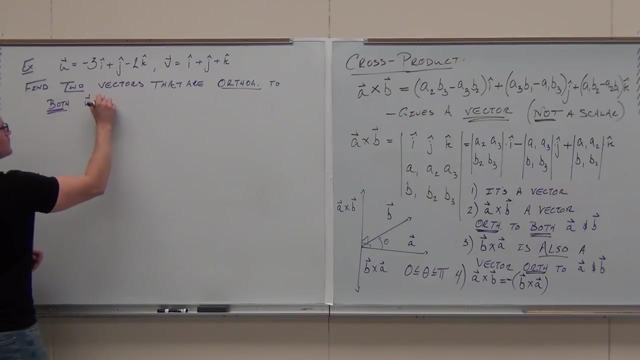 You want a test question? Yes, sure, Almost guaranteed. Here's the test question. I want you to find two vectors, Two vectors that are orthogonal to both U and V. Here we go, Is that all right? Write it down, then look up here. so I know you all have written it down. 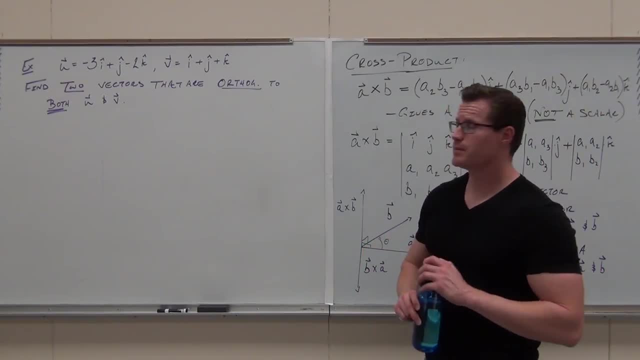 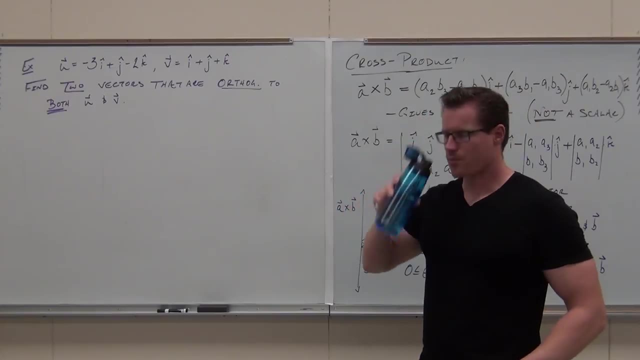 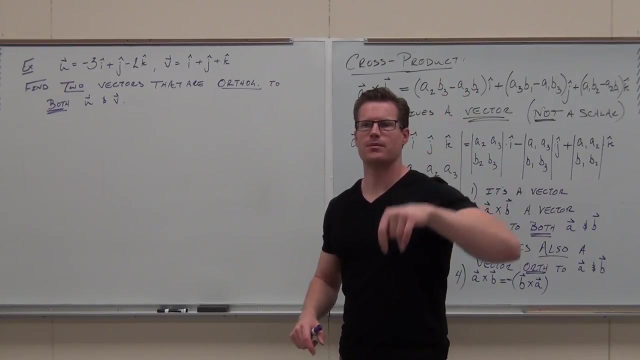 I can talk at you, okay. So we've got U, we've got B. Make sure you're writing that correctly. We want to find two vectors that are orthogonal to both of them. Okay, rapid recap: What's the dot product give you? 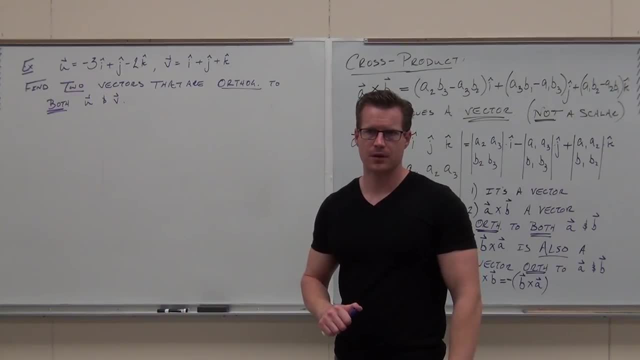 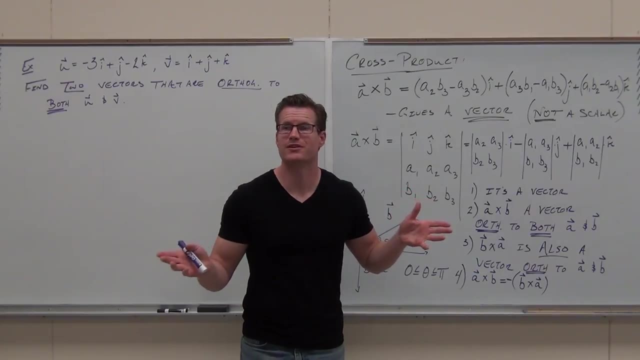 Vector, or scalar, Scalar, What's cross product. give you Vector, Vector that is Orthogonal To A Or whatever two vectors. I give you. So when I ask you, find a vector that is orthogonal to two vectors. 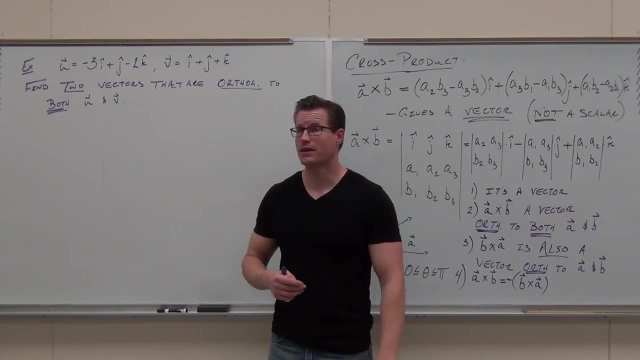 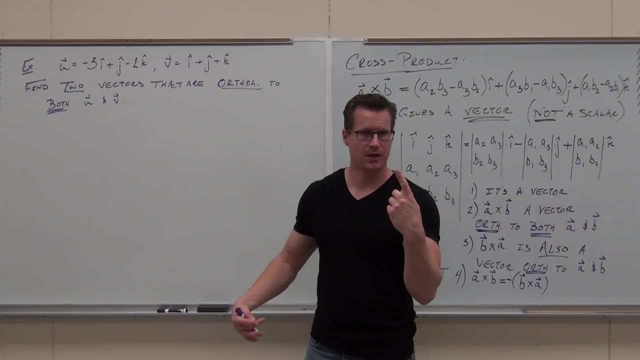 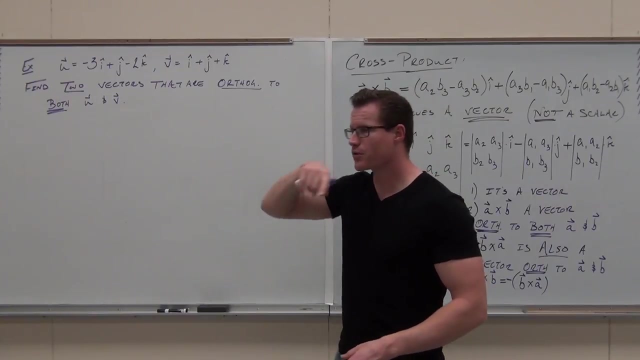 what am I really asking you? Cross product, That's all I'm asking you. So whenever we do the cross product, we are finding a vector that is just orthogonal to both the given vectors. So let's try that. Let's find a vector that's orthogonal to both U and V. 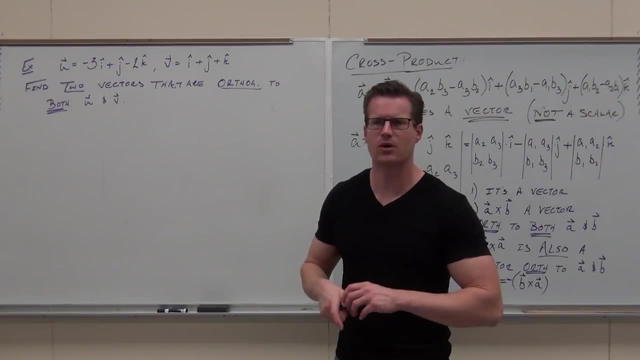 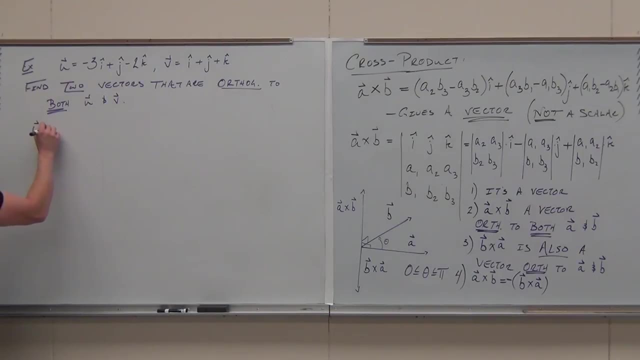 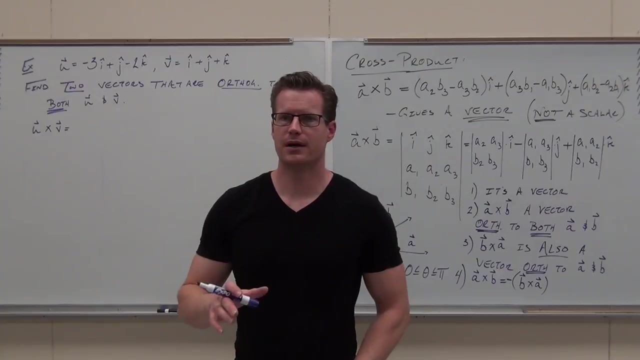 Let's find one of them and then go from there. Does that make sense? Let's find one of them, So let's, Let's cross U and V. Here's the way you set this up. The order does matter. I said: hang on to that question in your head until like right now. 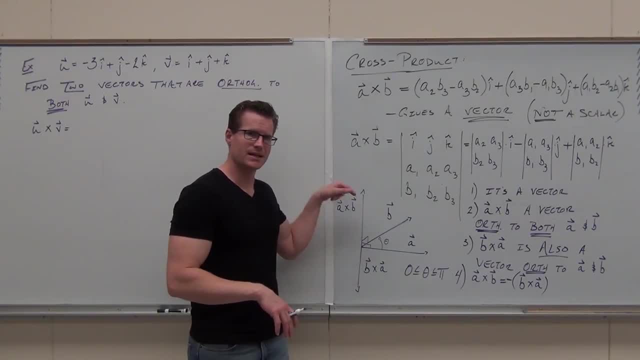 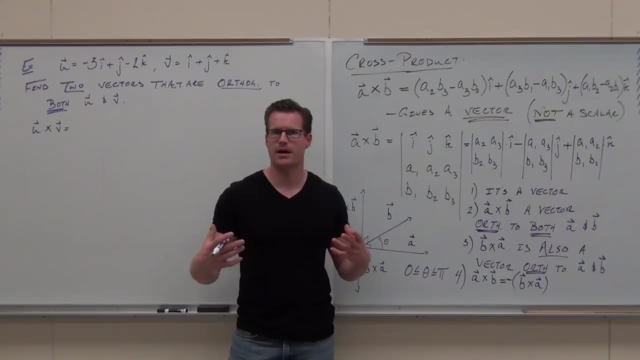 Here's why the order matters. If I do it in a different order, I get a different vector. Does that make sense? This is A cross B, This is B cross A, I get a different vector. Now, in the grand scheme of things, does it really matter? 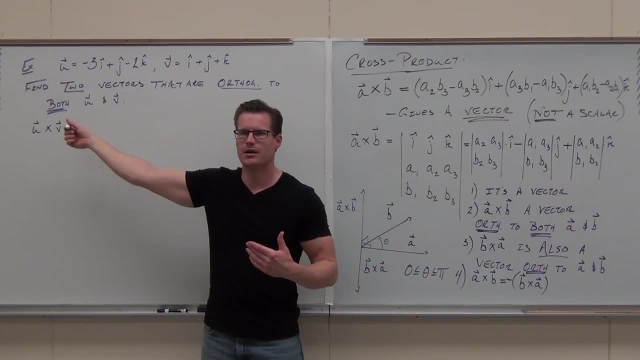 Well, This is the second part of our question. If I wanted you to find two different vectors that are both orthogonal to both of them, well, if I just switch the order, then U cross V is going to give us one and V cross U is going to give us the other. 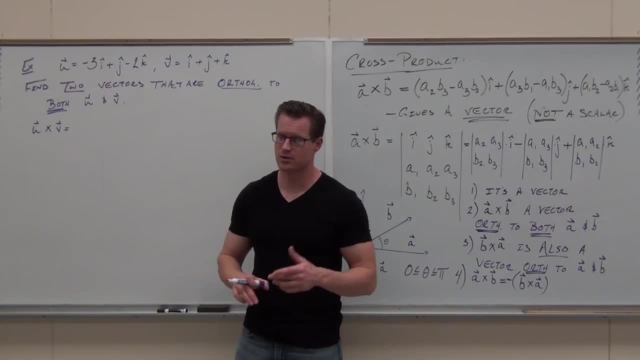 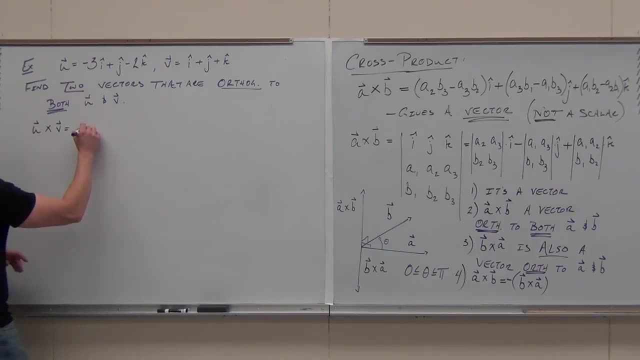 Does that make sense to you? So I'm asking you to do two cross products right here. So we'll try it. The setup is real important. all right, The setup always works the same way, Always, always, always. You put an I. 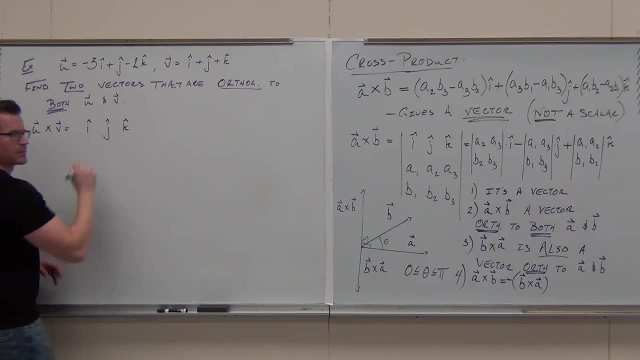 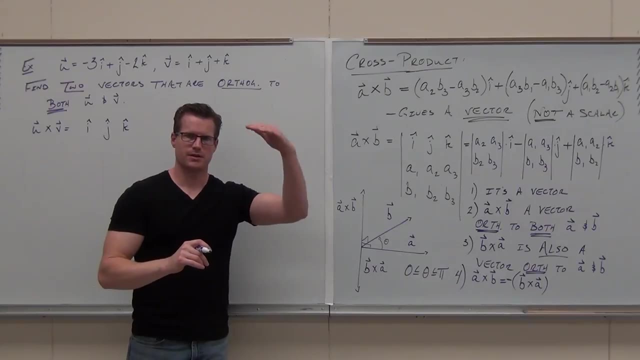 I, J, K, That goes first, because that's the order of our vectors. We put the U components first and then below that we put the V components. Make sure you do not forget signs, Make sure you do not forget the order. 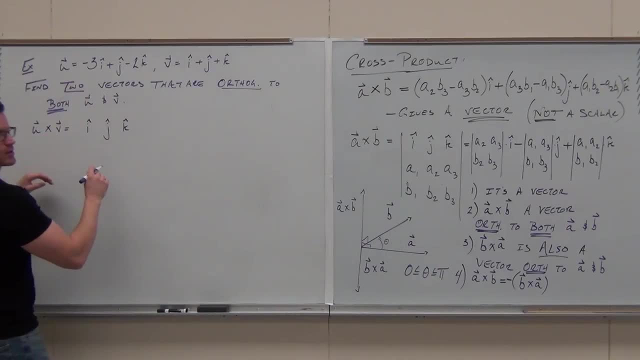 Make sure you don't switch them up in your head accidentally. So for U, tell me the components, Everybody, real quick. what's the components Negative? 3, 1, 2.. Negative 2.. That's it, You got it perfect. 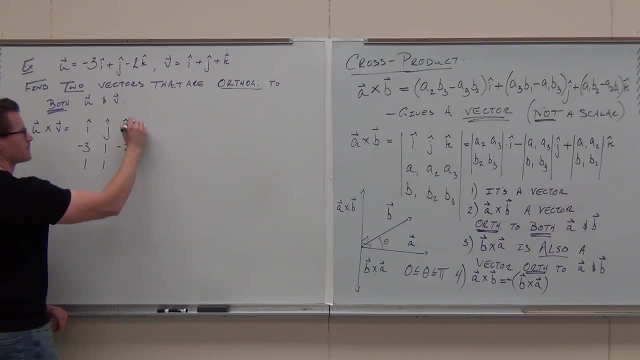 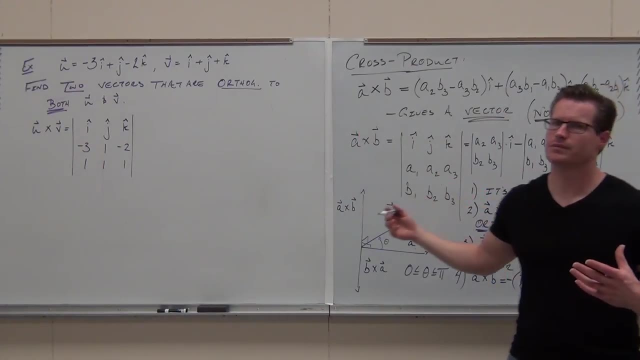 How about for V? Everybody? what is that? 1, 1,, 1, 1.. What is that? What is that? We're going to show that we're making a determinant, And then a lot of this stuff. look, this is a way to do it. 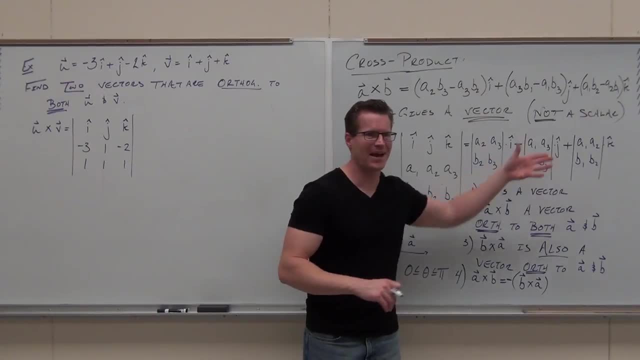 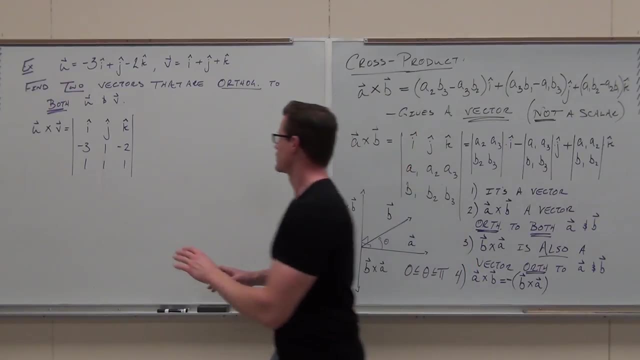 Don't write this. This is crazy. all right, Don't do that. Don't write all that out. Don't write the determinants. It's just telling that you need to do the determinant. So literally, here's what you need to do. 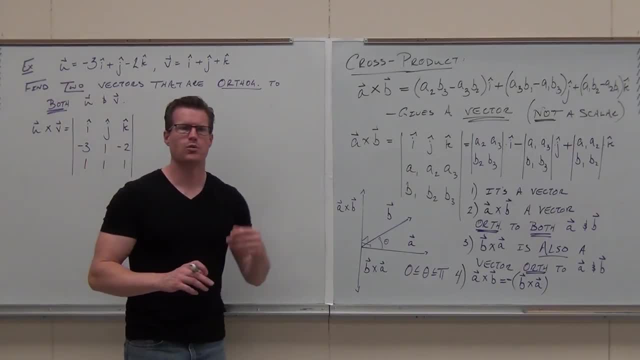 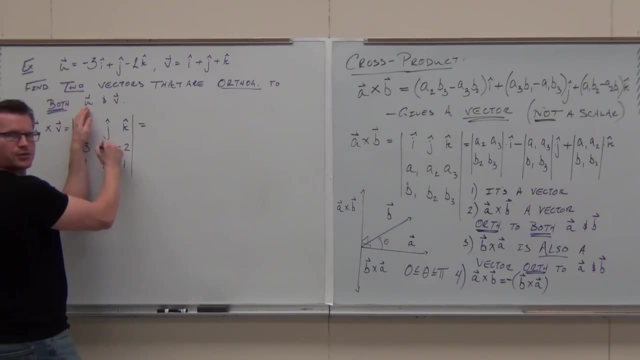 Cover up which one first: I. If you want the, I cover the I. If you want the J, cover the J. If you want the K, cover the K. We want to cover the I. We're left with this. 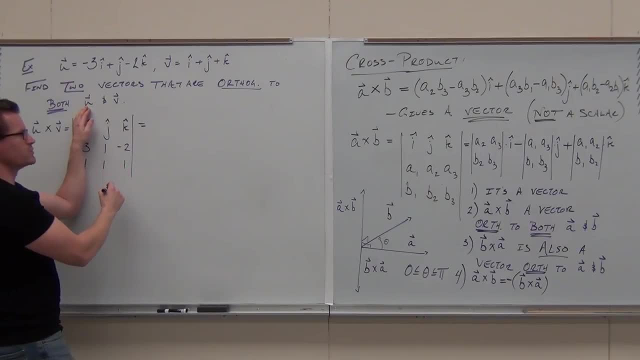 We're left with this square matrices. OK, We're going to find the determinant. What two numbers would you multiply 1 and 1.? What's 1 times 1? 1 times 1.. And then you subtract. This is where you're going to screw this up. 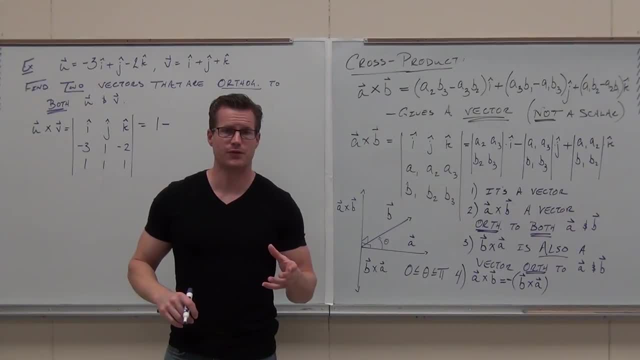 If you're going to screw anything up, it's going to be right here. I promise it's going to be sign errors. Seriously, I've been doing this a while. all right, I still make sign errors unless I do this. 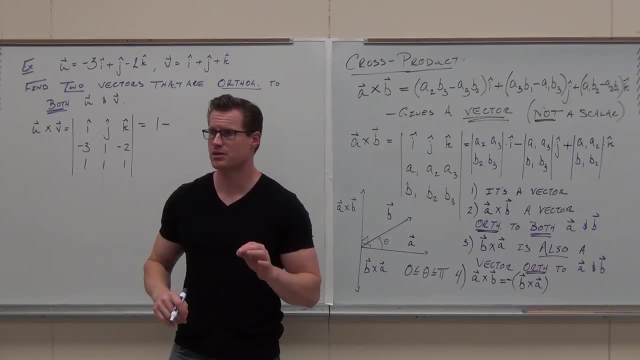 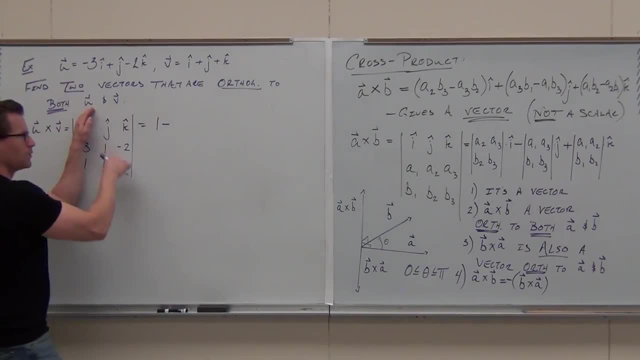 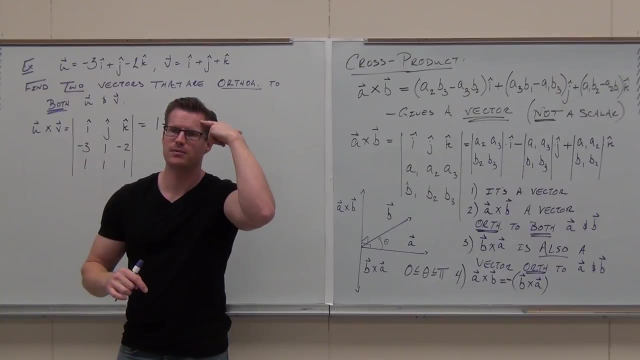 You want to do this. You want to do this. I put 1.. I put minus And I put what? the other one is? This right here, Because your head is going to want to make you think: minus 2.. Trust me. 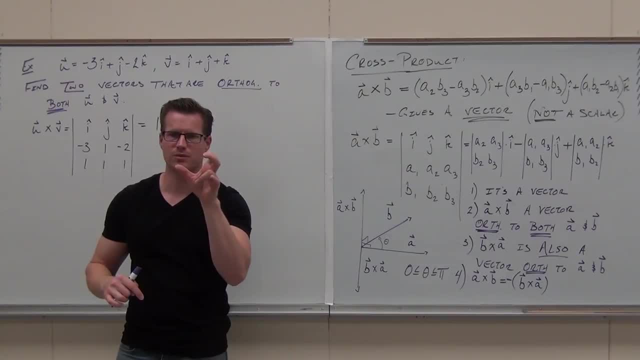 It's going to want to do that. So write down at least those two numbers being multiplied. Can you guys do that? Do it for you, Don't do it for me. Do it for you, It'll save you a lot of headache. 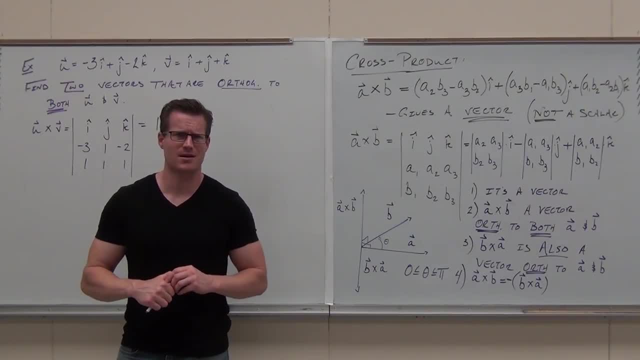 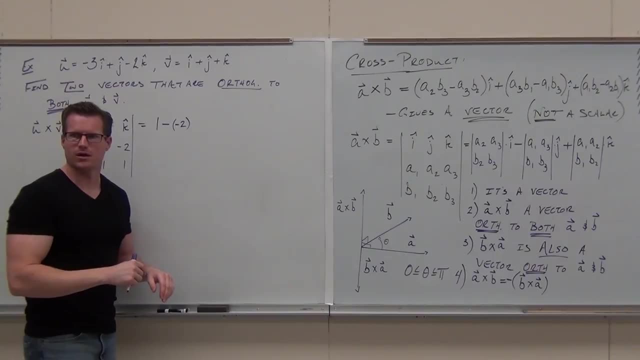 It'll save you a lot of time. I'm saving your life here. all right, Your life is time. I'm saving your life, Trust me. So 1 minus negative 2. You guys get what I'm talking about. That's all you've got to show. 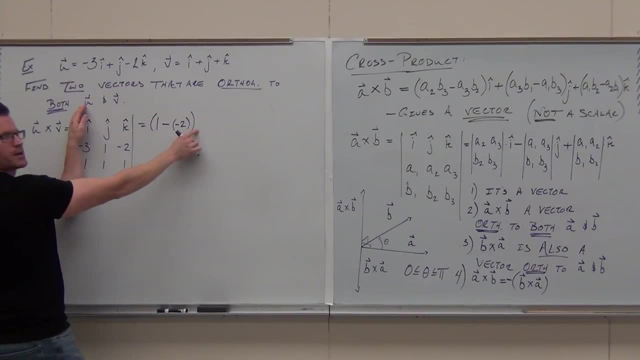 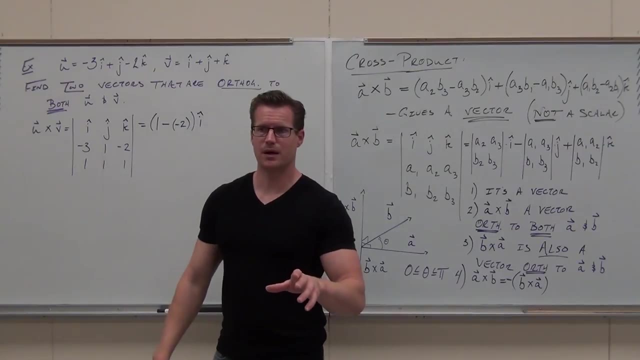 All right. And then what am I going to multiply that by Minus 5. Pi, Yeah, And then we continue. There's a big part. You're going to forget it occasionally, But don't forget it all the time. all right, 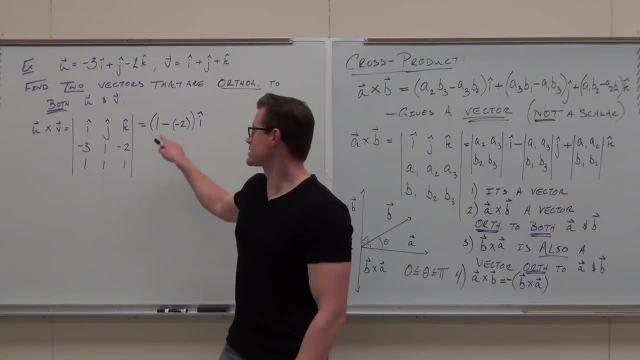 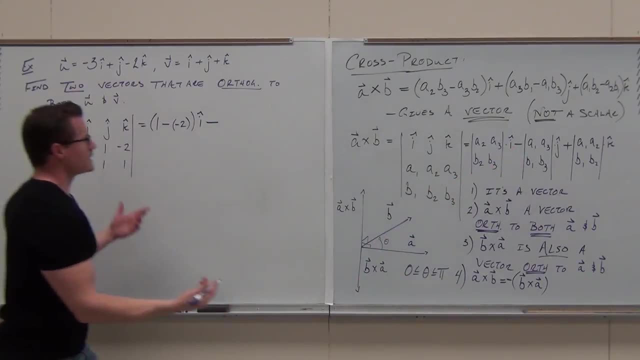 Go back And if you get the wrong answer all the time, you're probably forgetting this next thing. What goes right there? The minus, The minus. It says: hey, if you want the j component of this new vector that's orthogonal to both u and v. 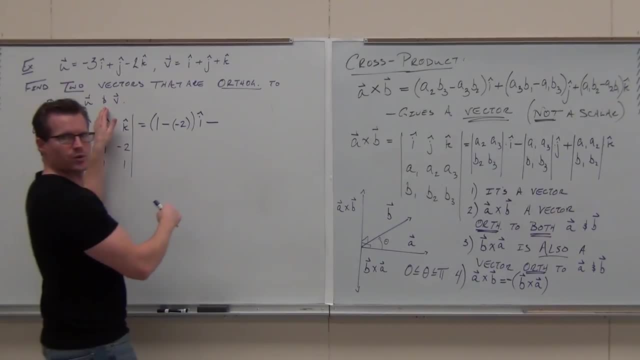 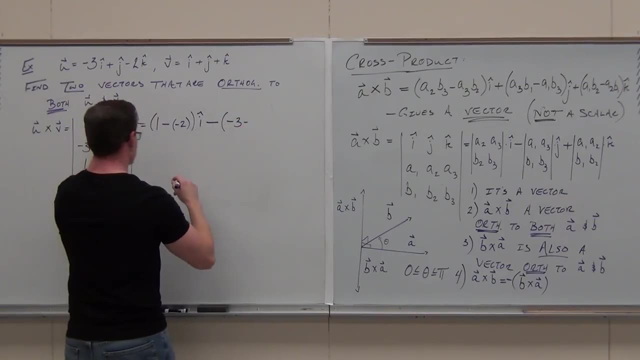 cover up the j. What's the first number we're going to write down, please? Negative 3. Minus. Negative 2. Minus what? Negative? 2. Negative 2. j. Let's make sure I get it right, because there's a lot going on. 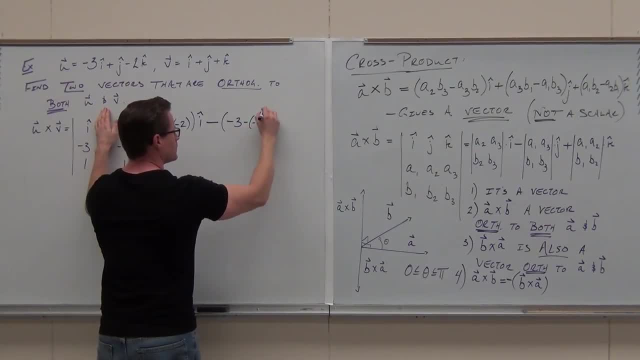 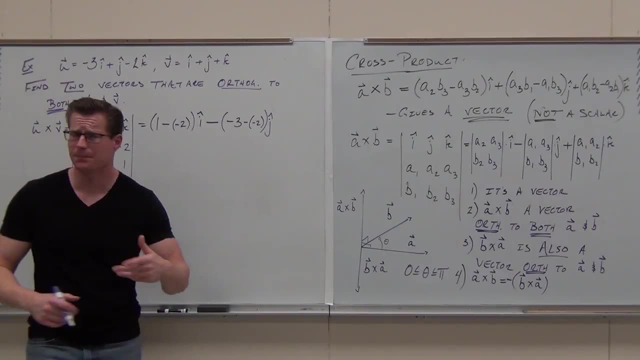 1 minus negative: 2. Got it, Minus, 9. Cool Negative. 3 minus negative: 2. Got it, j? What's the next one? A plus or a minus? j, j, j, j j. 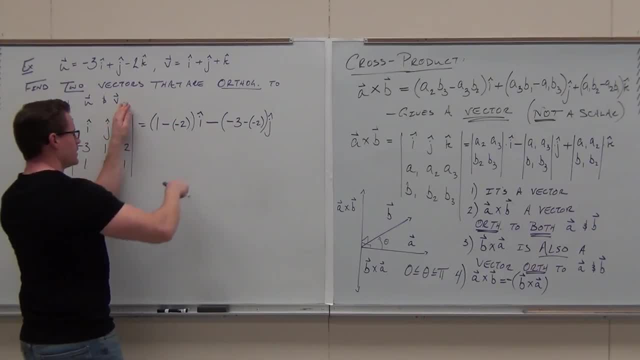 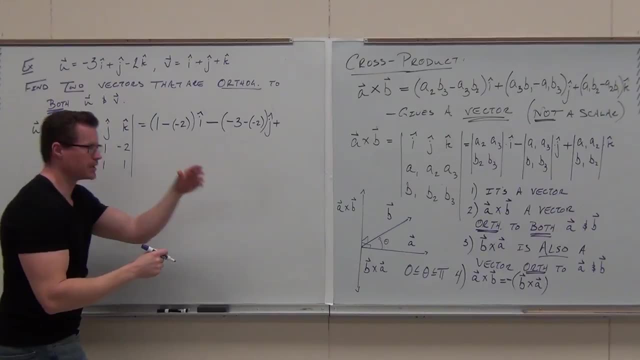 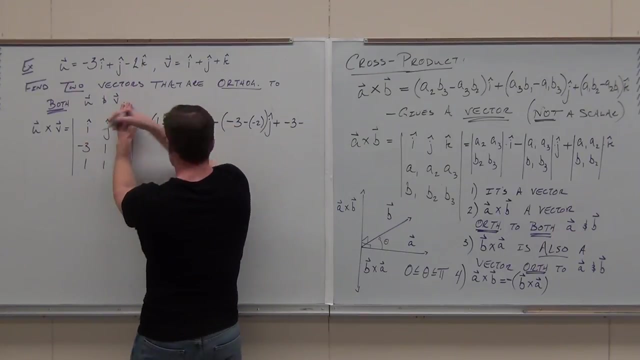 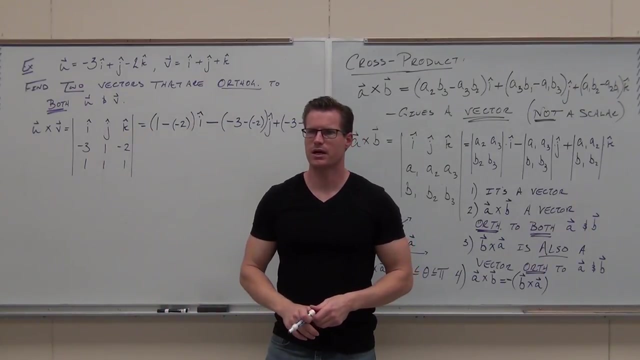 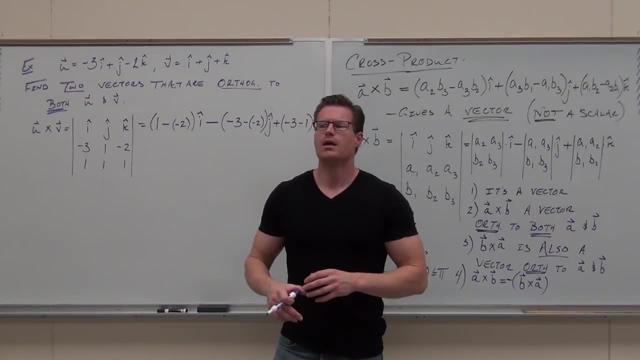 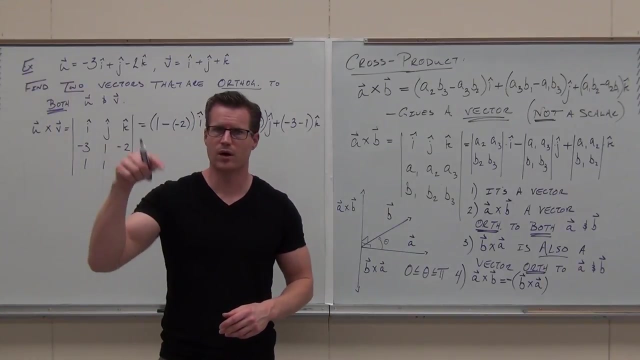 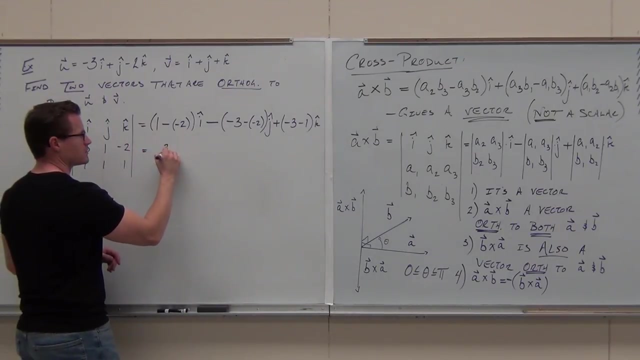 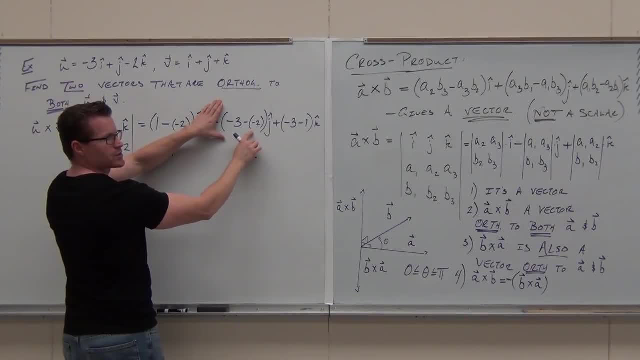 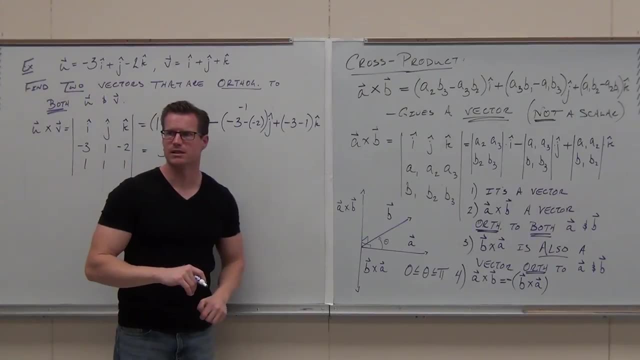 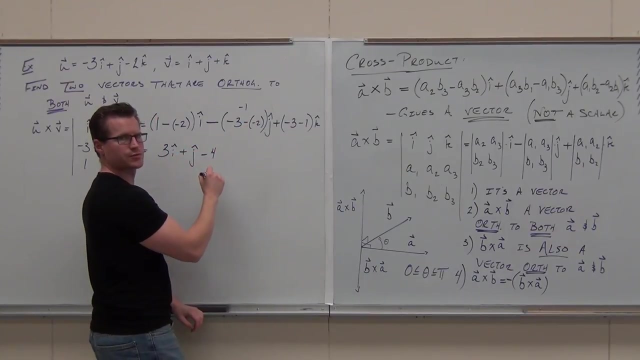 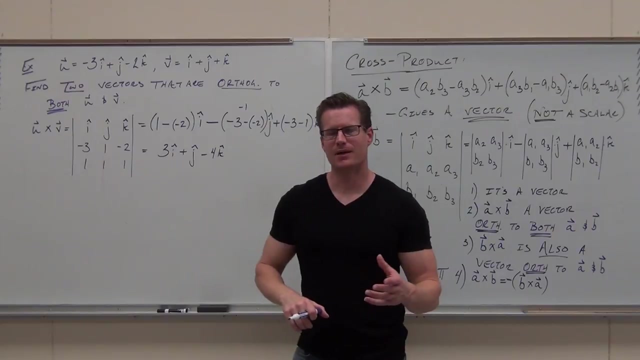 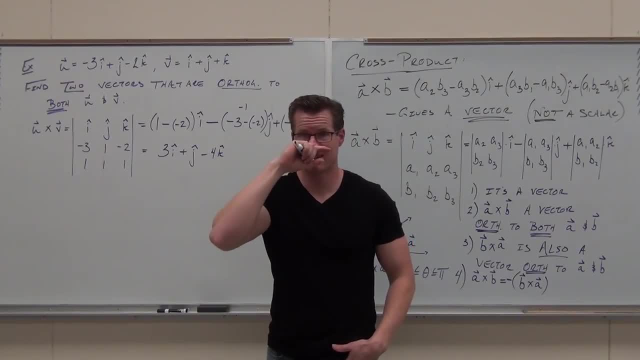 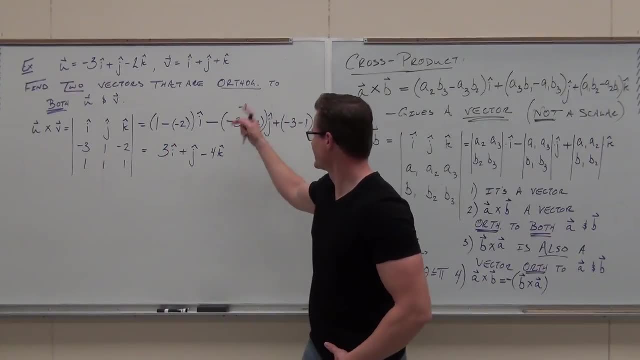 take a calculator out and just put the numbers in. trust me for real, because the last thing you want to do on a test or anytime you're doing homework really is fully understand a concept and give me like five right, because I think that can happen really fast. that's negative 3 plus 2, that's negative 1 and we're. 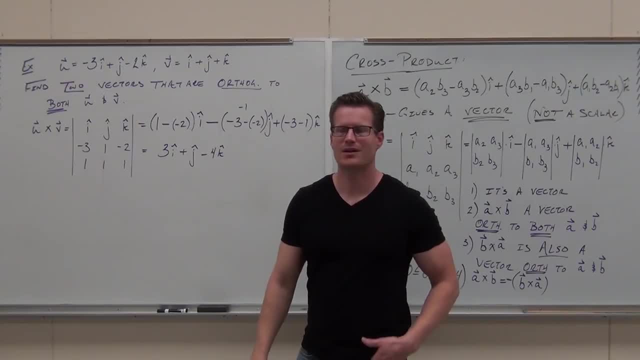 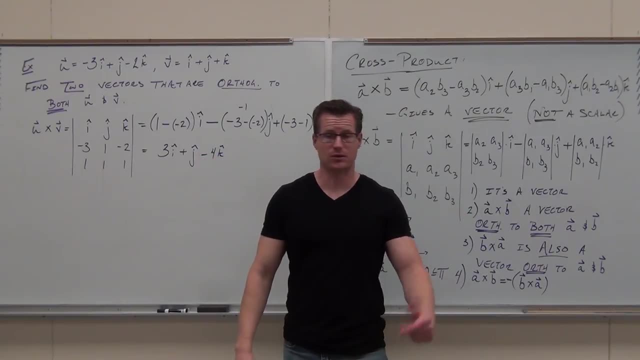 subtracting negative, that's. that's plus 1 and not you. okay, with that one. now, what is it? don't just do math, or the sick of math. that's how people fail classes. what is that? what's that thing? it's a vector. very good, yeah, and it's a. 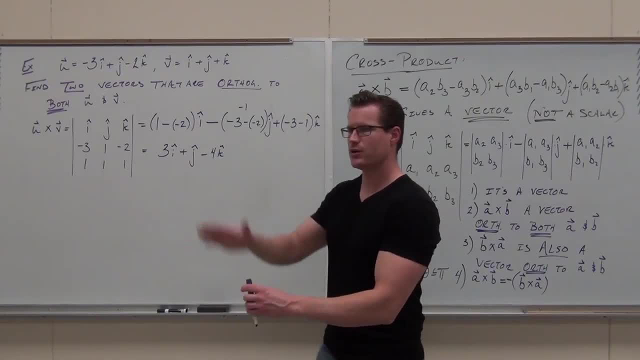 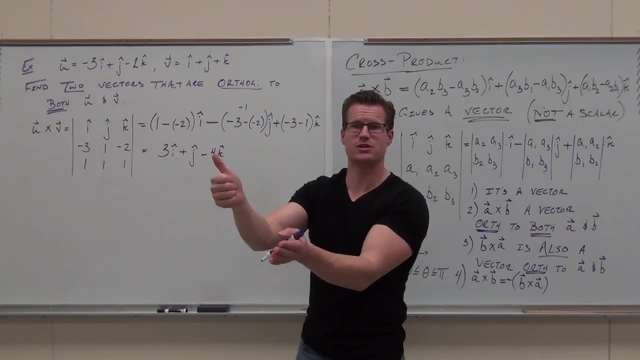 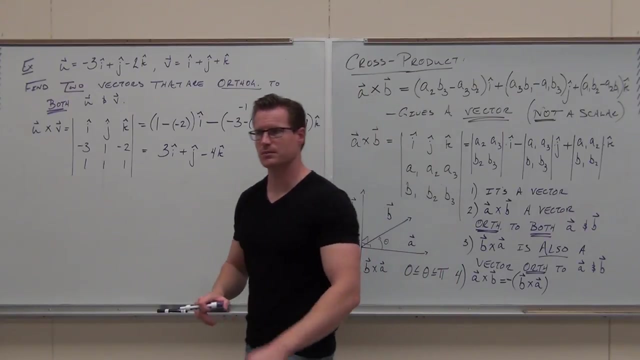 bigger this one. so if I have you and V this vectors going this way, verify that for me. how can you find another one of those vectors that's orthogonal, mutually orthogonal to both you and me? what would you do? do it, do it, see if you can do it. 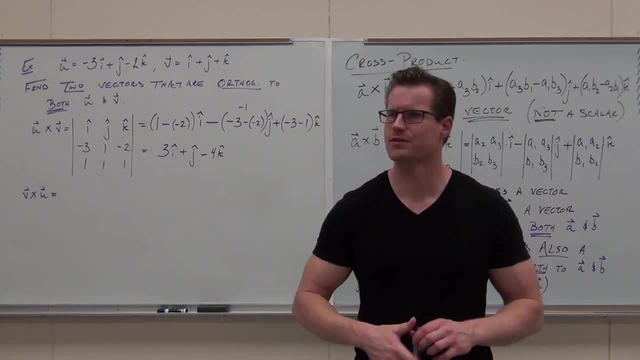 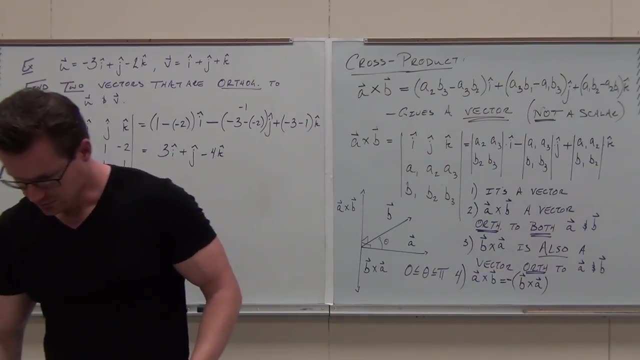 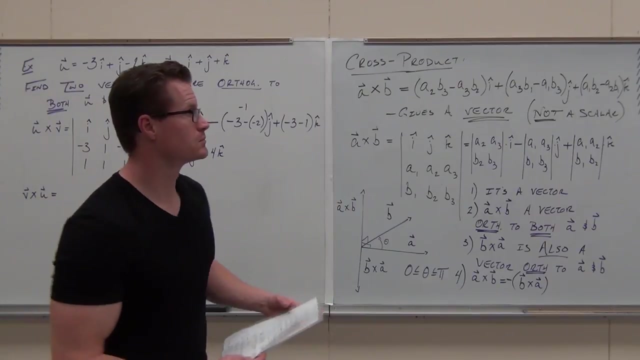 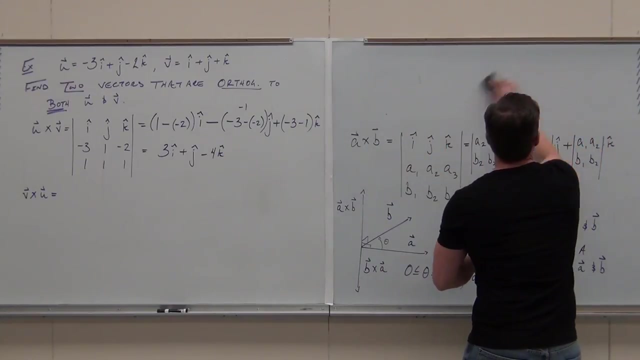 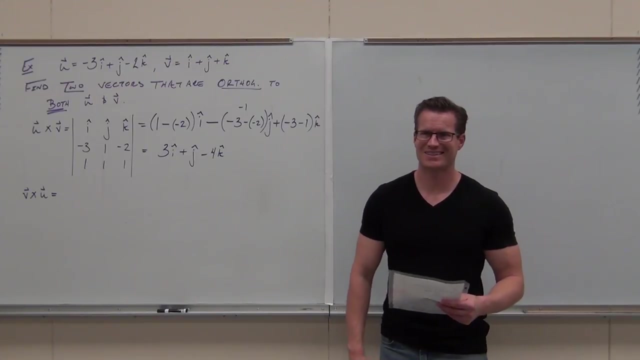 I'm gonna give you about two minutes. I'm gonna race the board. see that you can do you cross me. man, let's make no mistakes on it. all right, let's try that for you. you, you. is this not cool to you at all? is this kind of a little bit cool? a little bit? 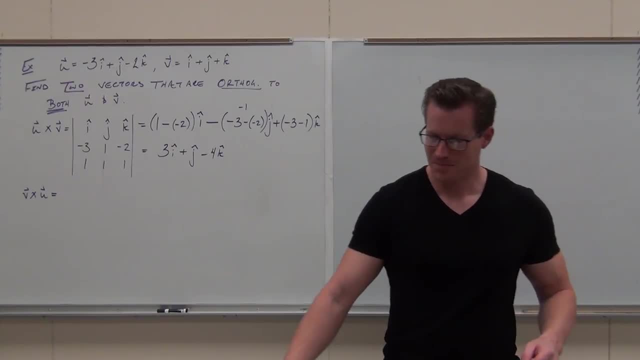 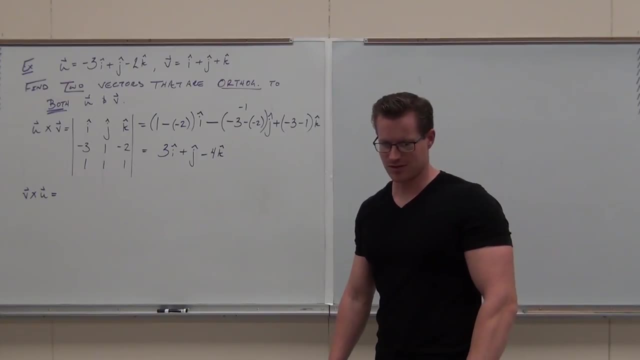 I love hearing that coolest thing I've seen all day. it's coolest thing I've done all day. I was stuck teaching calculation. I do like Calc 1, though it's kind of fun. What is Calc 4 all about? We don't even have a Calc 4.. 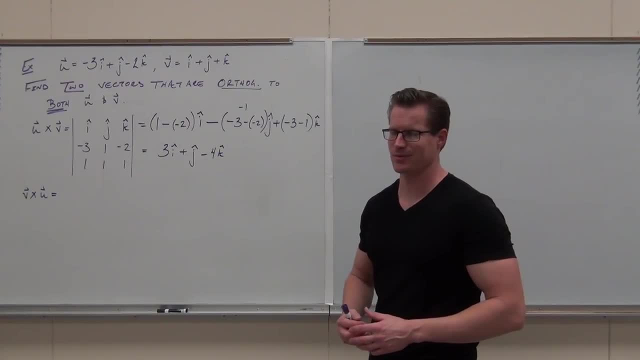 We just stopped, all right, so let's forget about it here. Quarter systems usually have a Calc 4. Usually they break it up a little different and then they'll have differential equations. We do Calc 3 and differential equations. that's how it goes. 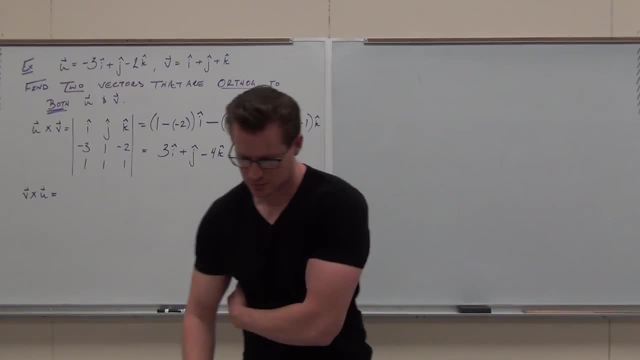 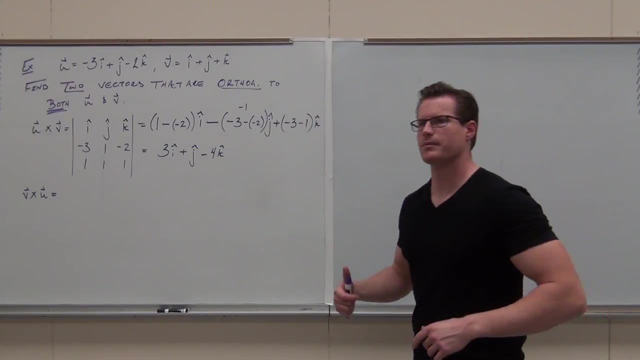 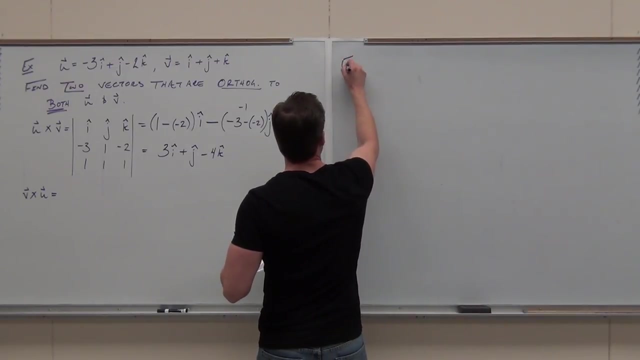 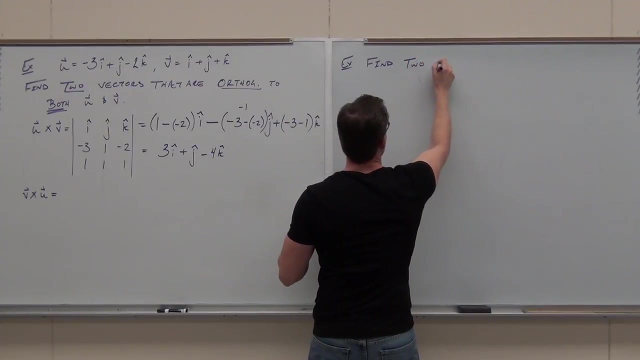 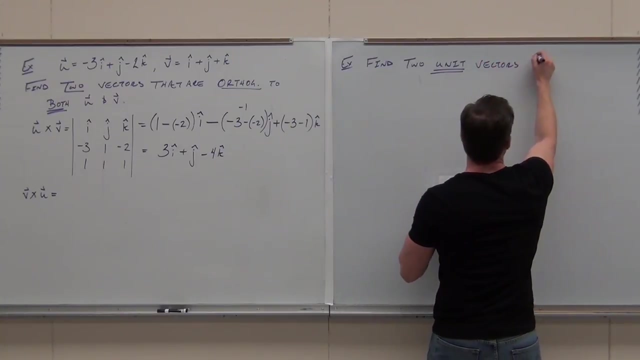 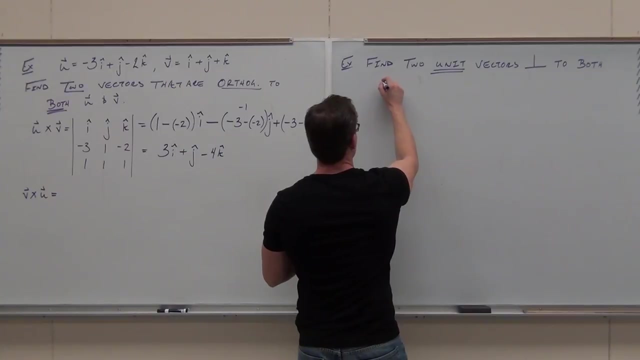 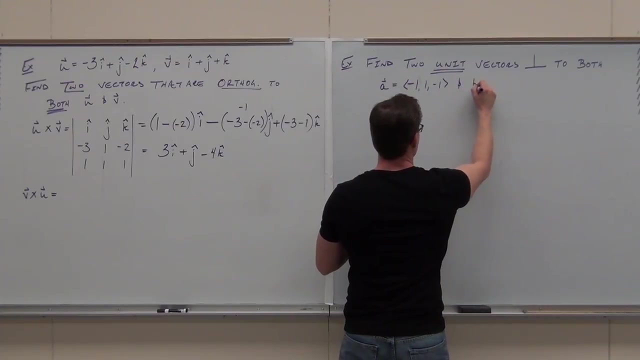 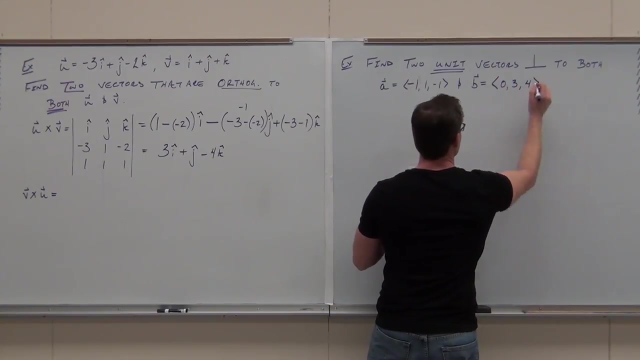 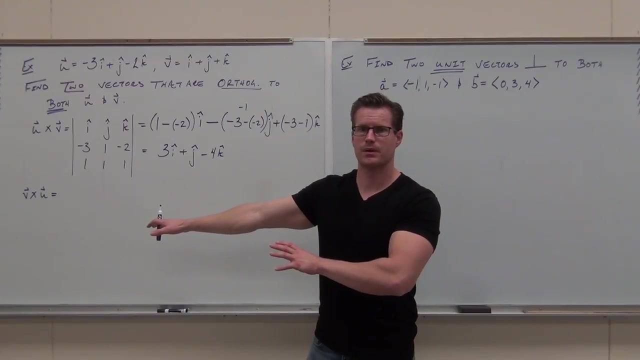 Some people consider differential equations to be Calc 4, kind of is If you're done with that already, or if you're a good thinker, then you're already done with that. try this one on your own. By the way, did you have enough time to actually do this? 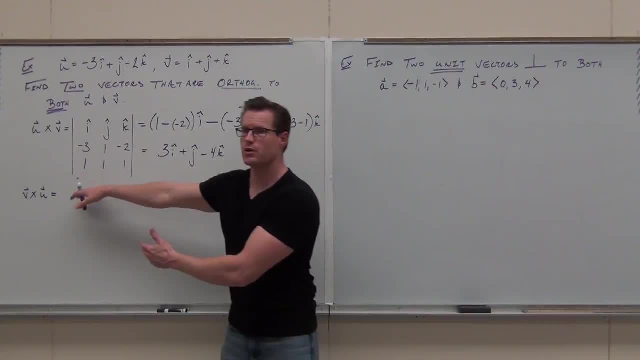 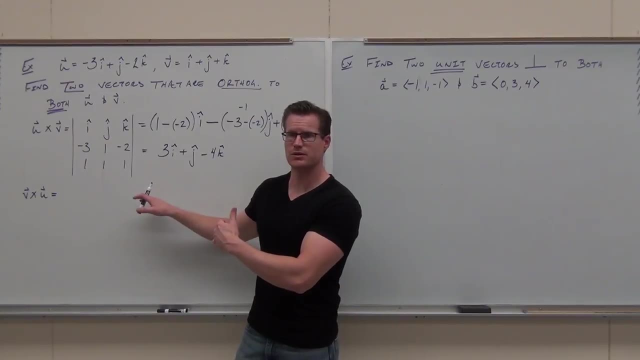 Can you focus up here for just a second? Okay, stop what you're doing. Did you do the whole matrix thing and do all that stuff? Yeah, Tell you what. did you look at your answer? Yes, Did you look at this answer? 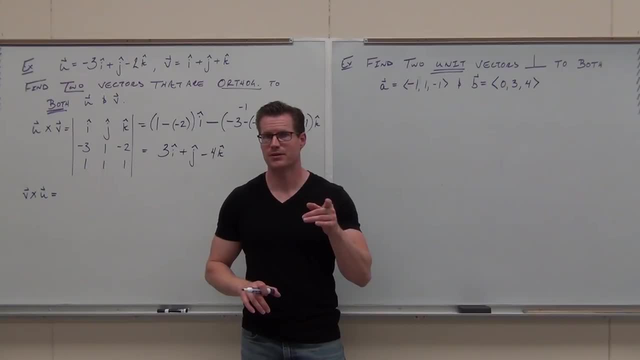 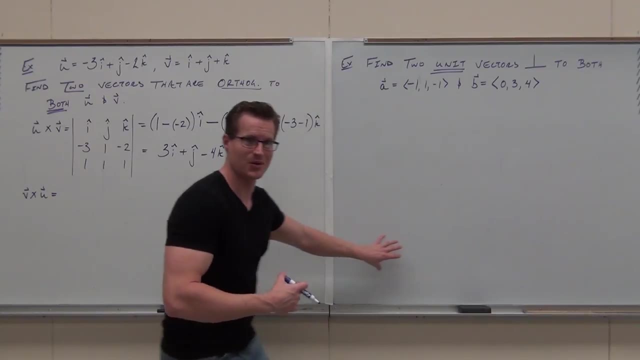 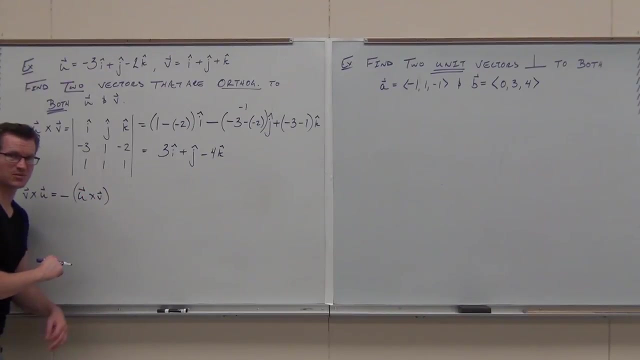 Yeah, Now answer this question. How do you find a vector that's the same length, but just in the opposite direction? What do you do? I gave you a prop tip here, right? I told you that this is that same thing. 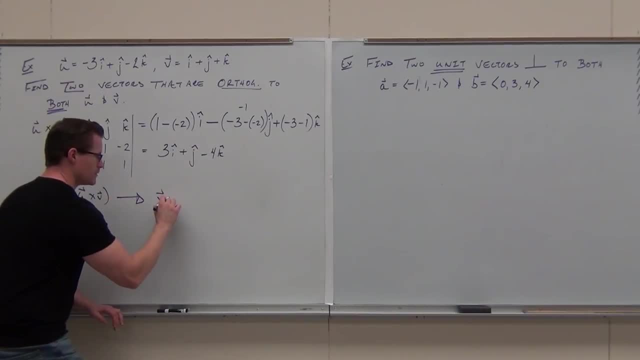 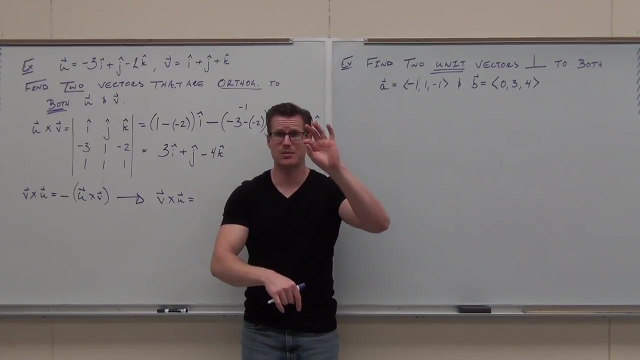 So if I want to find B, cross U. this is your understanding. The idea of a cross product says: hey, this thing, this thing, they do the same thing, It's just in opposite directions. If I want opposite directions, same length. 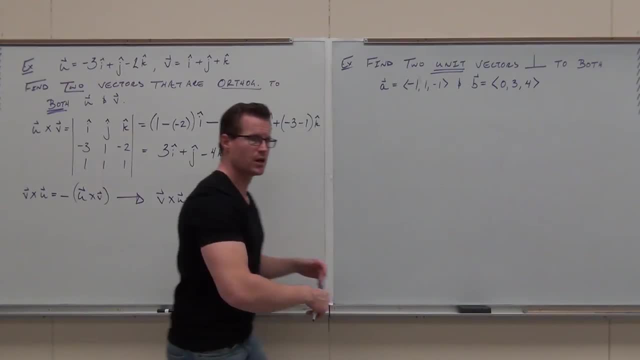 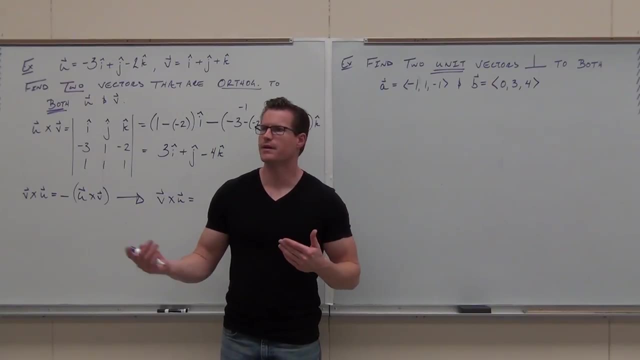 all I got to do is multiply by a negative. It switches the direction. So if I ever ask you for two vectors that are like, orthogonal to both, you just got to find one and then switch the sign. So right here we'd say, yep, this is going to be. 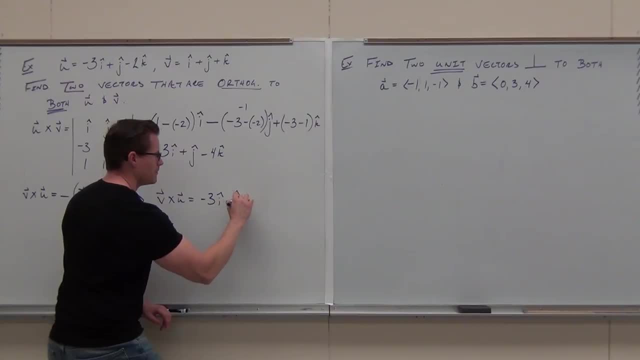 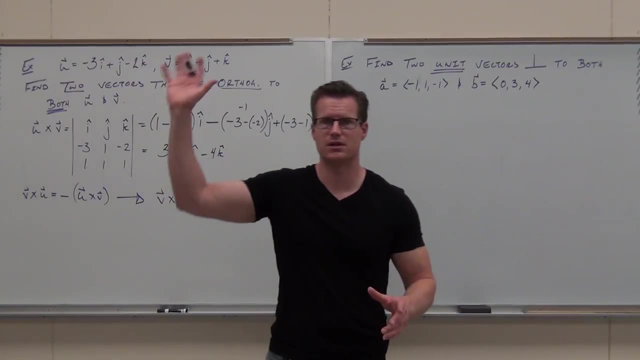 I guarantee it's going to be negative 3i Minus j plus 4k. I want to know if you guys found that one Either way, show of hands. if you did and you found that one, Good for you, that's fantastic. 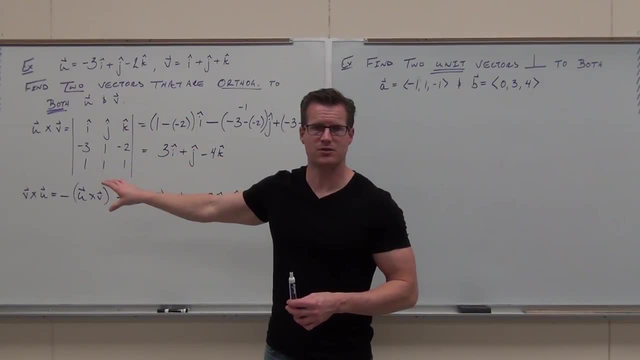 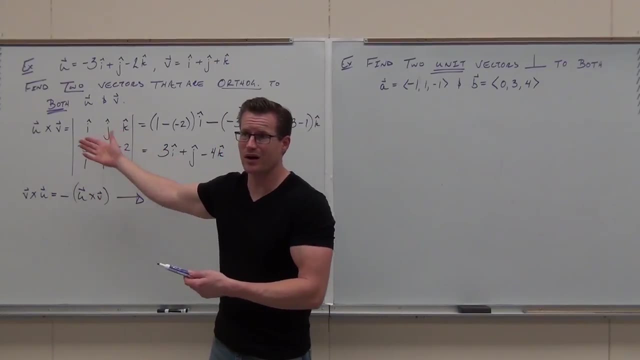 So next time you get the question, do you have to do both matrices? No, No, I wanted you two to get the practice on it to make sure you got it. but in the future you got to just find one and then you can switch. 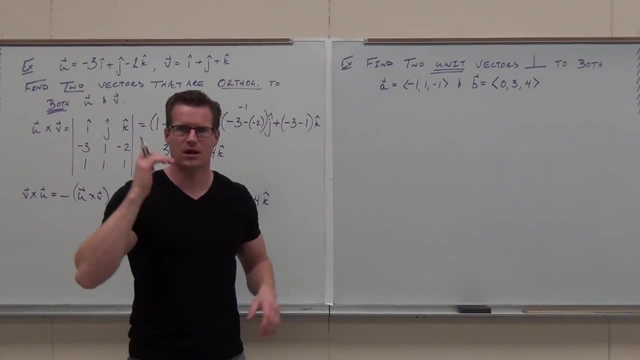 that sign around and find the other one. Try that on this one. I'll give you a couple of the minutes. I want to find two unit vectors. What I want is for you to at least find one and then you can switch that sign around and find the other one. 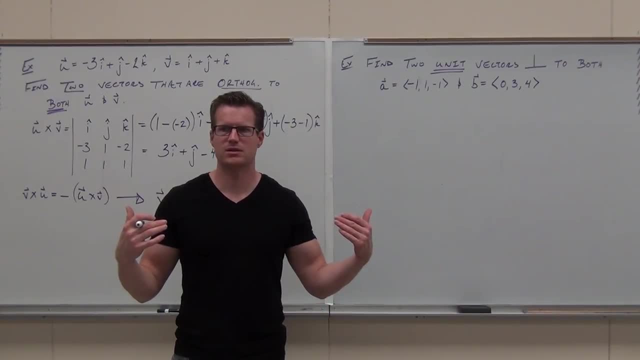 Try that on this one. I want to find the vector that is orthogonal to both, And then you can stop there. we'll talk about the unit part. It should be in your head. see if you can complete it. We'll do that in a second. 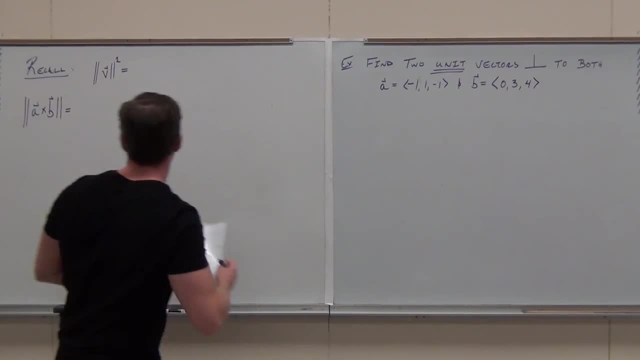 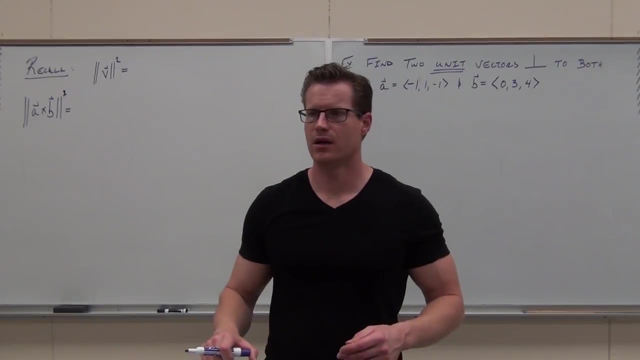 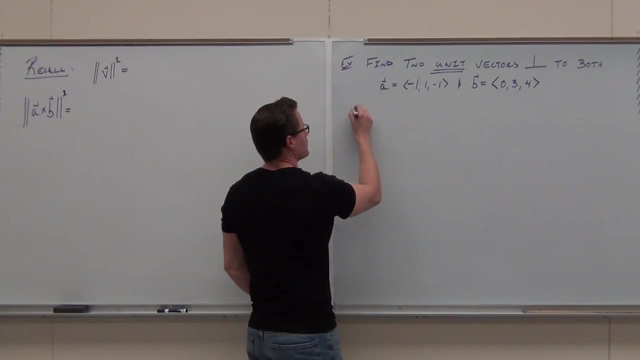 How far are you at? have you set up the matrix yet? It's going to let you solve that. Have you found the cross product of these things Good When we're asking for a vector that's perpendicular, orthogonal, normal, to two other vectors? 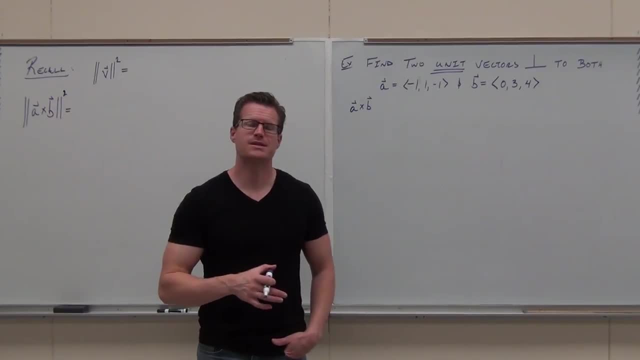 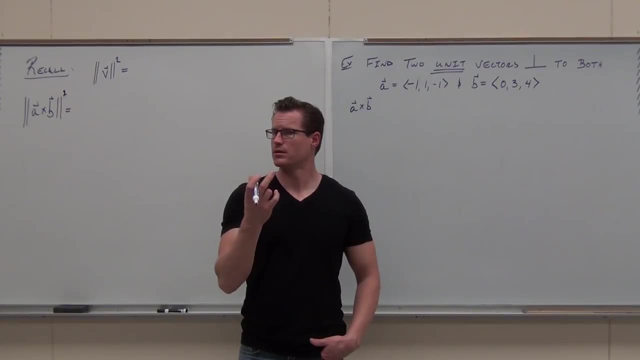 we are asking for a cross product. that's all we're asking for. Does the order matter? Does the order matter? in which are you going to get the same answer? if you switch it around, You're not going to get the same answer. 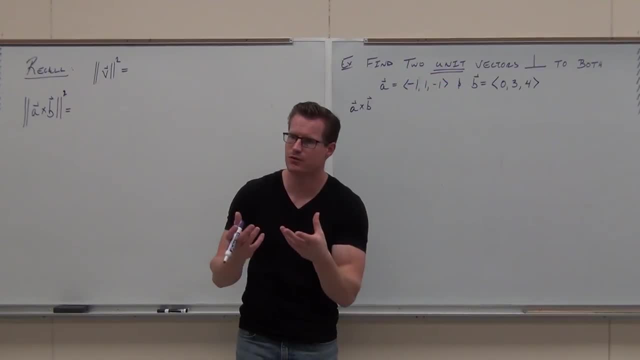 but you'll answer this question, no matter which way you do it, Because if you're looking for both of them, the reverse order of a cross product is what gives you both of those vectors that are mutually orthogonal to both A and B. So if we set it up, I'm going to do A cross B. 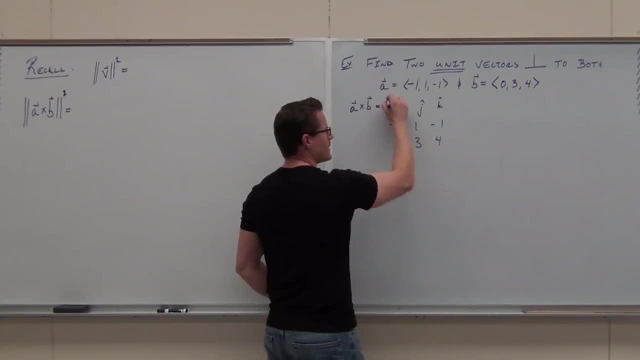 I'm really careful not to forget any signs. I want to be pretty organized in my work. I also don't want to do a whole lot of shortcuts because I know myself I know I'm going to make some mistakes on signs if I do. 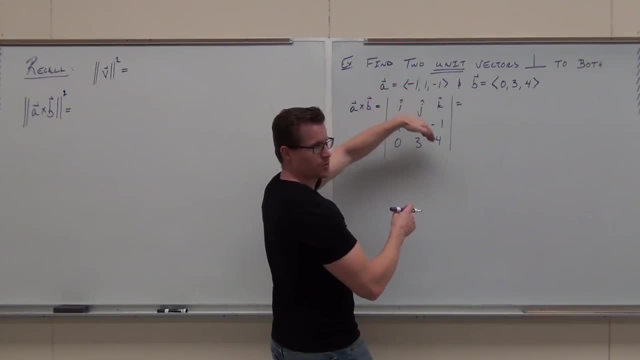 So the way we do it, we go okay, double check: negative 1, 1, negative 1, 0,, 3, 4.. We got that. We got I, J and K. So when we're doing this, we're going to cover up the I column. 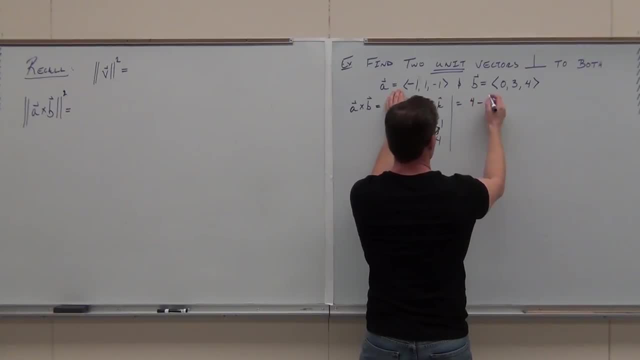 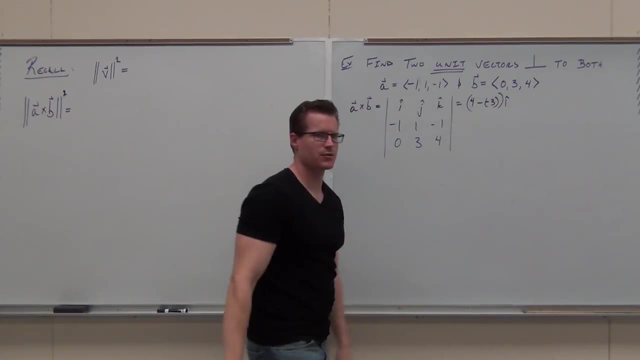 We have 4 minus negative 3I Did you get that. Next thing is what? Come on everybody quickly. Oh, that was like one person. What's the next thing in this method? What do you do? Negative: 4 minus. 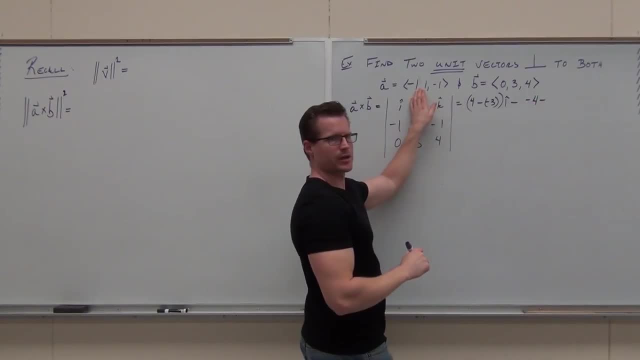 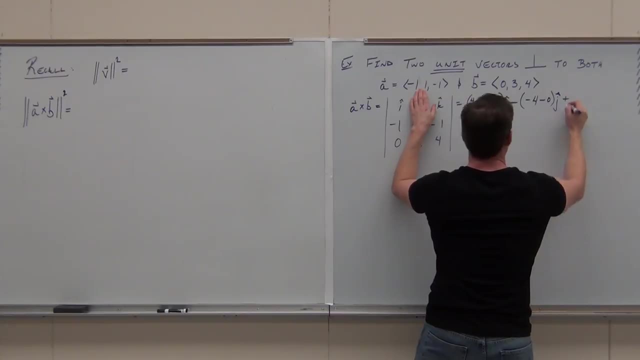 Zero. I love that. I love zeros. So we're going to do negative 4 minus Zero. I love that. Plus. you're noticing I'm not doing a whole lot of work in my head. honestly, for real, It's really easy to make mistakes. 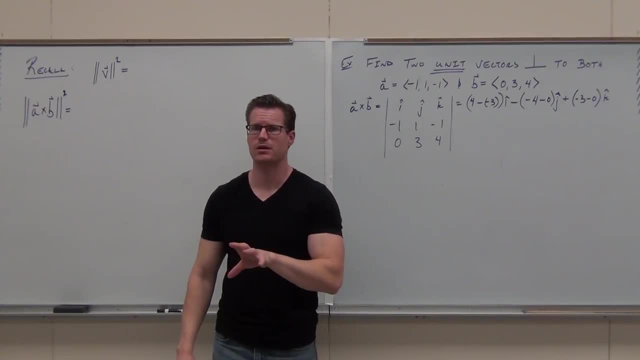 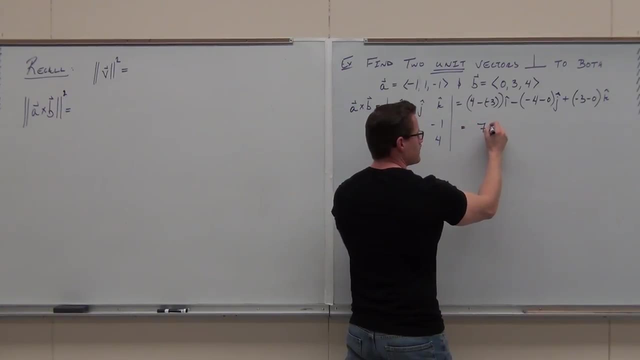 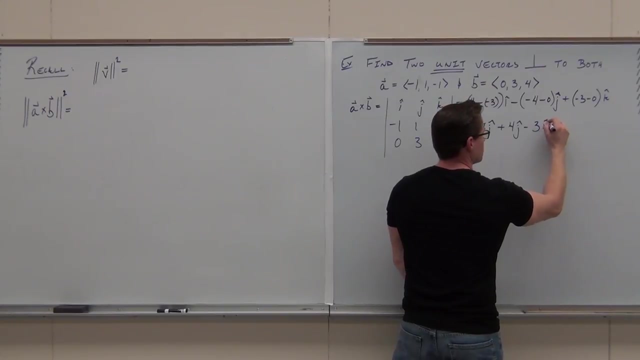 Hopefully I'm right. I want you guys to double check my work all the time when we're doing this. Did you get the same thing I'm getting? Okay, so let's complete it: A cross, B, 7I, 4J minus 3K. did you get the same thing I got? 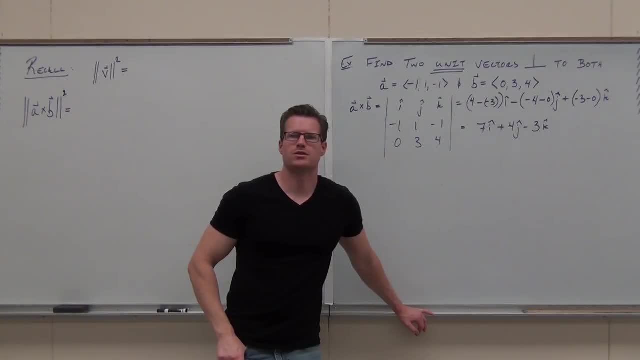 Yeah. Now here's my question to you all. We've got to think back. Did you answer the question? No, No, What was the question? Univector- Is that a univector? No, Okay, so what is it? 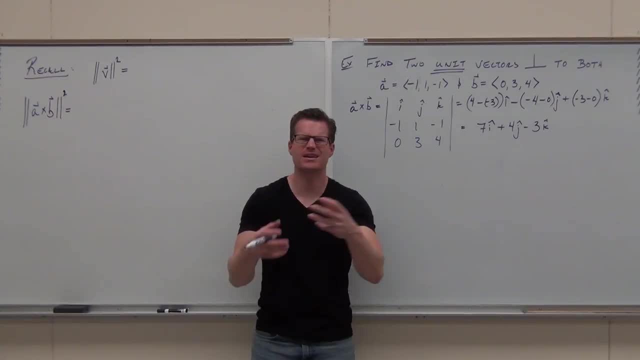 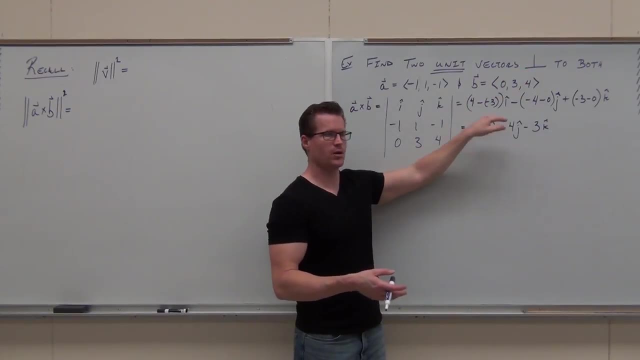 Come on, put it together. What do we have? It's a vector. It's a vector that is Orthogonal. Two, Eight, Both of them. That's great. That's like halfway there. So we've just got one vector that's orthogonal. 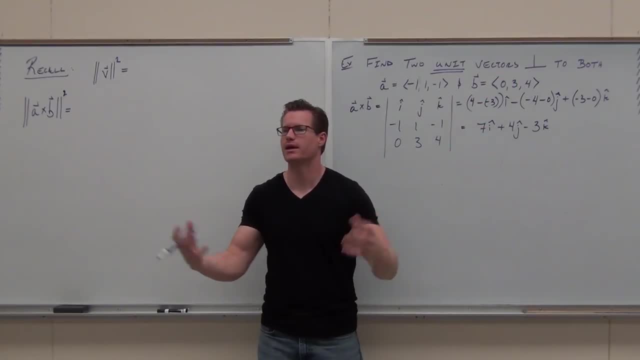 to both of those, but it's not a univector. Come on, everyone in class right now. how do you go from here to a univector? Quickly, Divide by magnitude: Great. So as long as we have that vector, that's orthogonal. 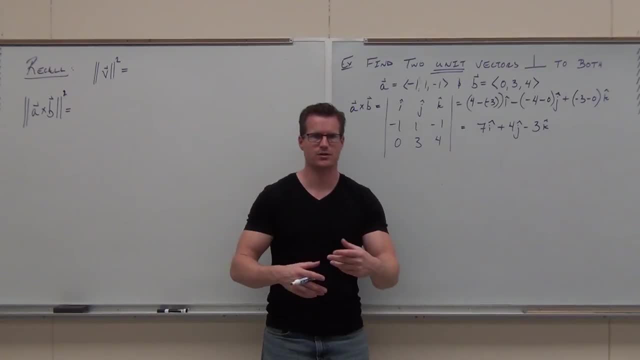 to both and we can find a magnitude. we can find a univector. A univector is always vector divided by magnitude. So if you haven't done it already, we're going to do it now. The magnitude of A cross B. 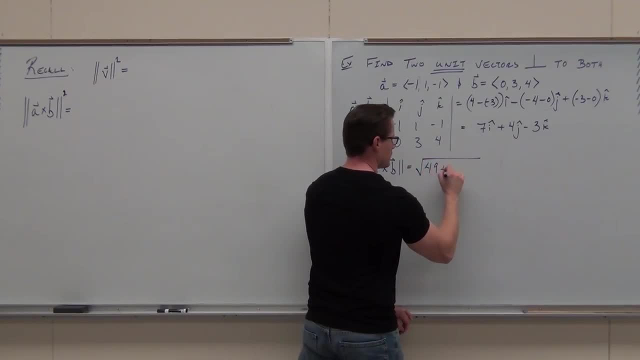 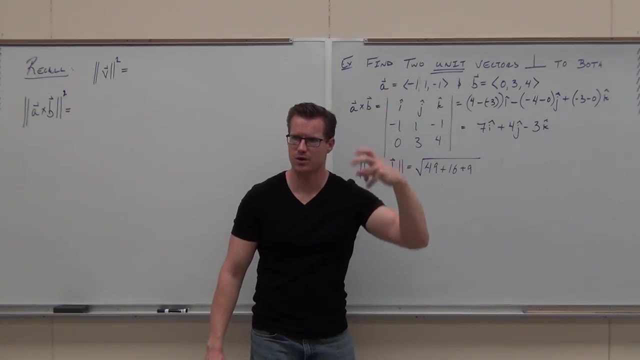 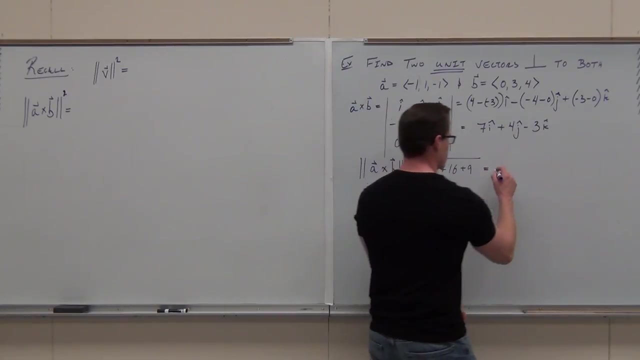 pretty easy to find: 49,, 16,, 9.. We take the squares, add them, square, root them. Never a negative in there, It doesn't even matter. Oh shoot, we're in 74.. Double check: 74?. 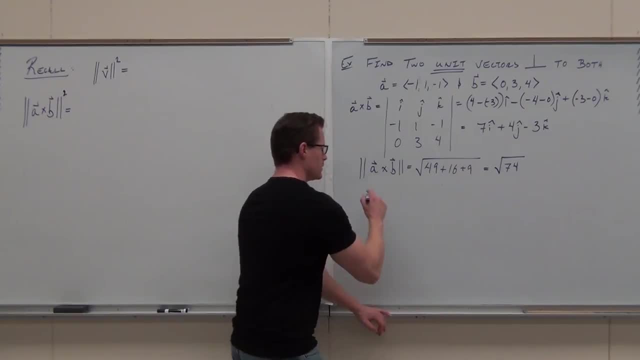 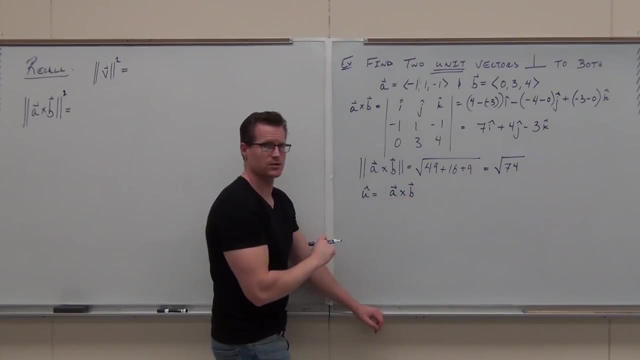 Perfect. What do we do with that? Unit vectors are always The vector itself. We have that Divided by the magnitude, Takes the length, divides it by the magnitude, changes it to a length of 1, same direction. That's why we say unit vectors are directions. 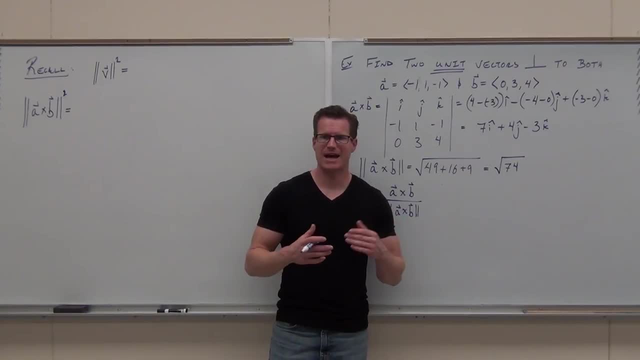 So what we're doing here? we're finding the vector that has the direction of the perpendicular. That's what we're doing. Why do we do all this stuff? We're going to talk about planes in the next section, Not this other place. 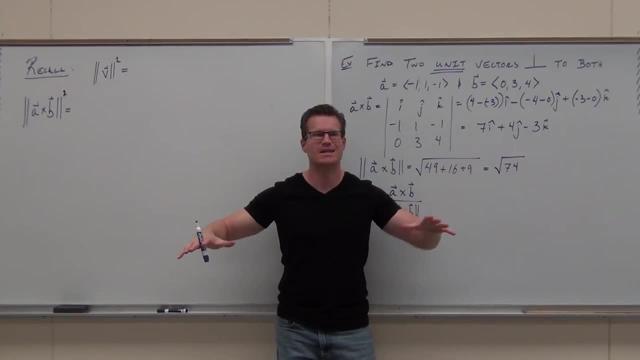 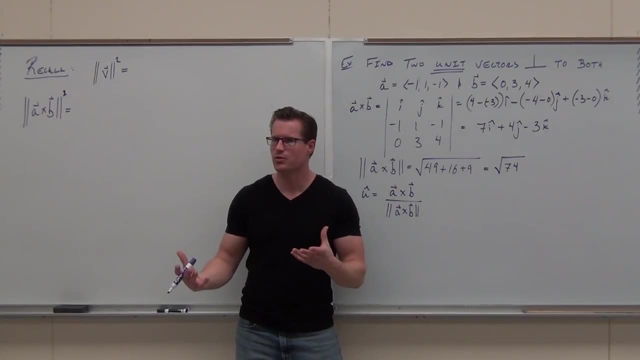 That'd be awesome. But, like I said, But like planes, And we need normals to do it, We need orthogonals to do it, We need cross product to even do it. So if we can't find an orthogonal, we can't even talk about planes. 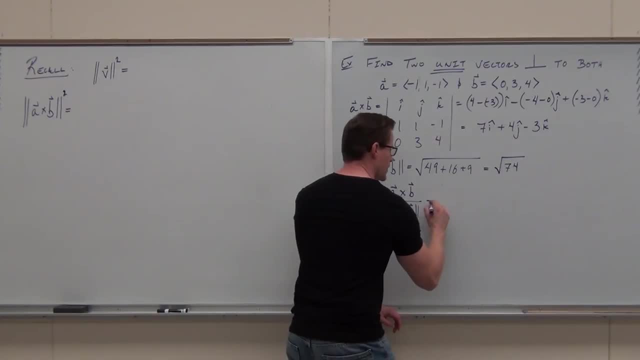 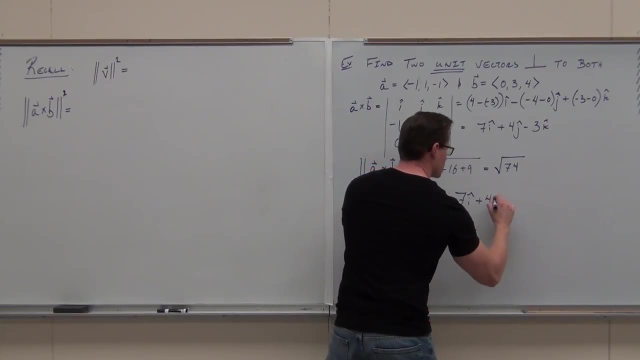 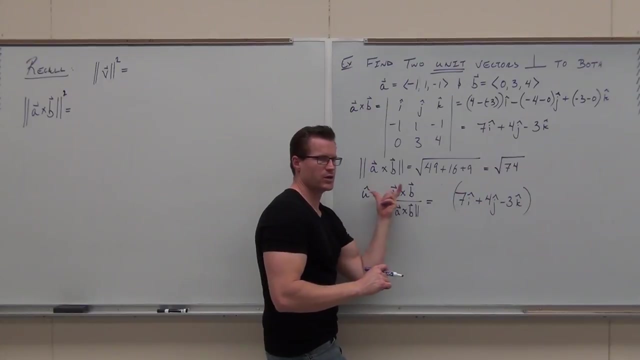 Did you get the idea? We're going to do that? So for us, right now, honestly, I'd put it like this: I'd leave my vector. This is A cross product. This is B. We know that when we divide by the magnitude. 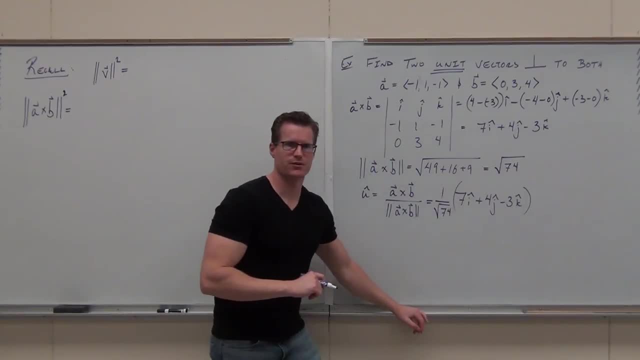 it's like having 1 over the square root of 74.. This is the same. Is that making sense to you? Same thing: It's like dividing, but you have 1 over that. You're probably not going to see that though. 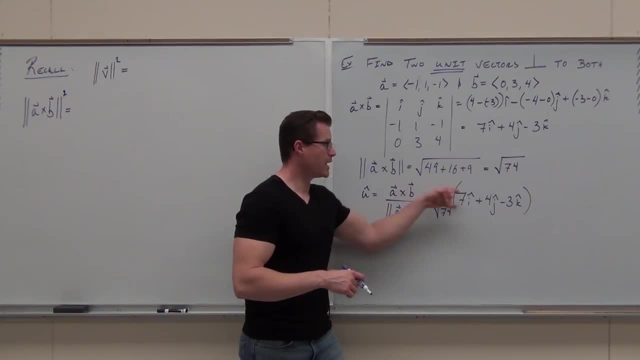 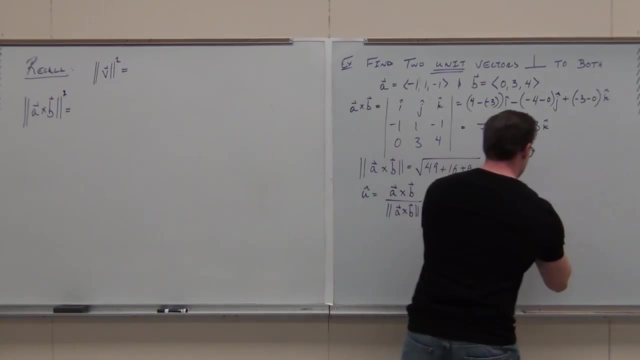 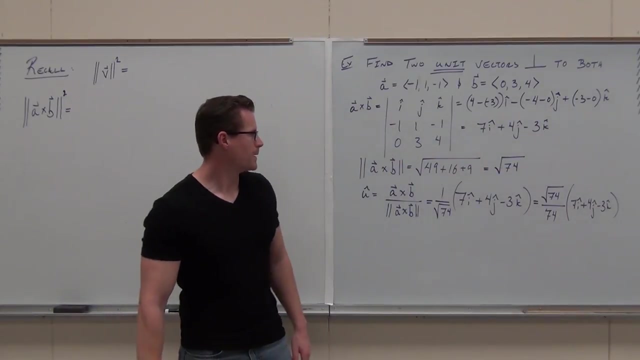 What are they going to do to you? Rationalize? Probably going to rationalize. Would I distribute it? Not unless I absolutely had to. A lot of times, unit vectors are really nice when you leave that nastiness out front. That's what I'm looking for. 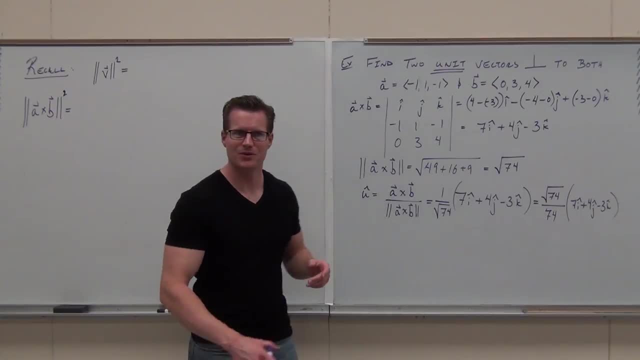 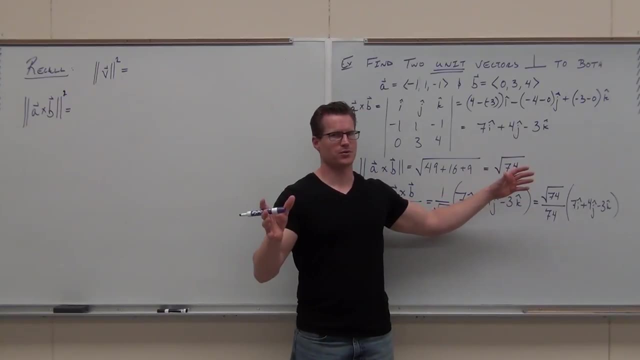 Have we answered the question No, OK, so now do we have to redo all of this work? if we want to answer the question No, This is OK, let's follow through. Is this orthogonal to both A and B? 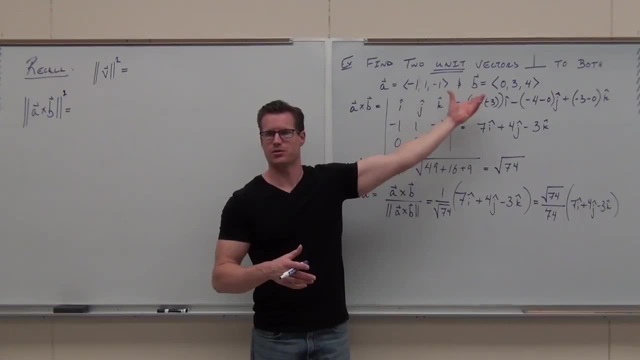 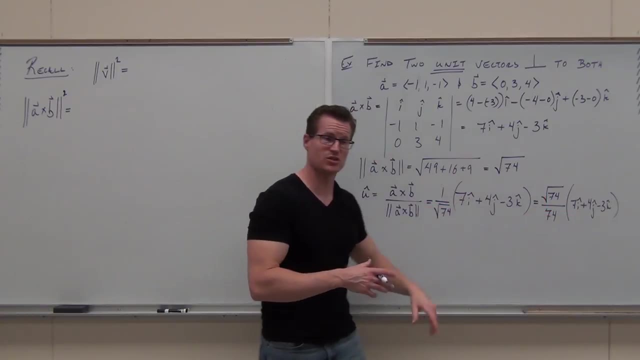 Yes, That's what cross product does. Is a unit vector orthogonal to both A and B? Yes, Is it two orthogonal vectors to both A and B? No, What's the other one Negative? So this is one of them and another one of them. 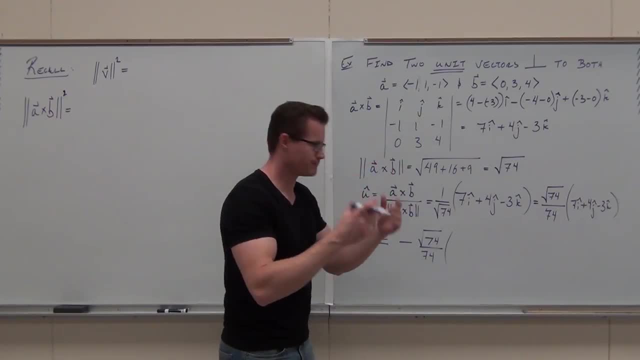 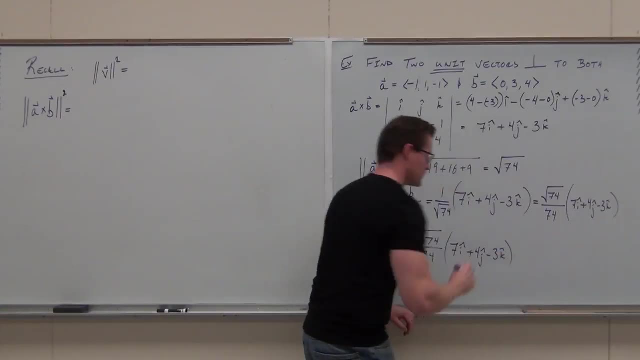 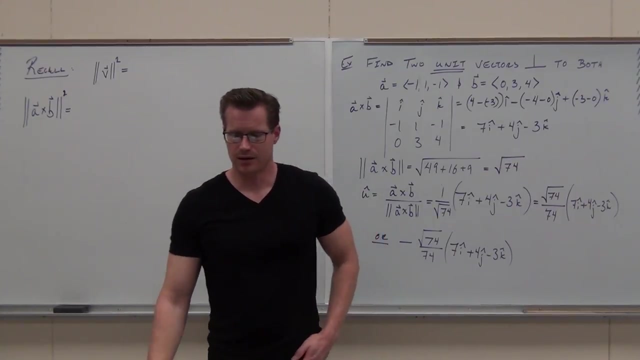 Yep Negative reverses the direction, Keeps the same magnitude. It's all good. Well, we've already done a lot of work. I'm going to deal with one more thing before our little break here. I'll leave you with a punch line. 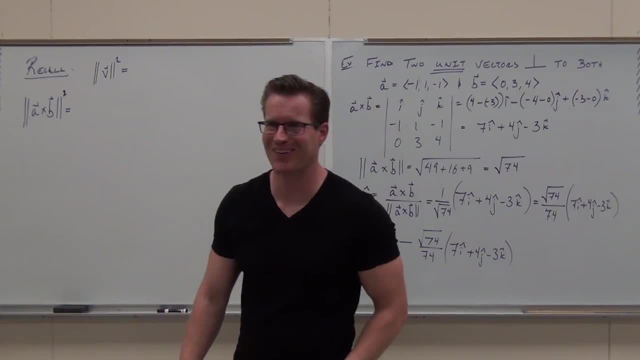 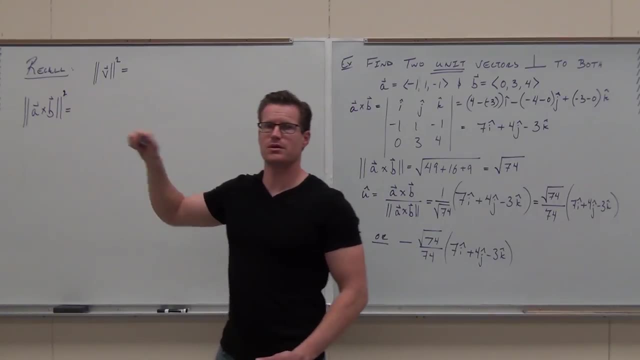 I'm going to think of for the 10 minutes that we have our break. It's going to be pretty cool. It's going to be pretty freaking cool, all right, So you stick with me on this one. Do you remember what this equals? 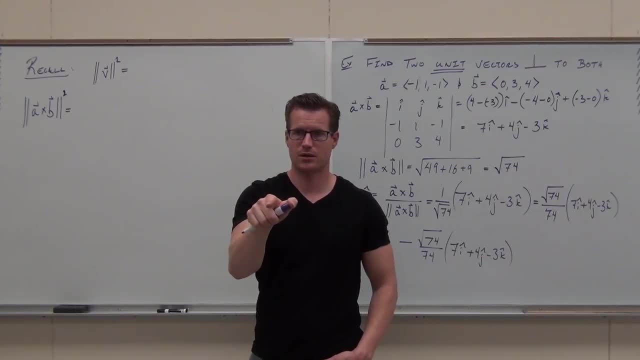 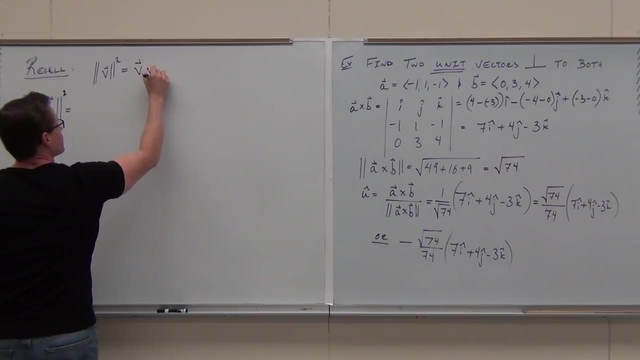 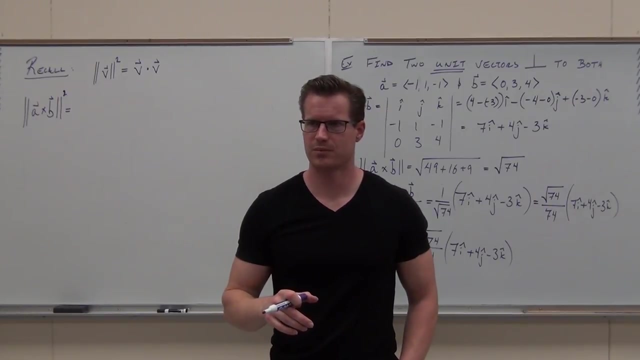 The dot product, The dot. So the dot of V, dot V. That's what it does. Do you recall that little thing that we did? Stick with me here. We're going to have something pretty awesome. OK, We're going to go a little bit past. 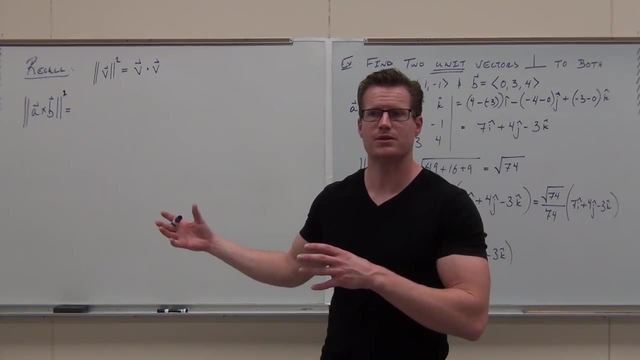 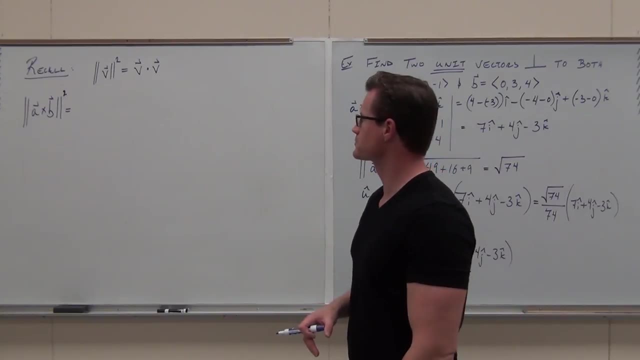 because we're kind of rolling here And I want to get this proof done so that you and I are going to do this proof for the rest of this section. It's pretty cool. Well, not the whole proof, but the corollaries of proof. 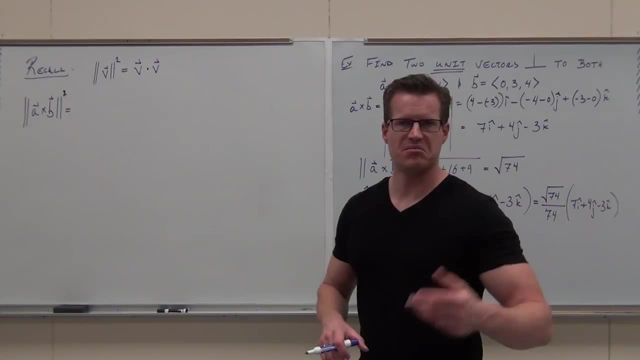 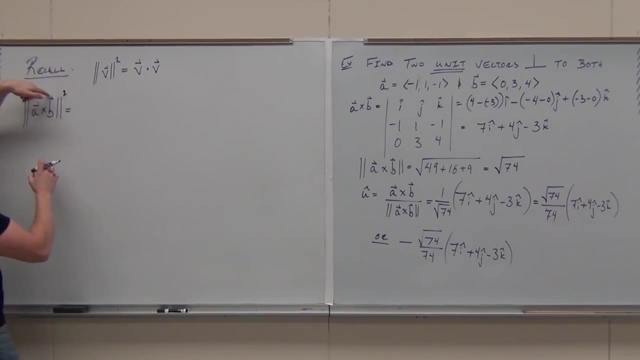 Well, let's look what happens. when I take the magnitude of a cross product and I square it By this definition, I get the magnitude of a vector. Verify, that's a vector. Come on, Vector Vector, Which means that I can take this vector. 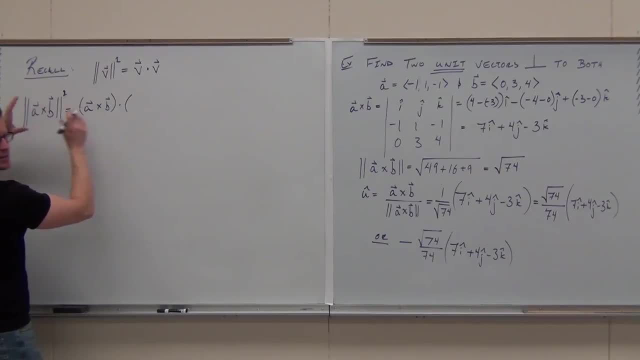 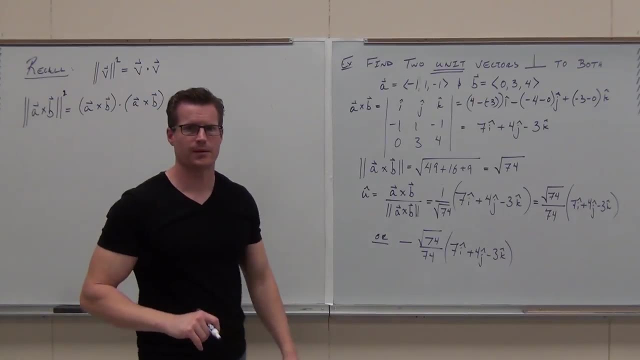 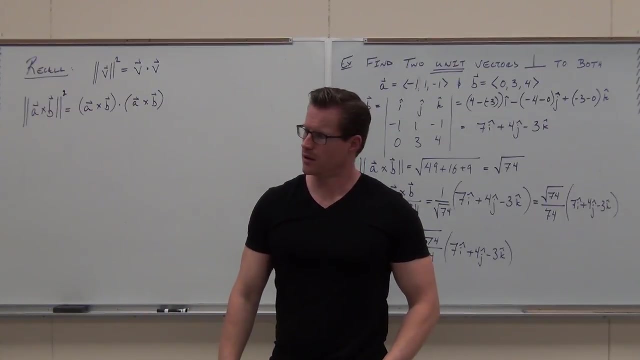 And say: this is equal to the vector dotted with itself. Can you actually do that? Yeah, It looks really nasty. All right, So for the rest, I really don't want to do all the algebra. Please don't make me. 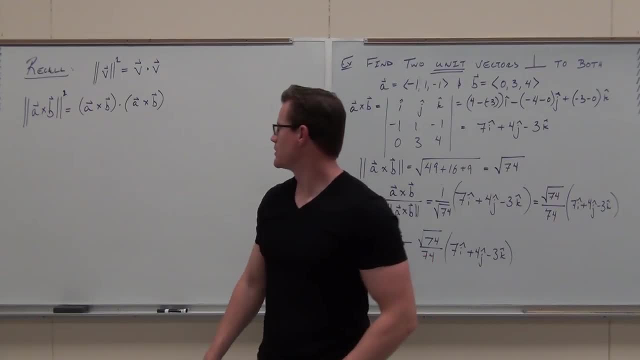 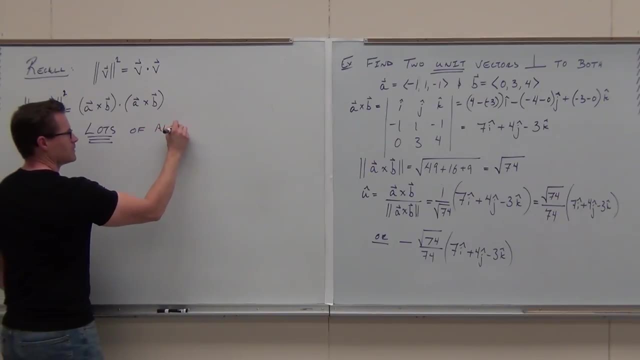 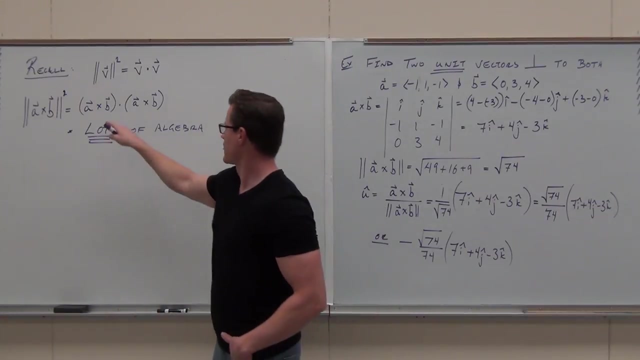 Please, Please, OK, I'm not going to anyway, So For real, all right, But you could do it. You could do it. You could set up: i j k a1, a2, a3,, b1,, b2, b3,. 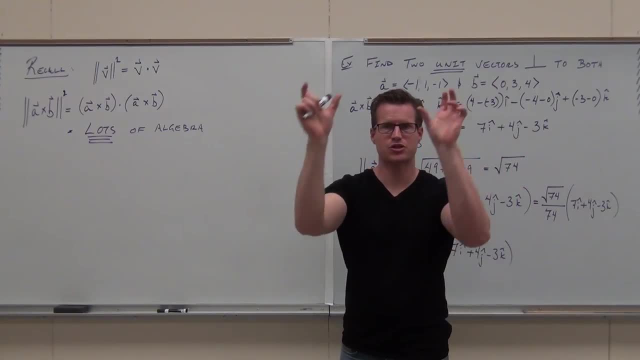 figure out both of those things, dot, product them, which means multiply each of those components together, do some crazy factoring, And then what we get after all of that stuff which I have on my paper, It's like this: all right. 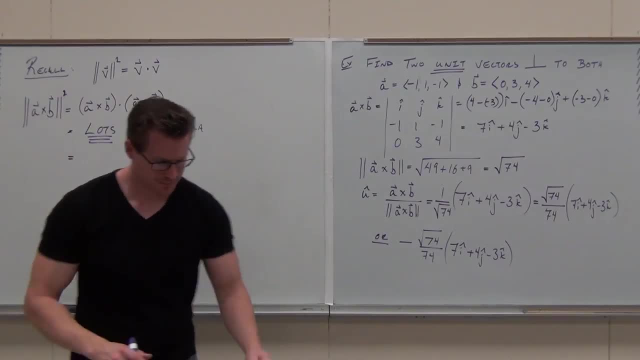 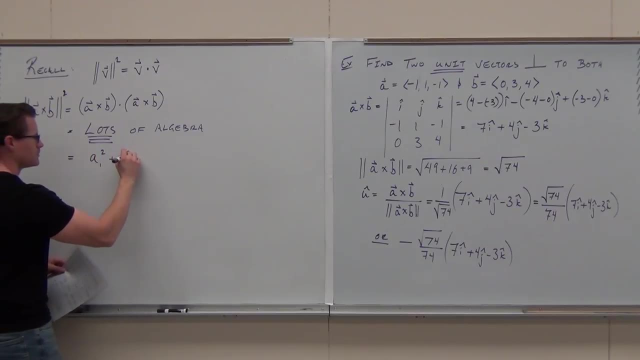 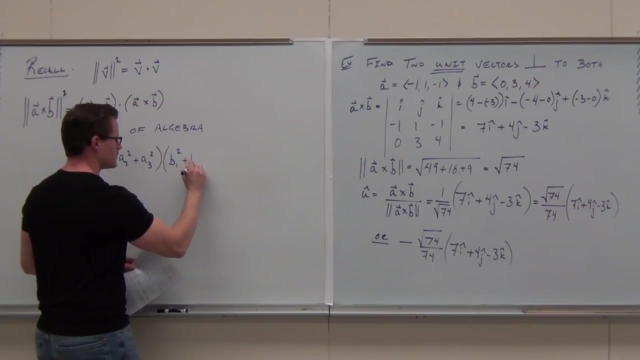 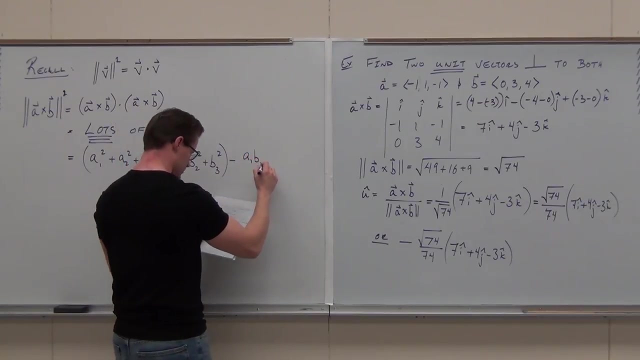 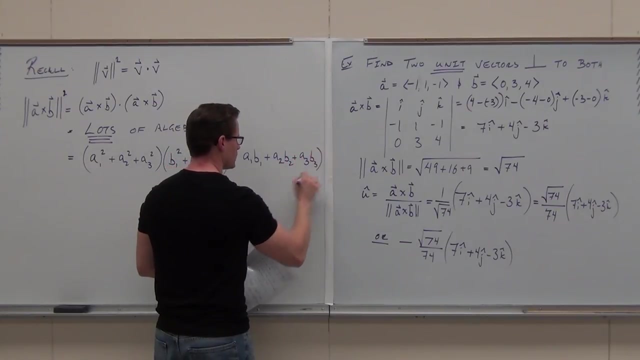 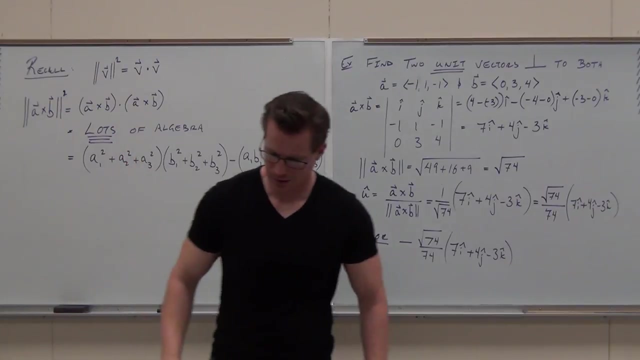 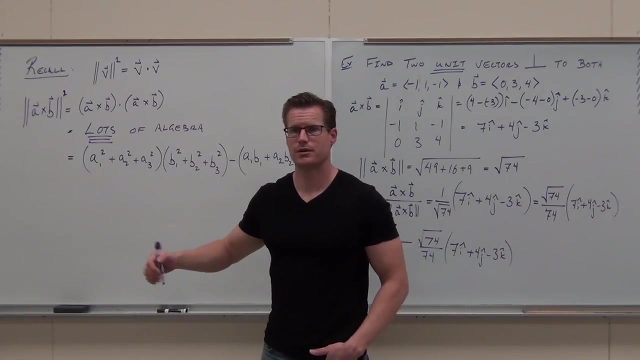 What we get is this. So lots of algebra, Trust me, ul. So what we get is this: We get a1, a2, a3, all squared added. Oh my gosh, Does that look familiar to you? 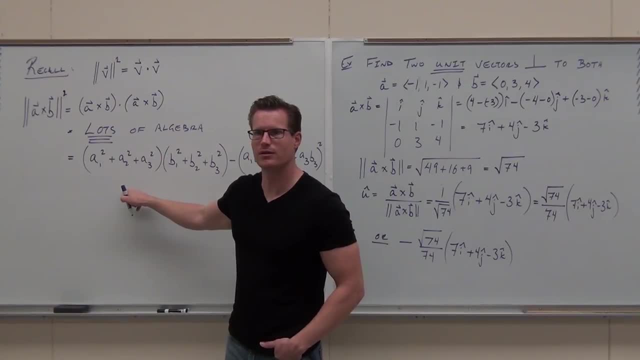 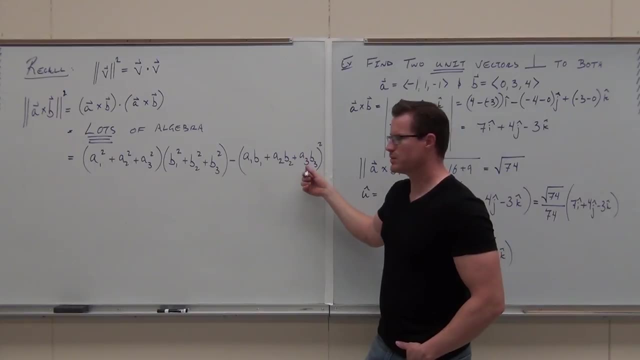 It should Come on, It should b1,, b2, b3, all squared added and we get this a1b1, a2b2, a3b3, and we're going to see what that is. 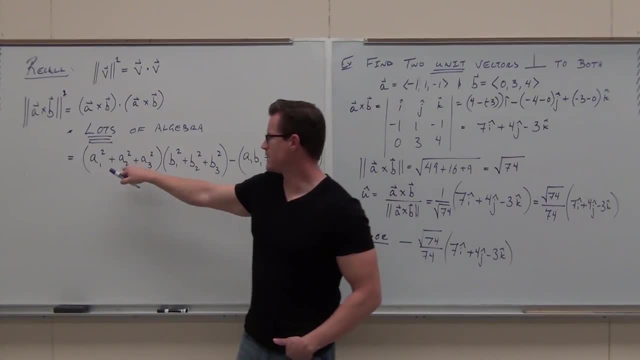 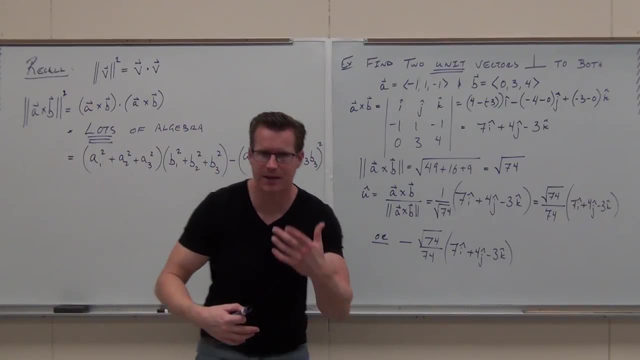 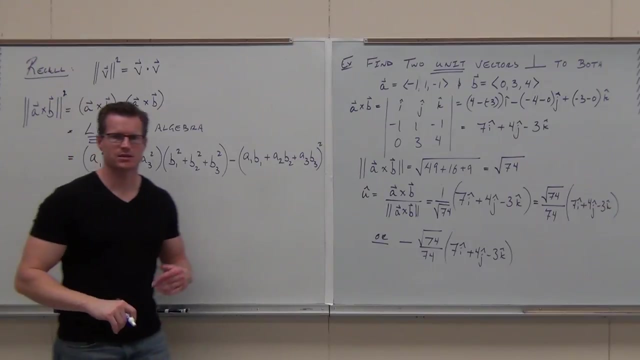 But these ones should look pretty familiar. In fact, what this should look like is the inside of a magnitude. Does it look like the inside of a magnitude to you, Or if it's the inside of a magnitude, that's the same thing as the magnitude squared. 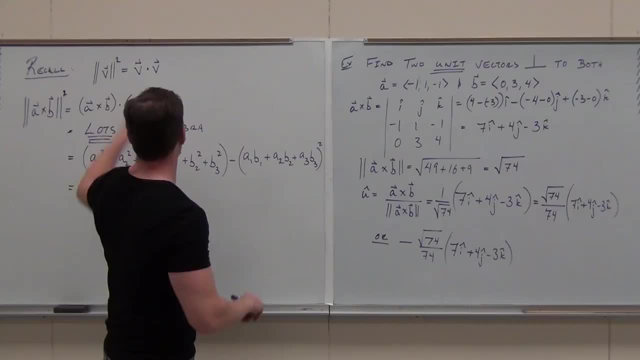 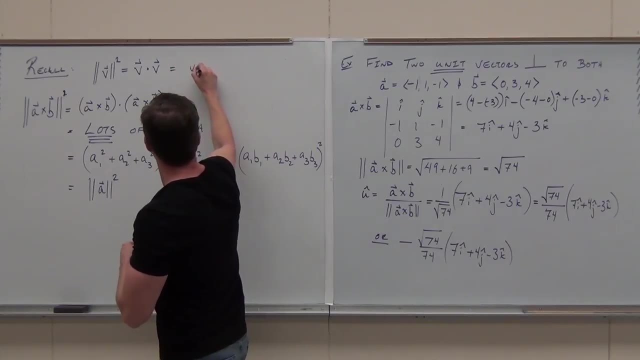 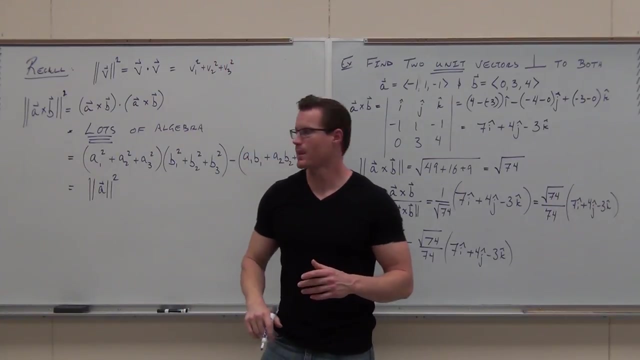 That's literally how we got. let's see that right there. That was one of those properties. This, Those are all equal. It was in a previous section, But that is the same thing as the magnitude squared: The first one times the second one minus the third one. 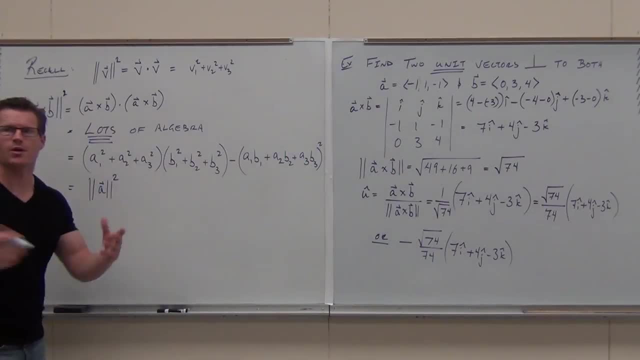 Minus. Well, let's keep on rolling. Come on, what's this one? then? You don't have to whisper, It's going to be the magnitude. If it wasn't squared, it would have to have a square root. Did you guys get it? 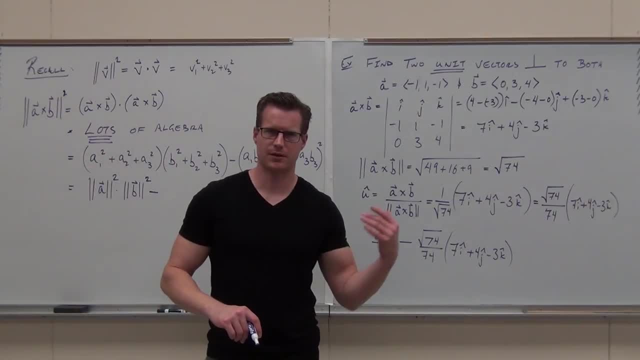 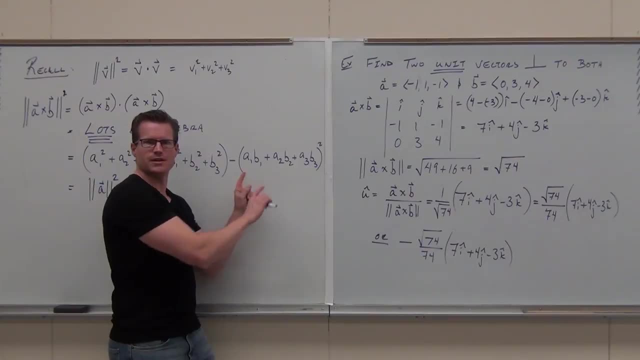 This one. I'm going to do it this way. You're going to have to just verify that this is true, But if you really look, if you're good at dot product, you can see what this is. This is the x components multiplied. 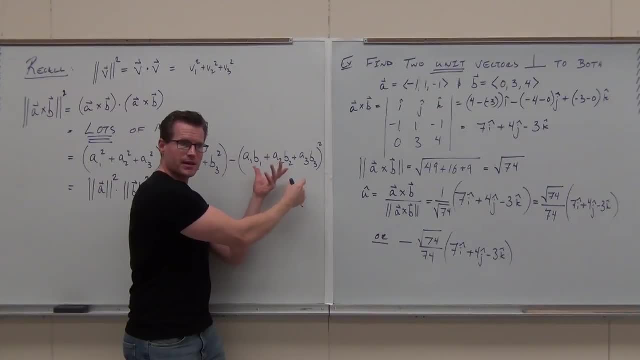 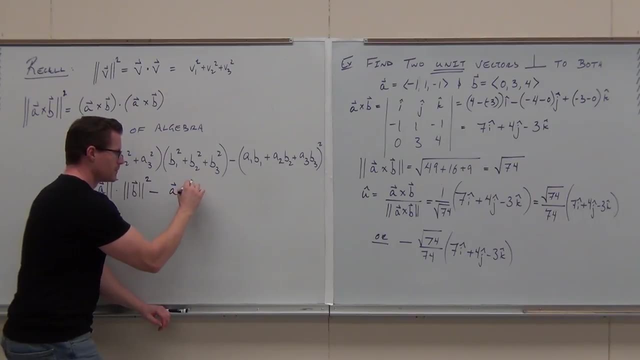 the y components multiplied, the z components multiplied and then added. That's a dot product Squared, This is the dot product of A1.. Try it if you don't believe me. A1 times B1, and then A2 times B2, and then A3 times B3. 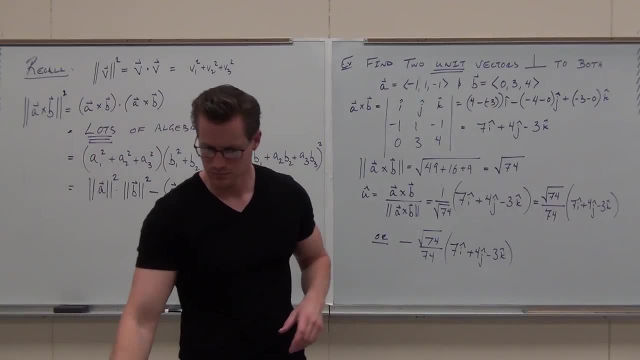 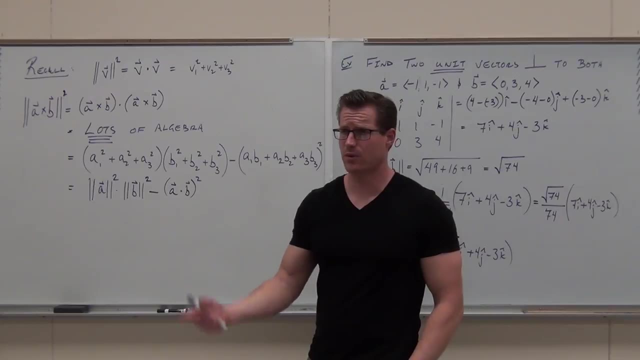 and you add them up. That's what that is. Y'all still okay with it? I know we're doing some crazy stuff. If you don't want to write down only the punch line, that's fine too. I don't really care. 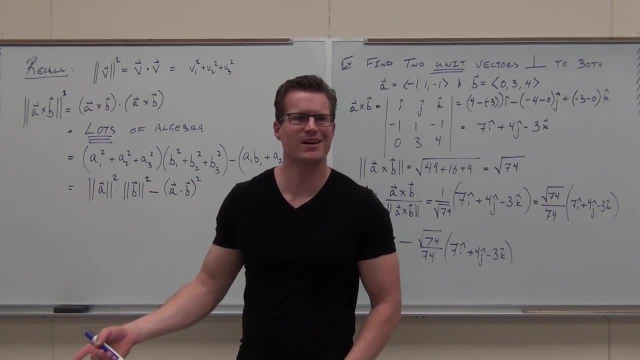 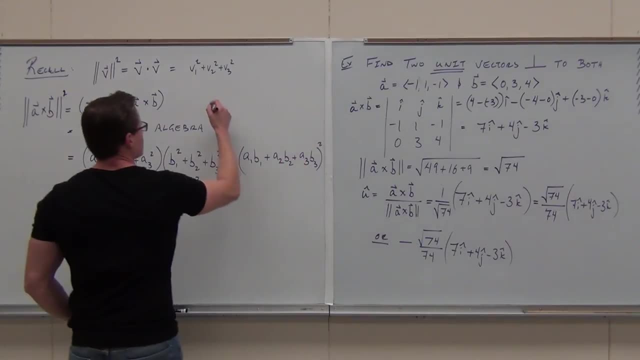 I just want you to understand where this comes from, Because if I just give you the formula, you know where does that come from. I want to show you One more thing, and oh man, I swear, we're almost there. Do you recall that one of the ways we could do a dot product? 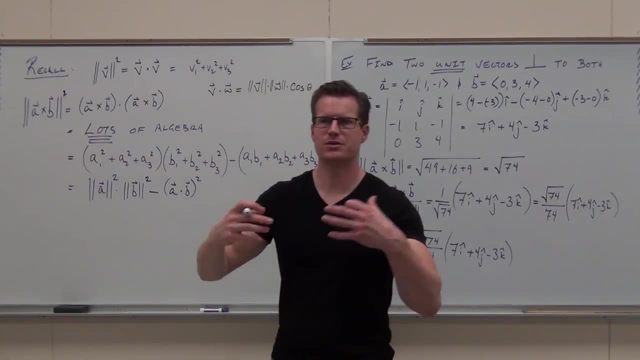 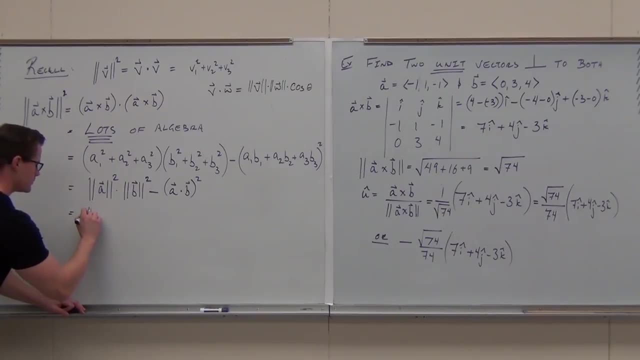 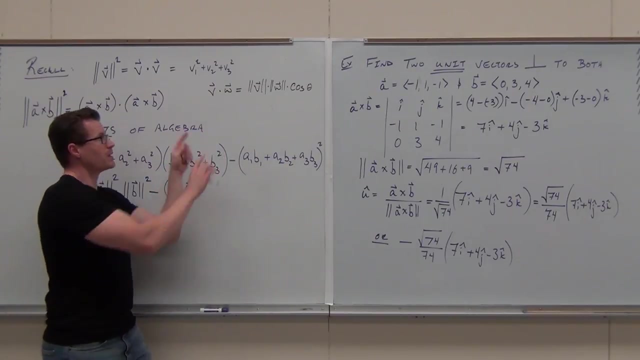 What is that? You recall that We had magnitude times, magnitude times the cosine of A in between them And what we have here. If this is now A and B, then we have- please just watch careful- we'd be squaring both sides of that to get down to here. 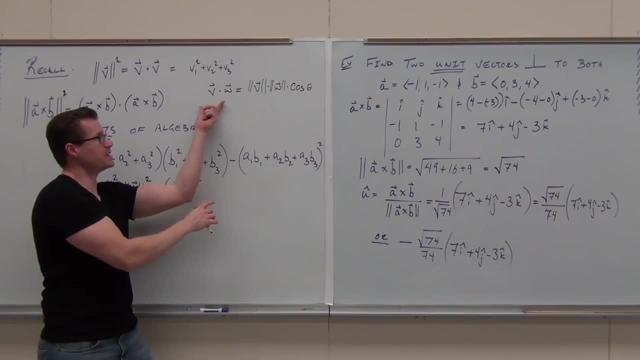 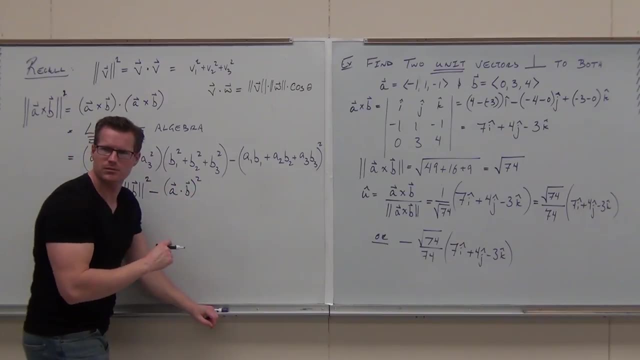 Does that make sense to you, Are you sure? So VW is magnitude B, magnitude W, cosine between them, A dot, B squared would be: you tell me. you tell me, left-siders, what would you have. Okay, Right-siders, what would you have? 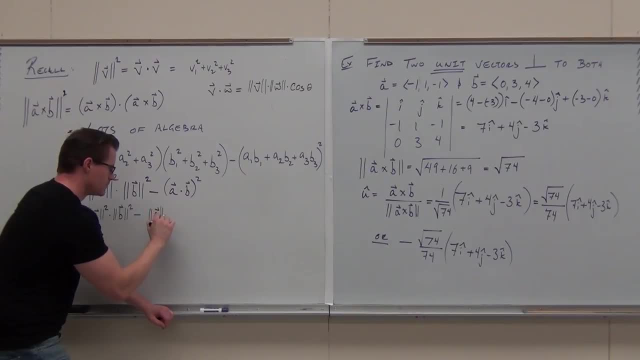 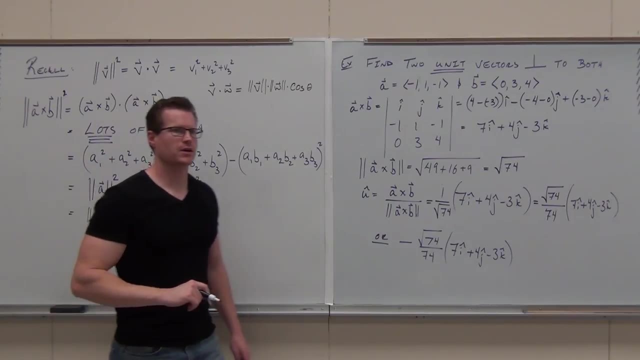 Magnitude A Magnitude A Times the magnitude of B times cosine theta. You're very, very close. I would get it. This would be, This would be exactly like this, but this is being squared. What's the square? due to all of this stuff. 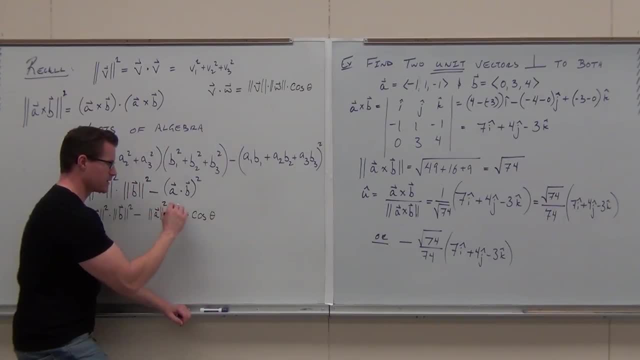 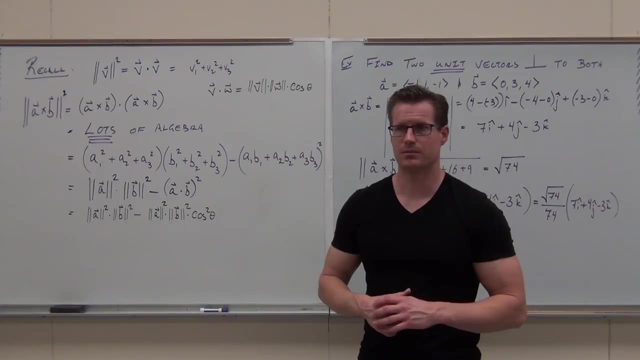 Square Because it's all being multiplied, I can say that square is applied here, it's applied here and it's applied there. Okay, still following what I'm talking about. I know we're doing a lot of algebra, but I hope that you're. 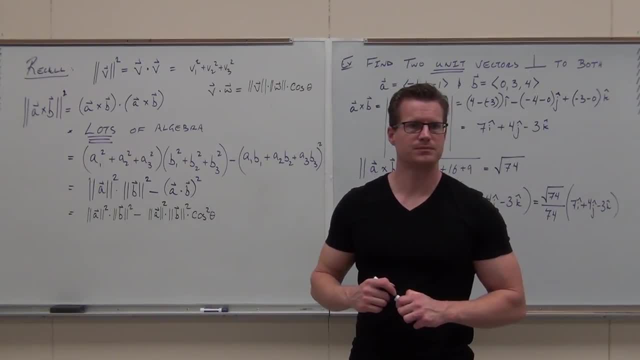 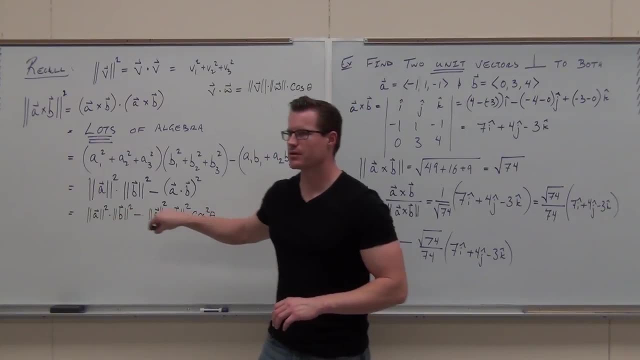 with me and not if you are, So okay, You guys ready for the rest. It's pretty cool, Check this out. How many big terms do we have here? Terms are things added or subtracted. How many terms do we got? 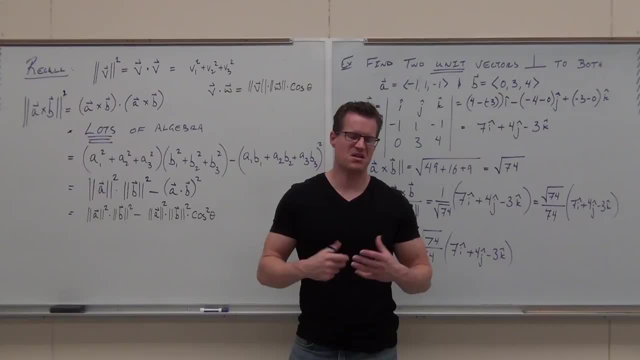 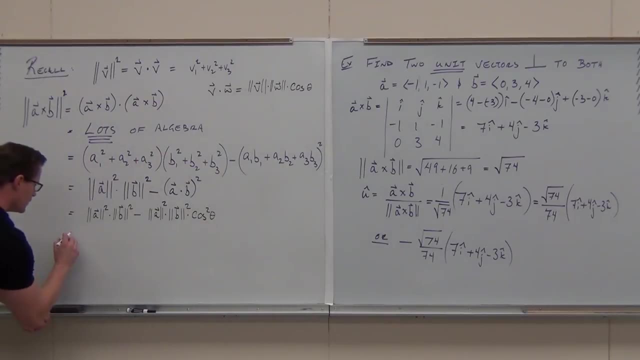 Two big fat terms. Do any of those terms have something in common in there? You know, let's factor it F word. you know, Oh, no, that's fraction, What? No, That's not a thing, That doesn't happen. 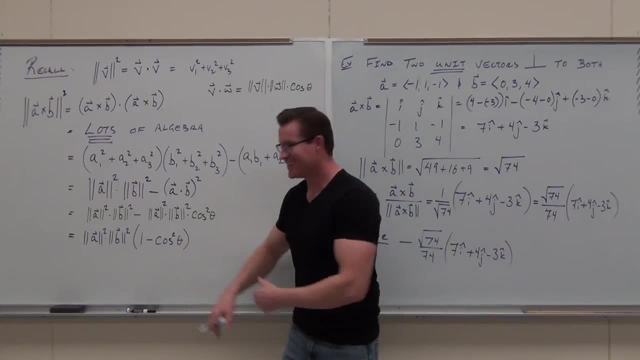 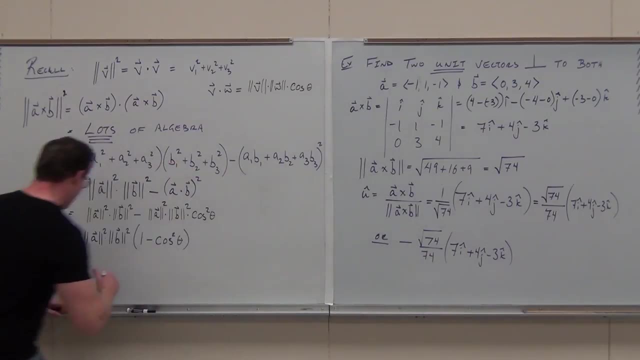 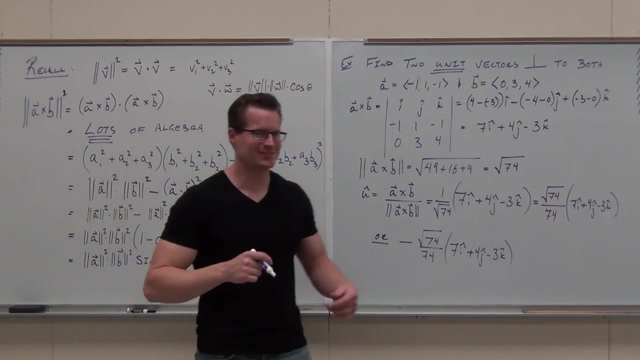 We don't get stuff like. We don't get stuff like that. Come on, you're in Calc 3.. What is that? That's not a great idea. That's cool. That's really cool. Now, I don't see the coolness yet. 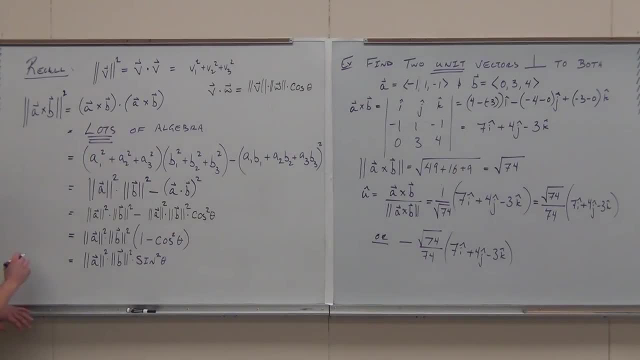 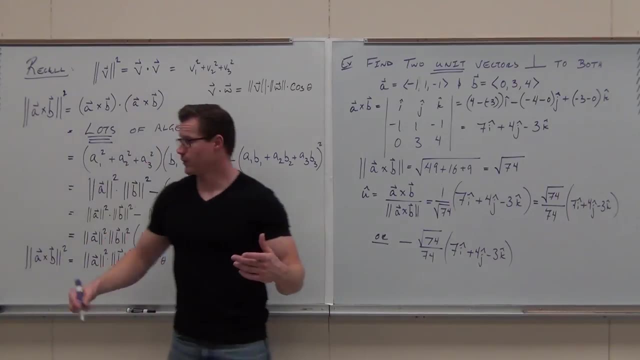 Don't worry about it, it's going to get chilly. Cool, That's cool. So what we started with was the magnitude of the cross product squared. That's what we started with. That's what this whole thing is equal to. 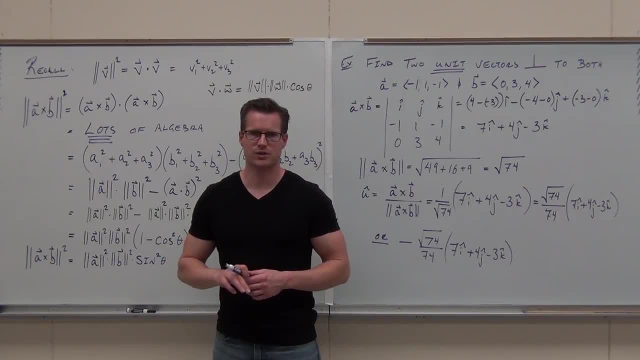 Are you getting what I'm talking about? Everybody in class right now. how do you get rid of a square? How do you do that? Can you square root both sides? Yes, Yes, Absolutely You can. Magnitudes always positive. 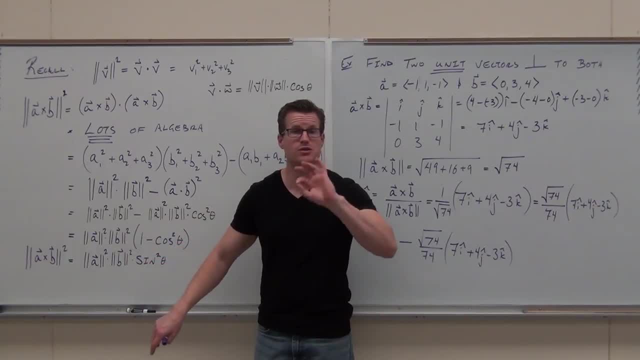 Magnitudes always positive. Magnitudes always positive. I don't have to worry about the plus or minus thing, because I don't care about the plus or minus thing, They're always positive. This guy we're going to talk about in a little bit. 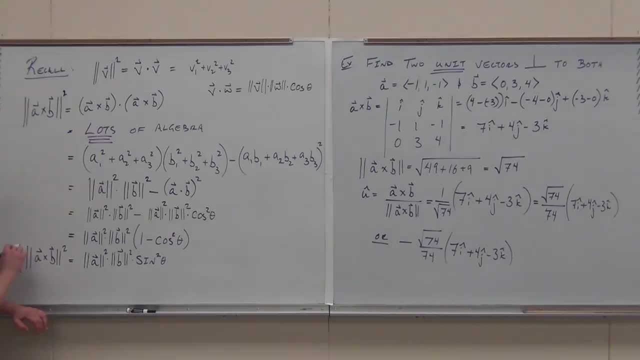 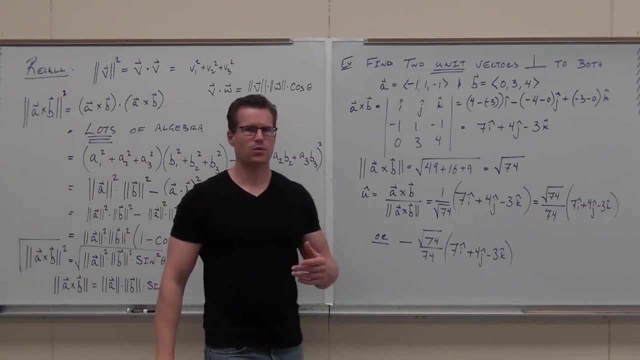 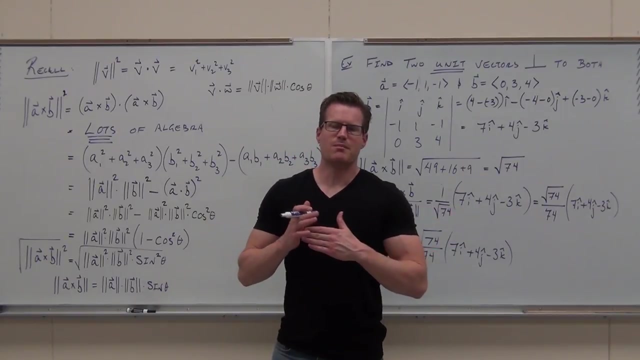 But if I square root both sides, If you're wondering if that's legal, why sine stays positive, I don't have the plus or minus. I need you to think back to the definition. It was right over here. Do you remember that? for a cross, you remember, you remember, you remember. 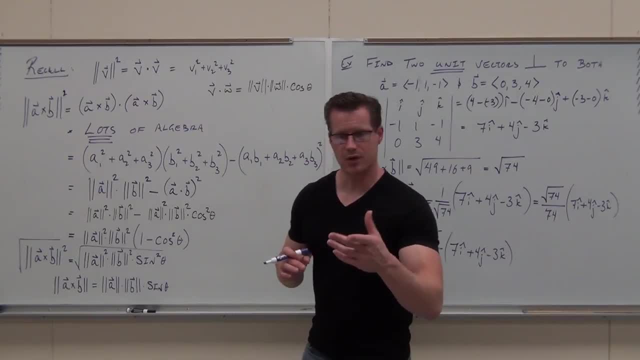 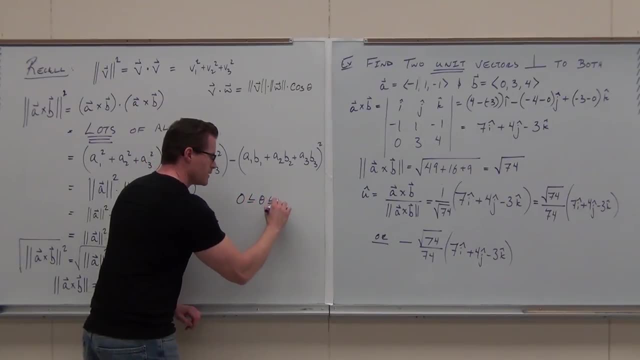 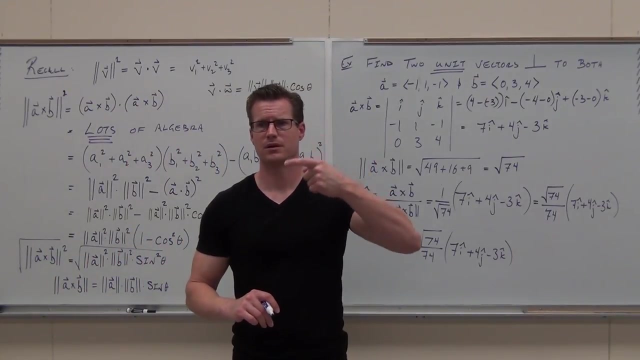 Zero to pi, Zero to pi. So for cross products, little sub note. okay, For cross products theta is between zero and pi. Tell me something about sine for any angle between zero and pi. Always positive, Always positive, Always positive. 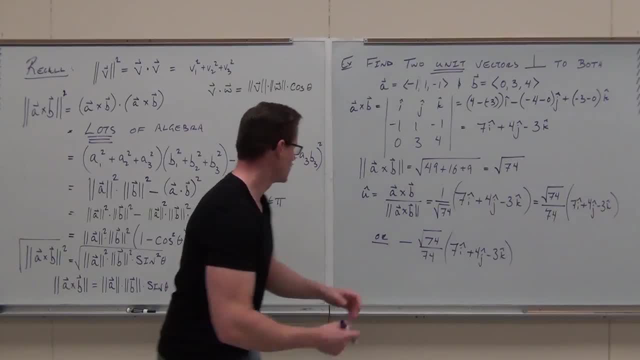 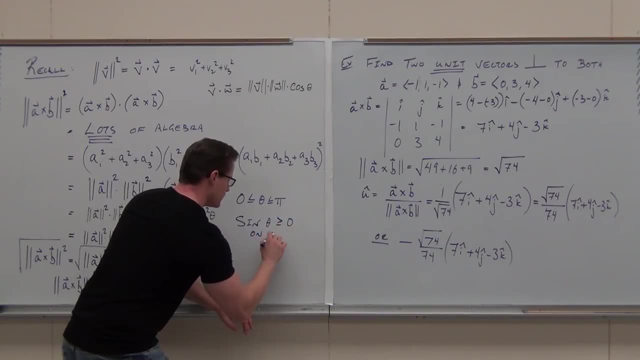 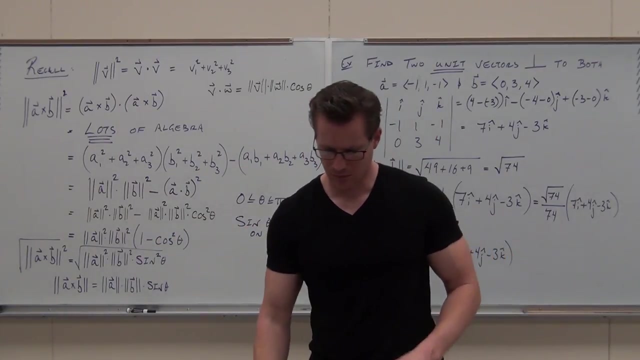 So when I take the square root, it's an always positive number. I don't have to worry about the negatives, Which means when I take the square root, we're all good to go. You still okay with what we're doing so far. 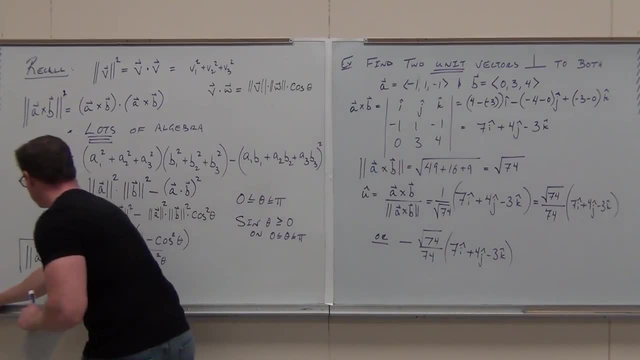 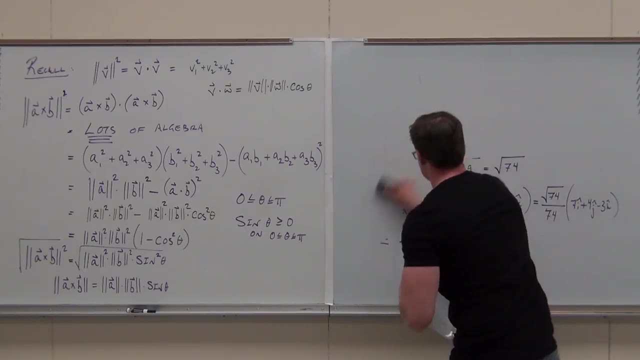 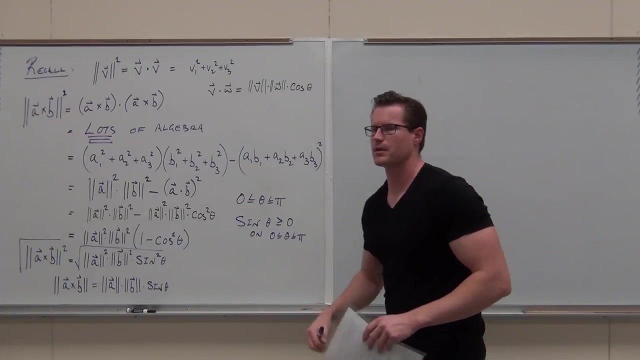 We're almost done. I swear It's been a lot of, lot of proof. Okay, I want you to feel the tension. This is the one you're holding on to, But it's it meant, it's the cool part. it's the cool part. 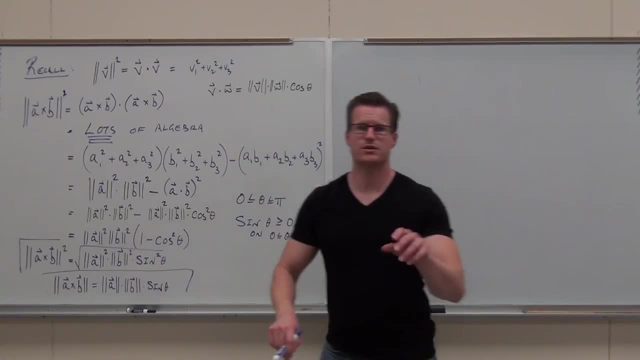 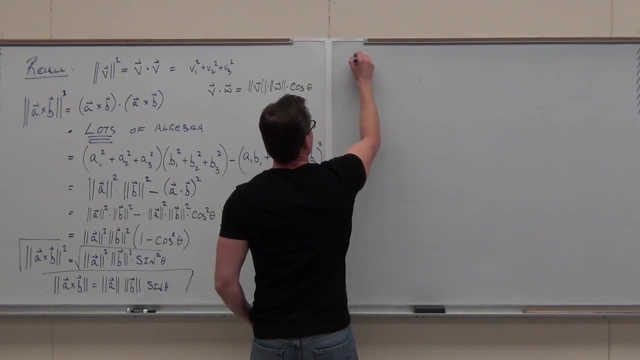 You believe this right Because I proved it. I hope it's the cool part. Now here's the deal. what we know is that any vector in the world can be written like this: The magnitude of the vector times the direction of the vector. 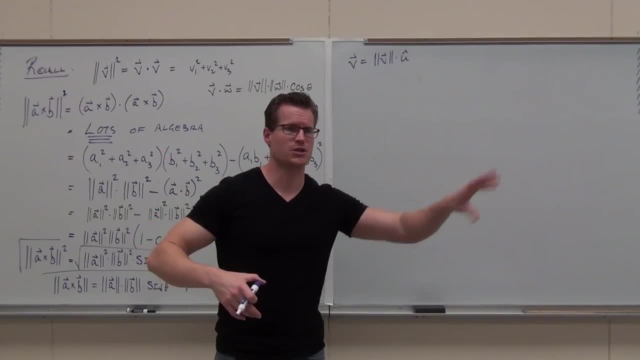 Vectors are magnitude times direction, so it can be written as magnitude V times a unit vector of the direction of V. Are you with me on what I'm talking about? Okay, so so wait a minute. is A cross B a vector? 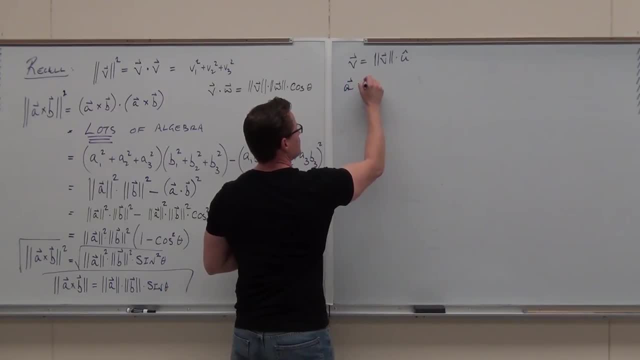 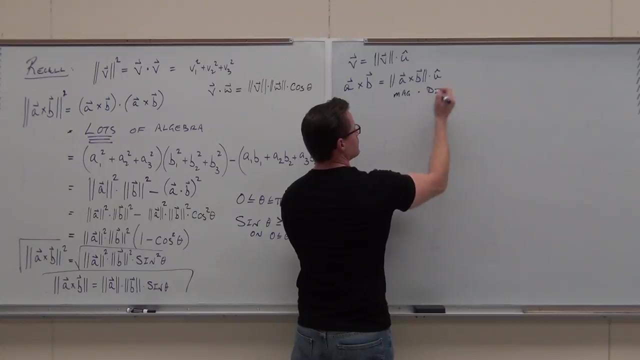 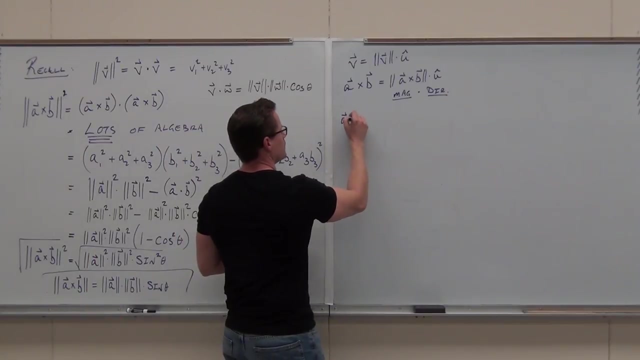 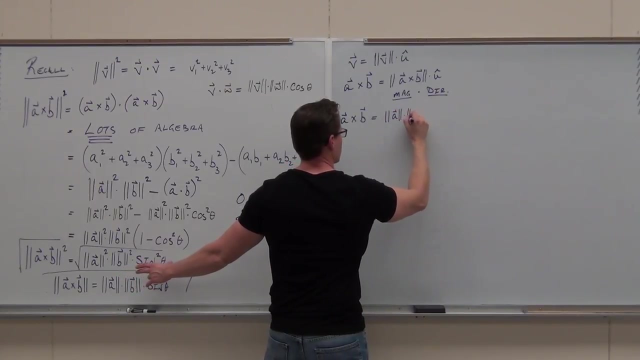 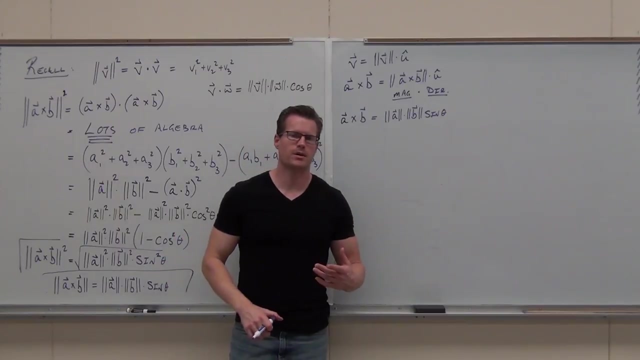 Yes, yes, Then A cross B can be written as the magnitude of the vector, times the unit vector. And what is the direction of the vector? Magnitude, times direction. But wait, we've got a formula for that now. The reason why I'm why I'm doing this is because I'm going 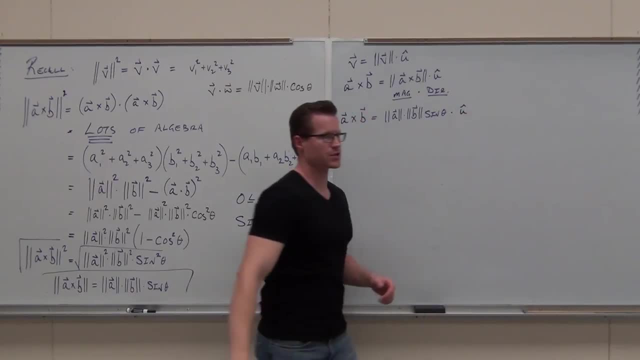 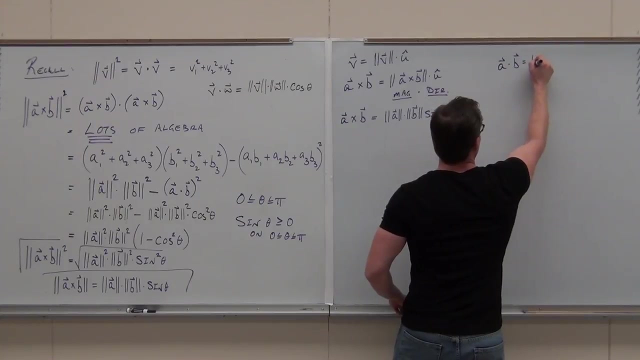 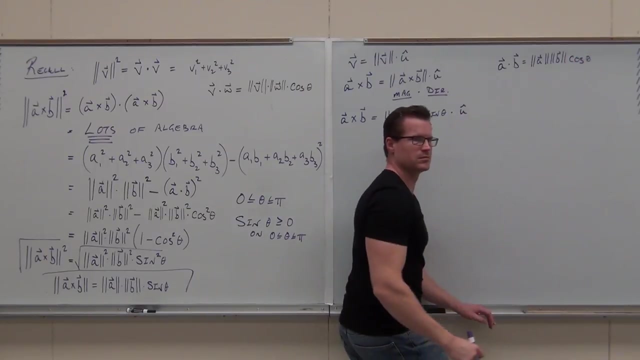 to become a parent in just a second. But do you guys see a similarity here? Do you remember the dot product? We had it earlier, the dot product of A and B? What's that thing? Do you remember that, The dot? 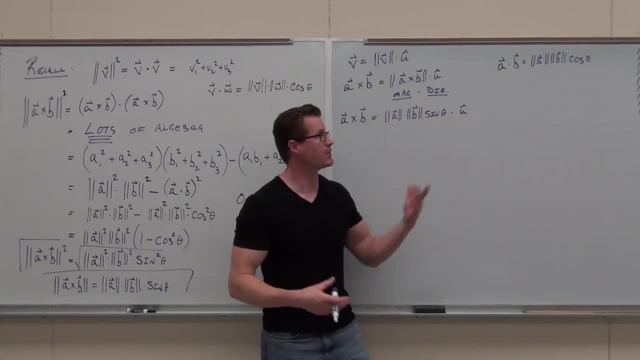 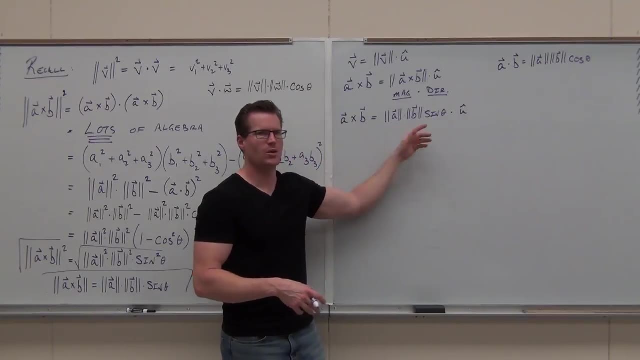 The dot product. that's really similar. We just had the sine versus the cosine. Now this gives us a scalar, this gives us a vector, But that holds the vector right there. just the U, just the direction, So that that's. that's pretty cool. 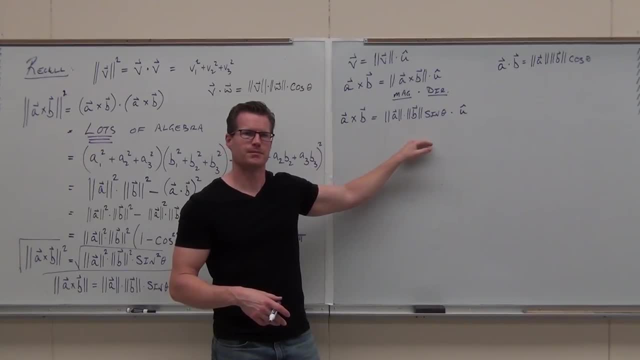 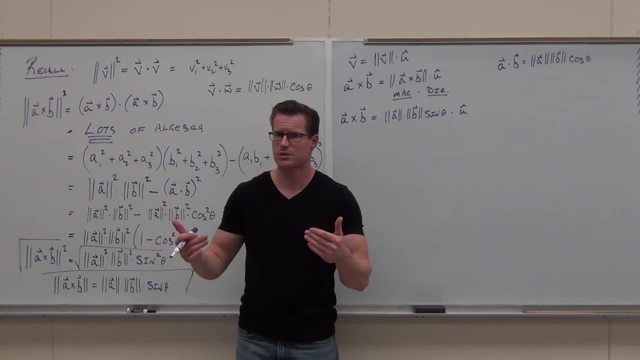 This is the other way that you can calculate the cross product, if you know the angle between the two vectors, And, and you can find the magnitudes right. So if you know the angle between the two vectors and the magnitudes, you don't need to know the unit vector. 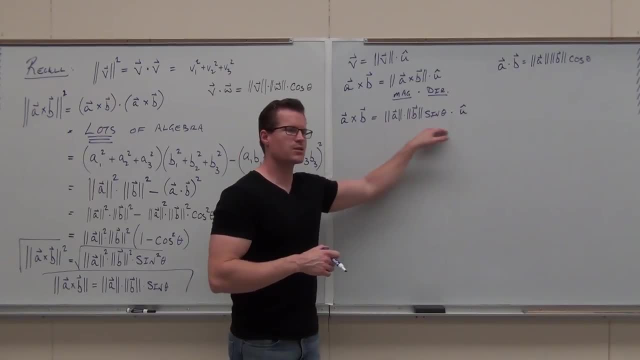 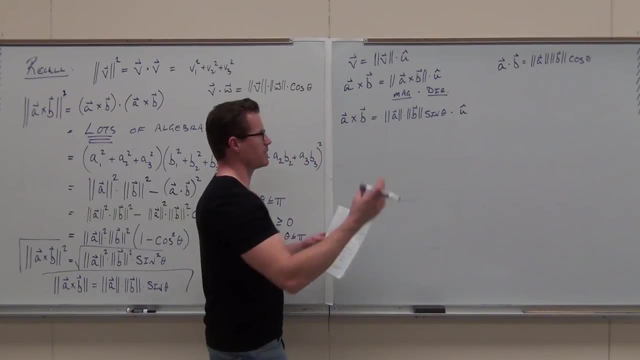 of the of the cross product, But that's another way that you can do it. Now here's what I want to talk about: the big old, big old punchline. So we got, we got two ways. now We got this way for vectors with angles. 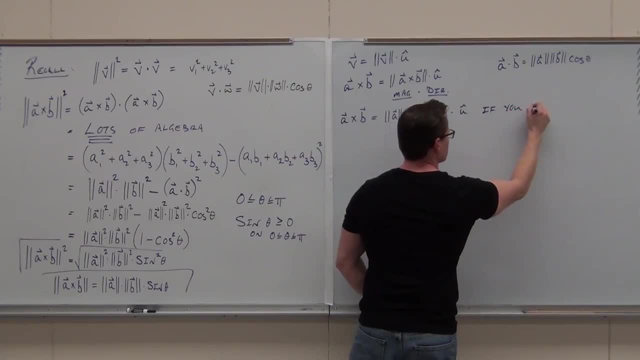 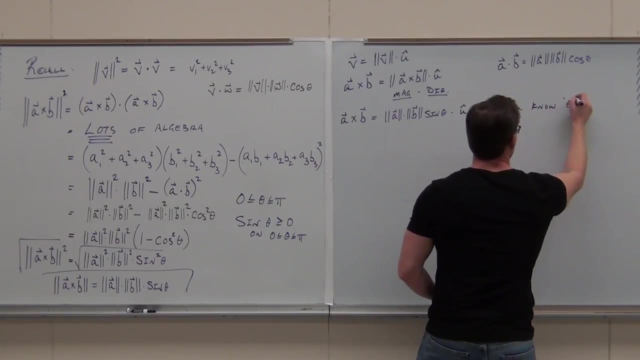 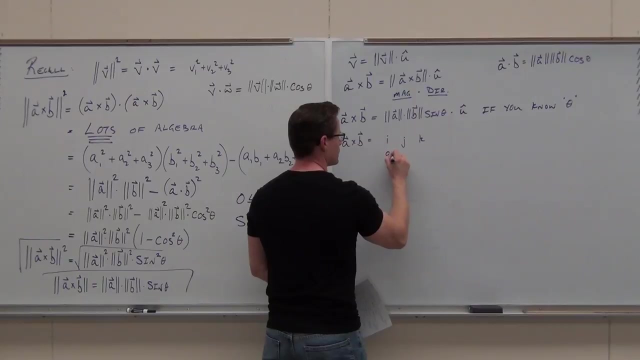 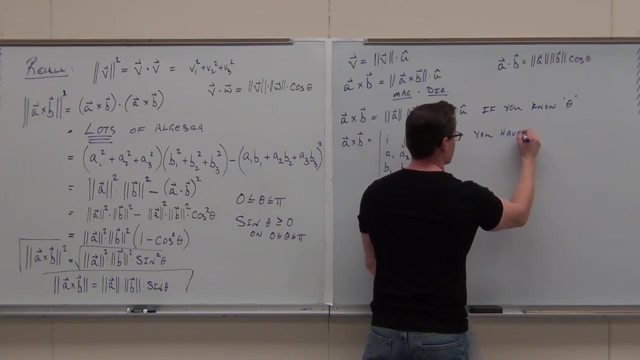 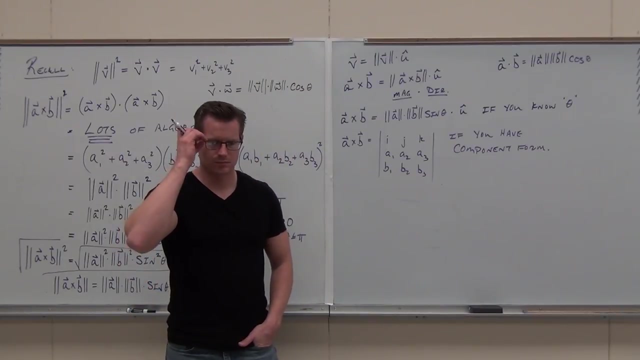 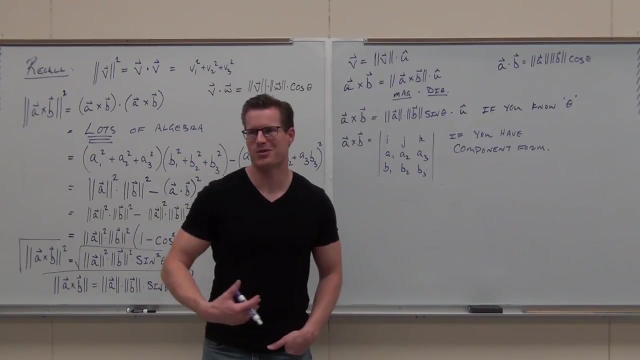 So if you know theta- And we had this way- If you have a component form, There's just a little bit more. I promise, I promise this time I really promise. I'm not even going to break my word. I promise we're almost done here. 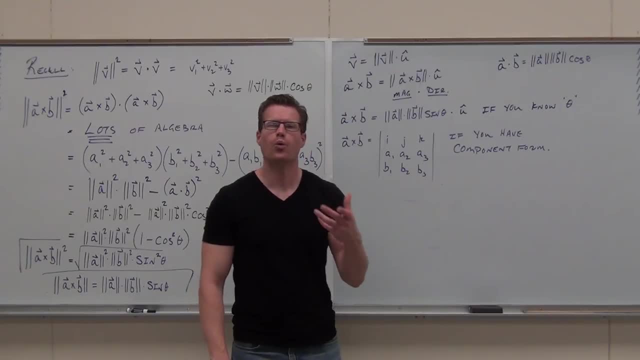 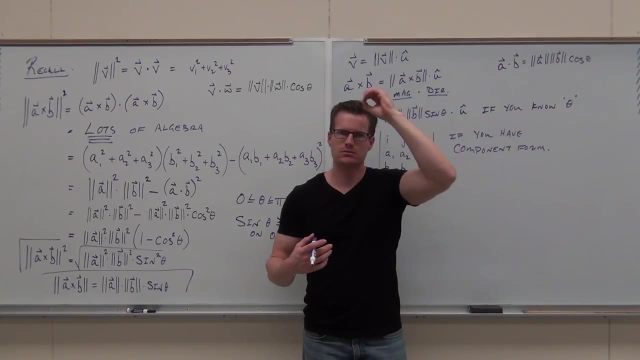 There's a big question. We know what happens. Oh, come on, stick with me here. What happens if a dot product is settled? What happens if the dot product is zero? We knew that right. Think through it: If the dot product is zero, the only way that happens. 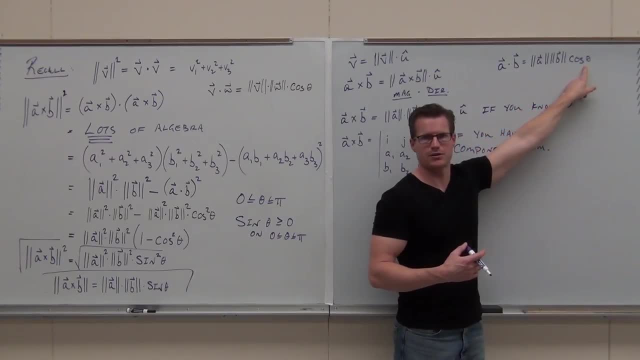 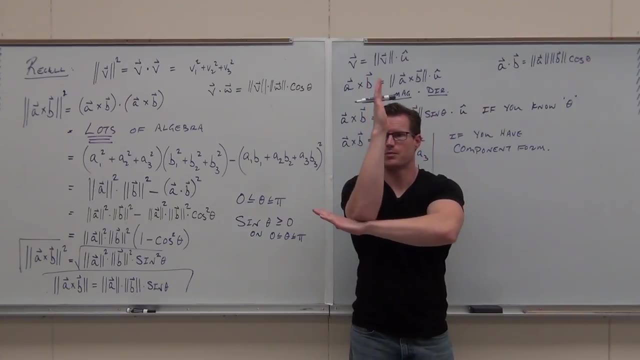 with non-zero vectors is when cosine is pi over 2.. Tell me the angle of pi over 2.. Come on, angle of pi over 2, what is that? If the dot product is zero, we have perpendicular. Are you following what I'm talking about? 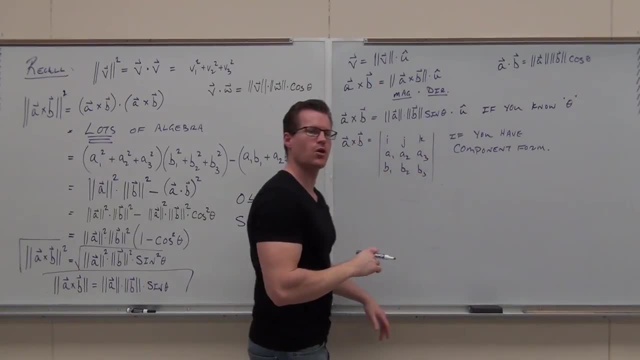 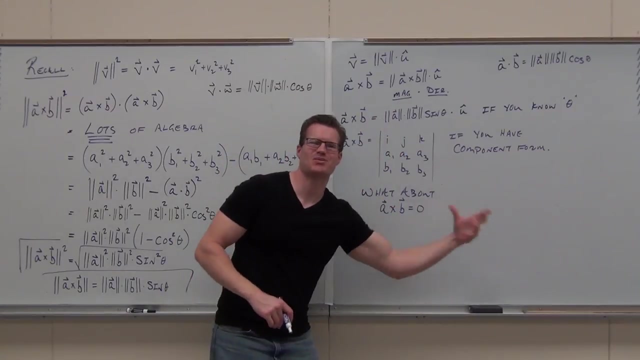 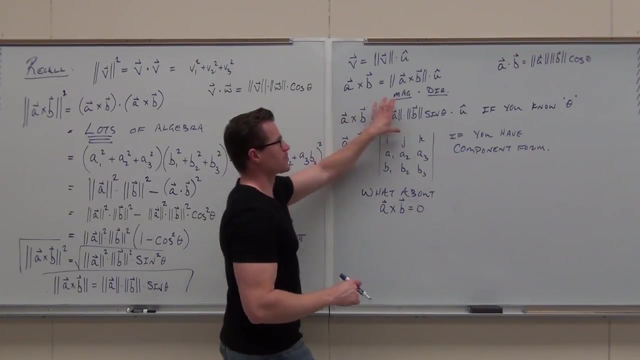 This is the one way we know What happens if the cross product is zero. The whole reason why we did this was so I could prove this little piece right here, But it's pretty neat, It's pretty cool If the cross product is zero. this is the cross product. 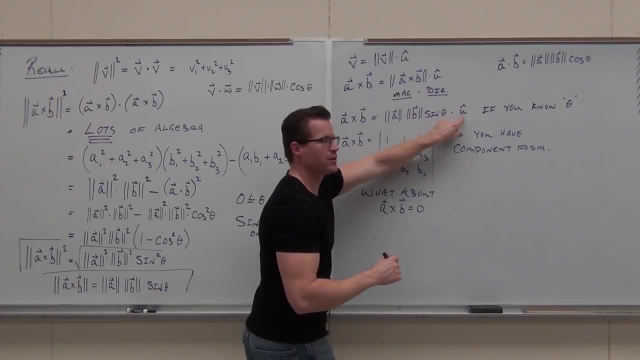 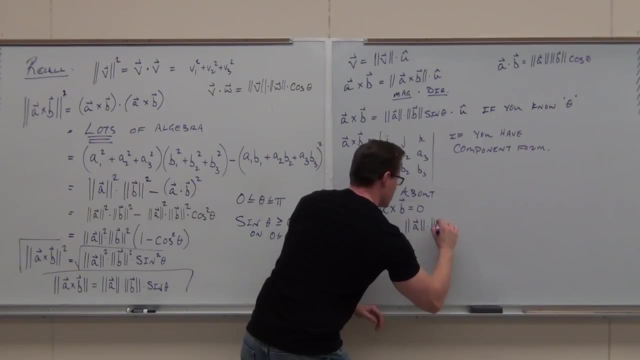 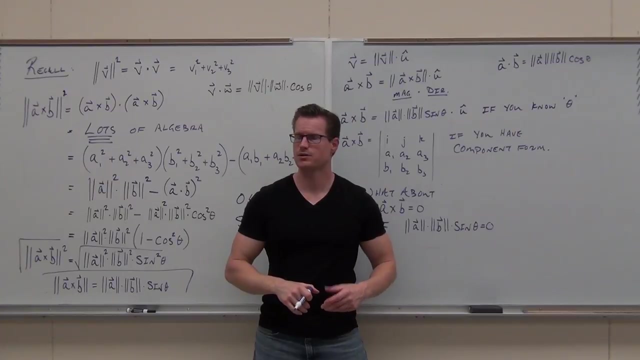 The only way that happens with a non-zero vector is if that's zero. That's the only way it happens. Do you guys see what I'm talking about? If the cross product is actually zero and you have a non-zero vector, so it actually has some substance to it. 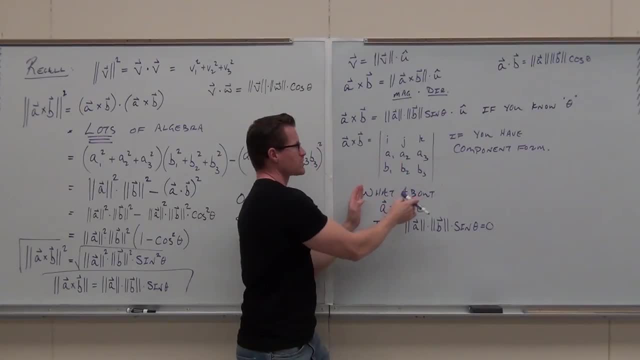 the only way that that happens is if this part is zero. So if the cross product is zero, it means this part has to be zero. But wait, If these vectors actually have length, these are not zero. It comes down to this. 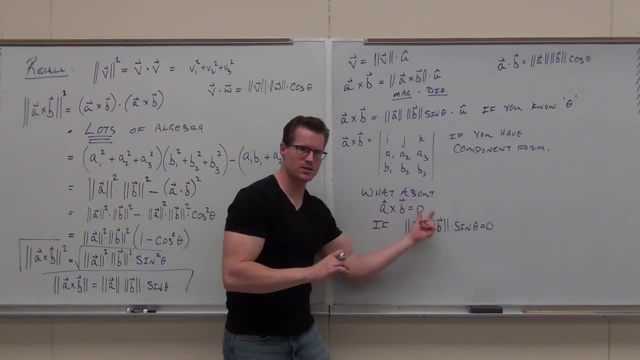 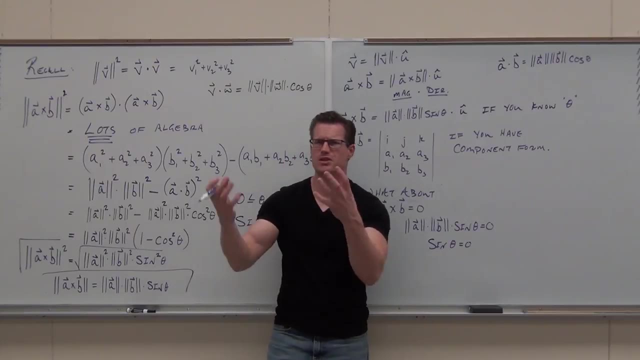 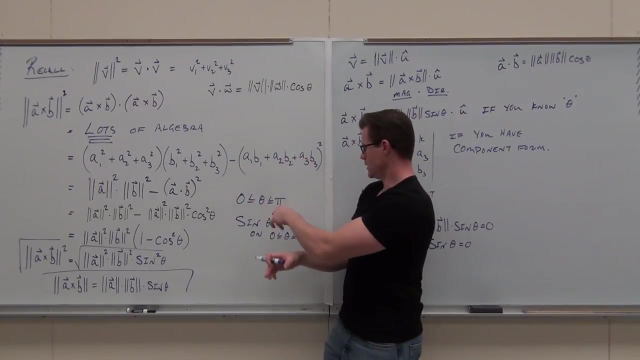 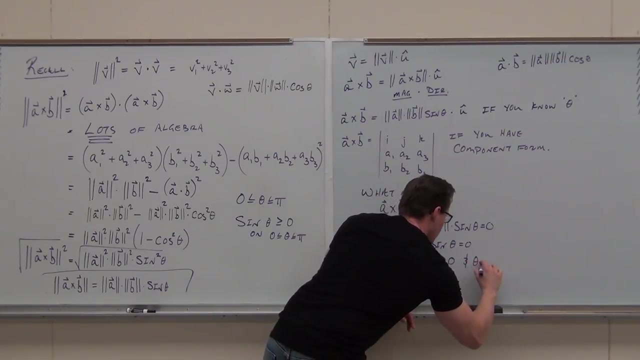 This can only happen. the cross product can only be zero if sine is zero. You tell me, Let's think about it. Put it together: Where is sine zero? And remember that we can go from zero to pi, but sine zero only at zero and pi. 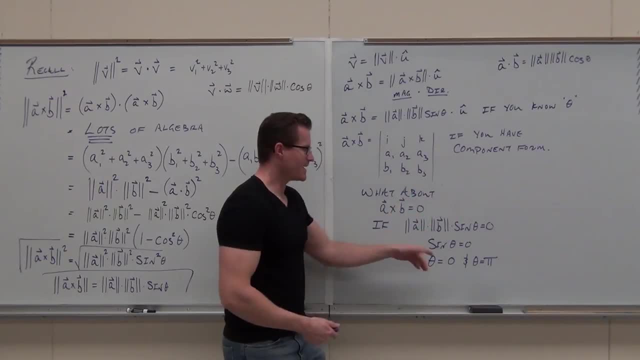 You follow me. Let's put it all back. Let's go backtrack. Hey, if sine is zero or sine is pi, we're going to have zero, We're going to have a cross product of zero. This is the only time we ever get a cross product of zero. 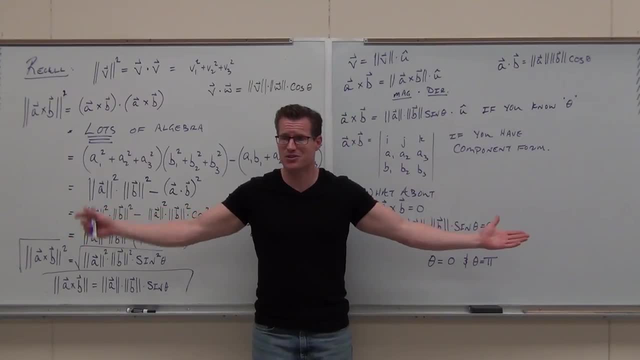 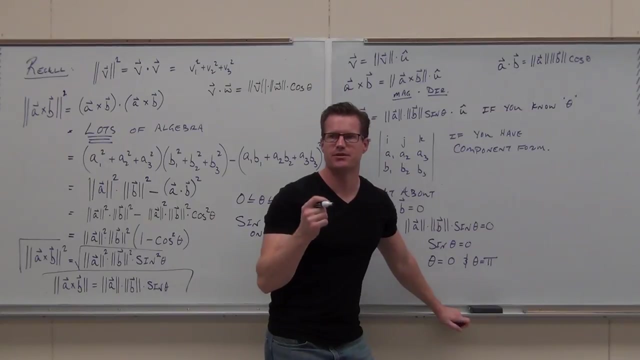 is if sine is zero or pi. Tell me what two vectors are: at zero or at pi. What are those two vectors? They're parallel. That's the point. What? That's pretty cool. So we have two pieces of information, One we just recapped and you know it. 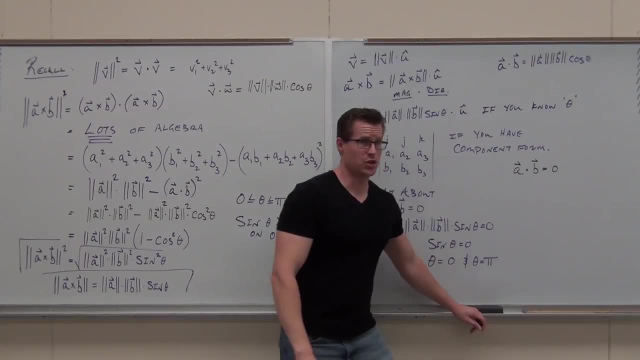 You should know it. What happens if A dot B is zero? What do you know about A? Not about the angle, I mean about the vectors. What do you know about the relationship between the vectors? What do you know? They are orthogonal. 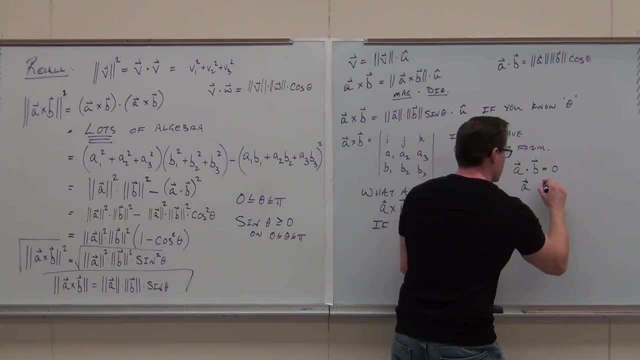 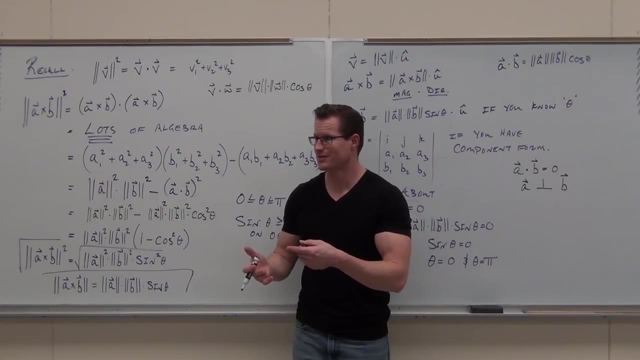 They are perpendicular, They are normal. That's basically what we know. A and B are perpendicular. Does that make sense to you? We just talked about it. What do you know if you do the cross product and you get zero? Or what happens when you take vectors that are this situation? 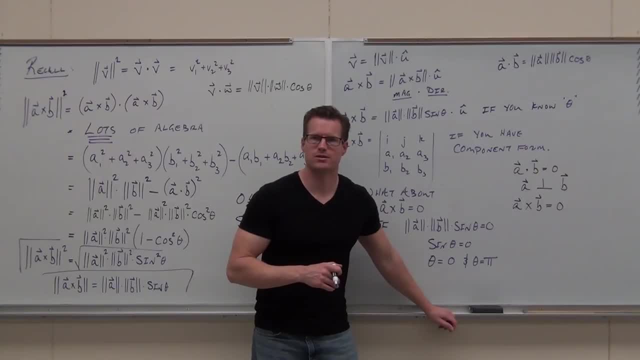 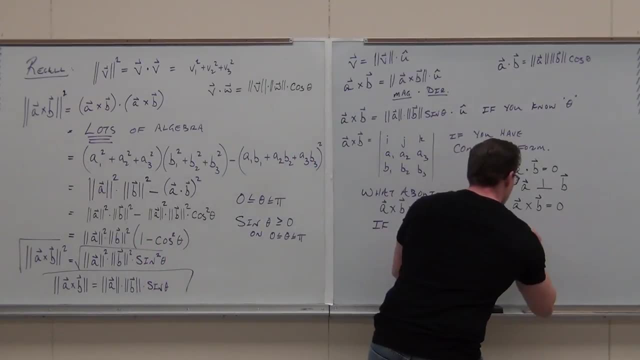 and cross product them, You're going to get zero. What are those two vectors? if the cross product is zero, They are parallel And they have to be, because only when it happens is if sine is zero or pi. Can I tell you something and you not get mad at me? 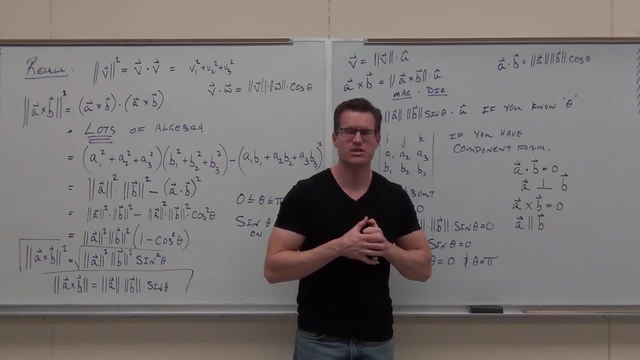 You're still going to be mad at me. probably just a little bit. This is the only way you ever check whether vectors are perpendicular, right here. Please don't freaking use this to check whether vectors are parallel, because still it's easier with scalar multiples. 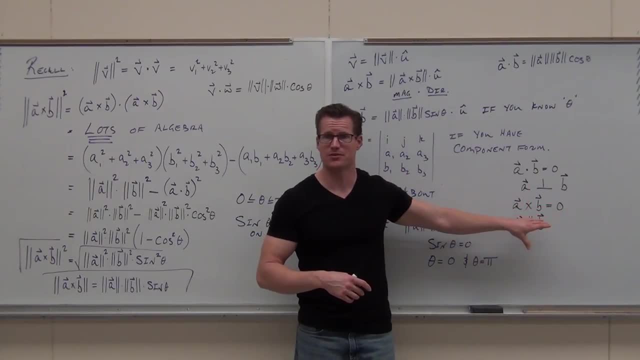 All right, We're going to use it. I promise we're going to use it for something called torque, But you still wouldn't use this to check whether vectors are parallel. Does that make sense? It's just a condition, It just happens. 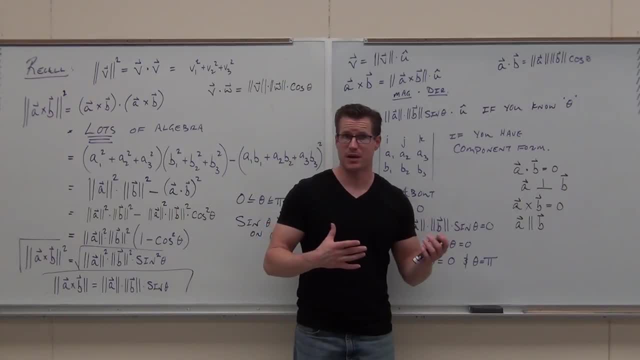 If the cross product is zero, you know the vectors are parallel. If the vectors are parallel- this is probably the most important, more important case- If the vectors are parallel, you don't need to bother finding the cross product. That's why we're doing it. 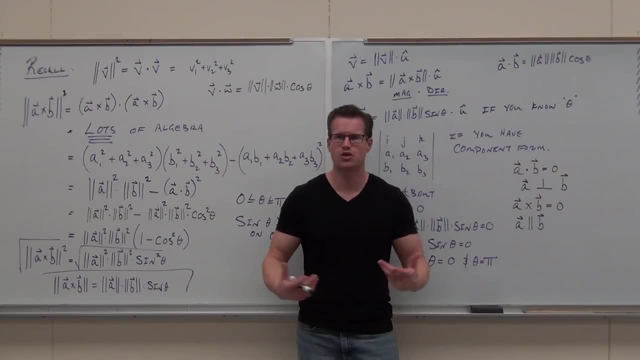 So if we know this, the cross product will be zero. Don't bother because the angle is zero or pi, You're going to get a cross product of zero. Does that make sense? Yeah, So how do you check whether two vectors are parallel? 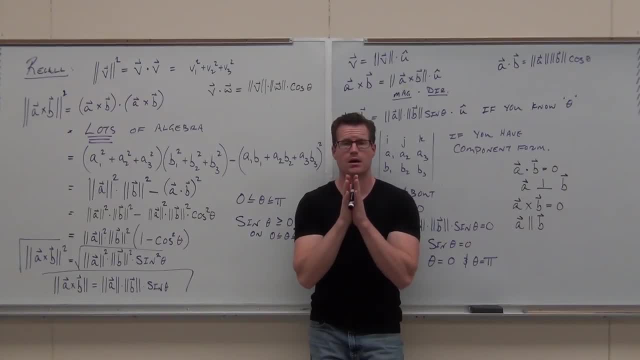 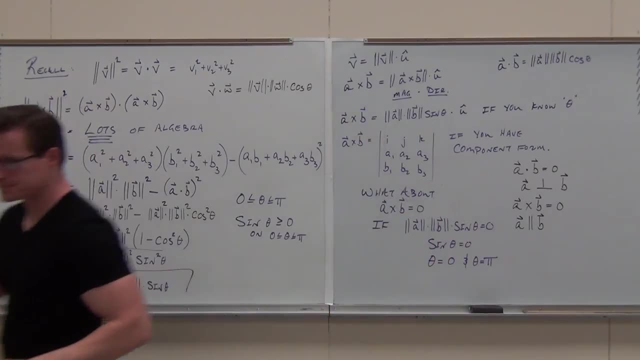 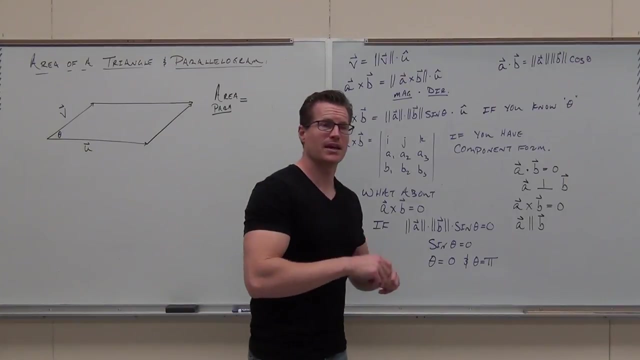 What would you use? Scalable- Scalable- Can you tell me how you check whether vectors are perpendicular? Still, That's where we're going to take a break. So, area, You're like wait, Does this actually do stuff? 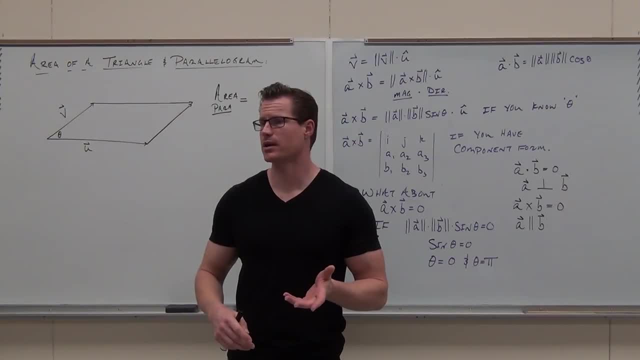 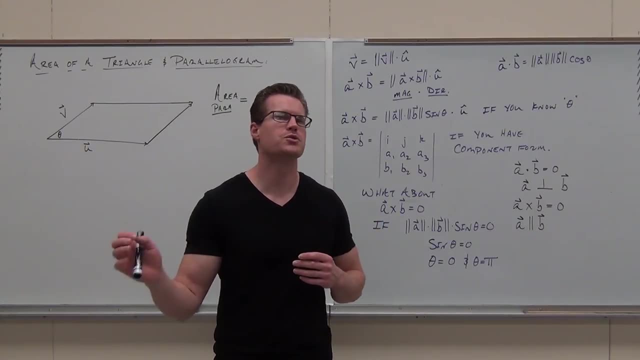 It does stuff. We're going to prove a couple things that it actually does right now. So we're going to talk about area of a parallelogram, area of a triangle, volume of a prism. We will talk through some of the properties. 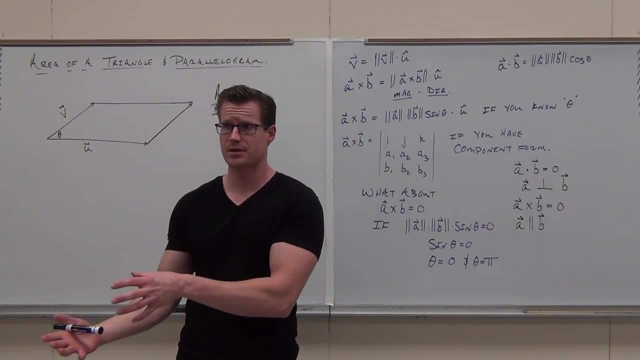 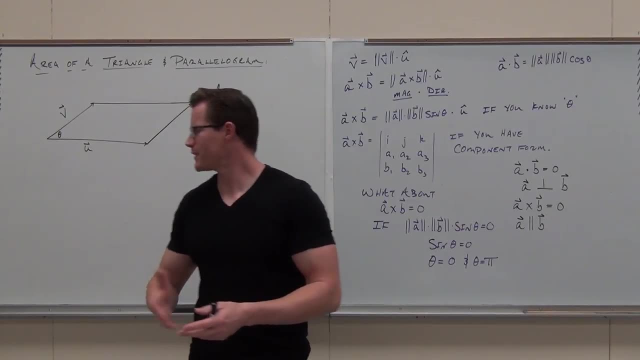 We'll do one example illustrating those properties, illustrating those properties, and then we move on to torque and I give you that proof that I said I was going to hang on to, okay, So let's talk about area of a parallel, very geometric idea, area of a parallelogram. 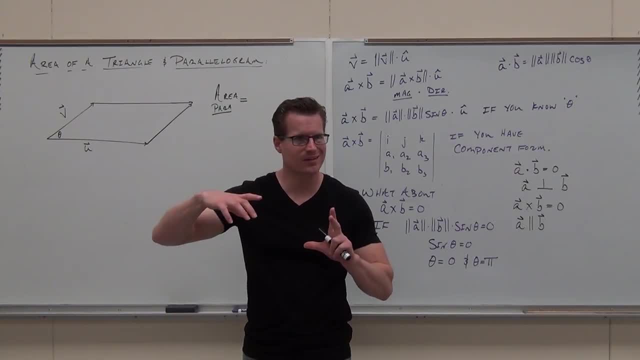 And in fact we know what area of like a rectangle is and a parallelogram has the same exact formula for the area. It's simply base times height. It's just the height. that's funny, because this is no longer the height. 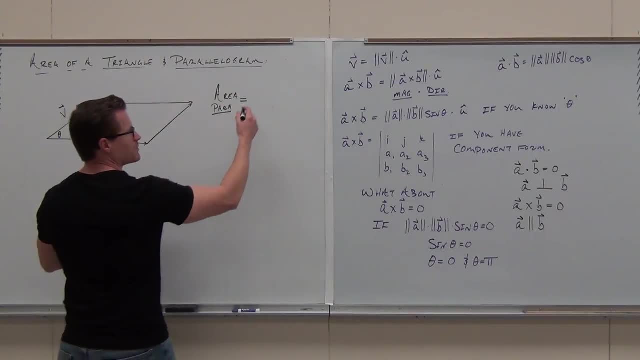 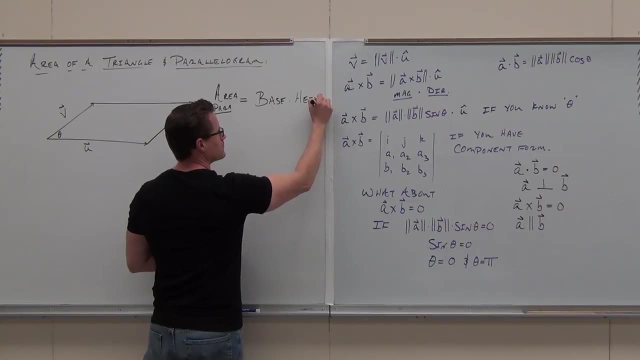 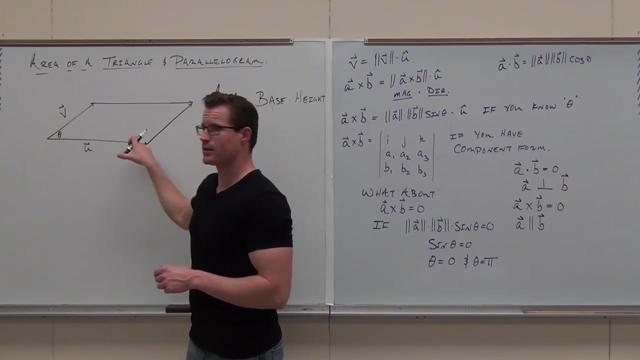 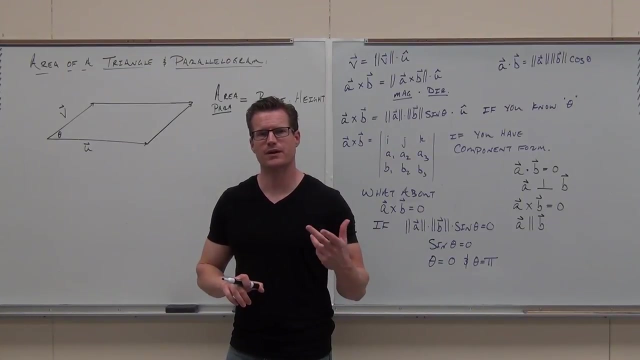 This is, like you know, a diagonal, So area of a parallelogram is still base times height. Now, you people out there, if this is my parallelogram, what's the base? U, U? No, It's not U, because U is a vector. 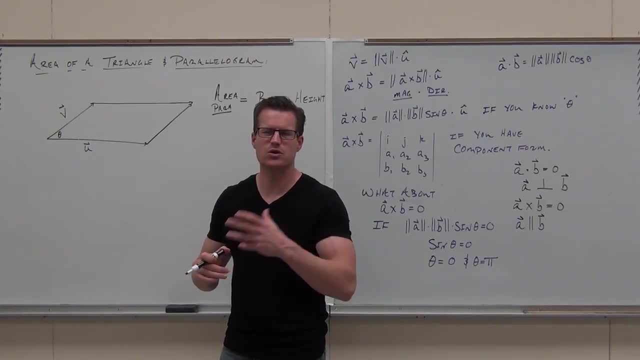 and U has a direction and a length. You can't be the base that we use for a computation, okay, because it's a whole vector. So I'm going to ask you again: what's the base? The magnitude, The magnitude of U. 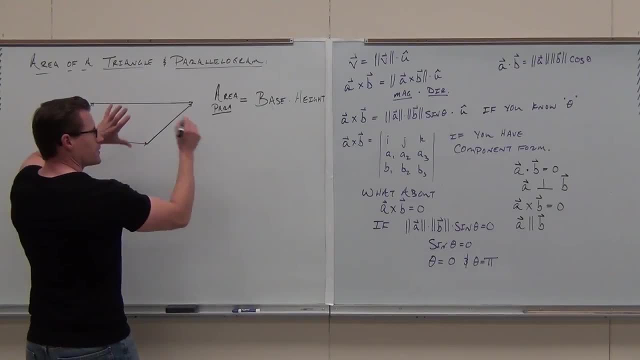 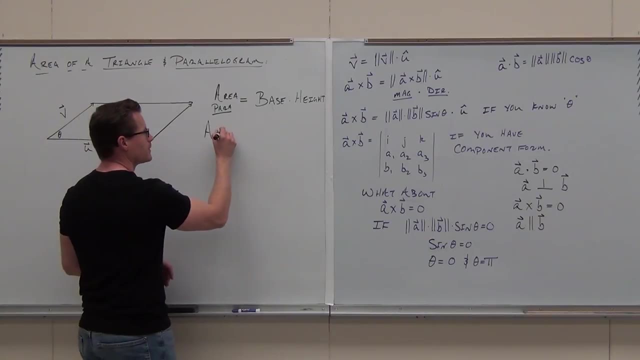 That's right. So the length of U would be the base here. So for us, for this parallelogram, I'm going to call it A sub P. okay, A sub parallelogram. Would it be base Sure Times the height. 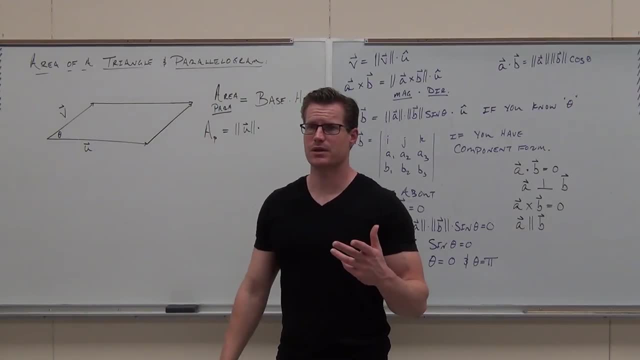 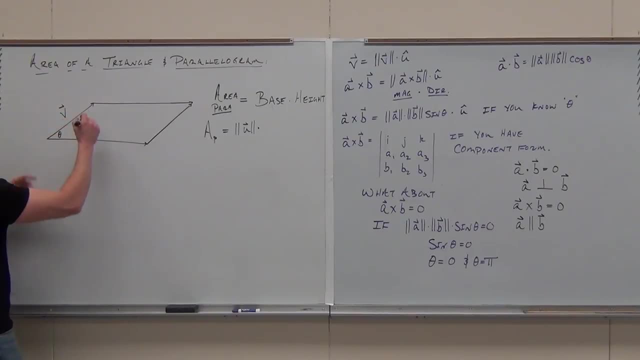 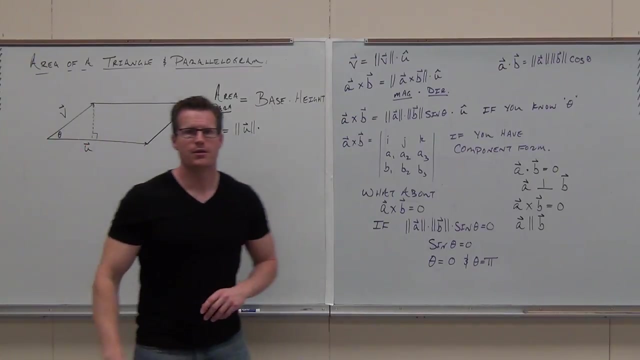 Now, okay, wait a minute. The height, True or false? the height is the magnitude of V. No, the height has to go from here to here. Or in other words, if I drop this, if I drop that, the height would be the distance of that dotted line. 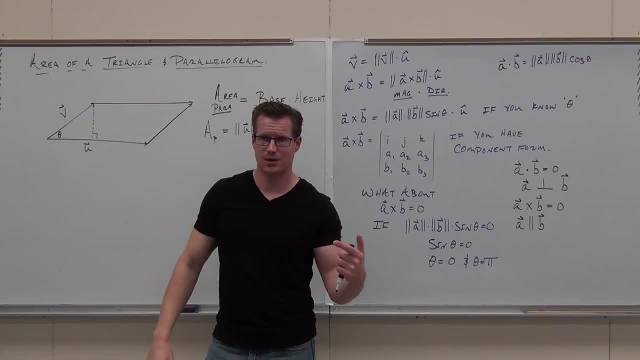 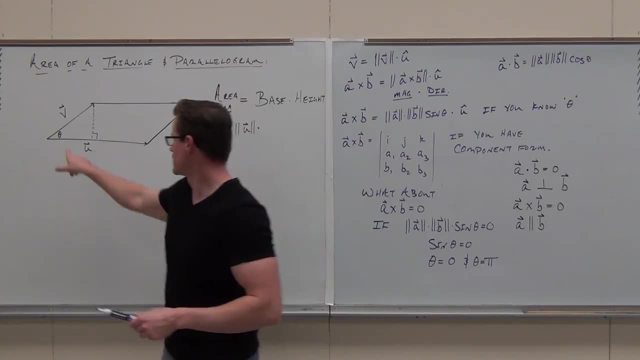 That's what the height is. Now, if we have an angle right there, which we do, let's see, you guys know this thing called right triangles. right so, right triangles. so here's our angle, Here's, I don't really care. 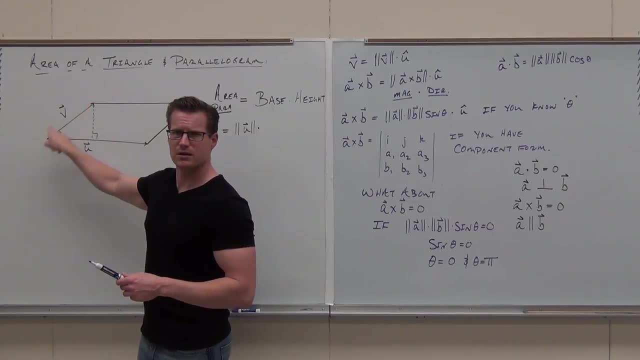 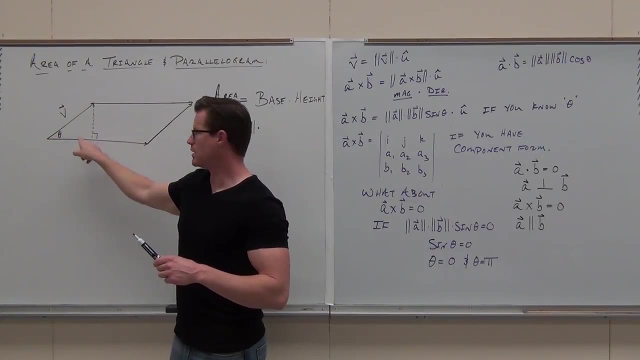 I'm focused on these two sides. What's this side? as far as a right triangle is concerned, Magnitude, Hypotenuse- And this side would be the adjacent to this one. This side would be the opposite. What relates the opposite to something that I already know: the hypotenuse. 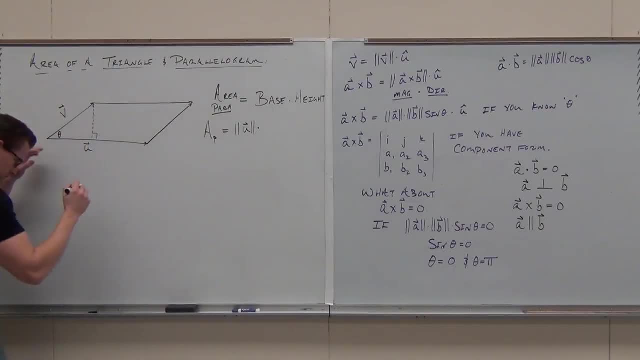 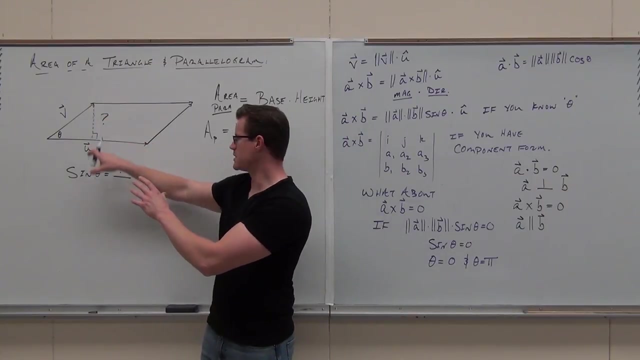 What relates that Signs? Okay, So this right here, Let's call that question mark just for a second. Sine theta is opposite over hypotenuse, correct? So it'd be question mark whether that happens to be over. what's this thing? 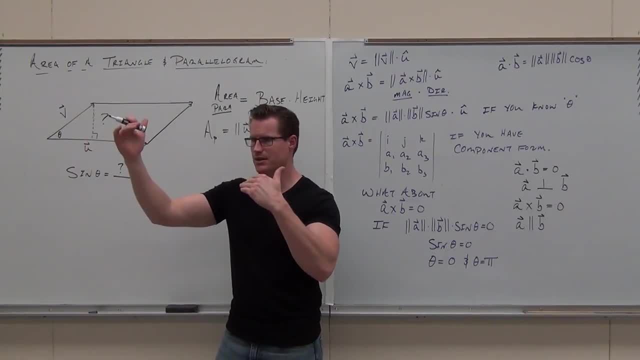 Magnitude. Yeah, it's not V, It's just the magnitude of V, Just that length, the length of that side. That's how trigonometry works: the lengths of sides. Do you guys get what I'm talking about? 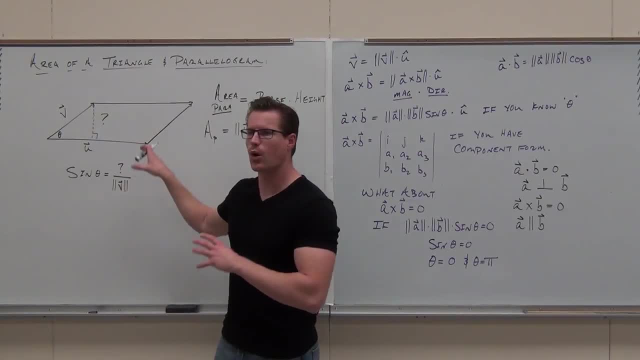 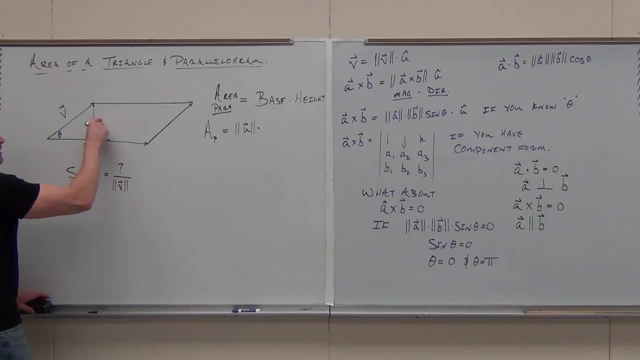 It's weird because we've got a question mark, but I want to put the thing up here. So if I solve for a question mark, Basically, just multiply both sides by the magnitude of V, We have this side. Magnitude of V times sine theta. 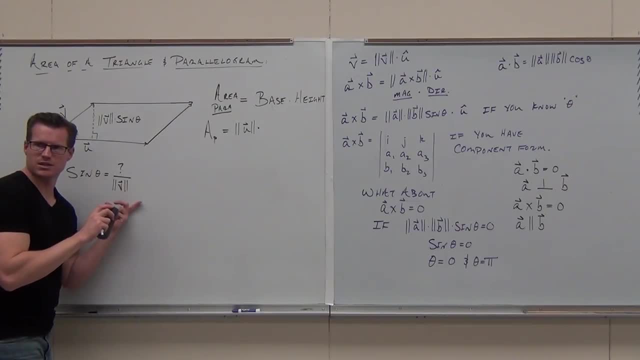 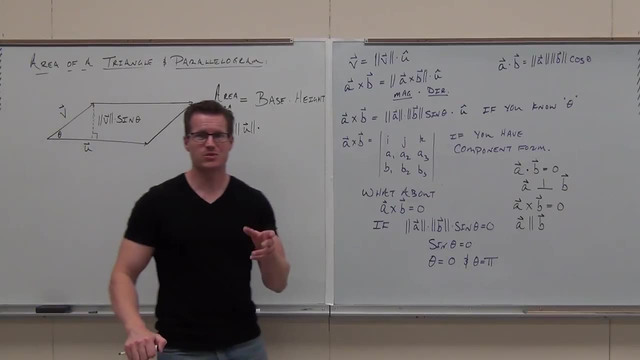 Do you guys have questions on this? before we continue, Do you guys see the relationship I'm talking about- Opposite over hypotenuse- Just solve for the opposite And we have that. Hey, do we have a base? Yeah, We've got this whole base. 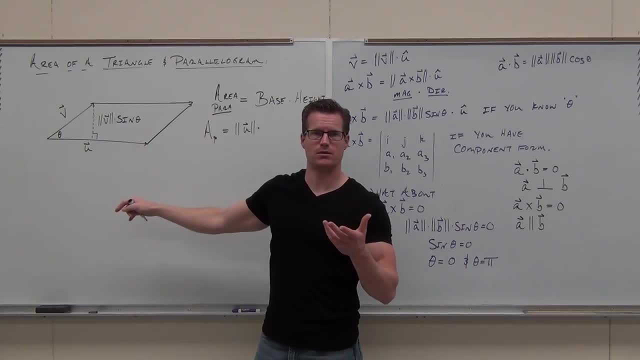 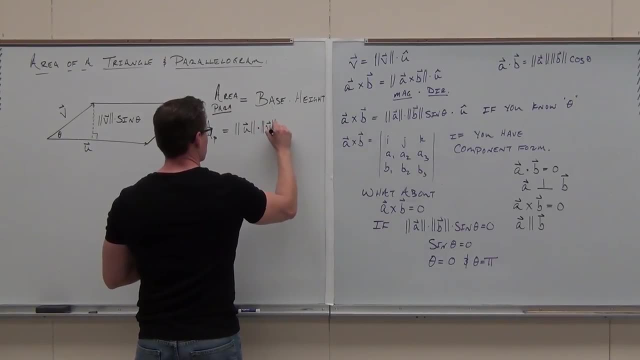 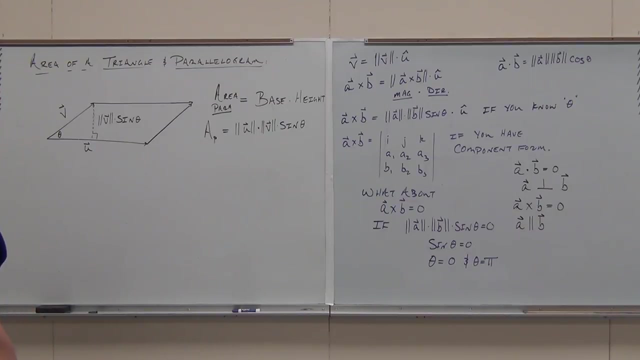 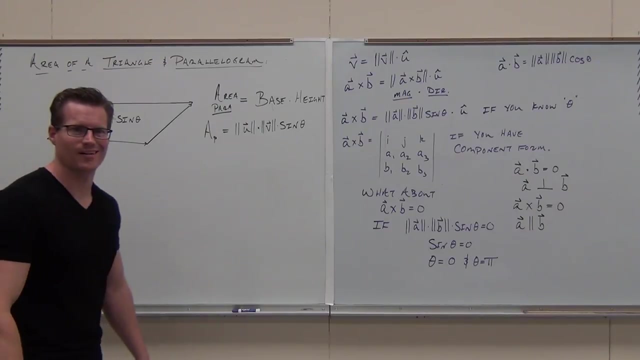 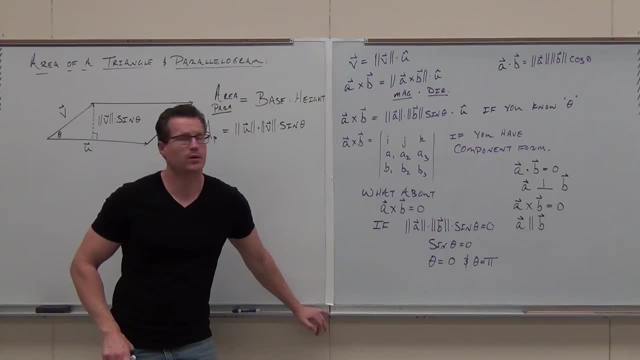 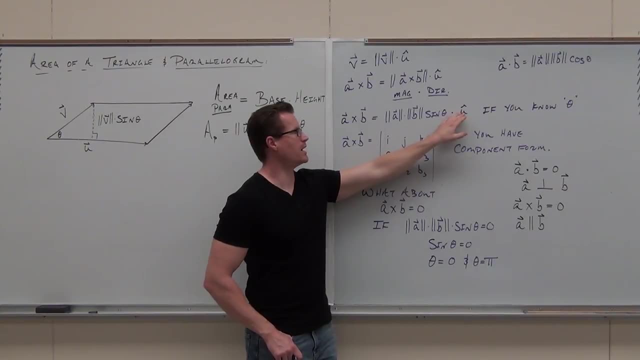 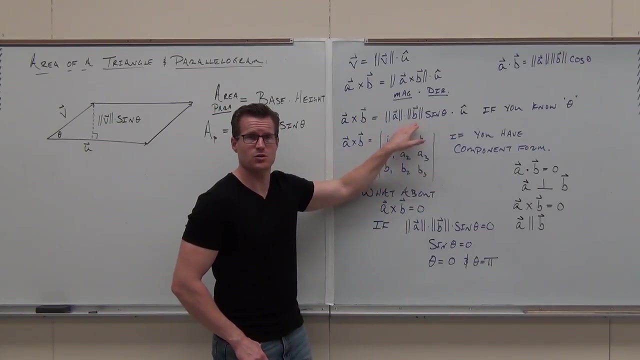 Cross cross, Not quite the cross product. is that it Not quite? because the cross product has this. I don't have this. I have just this. I got just this piece right there. What was this piece? Magnitude Vectors are magnitude times direction. 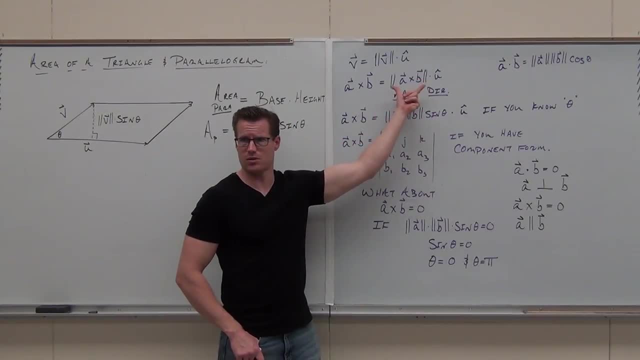 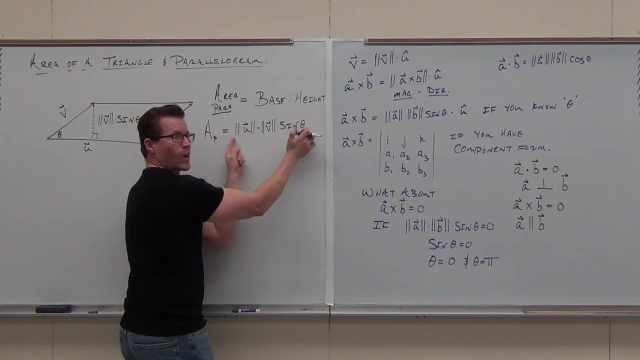 Magnitude times. This piece is the magnitude of the cross product. Are you following what I'm talking about? This is the base, This is the height, The way that we can get this. This is the magnitude of the cross product of the two vectors that this angle is between. 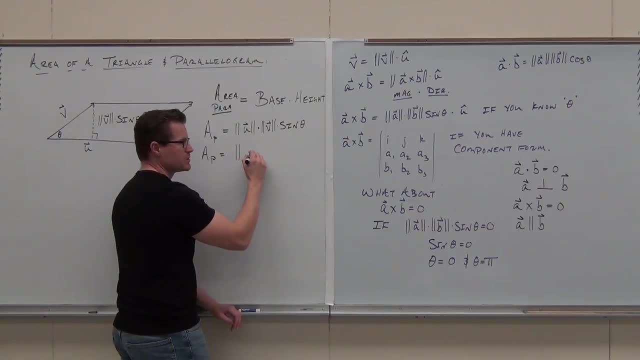 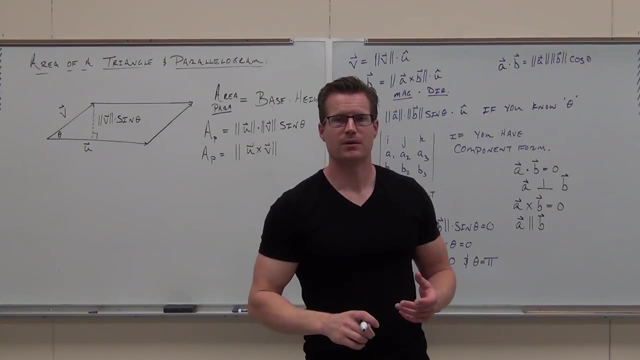 Since this angle is between U and V, this is the magnitude of the cross product of U and V. That's pretty interesting. So what's really cool is if I give you any two vectors and say, hey, there's only two vectors. 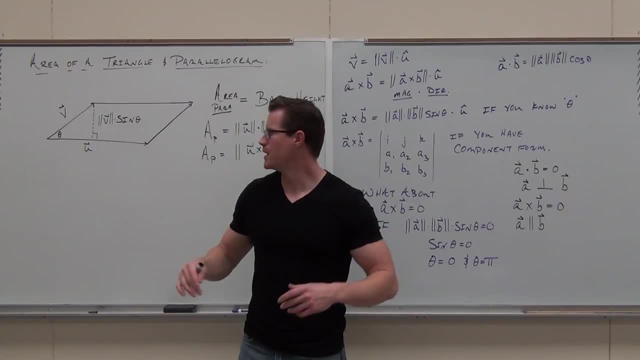 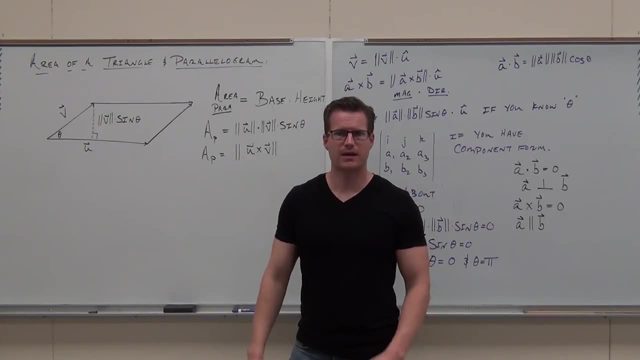 Those vectors. you know this by the parallelogram law makes up the parallelogram. So if I have the area of any parallelogram that's bordered by two vectors, it's easy Cross product magnitude done. That gives you the area that's contained by the parallelogram bordered by these two vectors. 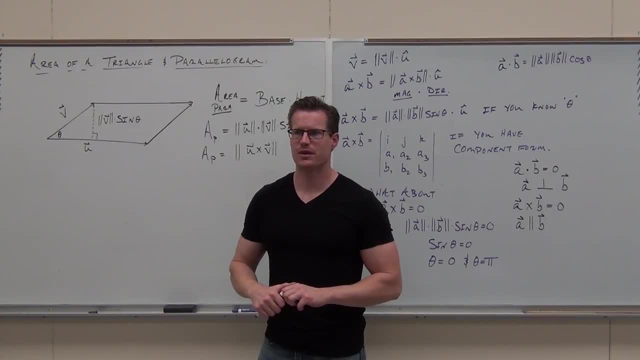 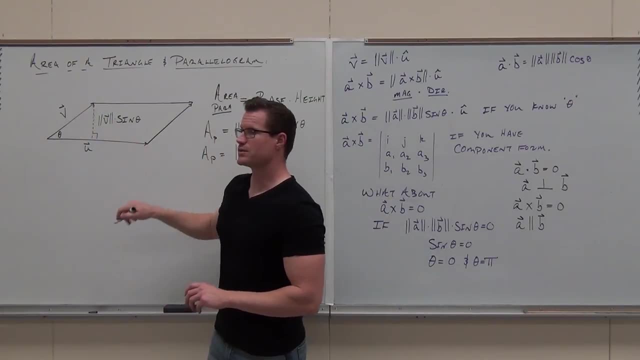 It's pretty neat, That's pretty cool. You guys, okay with the proof on that one. How about this? What's the area of the triangle that's bordered by these two vectors? Remember, the triangles cut parallelograms Like that. 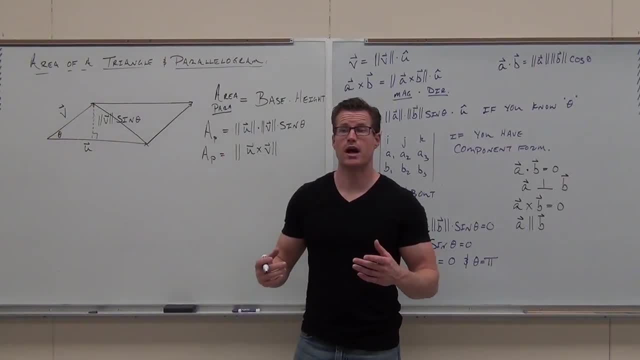 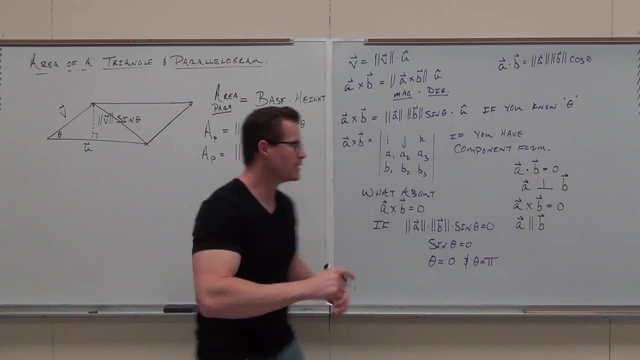 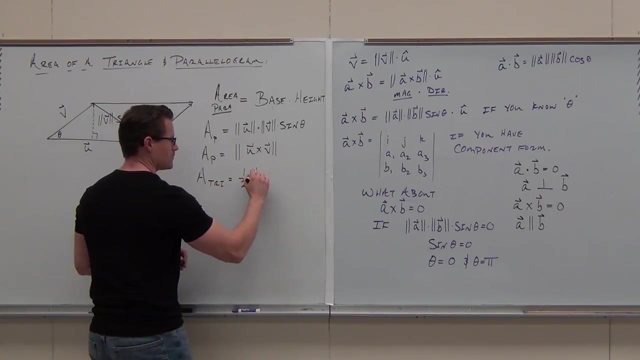 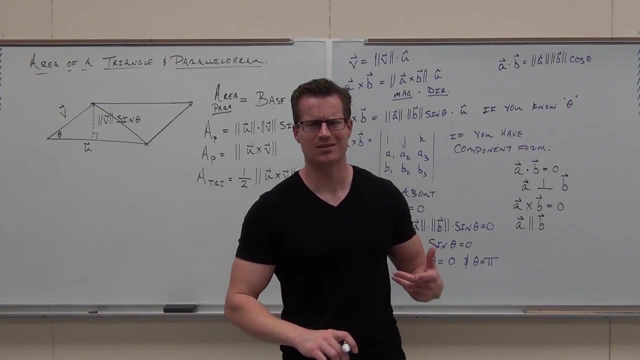 What would the area be for a triangle that's bordered by V and W? One half, Just half, Just like half base times height. It's half base times height. Did you expect that the cross product was going to have anything to do with this? 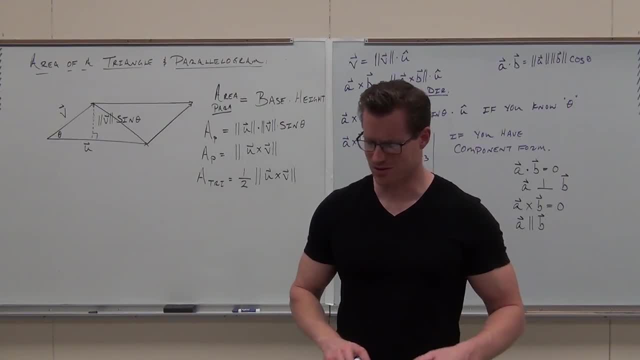 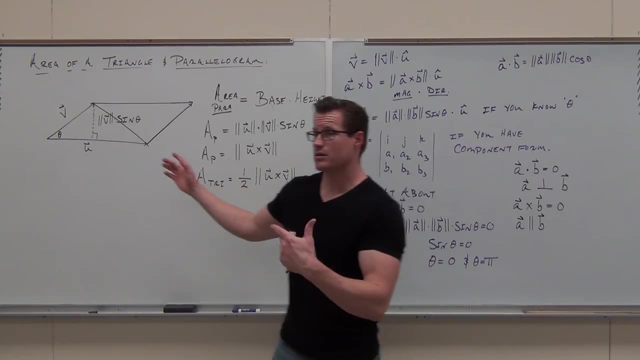 With the area of a parallelogram. It's kind of cool. It's really interesting If you really think about it. kind of funny. Think about it this way: The cross product would give you a vector that's pointed straight at you. 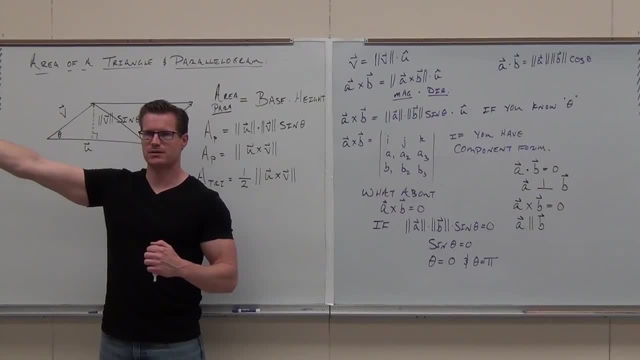 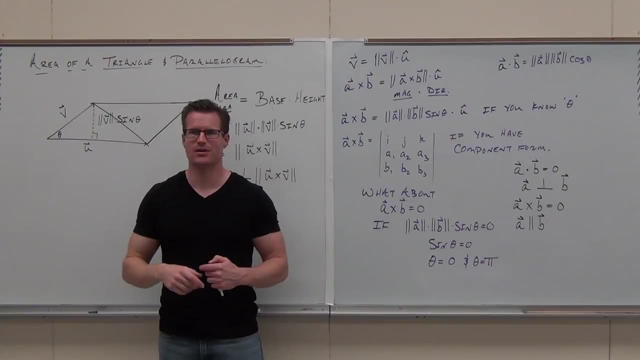 Does that make sense? The length of that vector is numerically equivalent to the area of that Half. the length of that vector is numerically equivalent to the area of that triangle. That's cool, That's really weird, And it all works out. 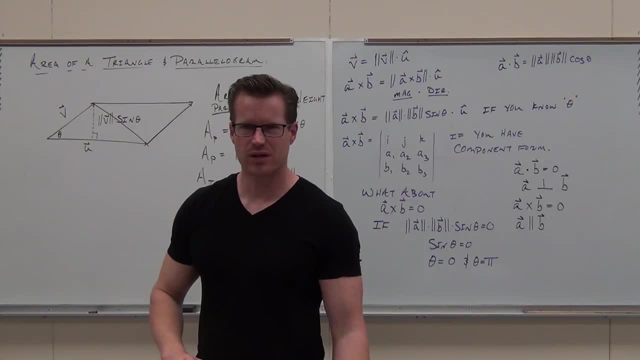 And I just proved it to you. You guys want to try an example just to illustrate this Before we go any further. I want to talk about some properties- You know one of them And we're going to get to this example- But some properties that you can use with a lot of this stuff. 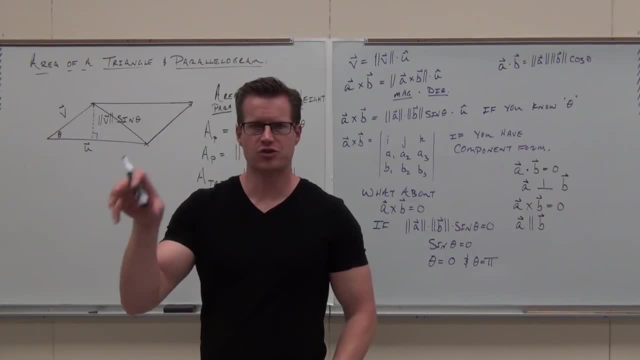 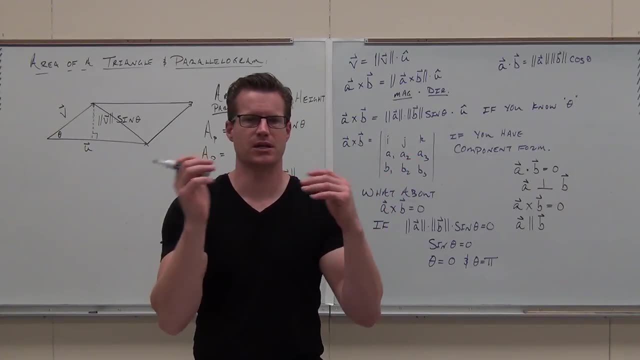 Number one: the cross product is distributive across addition. So if I want to find the cross product like A cross B plus C, You can do A cross B plus A plus C. A lot of the properties you expect are there. 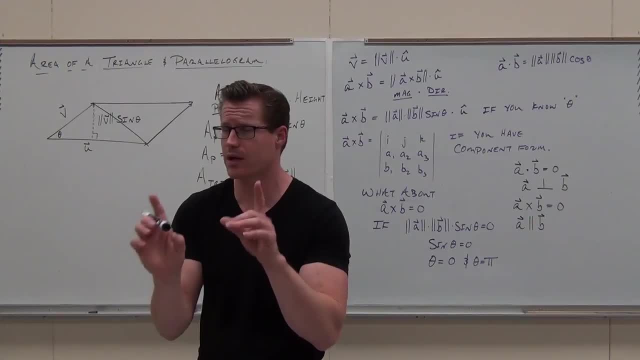 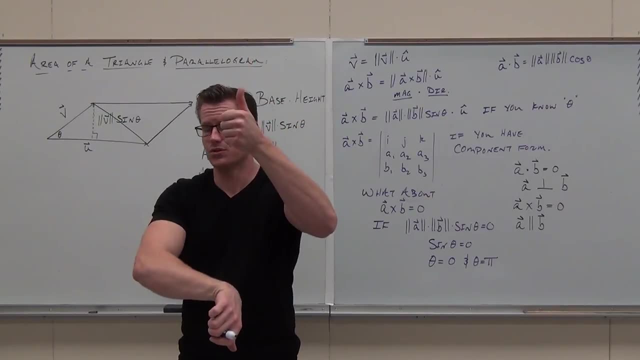 The only one is: commutativity doesn't quite work And you know it because we talked about it already. If I reverse the order, I get a negative sign Because the orthogonal vectors are going in opposite directions. Other than that, when I cross product with a zero, I still get a zero. 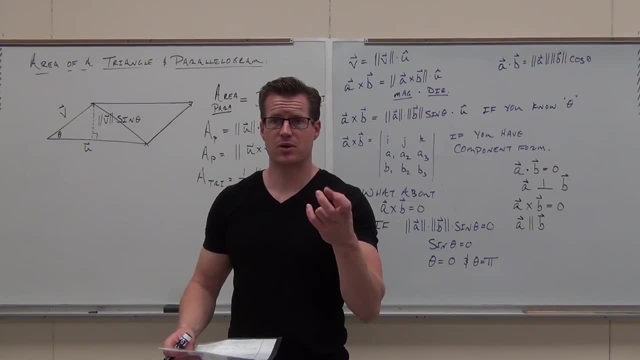 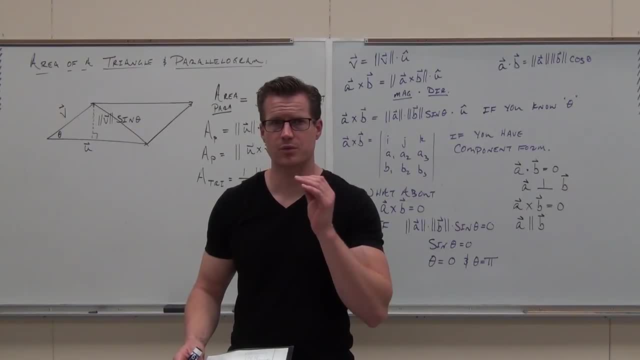 I don't know, I don't know. Cross, product a vector with itself, What would you get? You would get what? Zero? Zero. Why Parallel? Because a vector is parallel to itself. You have to get zero. That was only really the only surprising one that we have. 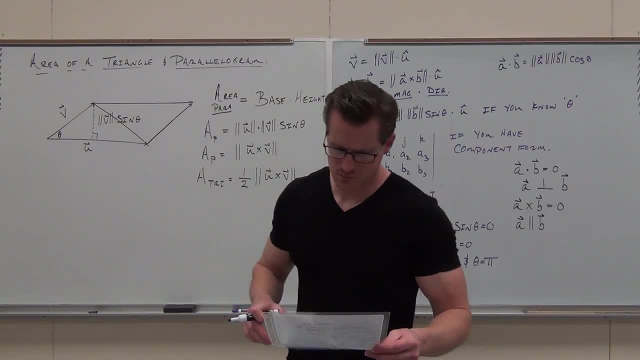 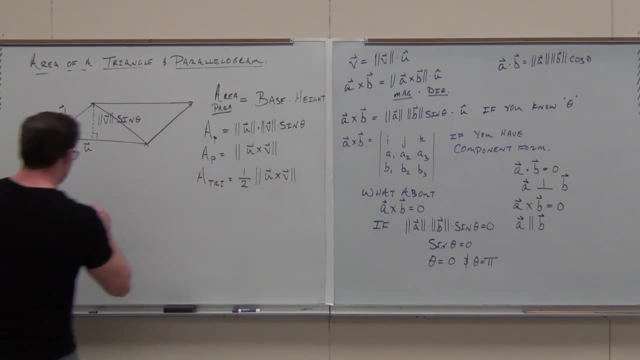 There is, yeah, there, yeah, that's pretty much it. I want to talk about this example, the area of a triangle, but that's not too bad as long as you know how to do the cross function. Let's put this together from one through an example should be pretty straightforward. 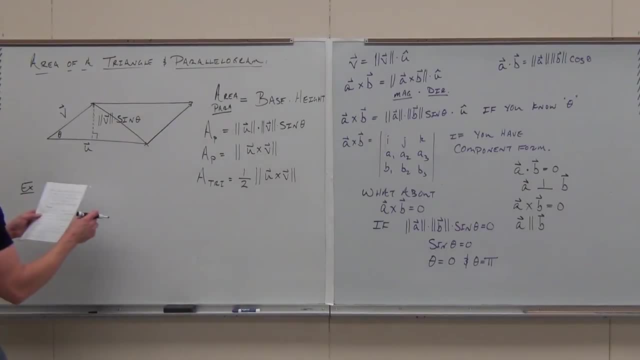 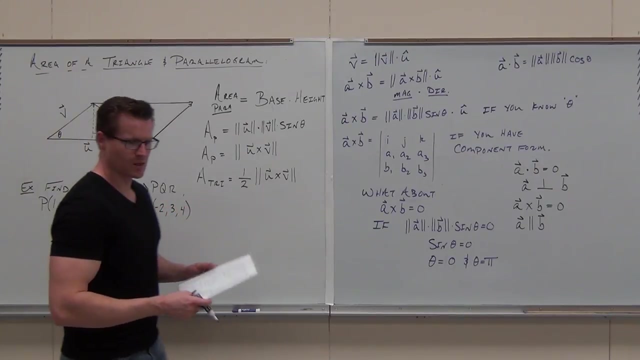 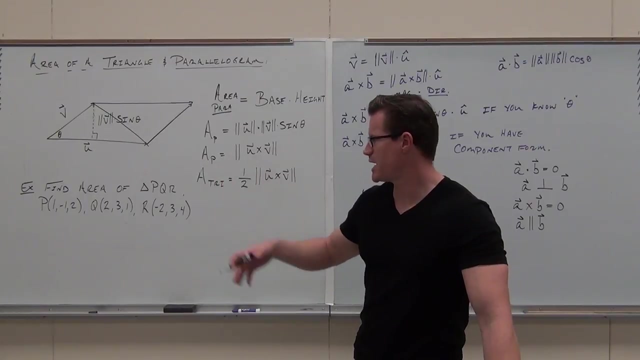 and then we'll talk about volume of a prism. Thank you, We've got this triangle and I've given you the points of the triangle. I want you to find the area of that triangle where P is that, Q is that and R is that. 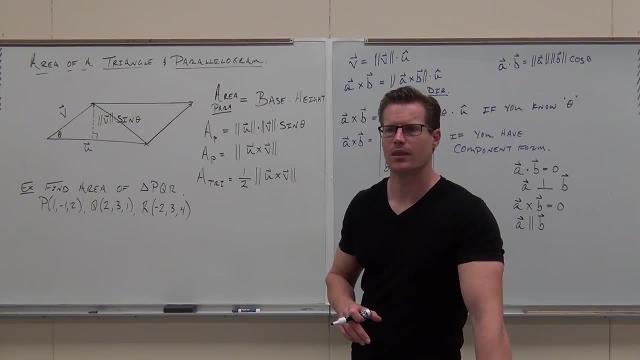 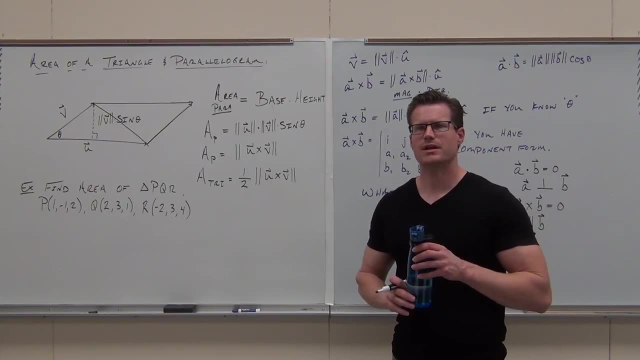 Write it down, Look up here so I know you've got it. Give me an answer here. Does the cross product work with points? No, Do you see any points up there? What do you see up there? I see vectors. Can you find vectors from points? 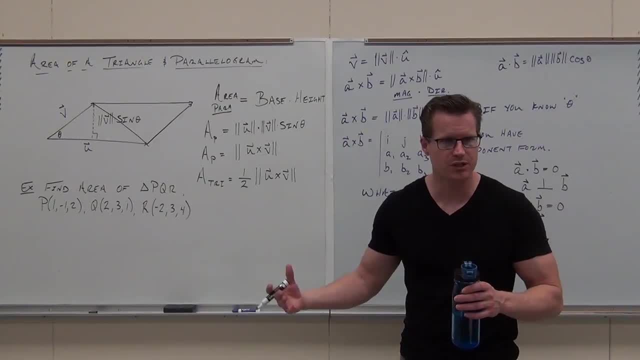 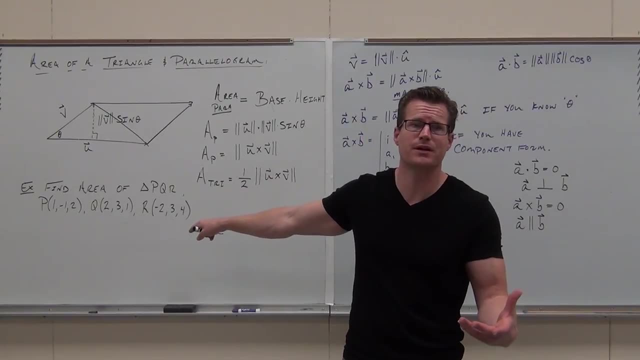 Yes, Yeah. So anytime I give you points, it's not a huge deal, but you do need to know how to find a position vector, which is why I'm going to give you a problem like this on a test, because it tests a lot of stuff in it. 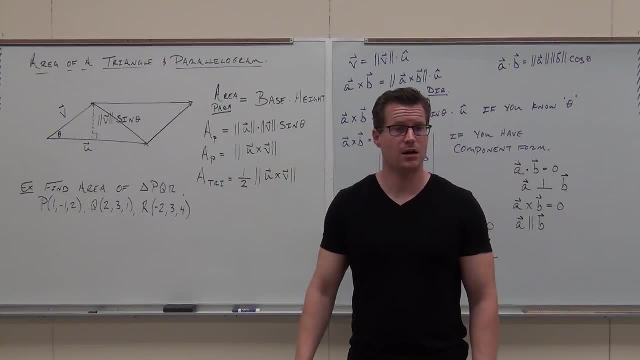 It says: hey, can you find a vector between P and Q? Yeah, Can you find a vector between P and R? Yeah, That's awesome. Can you find the area of that triangle? That's a cross product. Can you do a cross product? 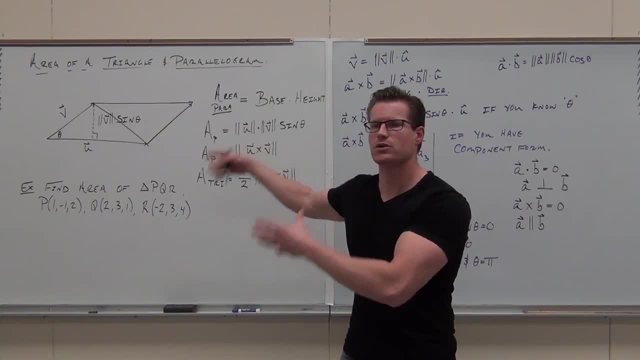 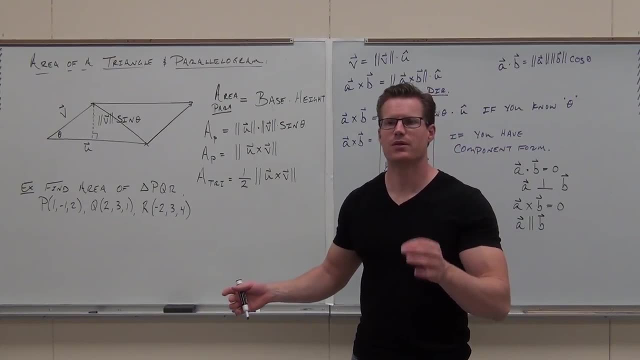 Yeah, Can you do a magnitude? Yeah, That includes all this stuff. Does that make sense to you? So when we have this triangle, you don't have to draw it, I don't care that you draw it, but you do have to do one thing. 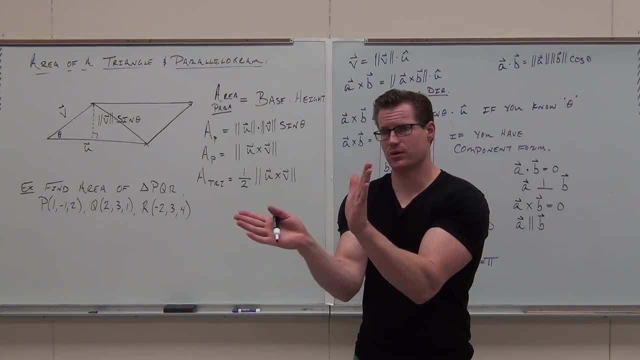 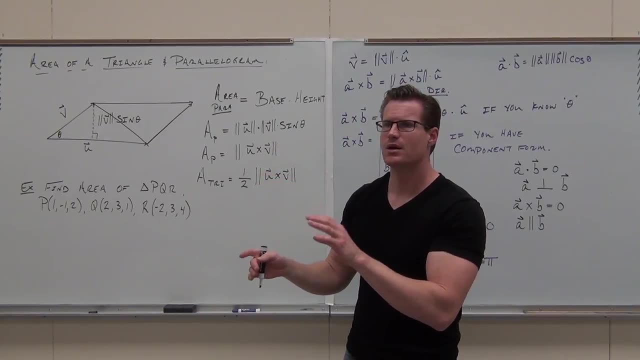 You've got to start with what the vectors are: that border, that triangle, Basically, that border, the parallelogram. then we're going to cut it in half. Okay, that's what's going on. My only advice to you is, whenever you do this, please start with the same letter. 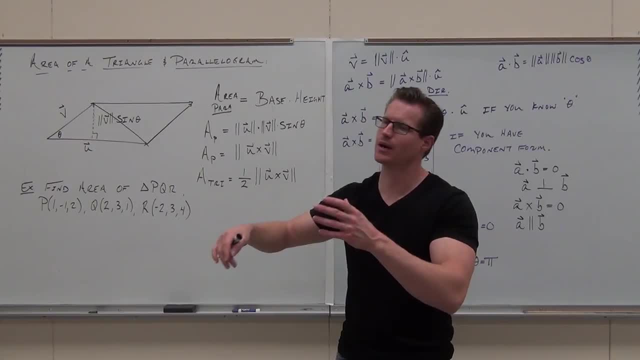 Don't do PQ and then QR Unless, Because, Because when you do that cross product it's going to be a little bit weird, okay? So when you start with one letter, keep starting with that same letter until you exhaust all the vectors. 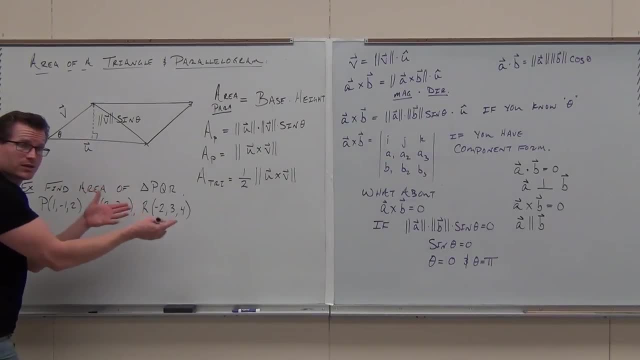 For instance, to find this, And it doesn't matter what letter you start with, Just start with the same letter. So I would start with PQ And then the next vector I'm finding is what? PR? Not QR PR. I hope you understand why. 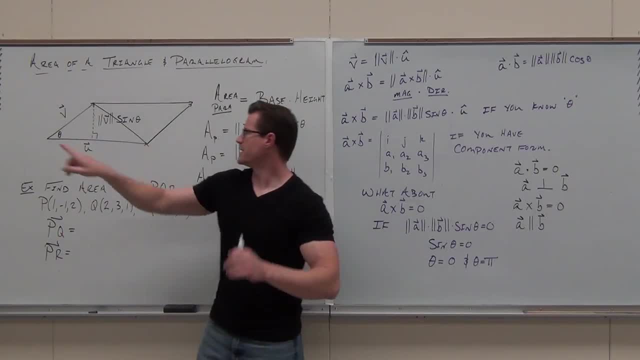 Okay, The idea is These things: in order to find a cross product, they need to have the same initial point. So if I'm starting at P, I want to keep starting at P. That way, when I do the cross product, they actually match up. 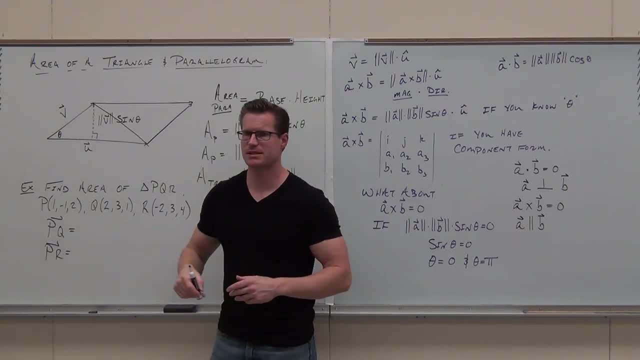 Does that make sense? I don't want to start here and then start here. That doesn't make sense. It wouldn't give me the same Well here and here. It wouldn't give me the same exact relationship there. So start with the same letter. 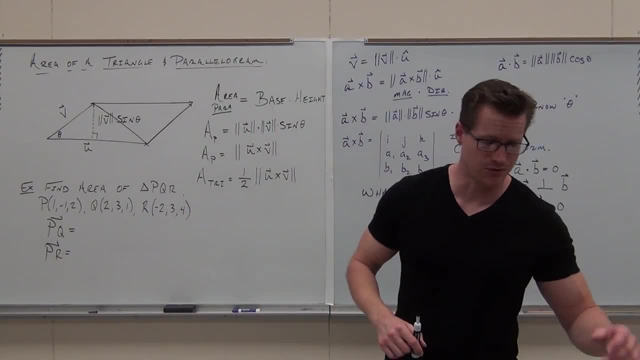 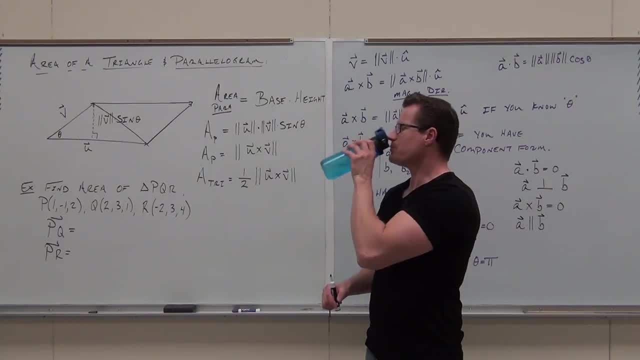 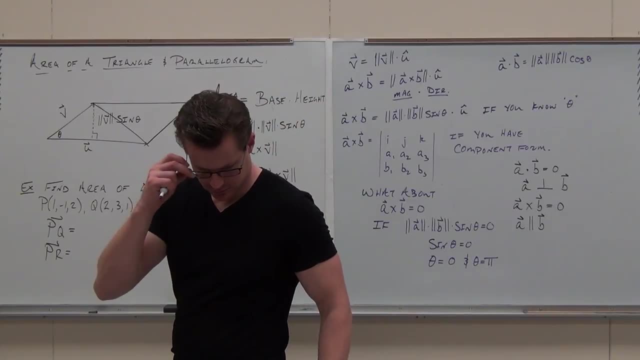 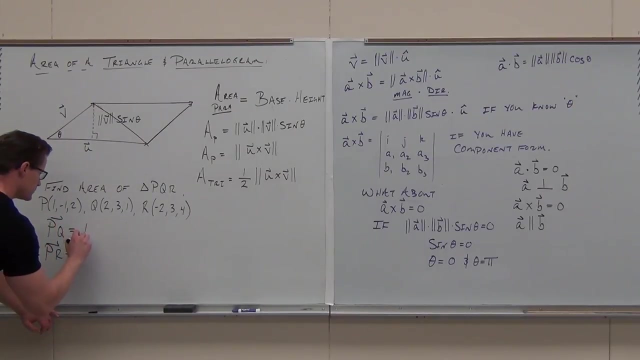 Okay, Okay, Okay, Okay. Whatever form you want to use is absolutely fine. Take some time when you do these double check. It'd be the worst thing in the world to know how to do a cross product right To know what position vectors are. 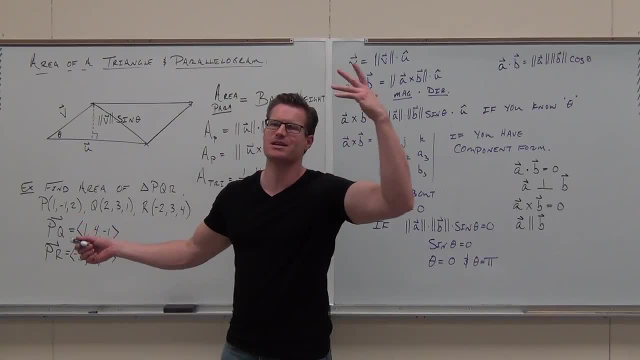 To get everything done Like: oh man, I put 1. It was negative 1. And you get the whole thing wrong. Don't do that to yourself. So take some time. Did you get the same thing that I got? 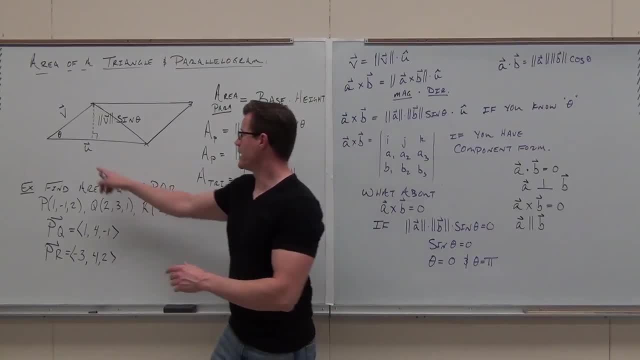 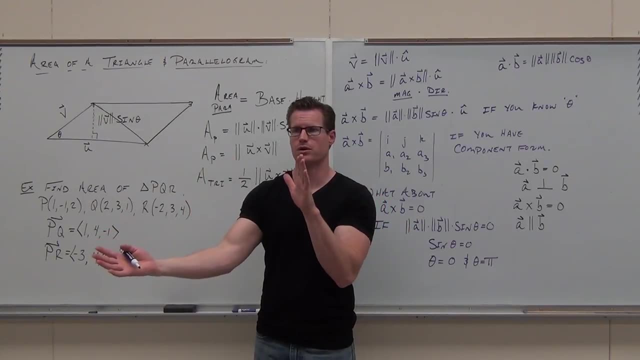 Yes, Yeah, Okay. So what we've done is we've found out this vector and this vector, and we're looking for the area of the cross product. This is the triangle that those two vectors border. What's the next thing that you're doing once you have those? 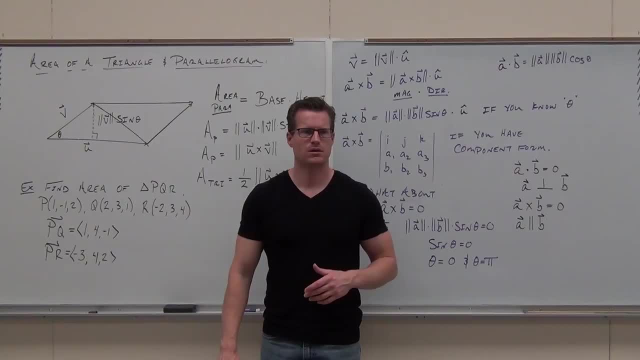 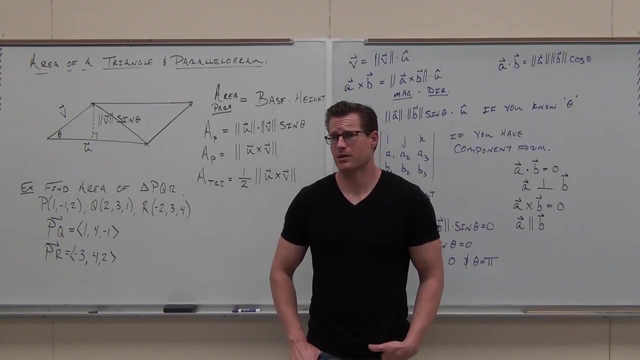 two vectors with the same initial point. What would you do? What gives you the area of a? Do you understand the question? Yeah, Find the area of a triangle. Triangles come from parallelograms, So let's find the area of a parallelogram. 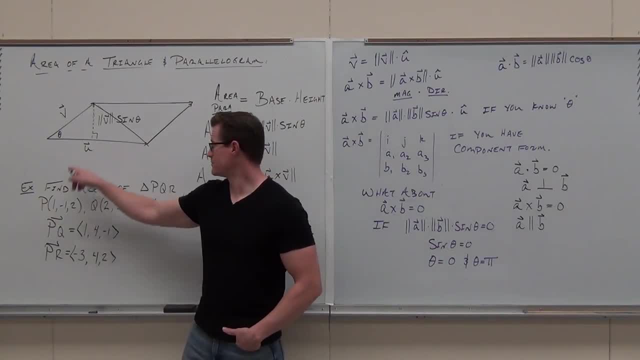 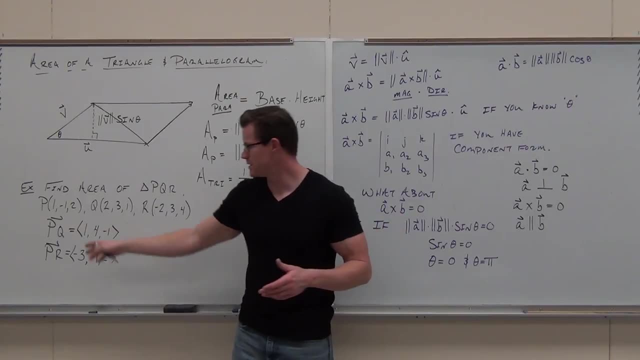 and then cut it in half. Do you guys get that? this is like, this is just like this vector And this one's just like that vector? So how do I find the area of the parallelogram that these vectors border? Come on, we just did it. 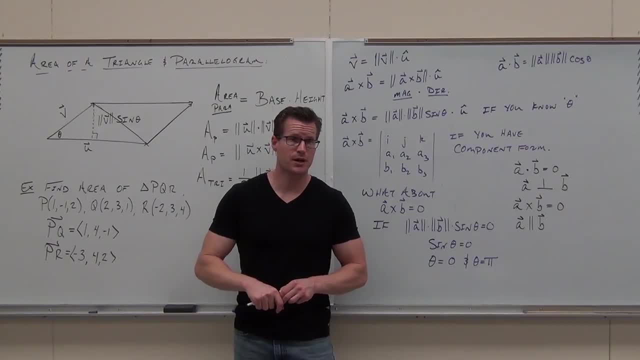 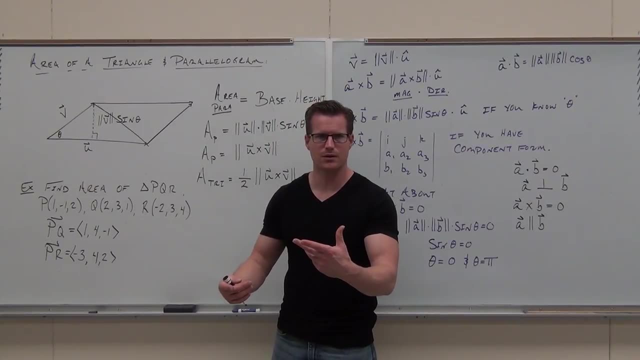 Why don't you give it a try? So let's find the cross product first and then we'll find the magnitude. You can't do it all at once. You've got to find the cross product first and then find the magnitude. Can you guys see what I'm talking about here? 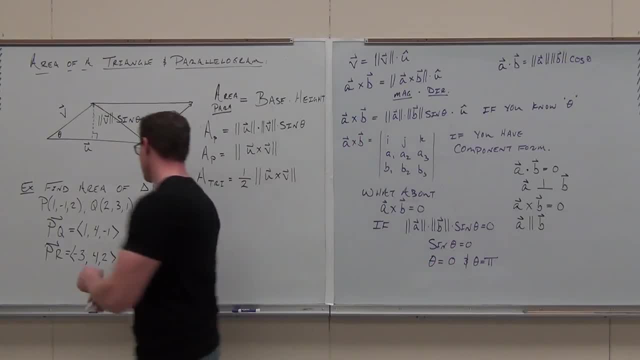 If it helps you and you're like man, I don't know about PQ. If that doesn't work, well, then call this one vector B and call this one vector U. I don't care what you call them, But it at some point it's going to be. it's going to be. 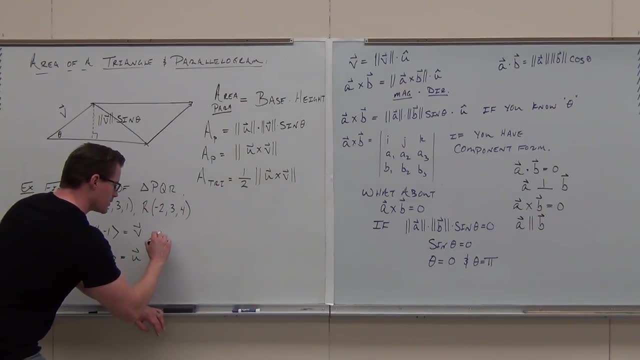 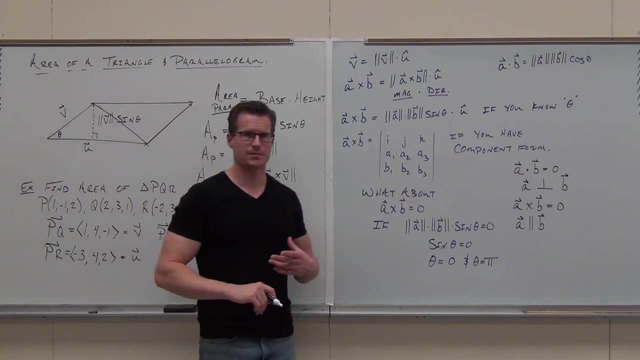 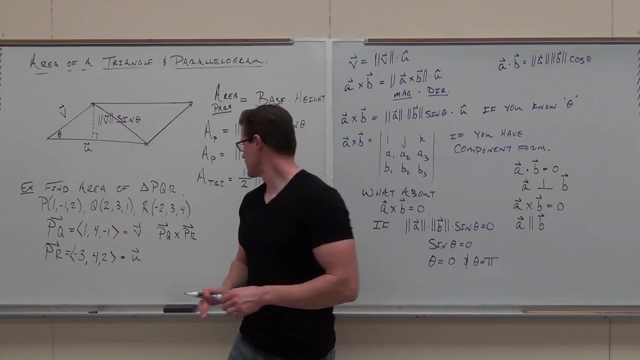 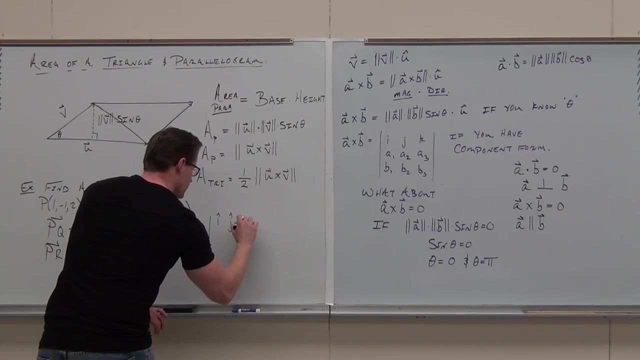 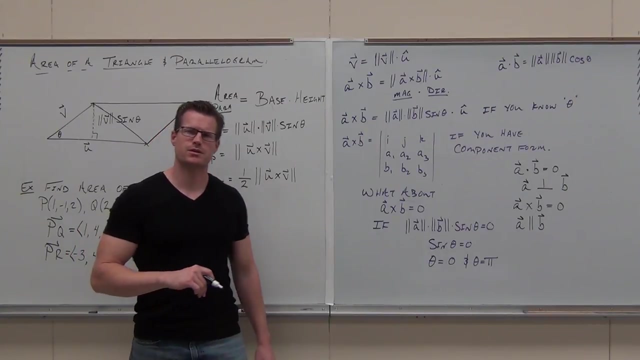 at some point you're going to have to do the cross product in order to find the area of the parallelogram. Well, at least find it easy. Question question to you: Does the order matter? Does the order matter when you're doing this? 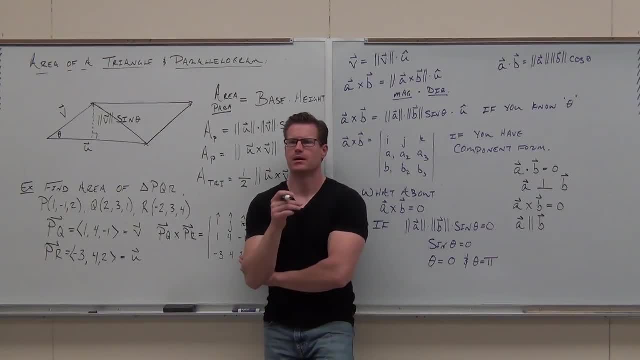 I'm going to ask you it again and I want you to think about it At the very end. when you do the cross product, you're going to be finding magnitude. Do negatives matter in magnitudes? So, no matter how I do this cross product, you can't. 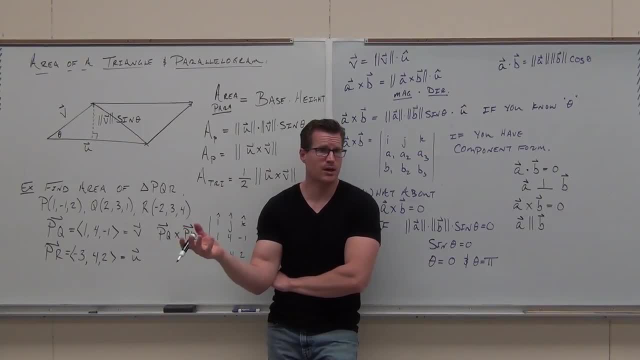 you can't mess it up, because if I get negatives, I'm squaring them anyway. If I get positives, I'm squaring them anyway. So I'm finding the magnitude of this thing. It doesn't matter the order, I'm just going to get a different vector, sure? 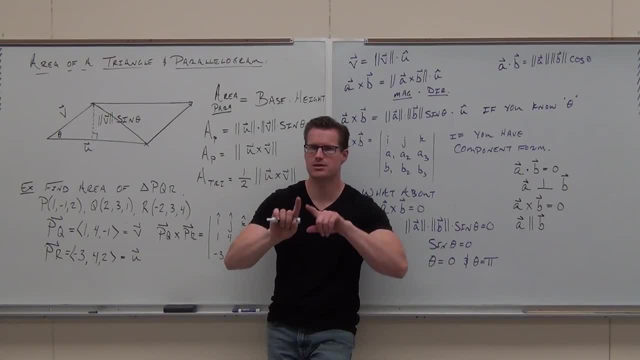 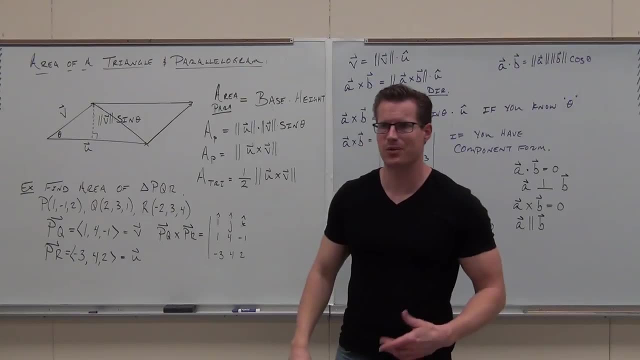 but magnitude of that vector is going to be the same. There's a whole point here: is that these two different vectors have the same length, just different directions, So magnitude has to be the same. Hopefully, as I've been rambling, you've been working. 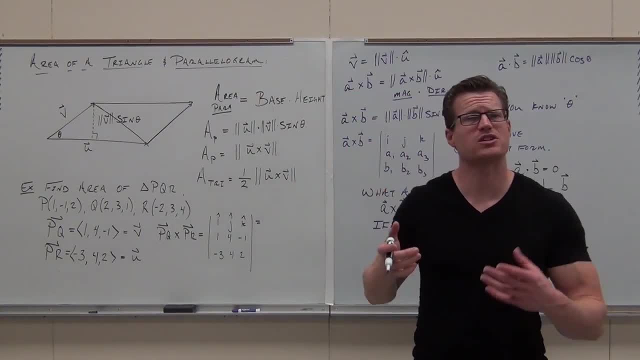 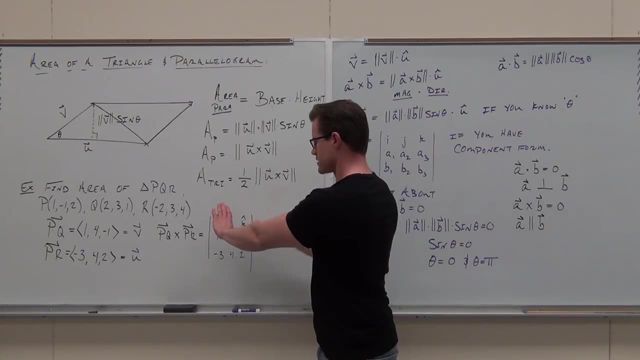 We're at the point where I'm not going to be doing a whole lot of work on the board. I'm expecting that you can actually do it. What's our, if you've done it already? what's our I component After you've done this and this? so 8 minus negative 4,. 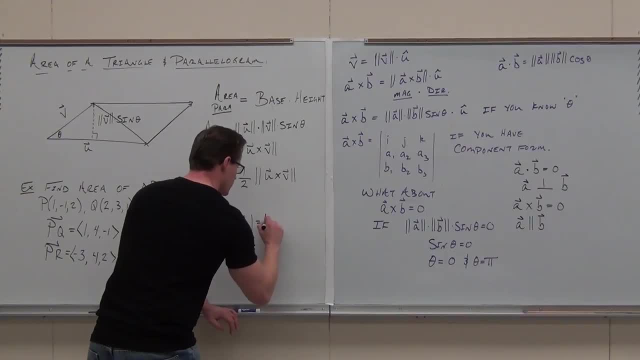 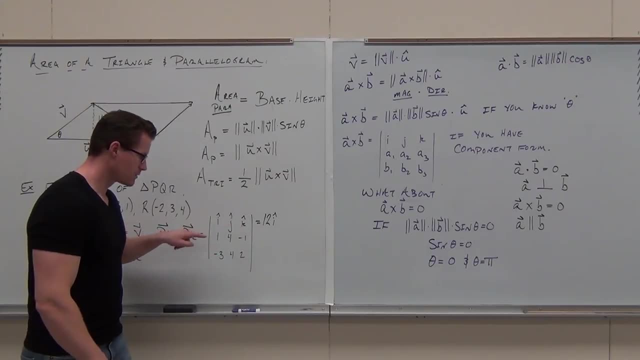 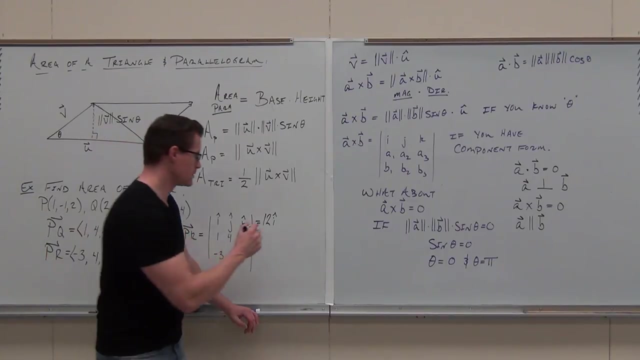 you've got 12. I's very good. Then we've got 2 minus 3, it should be negative 1, but you have a minus there, so you have plus J. Did you get plus J? Yeah, Okay, we've got 4 minus negative 12.. 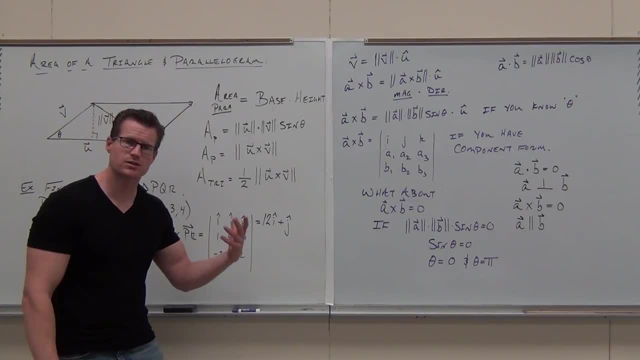 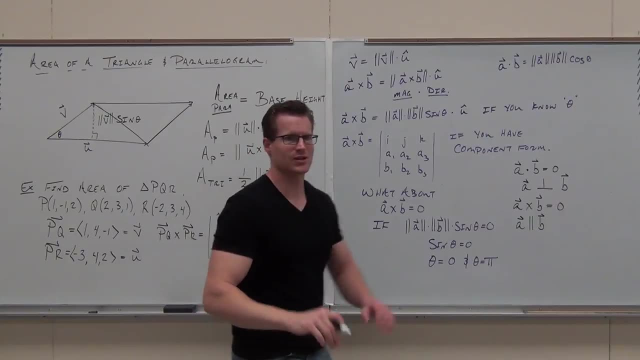 It's 4 plus 12. That's 16.. Did you get 16?? Yes, Awesome, that's fantastic. Show your fans if you're okay with finding that Perfect. Okay, stop right now. What is that? What is this thing? 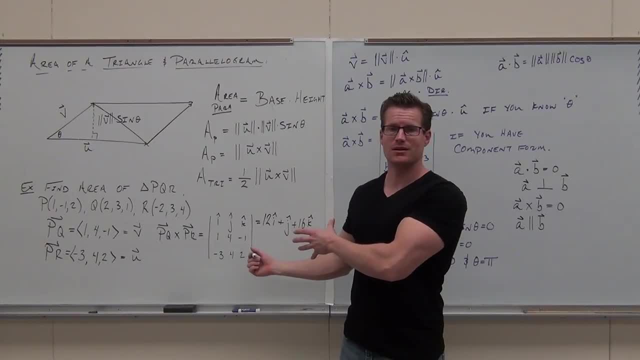 And don't just say it's a vector. What is this vector? Cross-product? I know it's a cross-product. If you just said that cross-product, what's it represent? Base: You want to see a teacher cry. This is what makes a teacher drink at night. 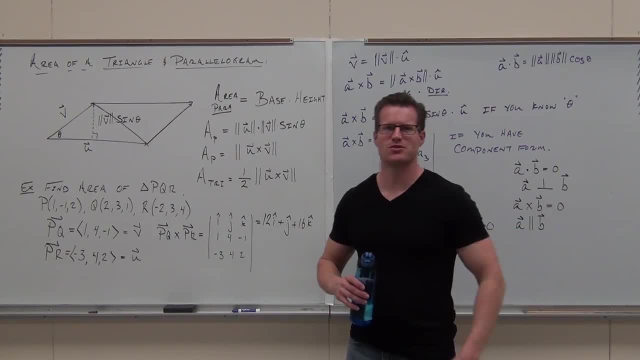 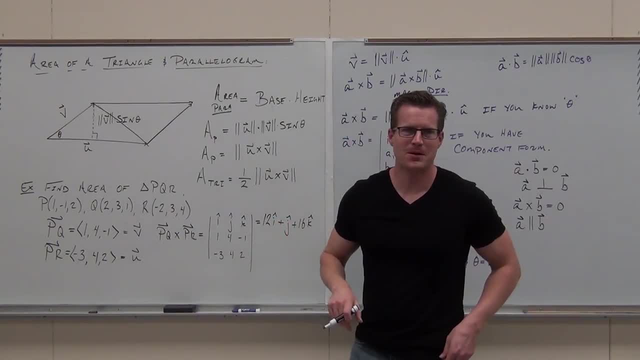 Maybe a glass of wine, like once a month on an anniversary or something you know It's fun. What Look? is this an area? Is that an area That is No? Can a vector possibly be a freaking area? Does it make sense? 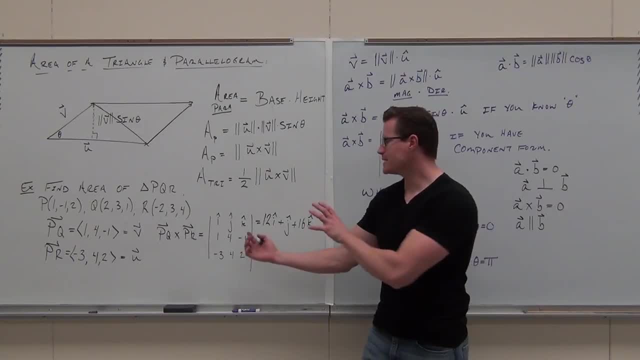 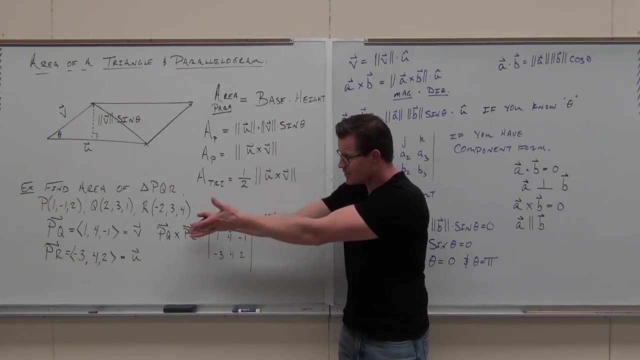 It makes sense. The magnitude of that vector, yes, But what does this vector represent? We just spent like an hour and a half talking about cross-product. What's that vector? What is that vector in relation to these two vectors? What is it? 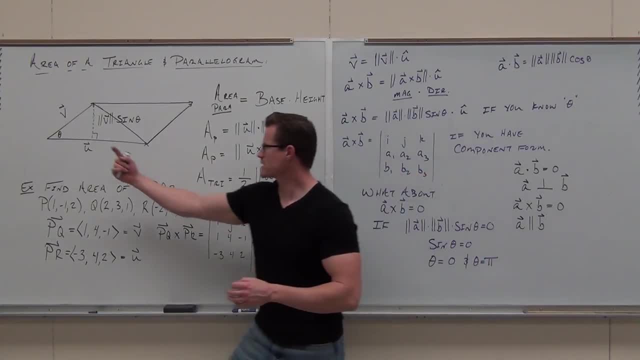 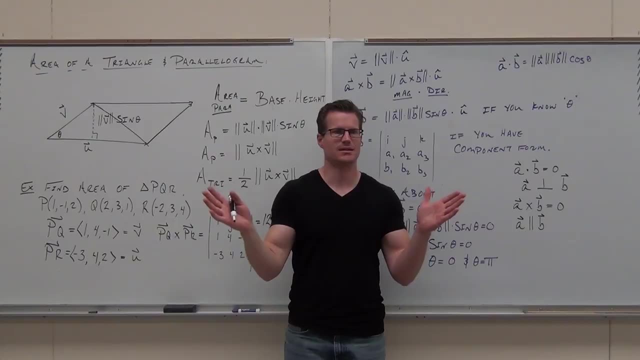 Orthogonal, It's orthogonal. So this is the vector that points out from the board like that, And it's at that point because that's where we did it. Does that make sense to you? That's what that vector is. Now, because of this really neat math I just proved to you. 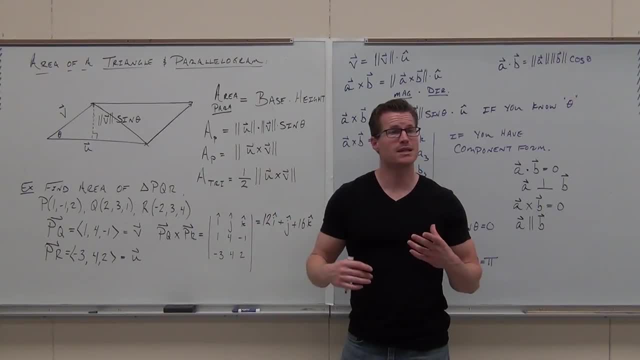 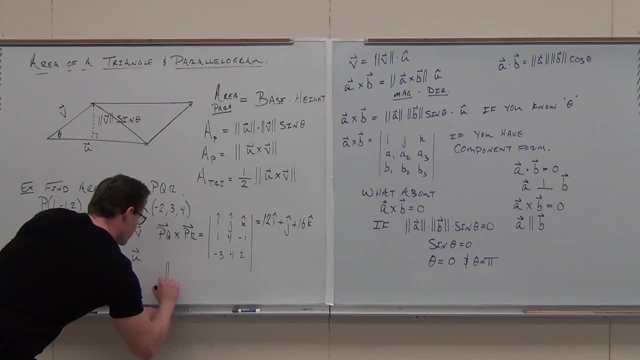 when I find the magnitude of said vector, it also represents the area of the parallelogram. So let's find that. Let's find the magnitude of this. Oh dang, I can't do that. Is it 256?? I don't know. 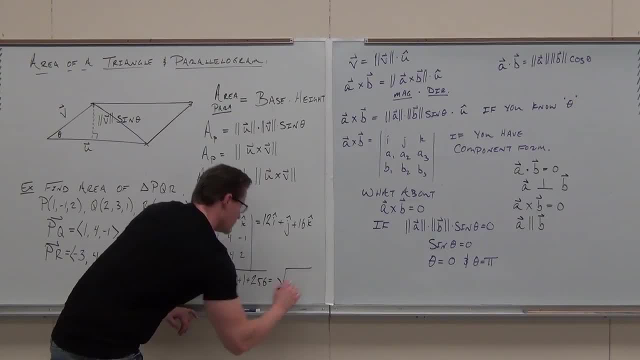 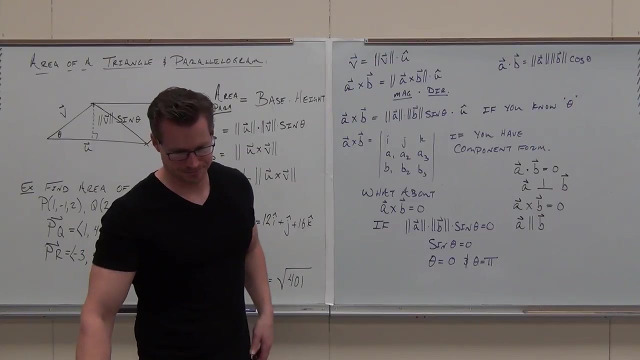 I guess I did know. Let's try it out now. How much? 401.. 401.. 401.. True or false, We're done. False, False, False. OK, What is this? What is it? Area? 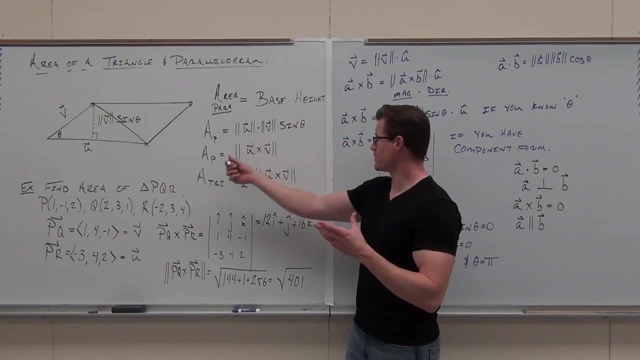 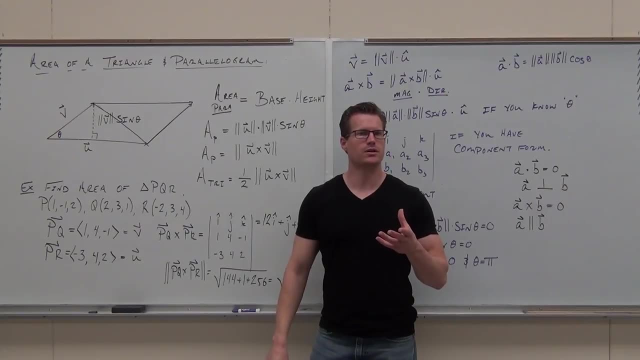 It's the area of Parallelogram. Parallelogram- Very good, Because that's the parallelogram thing we just had right there. How do I answer the question? the correct way: Area of a Triangle. So the triangle is going to have an area of. 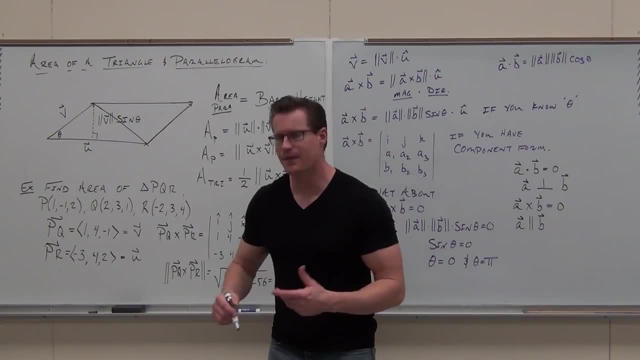 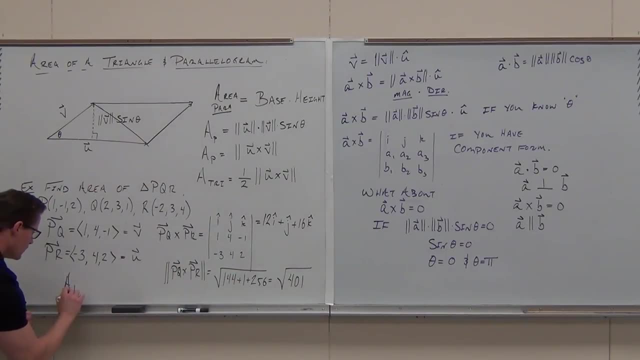 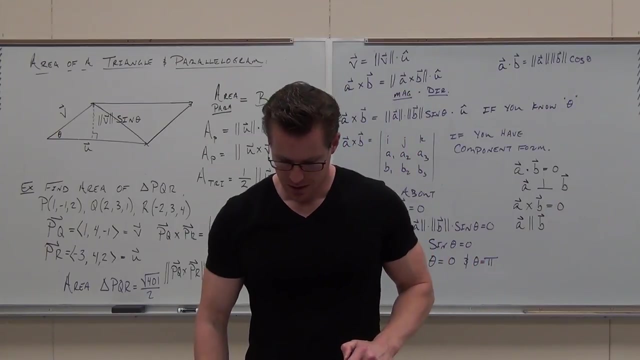 Just put one half in front of that thing and call it good Over 2.. And that's the area of the triangle Square root 401 over 2.. And you can approximate it And that's what I want you to know. 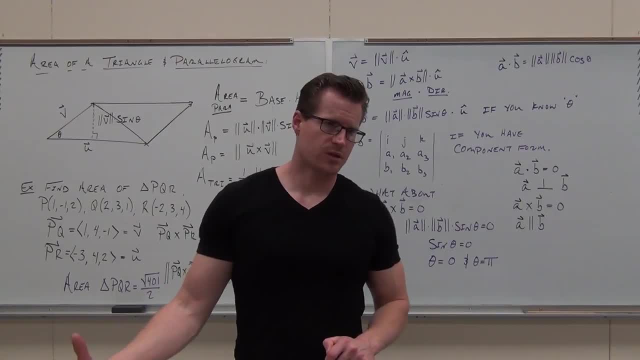 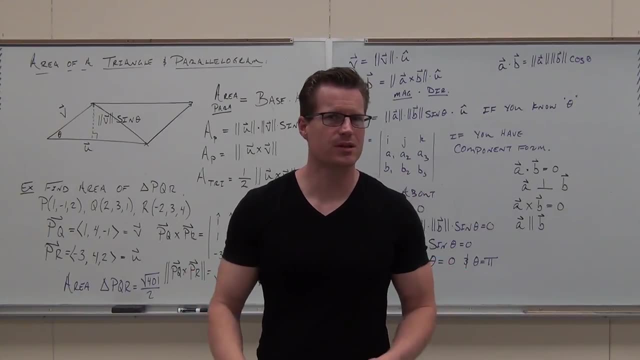 Head nod if you feel OK with what I want you to know. So we've talked about the properties, We've done one example. I want to extend the concept just one time. We're going to talk about volume And then we're going to be just about done with this section. 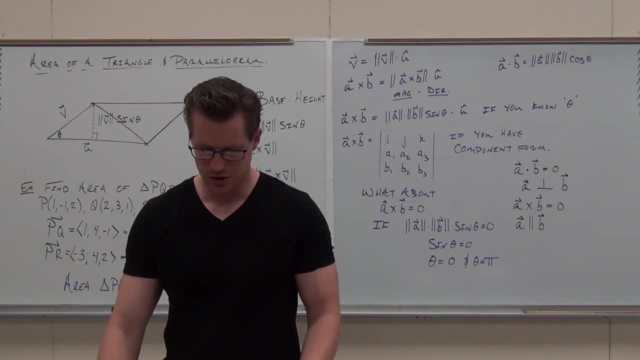 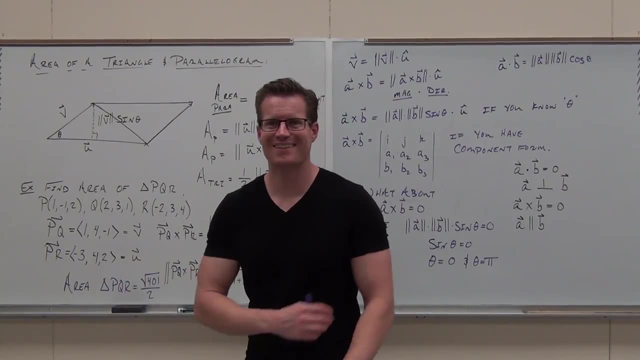 We'll talk about torque, and that one proof. Any comments, questions at all, before we can go in? No, Nothing Making perfect sense. Do you know how to find a cross product? Yes. Do you know what it means? Yes. 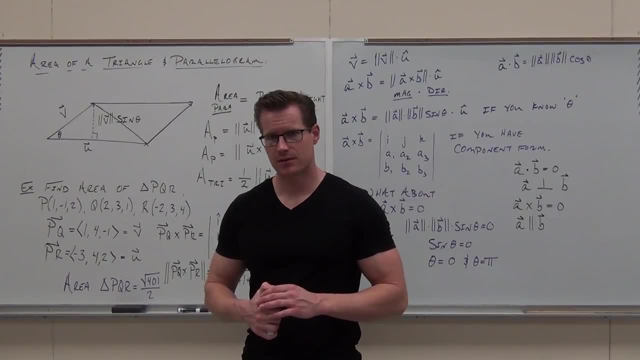 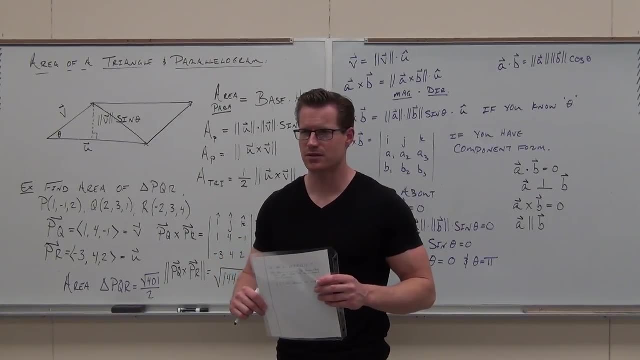 Do you know how to find a dot product? Yes. Do you know how to use it like 14 different ways? No. Do you know how to find the area of a parallelogram? Yes. Do you know how to find the angle between two vectors? 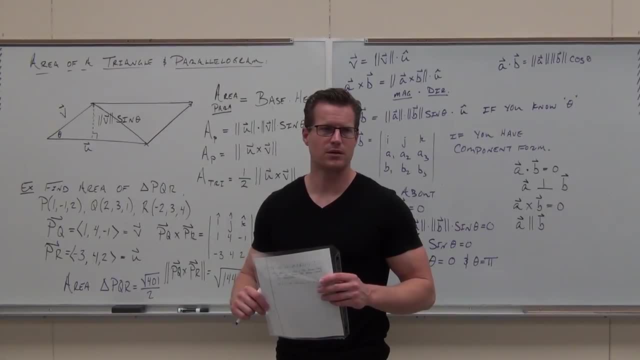 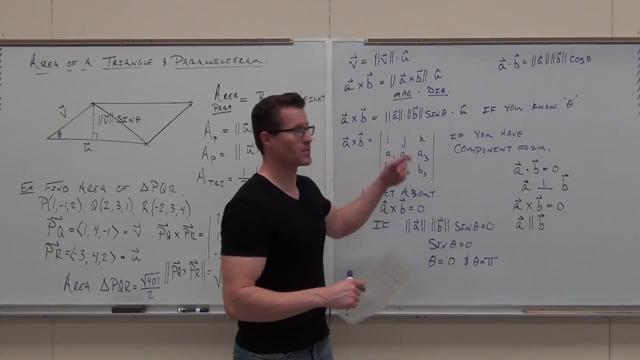 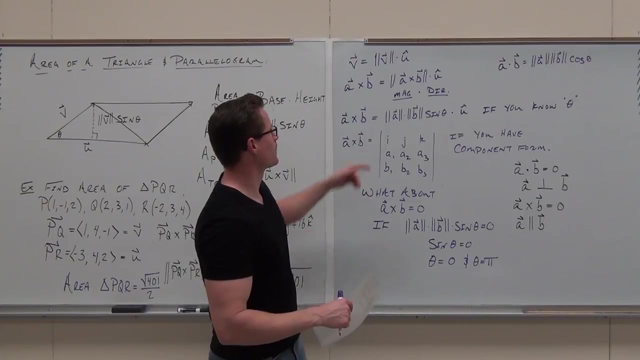 Yes, Yes, What's that involve cross product or dot product, Cross product, Perfect Area between two vectors. Actually, you really solve for it either When you think about it. cross divided by that would give you well magnitude. divided by the magnitude would give you sine. 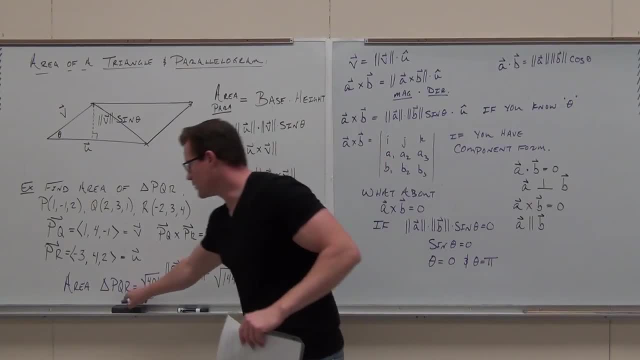 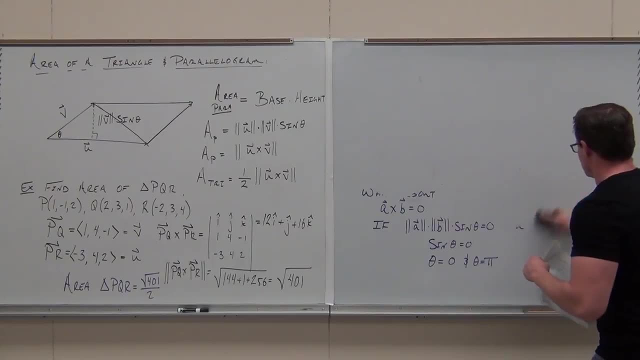 So pretty much either, But use the dot product, It's easier. OK, So I told you I was going to give you volume. Let's talk about volume. So let's go over to the souls. OK, So I'm going to give you volume. 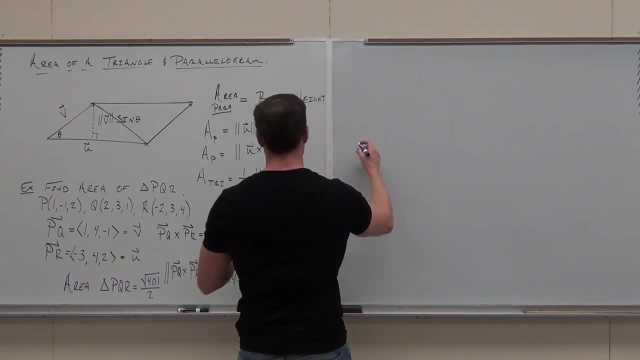 OK, OK, This is the size of the song, Right, OK, This is the size of the song, OK, OK, OK, OK, Yes, yes, Yes, This is the same volume, but a little bit different, OK, 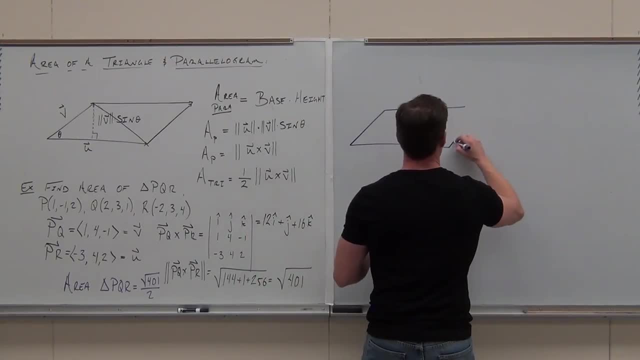 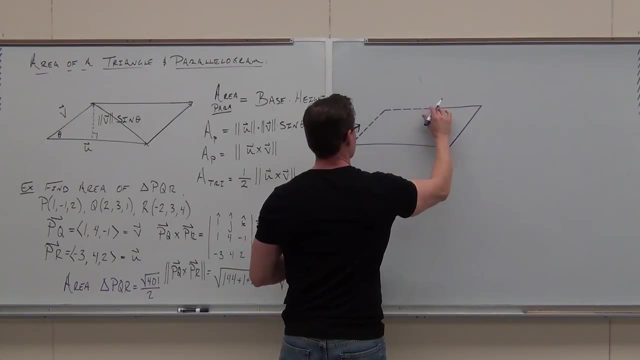 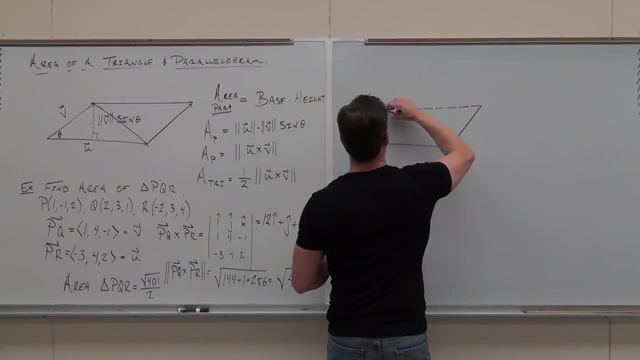 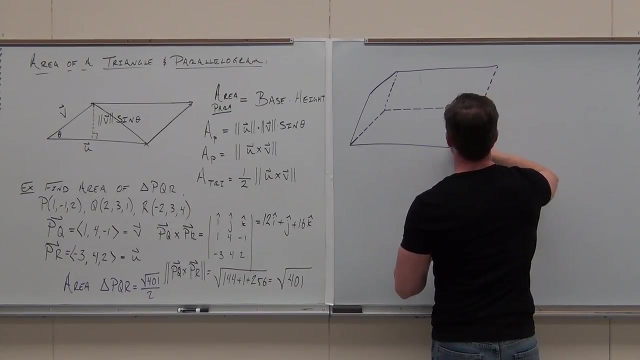 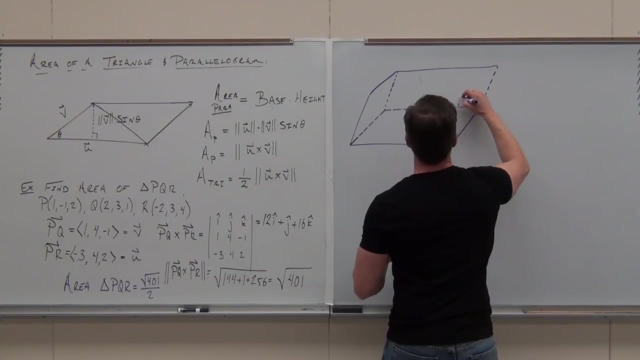 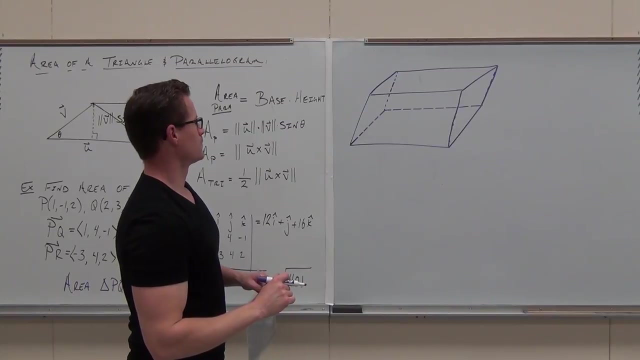 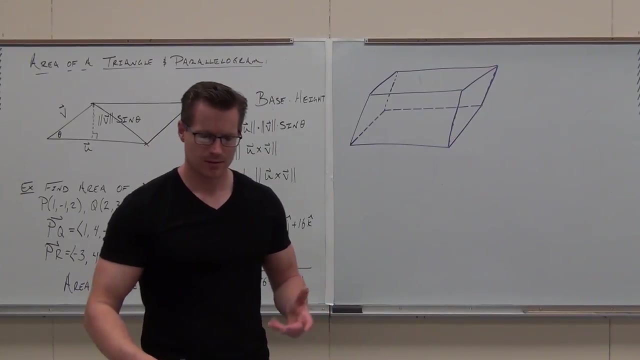 OK, OK, OK, OK, OK, OK, Thank you. Is that good enough for you? Did you get the picture? I'm not very good at it, so that's the best way I got This right. here is a really weird word. 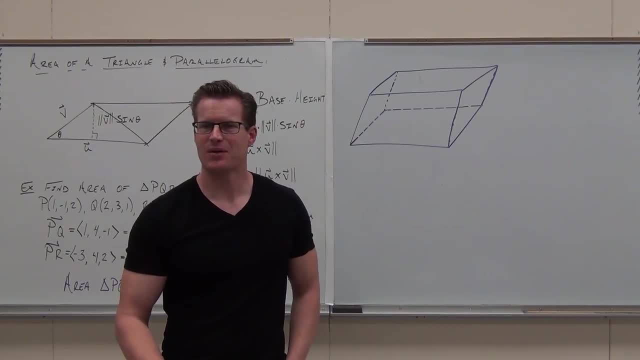 It's called a parallelepiped. Can you say that three times fast? Parallelepiped. Say that Parallelepiped. I said python. Somebody could have said pythons. That would be awesome, but it's not. 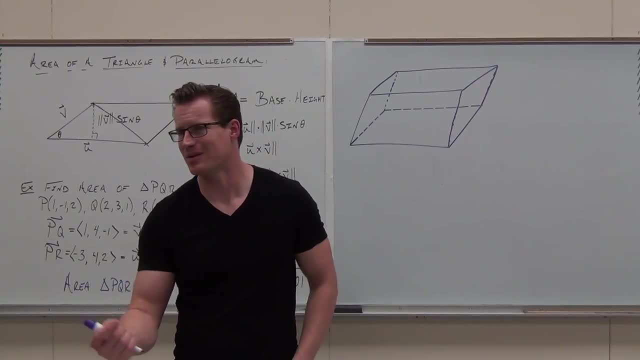 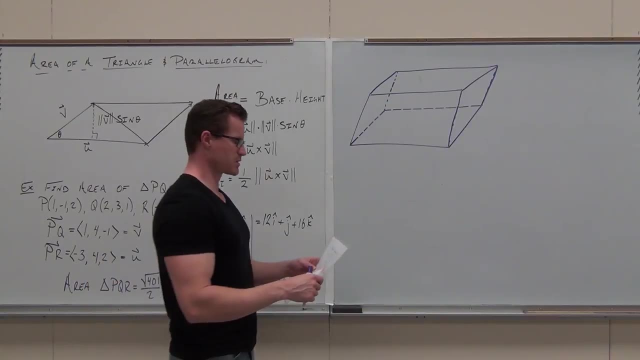 Parallelepiped, Parallelepiped- Yeah, that's what this is. It's a parallelepiped, That's that It's like a parallelogram in 3D. That's what we got here. So let's say that I'm going to use some different vectors. 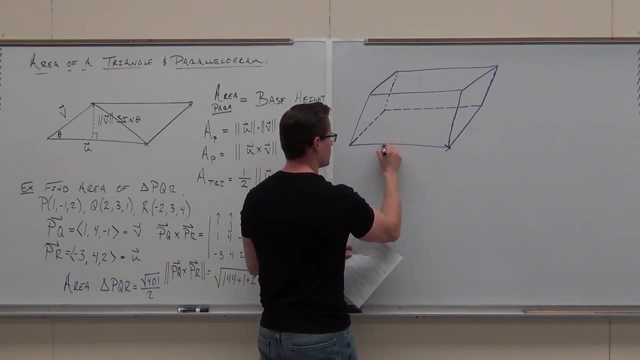 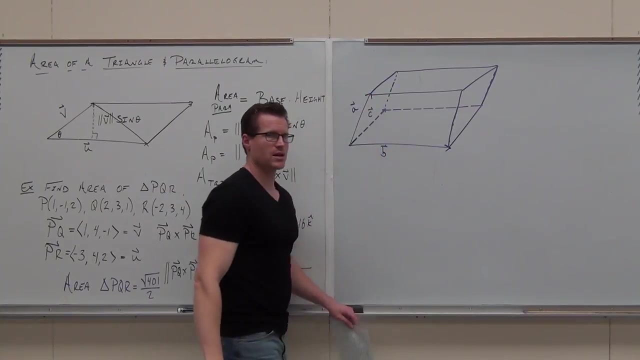 From this point. we've got a vector B, Got a vector C. I'm going to remake it. Got it. We've got a vector A. You guys okay with the picture. If we think about how you really find the volume of something, 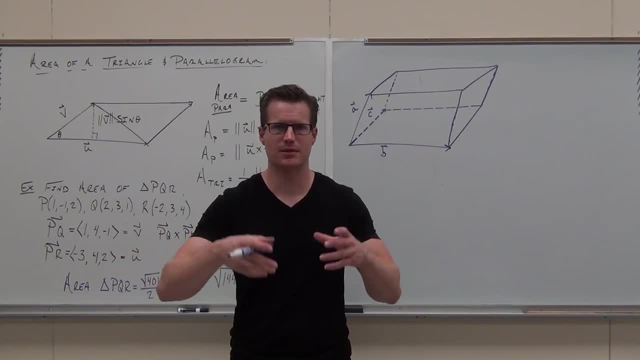 look, I know it's base times: length times, width times height. That's what volume generally is of a regular geometric figure. but you can also do it this way. You can do this Surface area of the base times the height. Why would we want to do that? 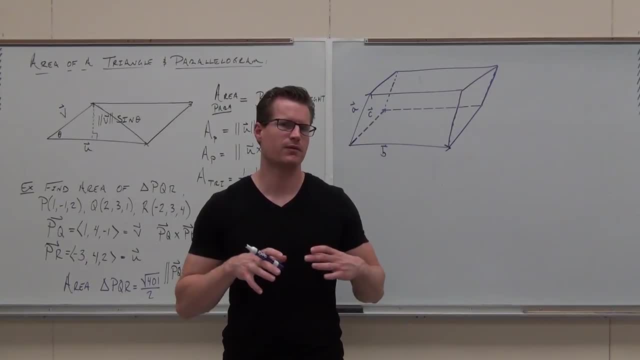 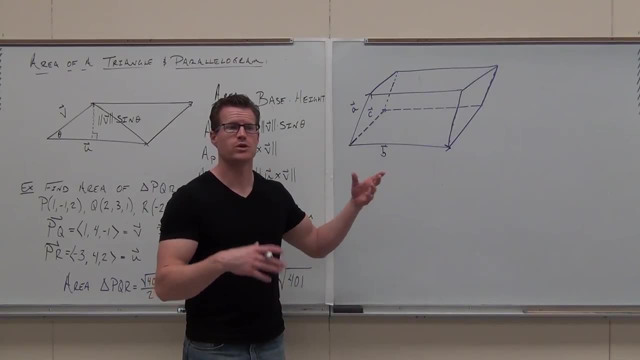 Why would we want to? instead of reinventing the wheel, why would we want to do? the area of the base Surface area of the base times the height. What is the shape of the base Parallelogram? Do we know how to find the area of the parallelogram? 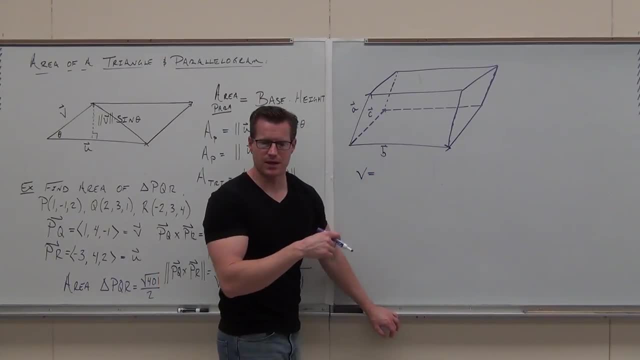 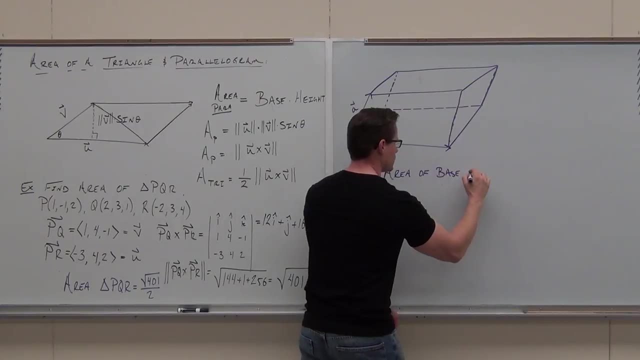 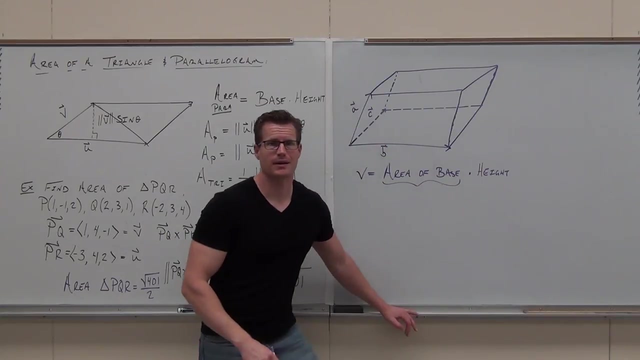 So if the volume is the area of the base times the height, what would the weak point be? So we're going to do that. Yeah, cool, One more Cool So — The bottom of the base is. we're going to do that right away from the bottom of the parallelogram and the basis. 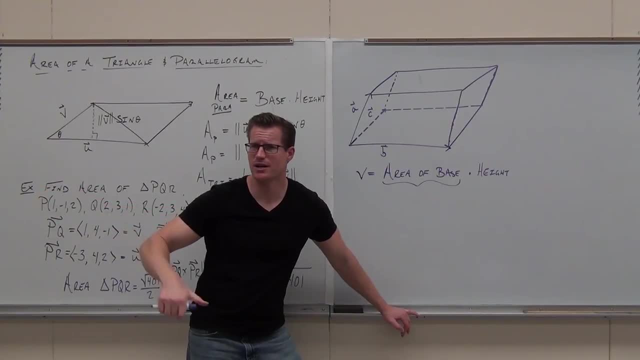 is the second area of the base. It's a magnitude of Magnitude of cross. It's a magnitude of Cross. You were not as excited as you should be on. this is pretty cool. We're putting everything together here and you're going to see some neat stuff after this. 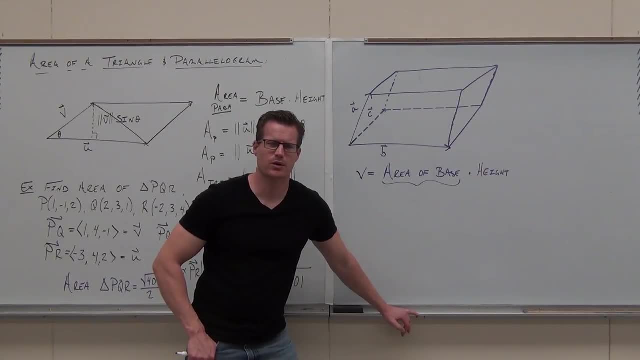 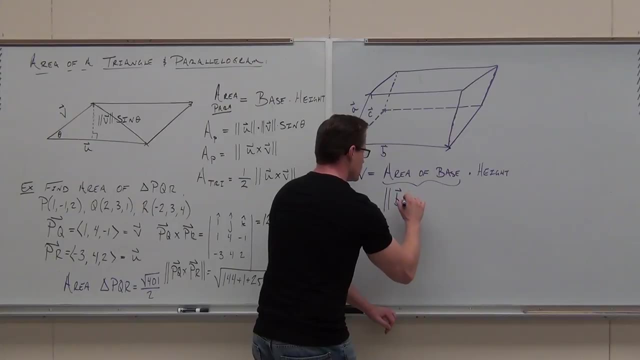 What's the? what is it? It's a magnitude of Cross, Cross. The Cross, Which two vectors would represent the parallelogram, quickly Cross. What is it? So this would be the magnitude of B, cross, C. Now the height, height is interesting. 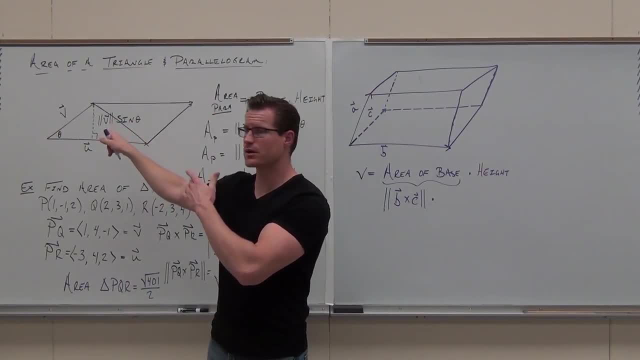 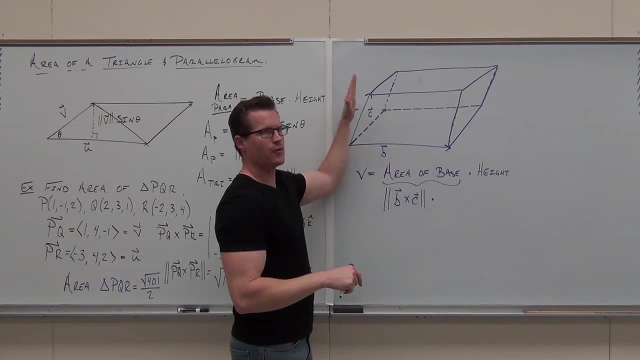 The height. we're gonna do something very similar to this over here. So here we. okay, let's make a right triangle. Well, the height? I don't want it this way. I want the height as an angle off of the actual. 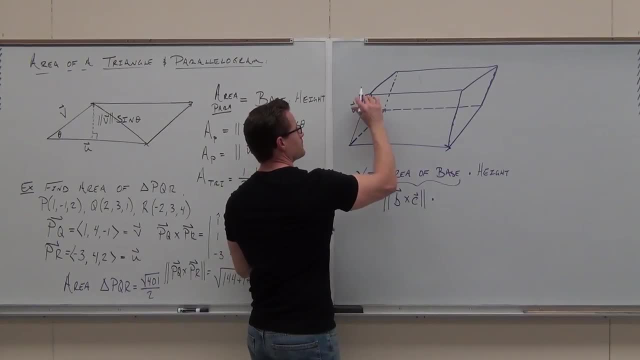 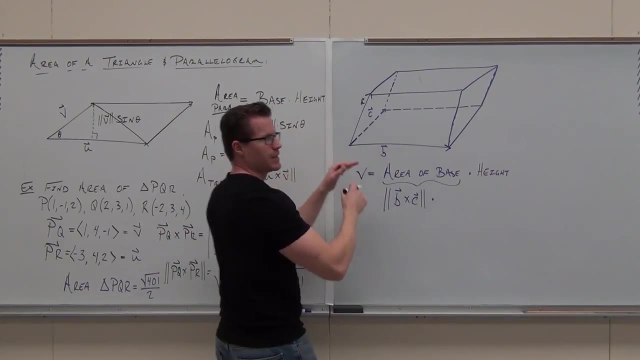 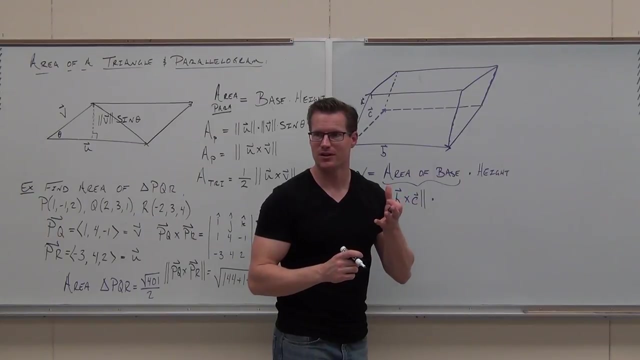 vertical height here. So if I do that I'm gonna make this a little smaller, but that just says A, If I stick something that is mutually orthogonal to both B and C- you hear my emphasis there- mutually orthogonal to both B and C. 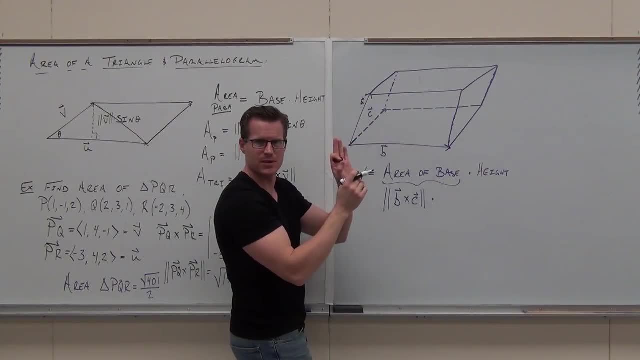 it's gonna represent at least the direction of the height. Does that make sense? So let's just do that. If A has an angle off of that, then really what the height is would be the projection of A onto that height, just like we had the projection. 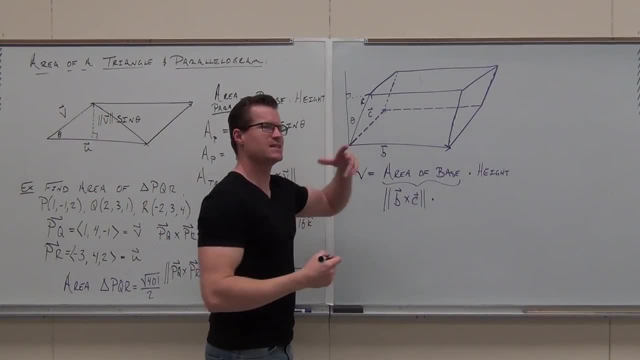 of B onto this height. same idea, only it's a different side relationship. Come on, you know it. you've taken trigonometry. If I have an angle here, and this is my what's that? as far as a right triangle, 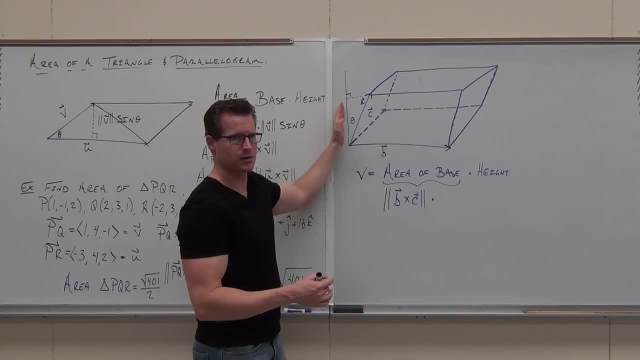 High-bottomed noose, High-bottomed noose, High-bottomed noose. What's this side? It's adjacent, It's adjacent. What compares, adjacent and high-bottomed noose to us Cosine? So from here, this height question mark, if you will. 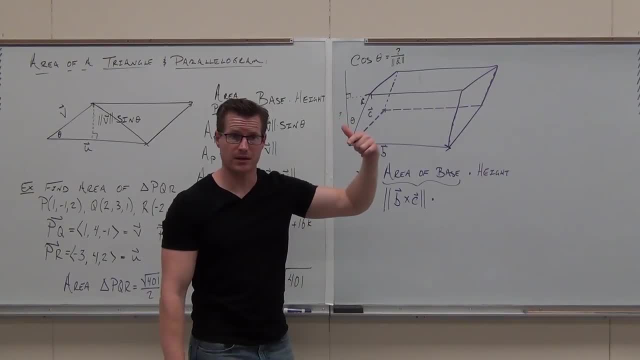 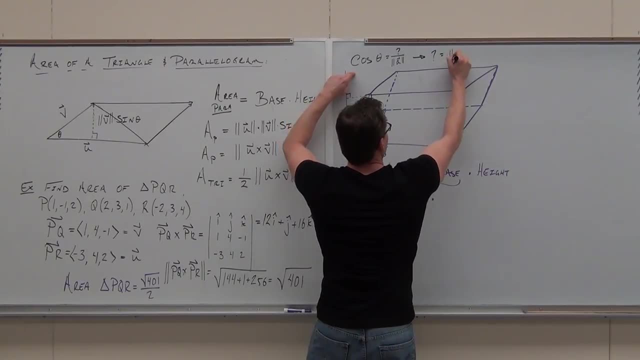 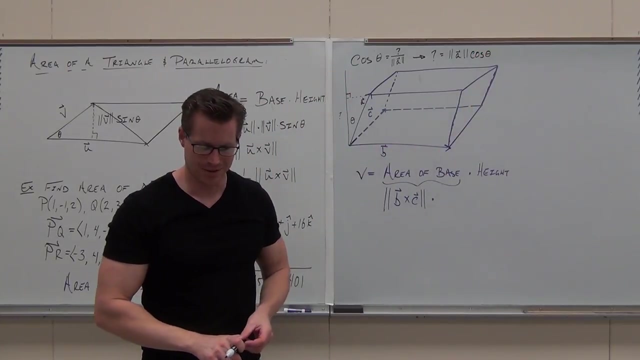 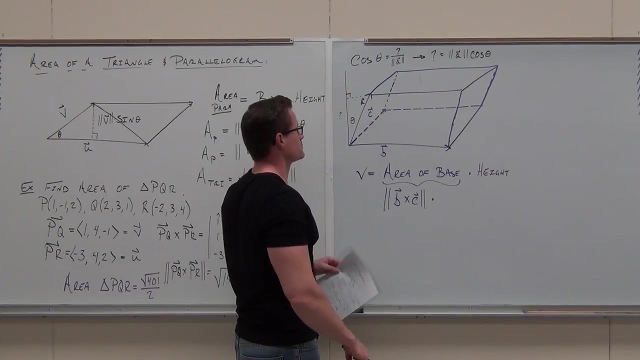 Cosine theta is always adjacent over high-bottomed noose. If the high-bottomed noose is the magnitude of that vector A, then when I solve for question mark we get that. Okay so this question. okay, so this question mark. 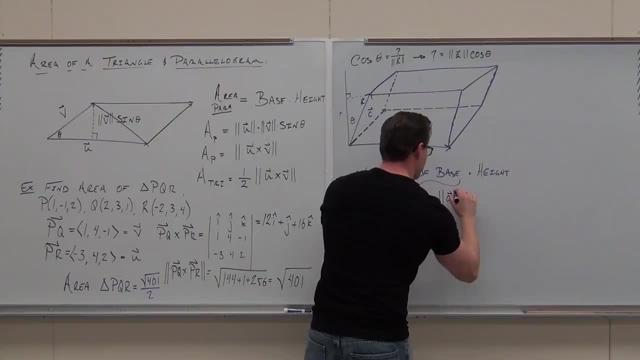 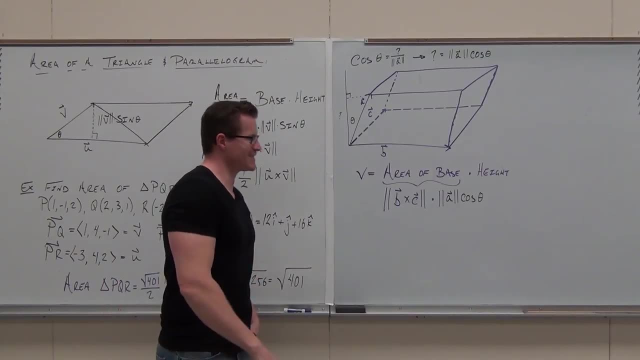 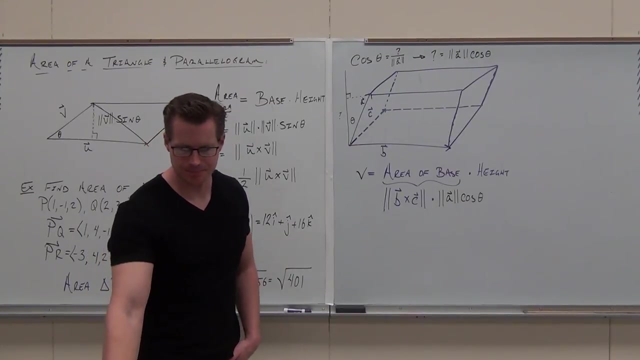 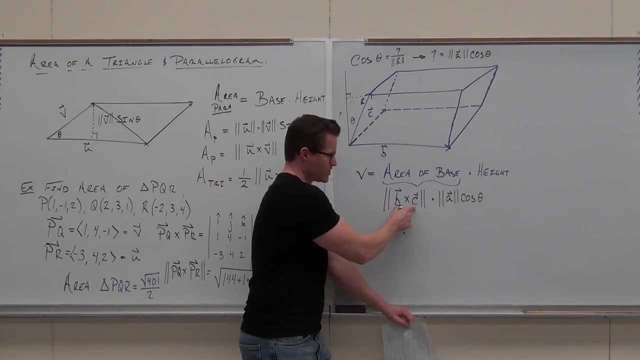 the height. How goes it exactly for that Awesome? what's it mean? Let me tell you. Firstly, let's look what this is. this is a vector or scaler. this, just inside Magnitude, gives us a what's this. 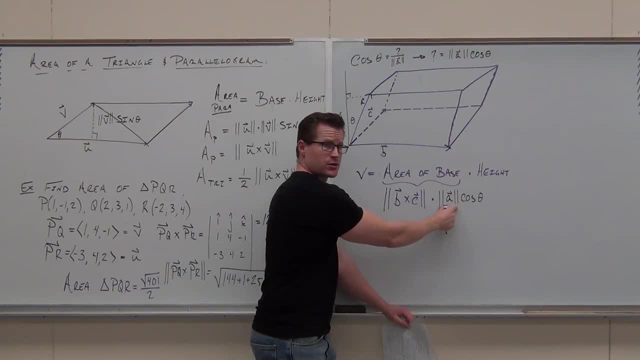 It's vector or scalar, come on, Scalar, Scalar. what's this Natural? If they're all scalars, then that means I can read over. That's what are you doing here? possono ist consider, emp Rama? 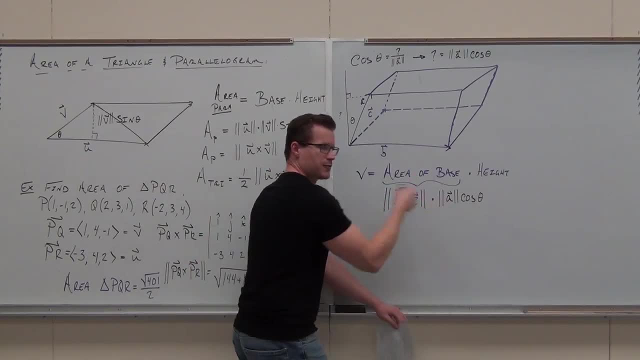 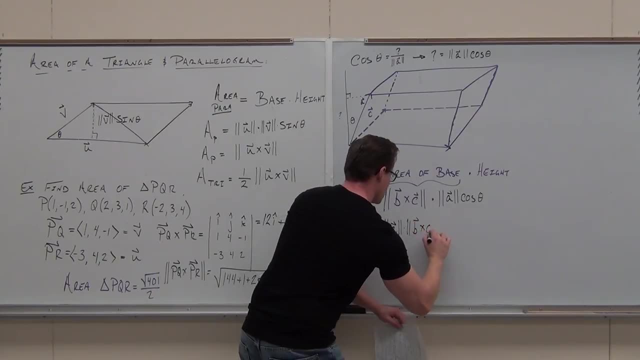 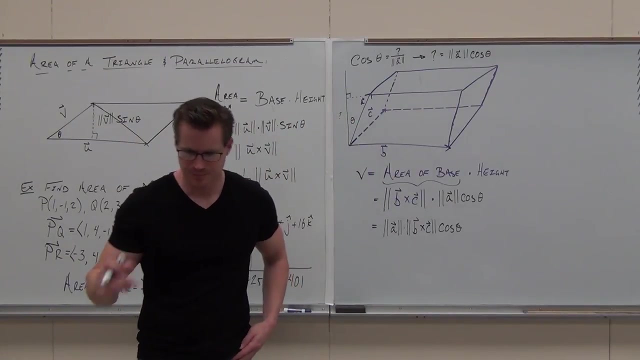 In this equation you have a problems by亲 belomine di Y seconds them. be just fine, I'm going to do that. so what I'm going to do is reorder the a first, and then we're going to use. we're going to use this one more time and then we're 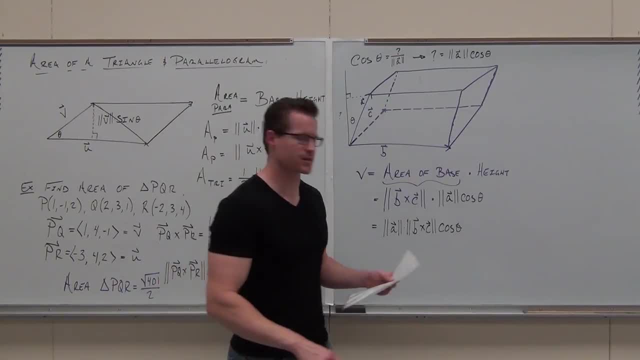 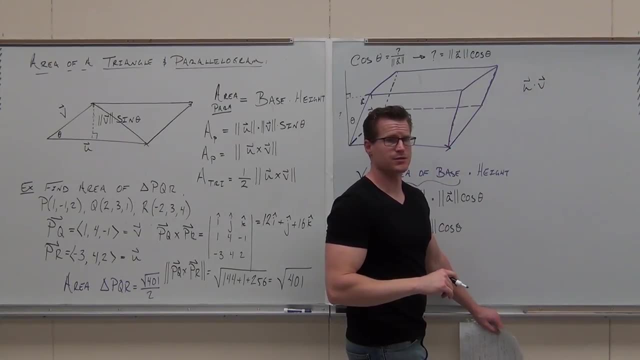 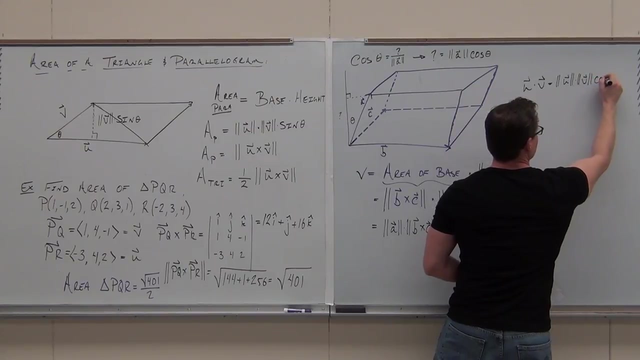 going to bring us some pretty freaking awesome. okay, check this out. you don't need to rewrite this. it's in your notes at least five times. it's there at least five times. you know that this equals that, correct? please look at it carefully, because I'm going to do it here. look at. 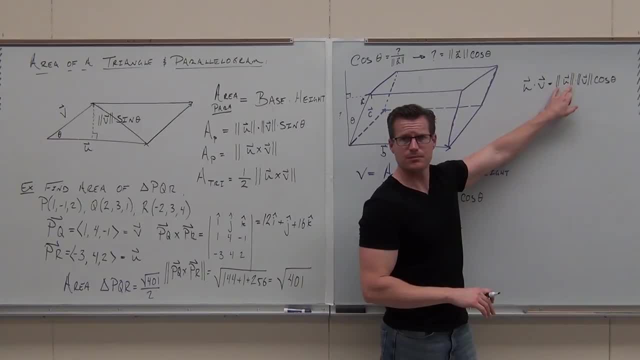 it carefully what this has. it has a magnitude of a vector. it has a magnitude of a vector. it has a cosine of the angle between them. that's what it has. you guys get what I'm talking about. and it equals a dot product of this vector. the first: 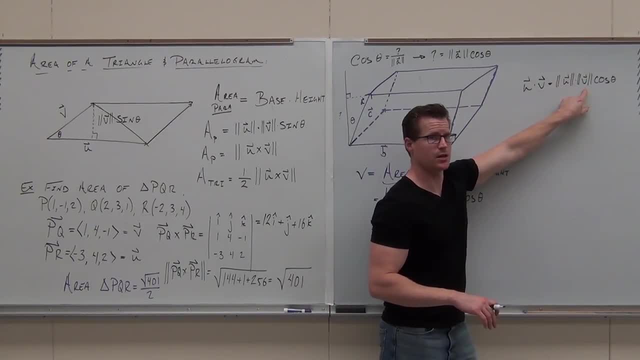 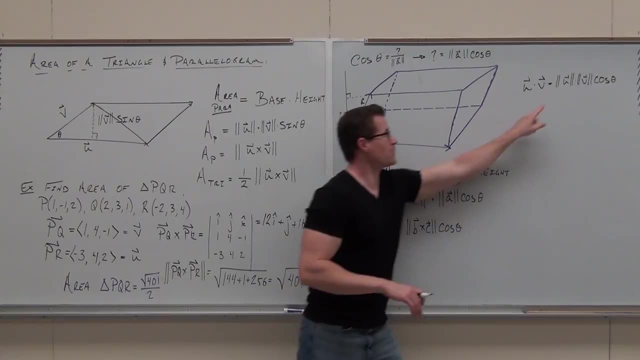 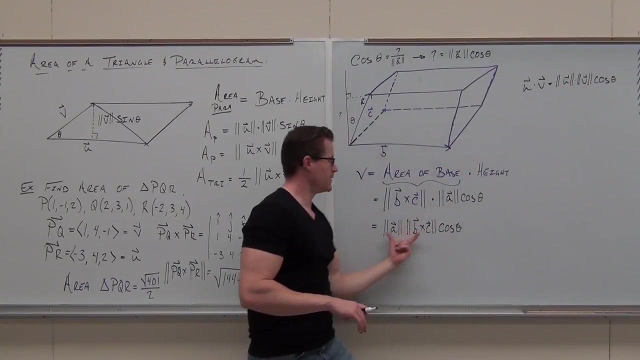 one with the second vector. whatever's in there, check this out. this has the magnitude of vector. this has the magnitude of a vector- do you guys see it right there? and that has a cosine of the angle right there. so if I let this fill in this gap, then this represents the dot product of the inside vectors which 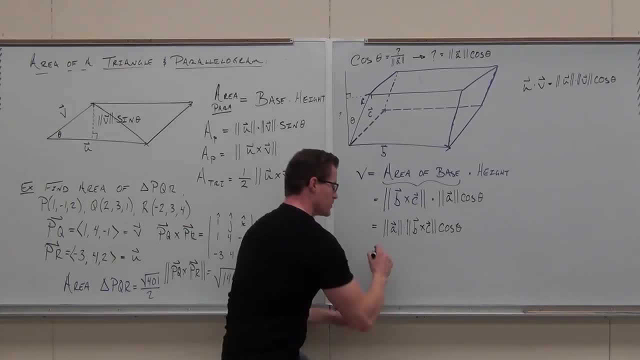 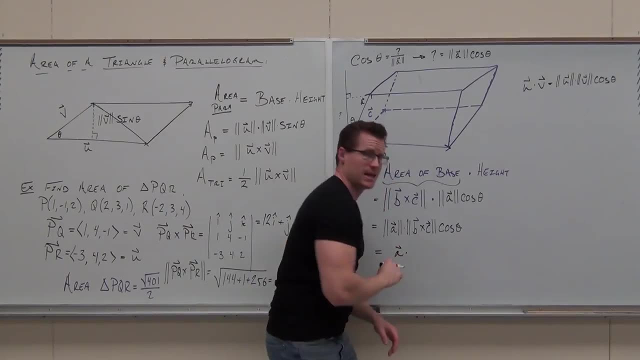 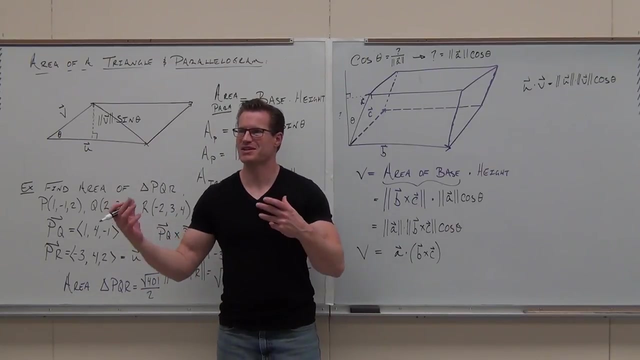 means right here. these are the inside vectors, so this is equal to a or way a dot. so that's the first vector. right, that's in there, a dot. what's the second vector? because B, C gives us a vector volume. is that pretty neat? remember all those things where we did like a cross. 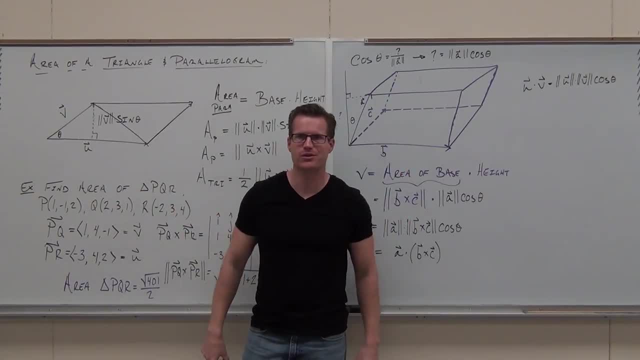 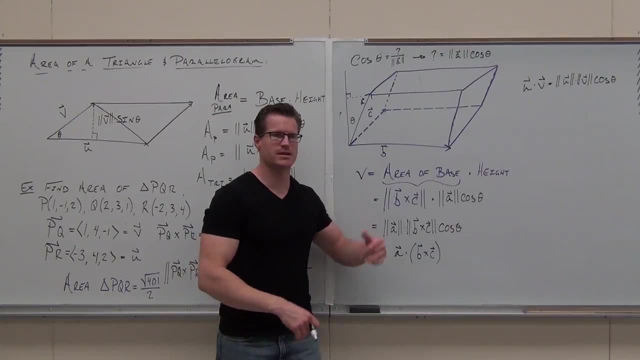 product and that a dot product on it did the homework on that. like where am i ever going to use this stuff? right here, right here. This says: yeah, you oftentimes have dot products with cross products. Why? Because that represents the volume of a parallel. Isn't that pretty cool? 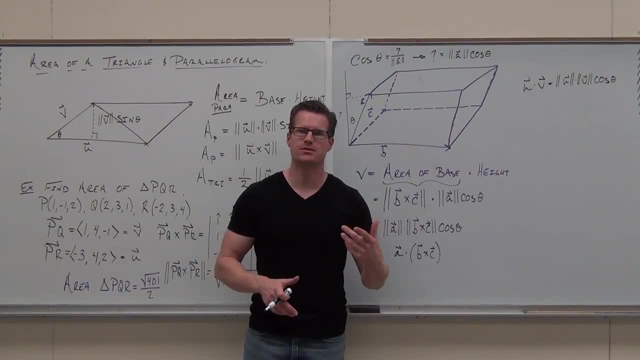 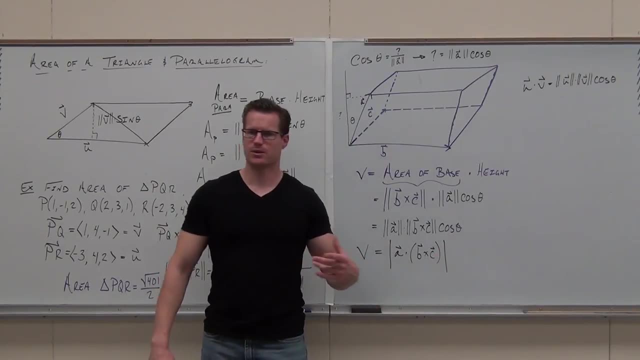 It's pretty neat. There's one more thing that we do. Sorry, I know it's dry, It's a long day. All right, Stick with me, though We do this. That's not a magnitude, because it's already a scalar. It's not a magnitude, It's absolute value, because sometimes we can get a. 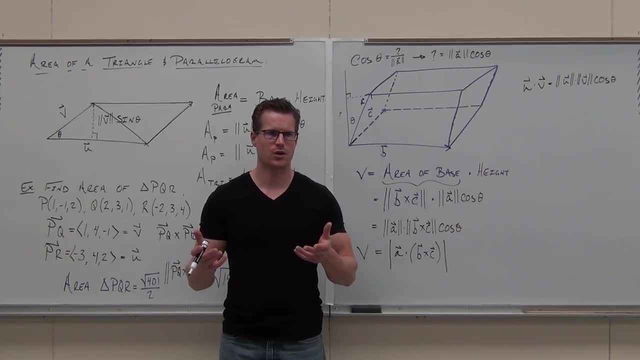 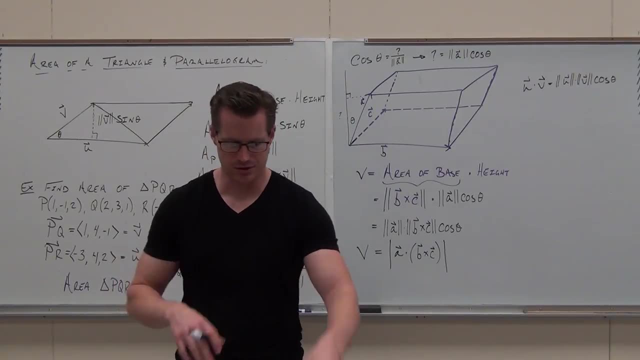 negative. but you go, hey, can volume ever be negative? Nope, That's why we have the absolute value. See, volume is not negative in this case. It just happens if we have our cross product out of whack or something, Y'all still okay with what we're talking about. We're going to wrap it up. 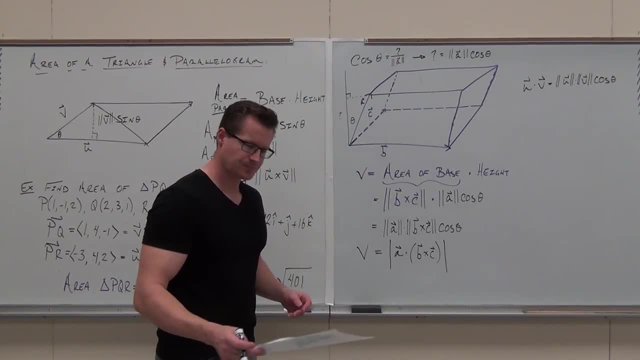 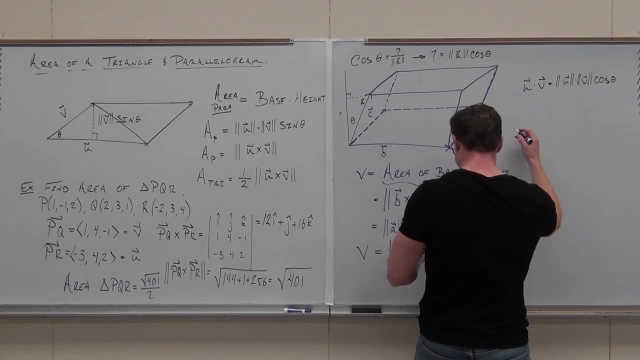 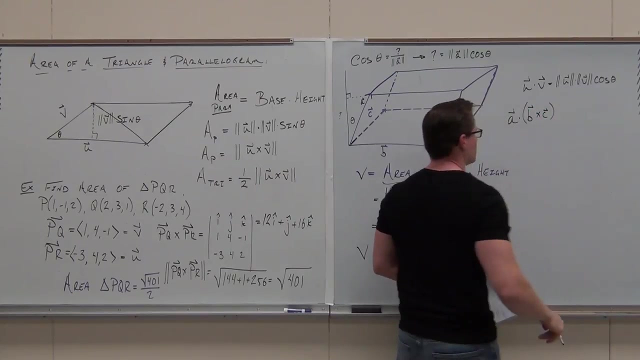 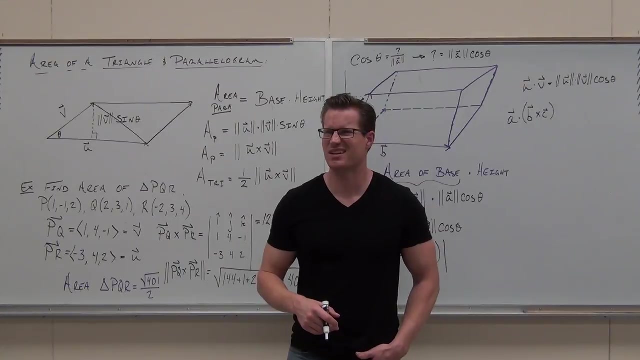 I want to do one example Before I do that. yeah, I'm going to have to prove it. I'm going to do it. I really hope you like this. It takes me a lot of time to actually go through this thoroughly and do this. I could just give you the formula, but it sucks. I don't want to do that, So I hope. 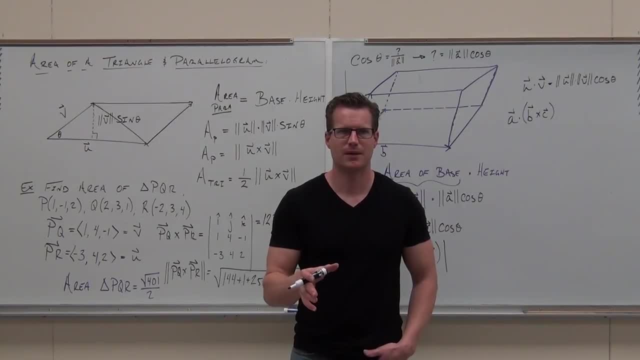 you enjoy it, because we're going to take a little bit of time to prove this. but check this out. If you wanted to do A dot B cross C, you would do the B cross C first, because the only way that you can figure this well, you could distribute it. but I would do the B cross C first. 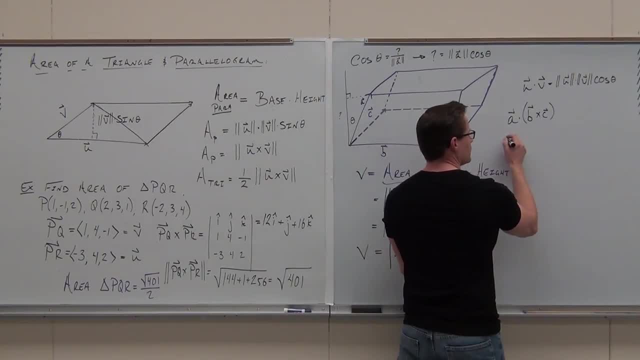 So I'm going to start with that. So what this would equal, what this is, we would get this whole IJK B1,, B2,, B3, and all this stuff, And you know what. If you want to write it down, great, If you. 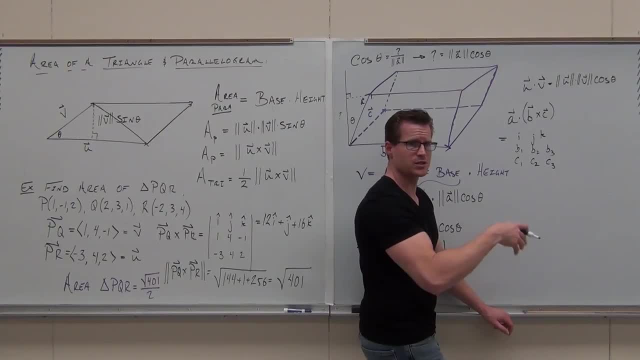 don't want to write it down, that's fine. You don't have to write it down, but what you need is the punchline on this, because I'm trying to make your lives easier. Okay, this is going to make your lives easier. It's really cool. That's what I want to give it to you. 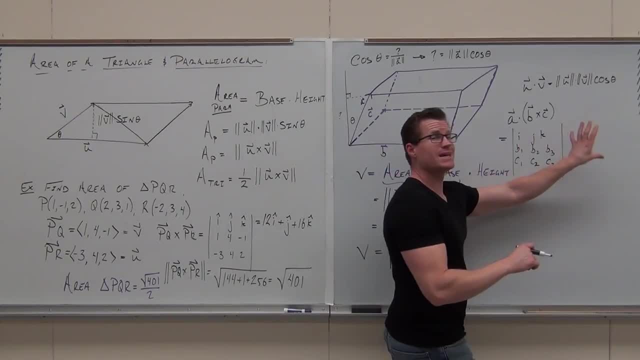 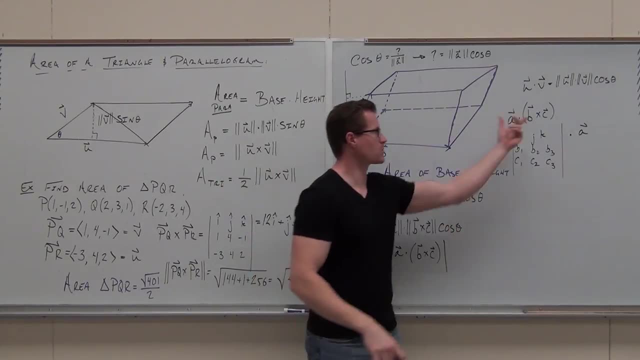 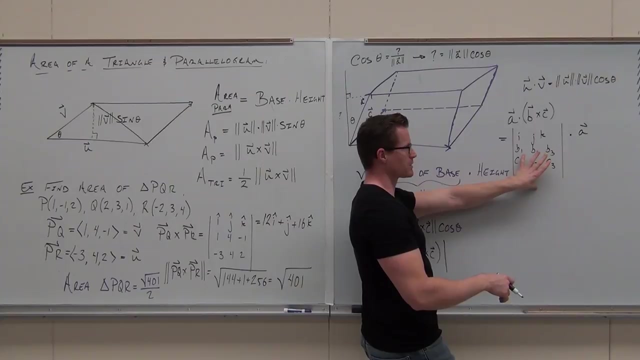 And then whatever we get, whatever we get, we would dot it with A. Why? We know dot product is commutative, so we know we can switch around. So if I do the cross product and the dot product afterwards, that's fine, Same thing. So whatever I get out of this, this is the cross product. 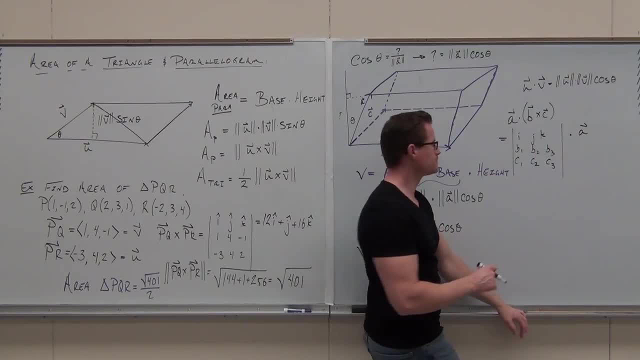 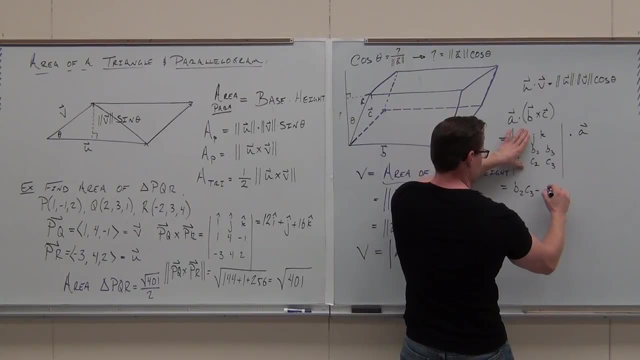 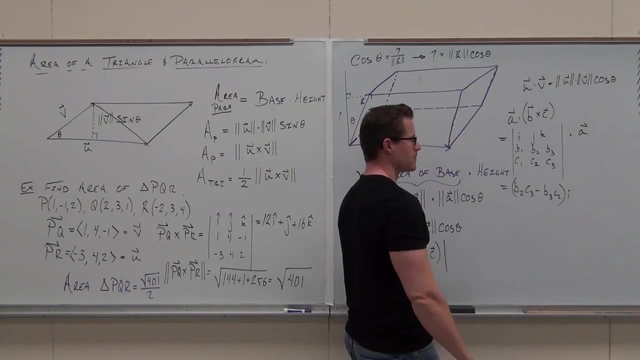 I'm going to dot it with A. You follow what I'm talking about. Check this out This whole thing would give us, But I'm going to write it this way: I minus. so this is this, And if I make a mistake on the notation, please stop me. I don't want to get all the 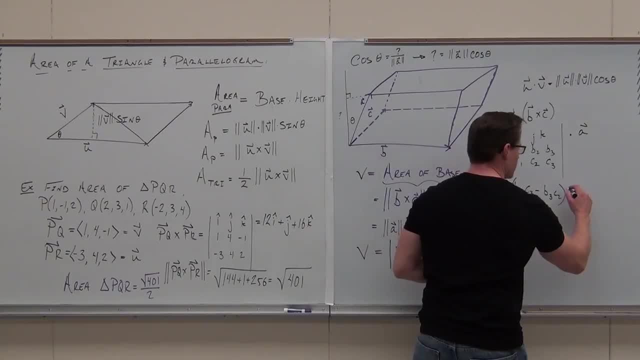 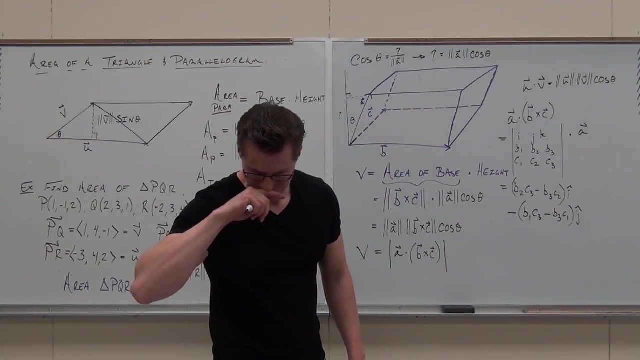 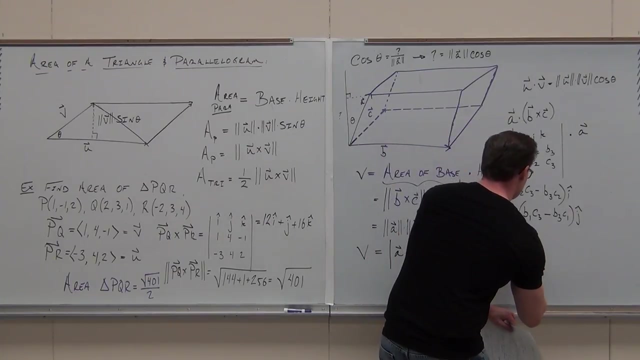 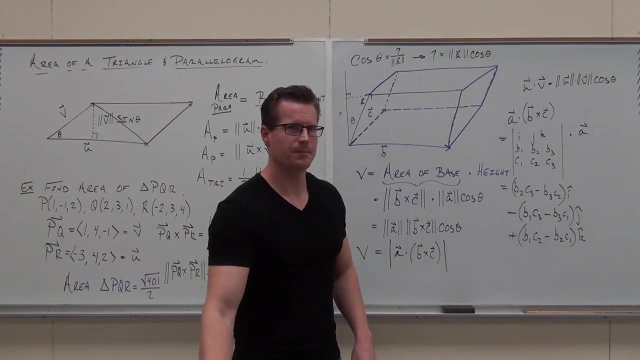 clues and have something wrong. all right, So this, this with our I, You guys okay with it. And then we would go: okay, all right, Cover up the middle With the J. That's what we'd get, yeah. 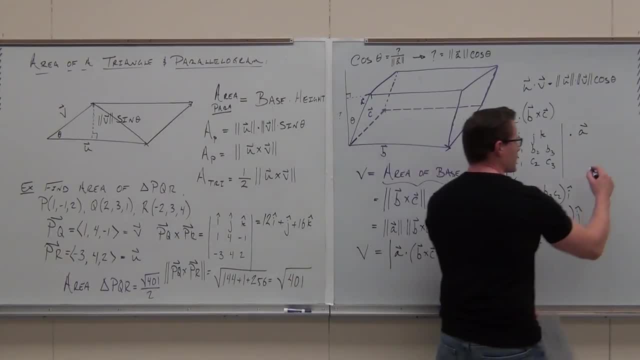 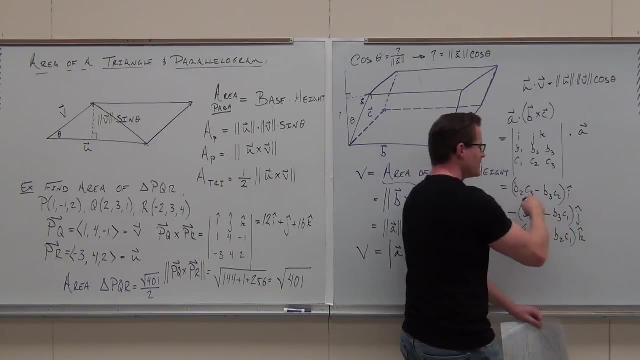 But here's the interesting part: If you dot product this with A, what happens is all we would do is we would multiply. Can we do something just kind of crazy here? Can we just call this number one, number two and number three? 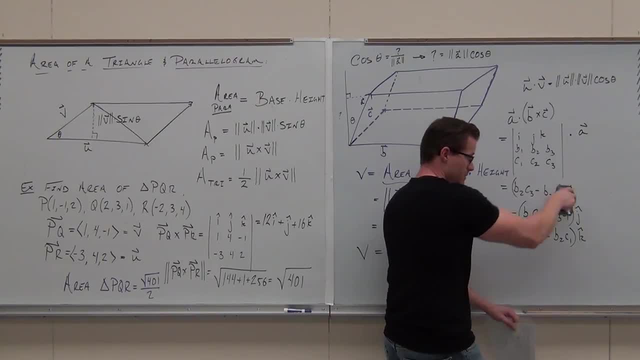 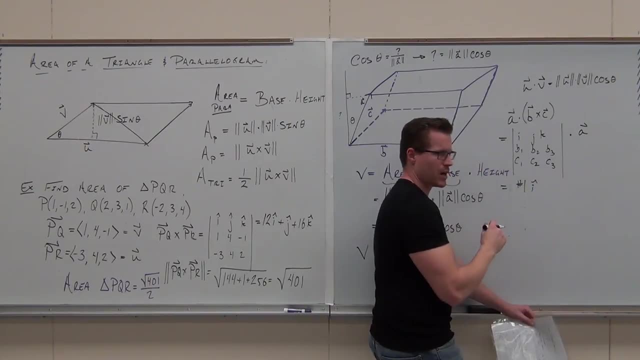 Would that be helpful for you, so we don't get all screwed up on this? So what this is going to give us, I mean this, this is it, But this would really just give us this A number with I, some other number with J. 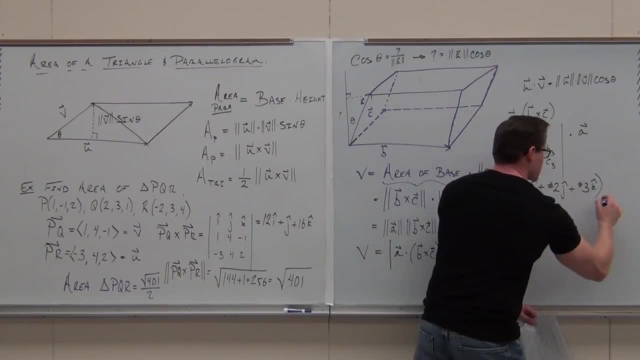 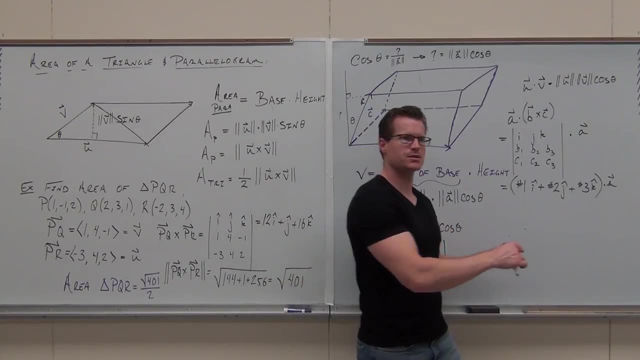 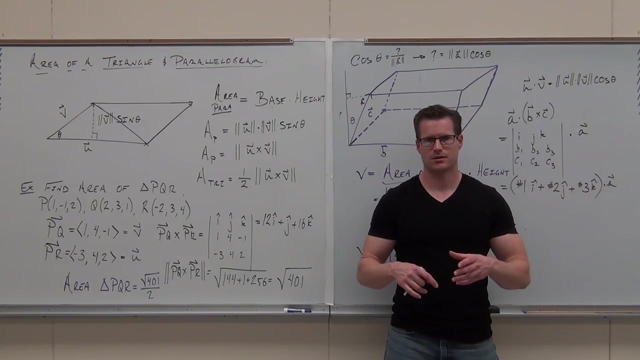 some other number with K and then I would dot this with A. But when you dot that with A, check out what happens. What happens when you take a vector dotted with another vector? Do you get a vector, What do you get? 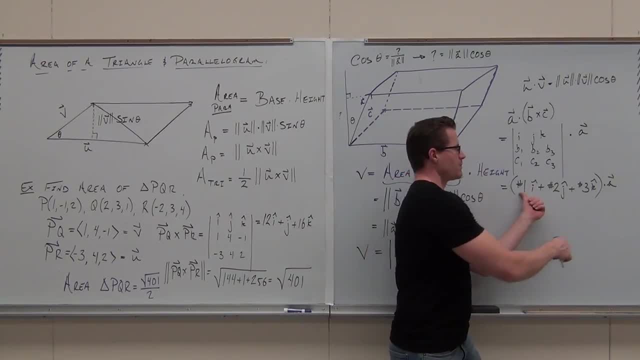 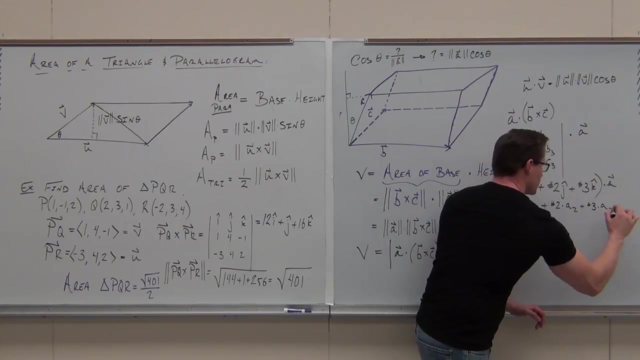 You get a scalar. In fact, what happens? I would take my first number and my first component. I would have number 1 times a1.. I would have number 2 times a2 and number 3 times a3.. That's what that dot product would actually look like. 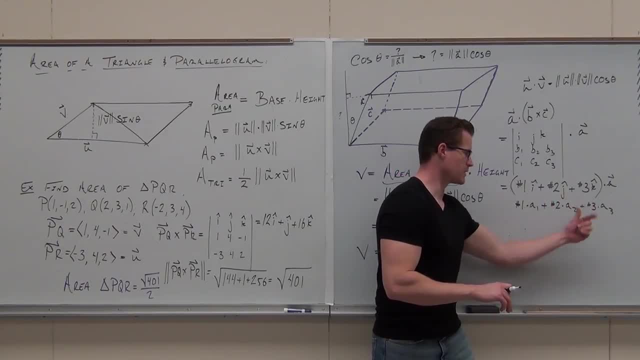 A1 and put it here. A2, put it here. A3, put it here. I'd have no, i's no, j's no, k's whatsoever For real. are you guys okay with what I'm talking about? 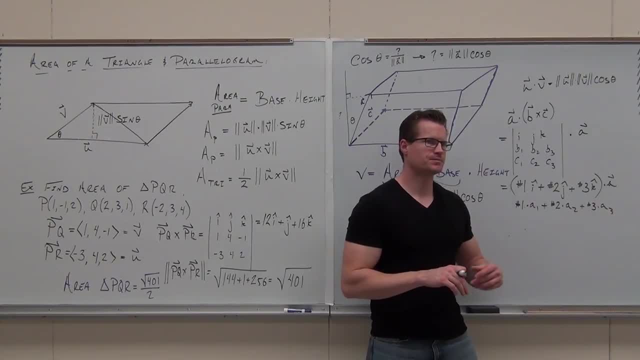 Here's the cool part. What would happen if, instead of having i, j and k, I just put a1 and a2 and a3?? Do you see that a1 and a2 and a3 are simply taking the places of i and j and k? 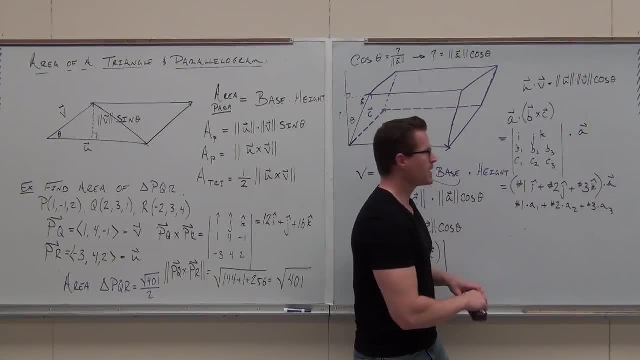 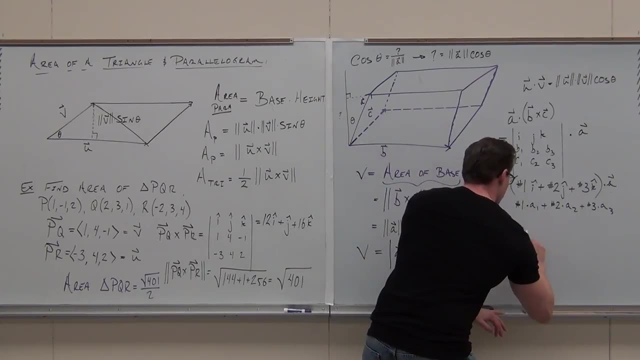 Do you guys see that? Then there's another way to do this. If you ever have a dot product with a cross product, the easier way to do it Is that right there. Replace i, j and k with a1,, a2, and a3,. 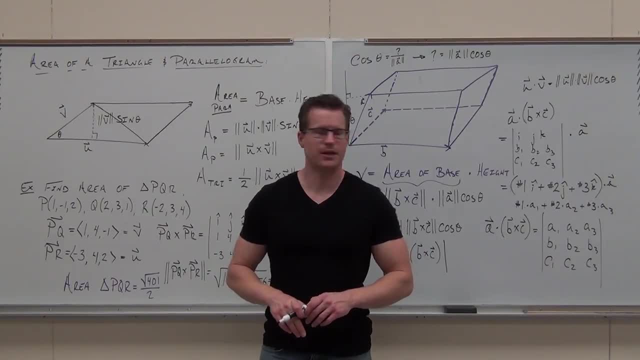 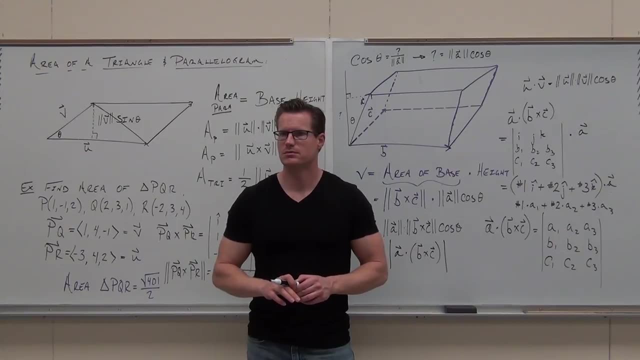 and you save yourself the headache of a dot product at the very end And you do it exactly the same way you do any other 3x3 matrix determinant. Isn't that kind of cool? Do you guys want to do an example now? 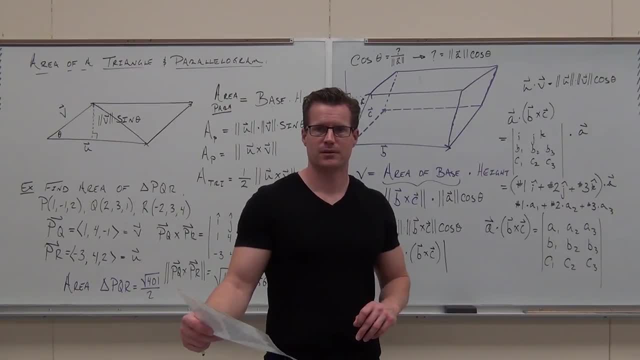 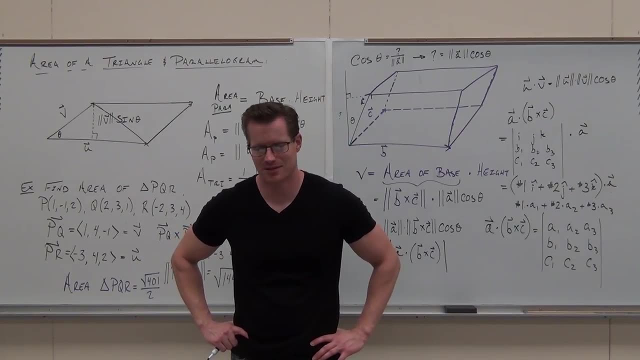 or do you always want to take a little break and then come back and do it? You guys really are not going to talk to me today. huh, You've beat my head into submission. I don't care anymore While it's fresh. 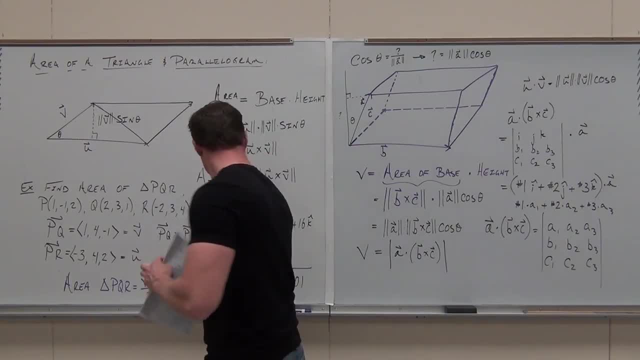 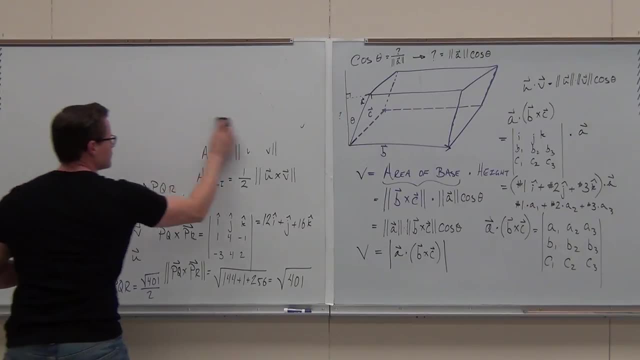 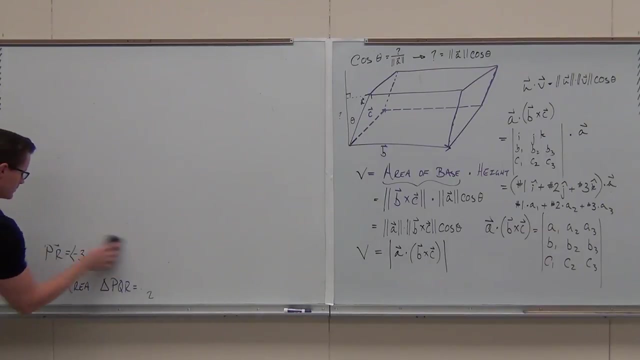 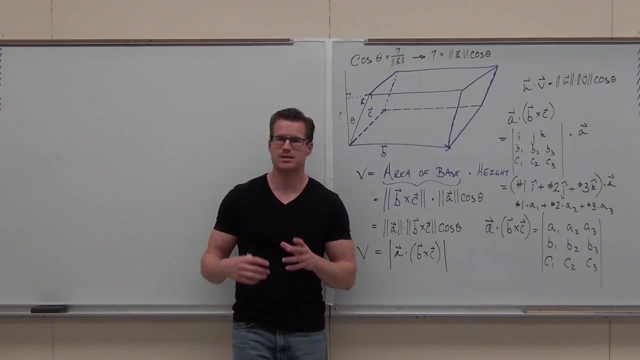 let's just go ahead and do it This right here. No, it's not a magnitude because it's not a vector. What's this thing going to give us? It doesn't have any. i's, j's or k's. 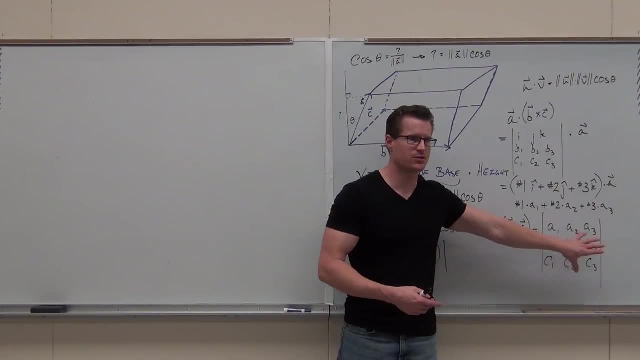 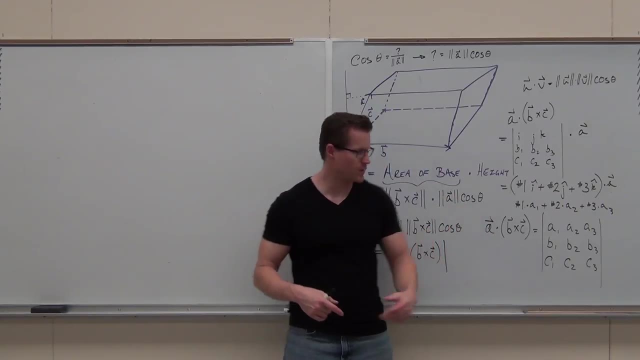 So when I find the determinant of that matrix, I get just a number, and so I don't have to find a magnitude. but I do have to keep it positive because our volumes are positive. That's why this is absolute value here and we don't need that magnitude. 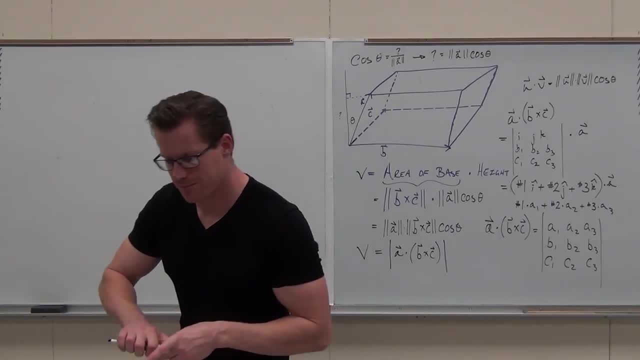 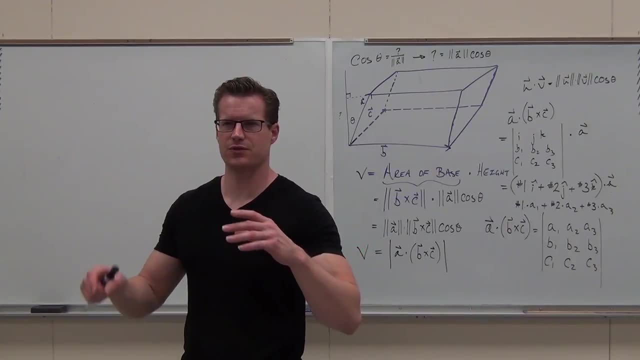 Does that make sense? Let's try one. So I'm going to give you. How many points do I need here? Three. I needed three points for two vectors because I have originating point end point. I have originating point, end point. 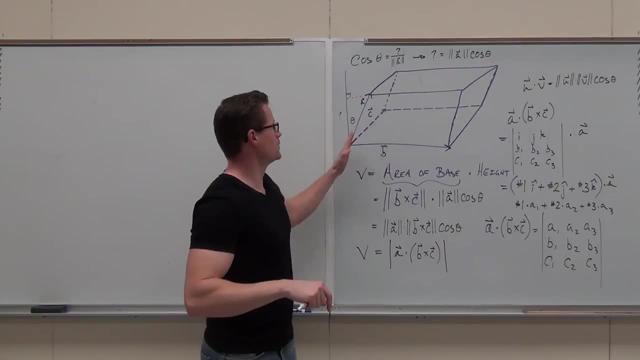 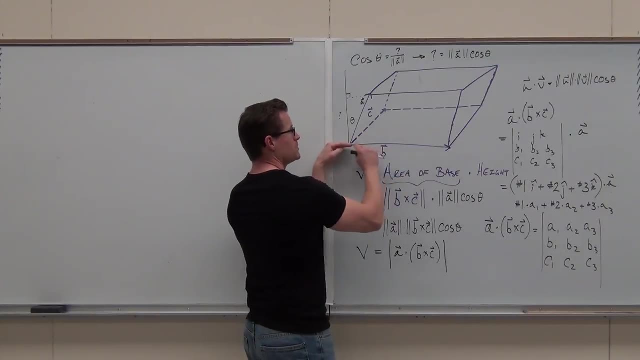 How many do I need for one, two, three vectors? How many points? I need four, because I have one, two, three and four. Did you guys get it? So I'm going to give you four points. We're going to find the volume. 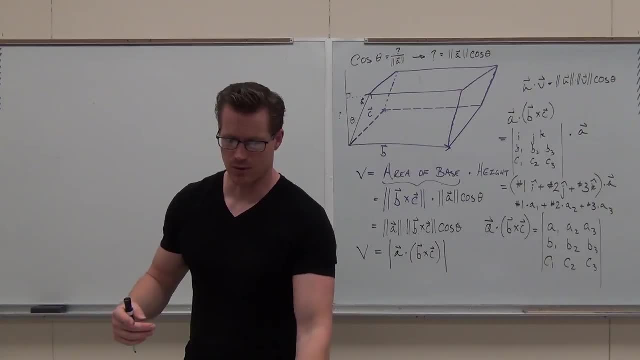 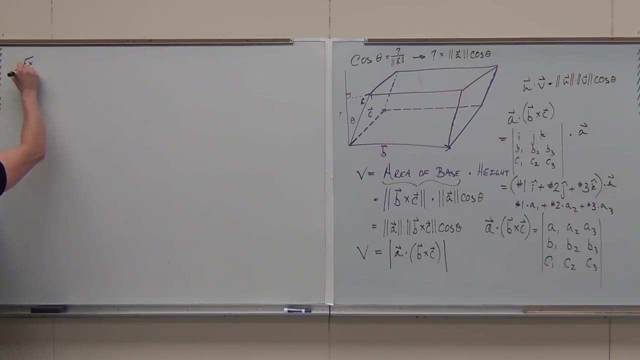 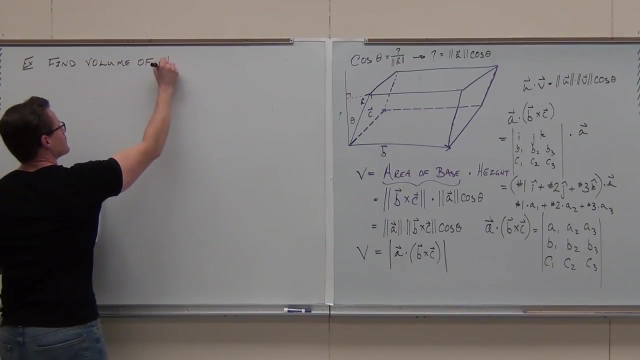 of the parallelepiped and then we're going to call it good. I'll talk about one more question and then we'll take our little break because we need it. That's parallelepiped Find volume of the PP. Find volume of the parallelepiped. 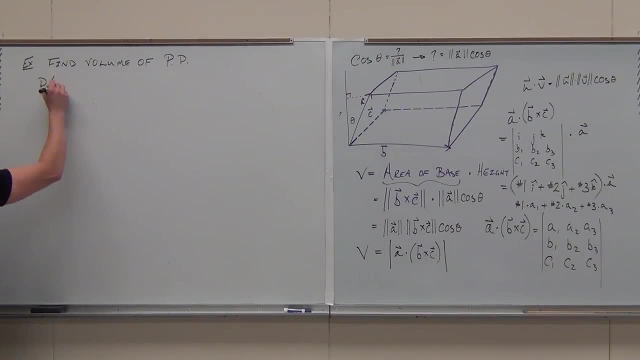 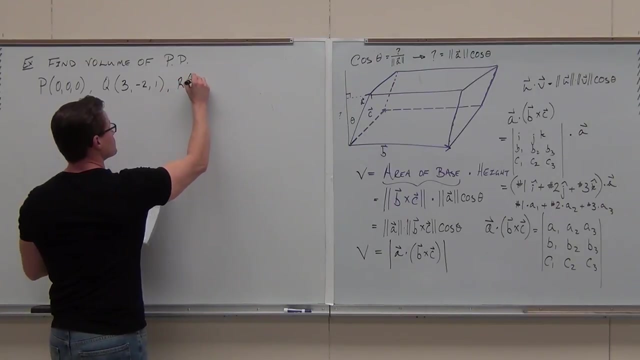 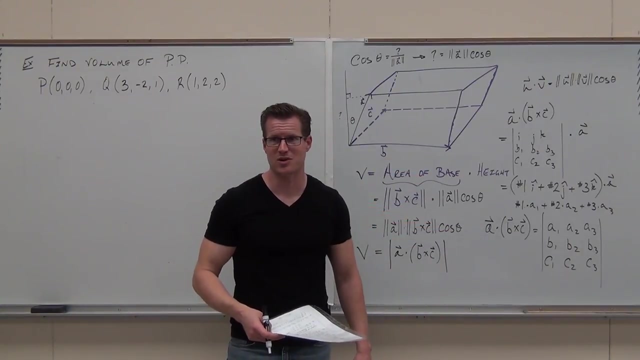 when. here's your points. By the way, some of you were giving me death looks when I was doing this and you're like, oh my gosh, Leonard, I hate you so much. right now You're going to love me. 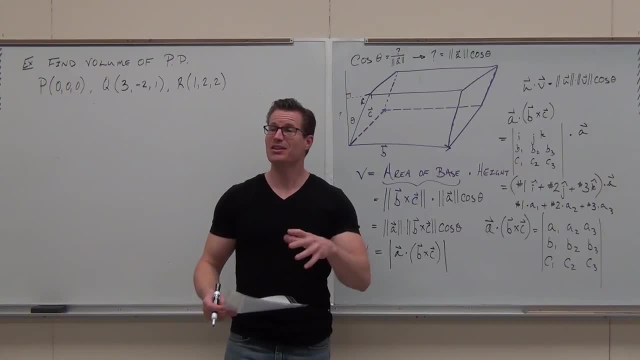 Love me, Love me. You're going to love me when we do this problem. Trust me. This is going to be a test question. It's going to be the easiest one, unless you mess it all up. All right, It's not messed up. 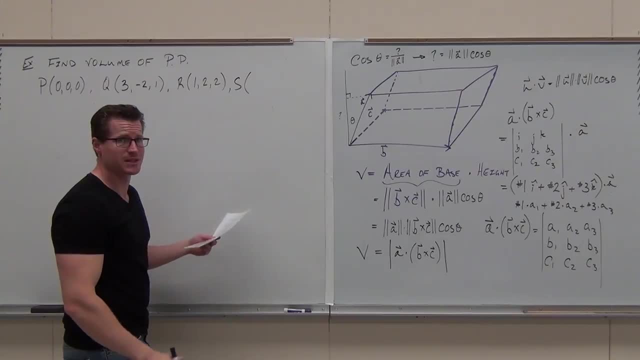 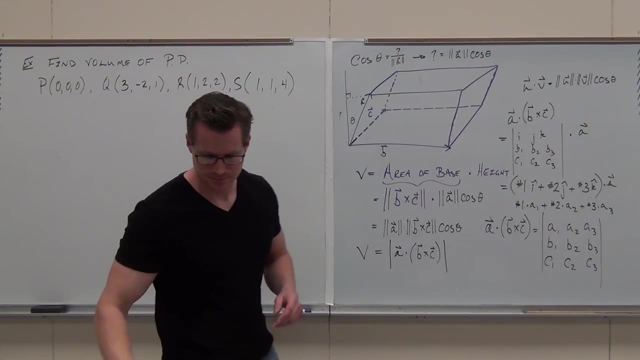 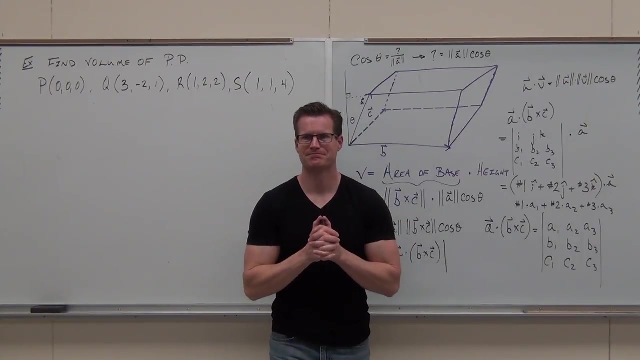 It's going to be the easiest one because of what I just showed you right there. Trust me, Trust the Leonard, It's going to be nice. It's going to be nice. Are you ready for it? Do you have it written down? 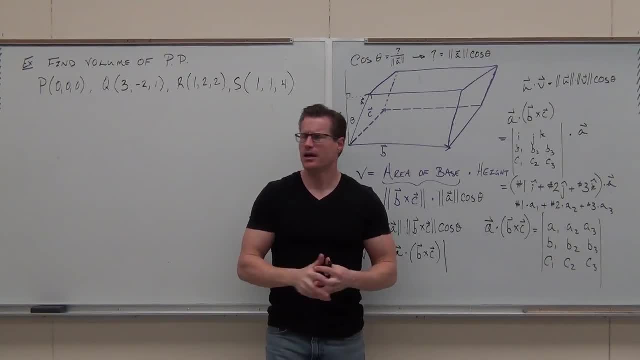 Firstly, what are we looking for? Volume Area- What is it? And I give you these four points- What we're drawing is this picture. Do we actually have to draw it? Thank goodness, no, We don't have to draw it. 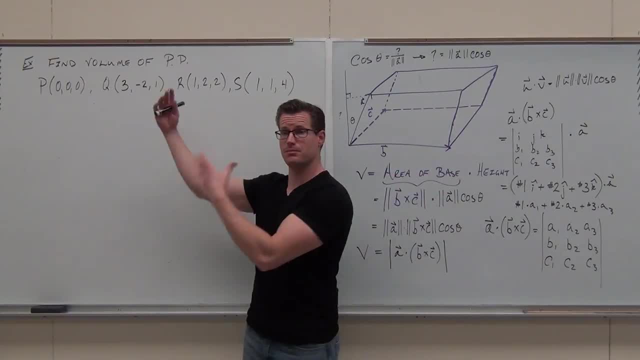 But we do have to know what this is based on. Is this based on points or is this based on vectors? What it is, Points. This is points. I want vectors. Can you give me vectors from the points? Yes, That's a big part of the class. 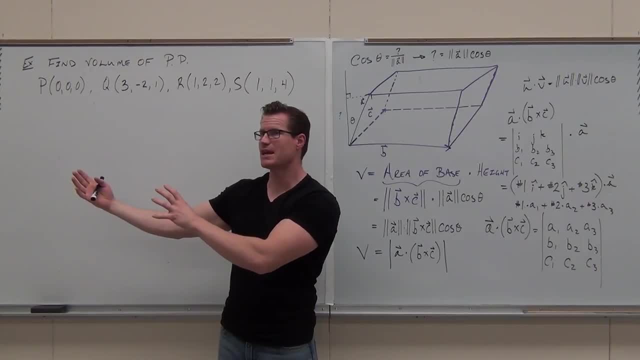 Find me vectors from my points right now. It's going to be really easy. if you start with what letter E, Please start with P, because it's zero, zero, zero. You'll be subtracting zero, But go through and find me the vectors. 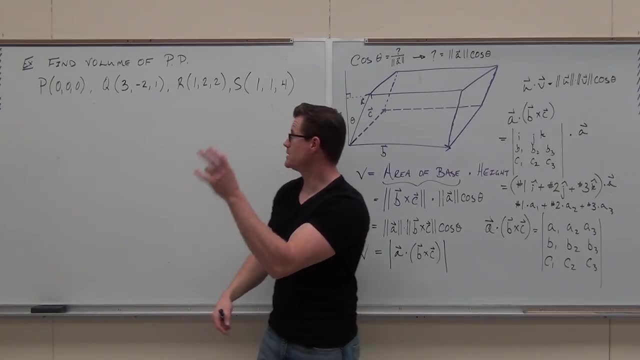 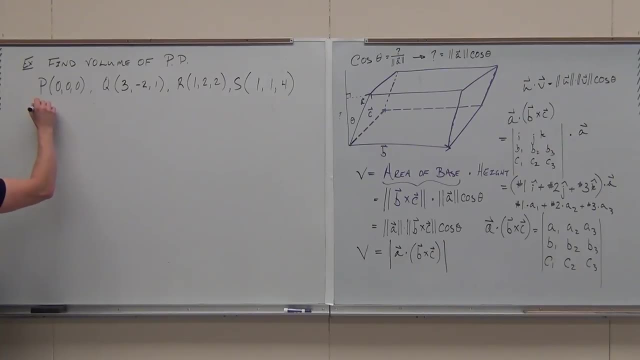 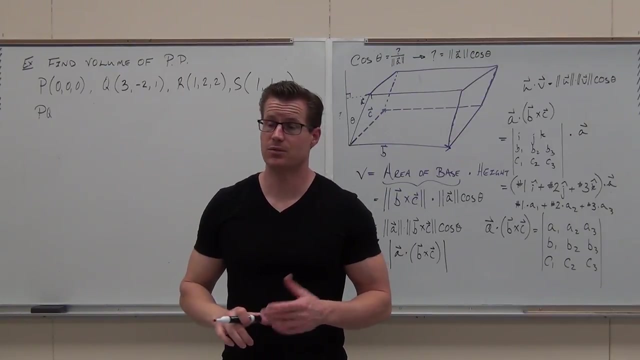 You're starting with P every single time also. So I want PQ, I want PR And I want PS. If it helps you to define these as like vector A, vector B and vector C, that's fine too. It really doesn't matter. 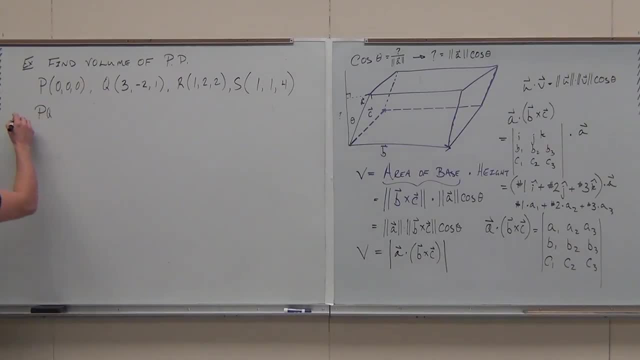 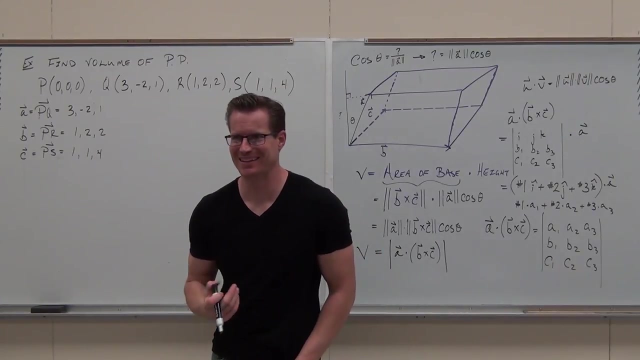 But if it helps you, then do it. I really hope you had an easy time doing that Praying man. please let them get at least this, please, please, Why is it so easy? Because the origin and we know position vectors start the origin automatically. 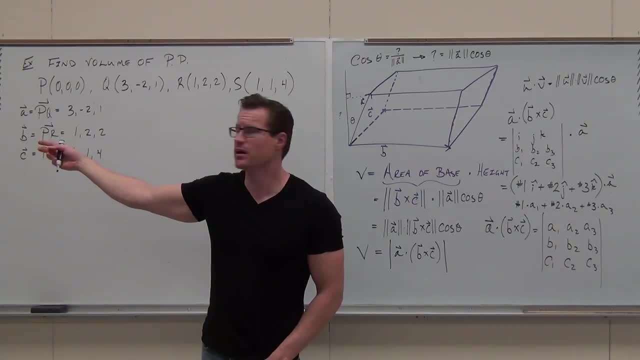 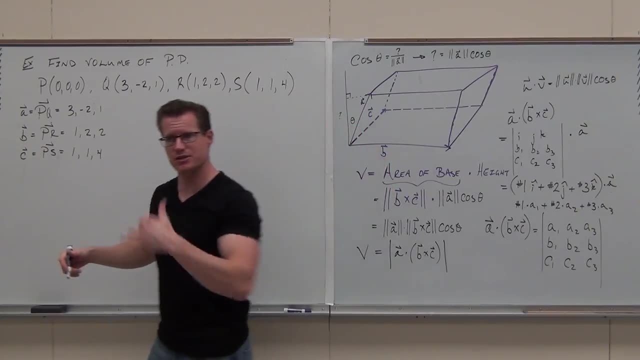 at the end of the terminal points, But I've left the notation free. What notations do I have here and here? Phrasings, or those little brackets? Phrasings, Because now they're vectors, now they were Okay, so you're on your homework. 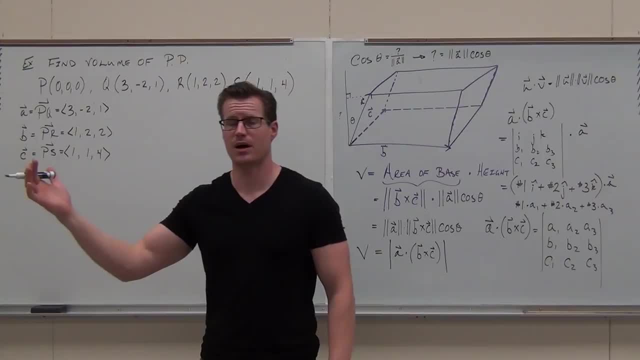 You're doing some of these problems. You come across this, You go. man, I don't know how to find the volume of parallel pipette. There's a formula for it. You get to have it, That's fine. How do you find the volume of parallel pipette? 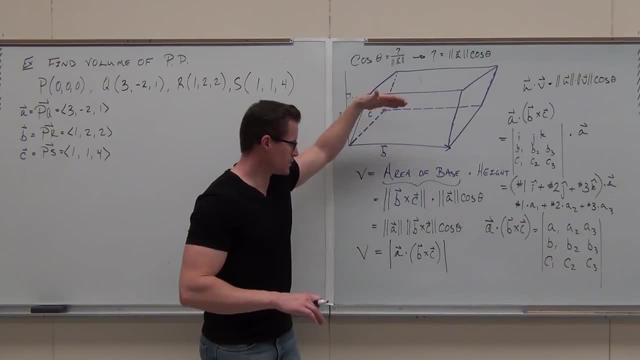 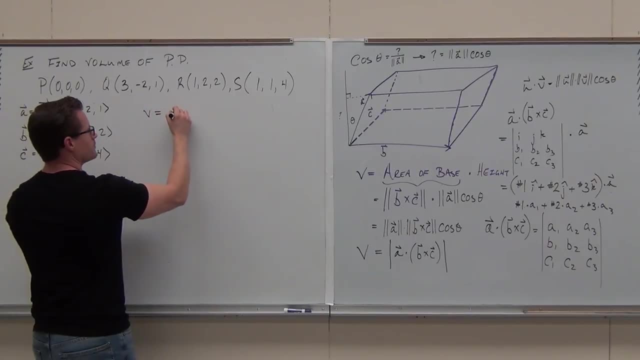 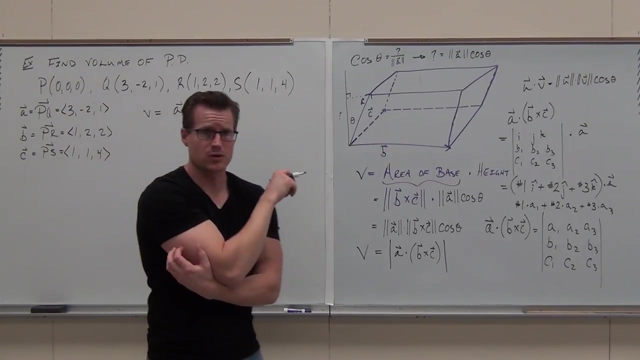 Why we did all of this work- because it was a lot of work- is you get down to right here And you go: okay, the volume Is A, dot B, cross C, And if we get a negative, then we're going to change it to a positive, okay. 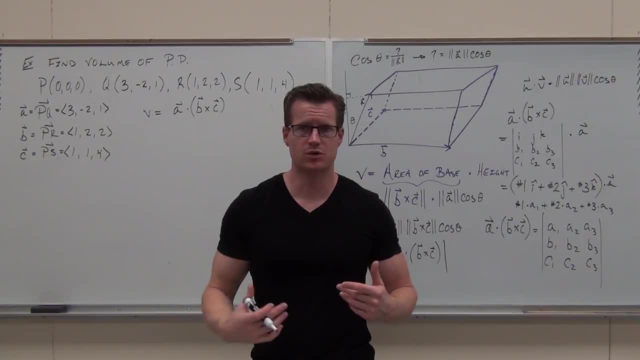 Because it does have absolute value around it. I'm not putting it because I don't want to confuse you with magnitude. It's already scaling. You can't even find magnitude, But it does have the absolute value. Nod your head that you heard me. 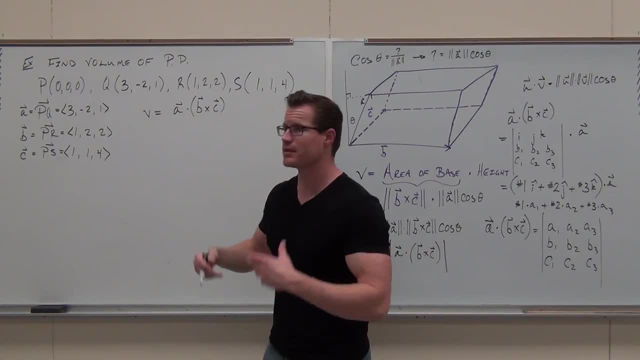 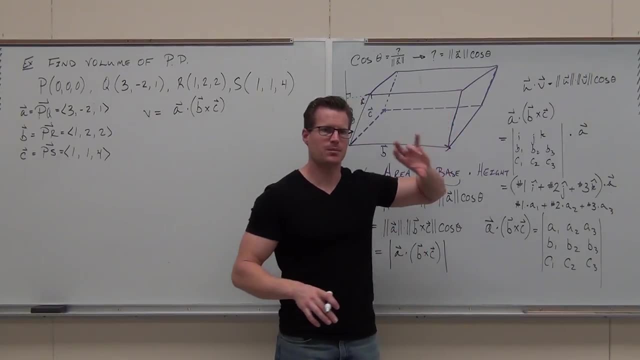 You understand what I'm talking about And you go: man, that's nasty, You've got to find a cross product, then a dot product. And they go: wait a minute, We burned 20 minutes of class, so we go over here and go a dot product. 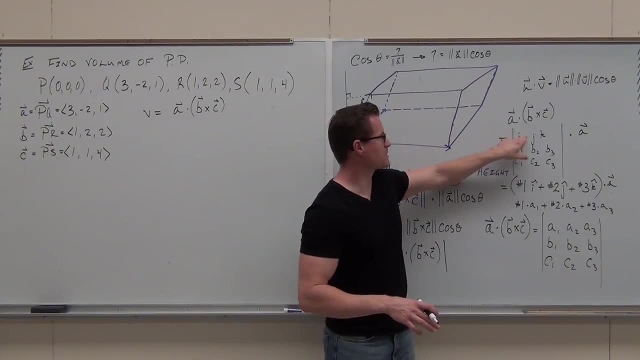 on a cross, A cross product, simply replaces this vector, this unit, well, this coordinate vector. we'll call it The I, the J, the K. It replaces this vector with this vector. Just slide this one right over, And that's exactly what we've done. 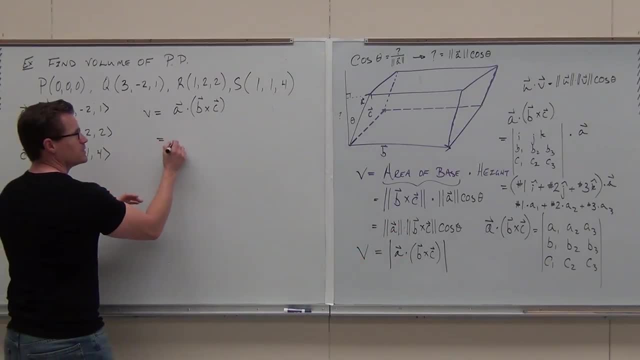 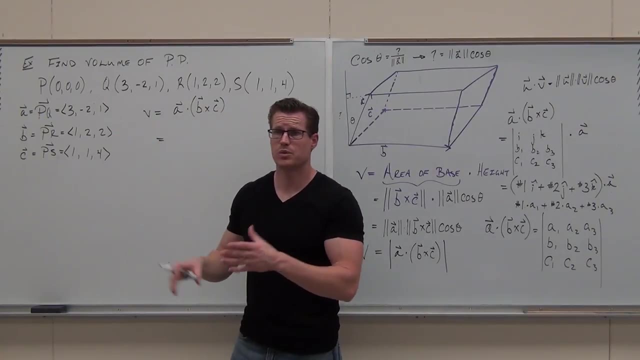 So literally all we have to do- follow the clip carefully, okay. All we've got to do is go: okay, hey, what's A, What's the vector A that we have up here? Put that, What's the vector B? 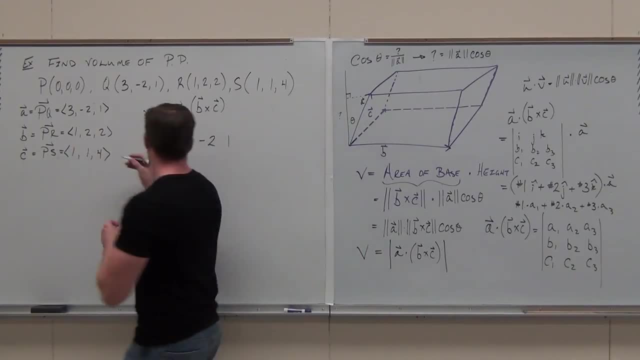 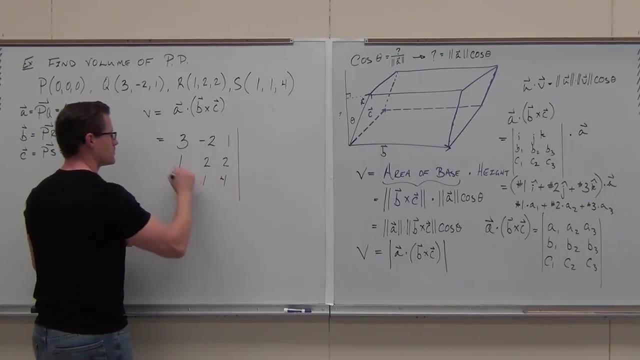 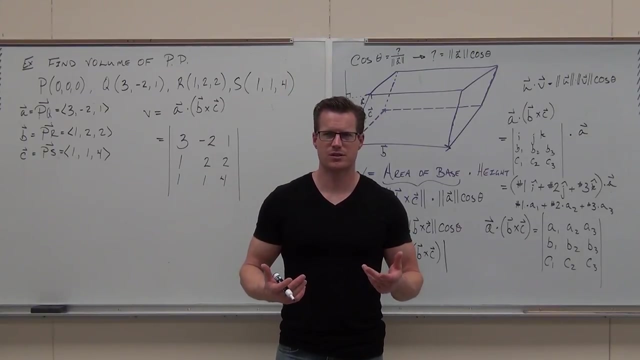 Okay, What's the vector B, What's the vector C? And find the determinant of that thing That saves you the dot product. If you're seeing where those numbers are coming from, I really do need to know. Are you guys for real okay on it? 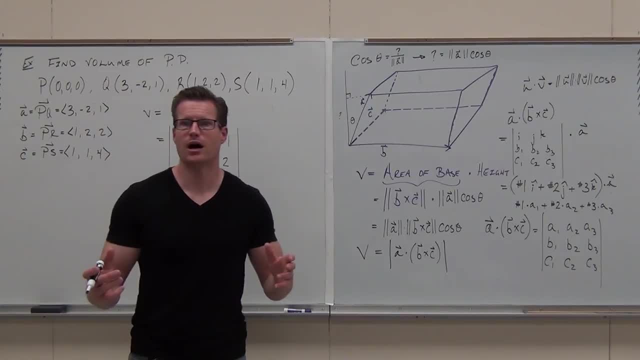 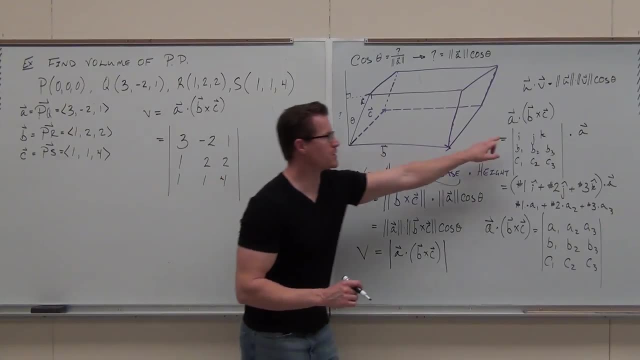 Now how you do it. don't let it confuse you. Where's the I, Where's the J? Where's the? You're not getting the vector anymore, are you? You're getting a number, So just replace what you would normally do with the I, J and K. 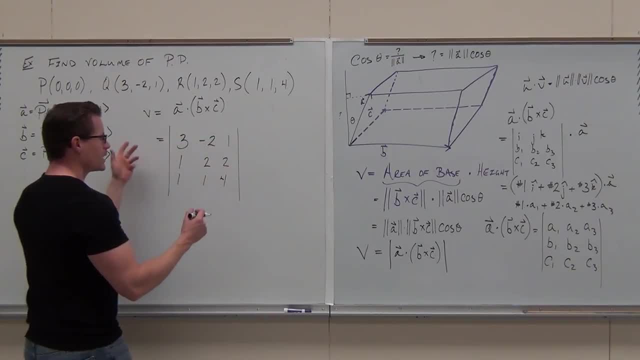 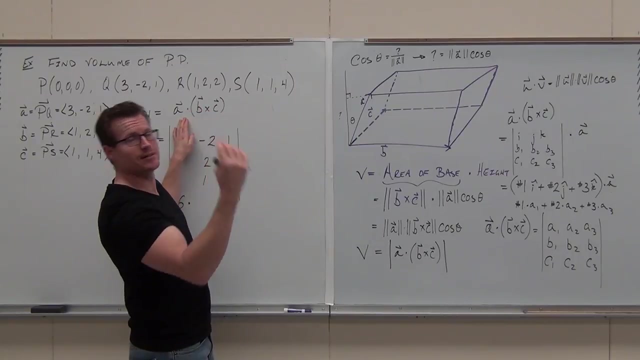 with these numbers right here: the 3,, the negative 2, and the 1.. So we go: okay, well then this would be covered up. We have 8 minus 2, which is what Times normally it would be: I, I, Nothing to survive. 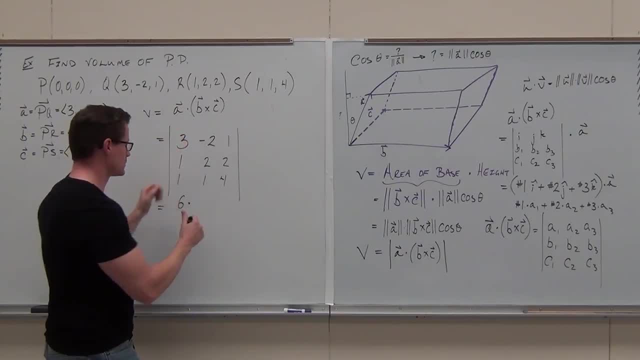 But now, because it's not I, it's 1,, 2, 3, hey, that's it. What's the next sign that we put Minus Cover that one up. I've got 4 minus 2.. 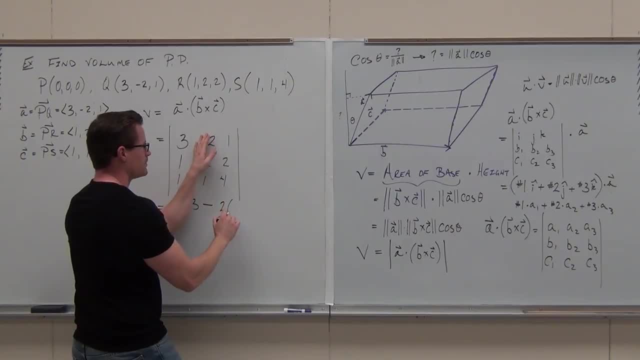 How much is that 2.? But then I'm going to be multiplying by 2.. Be careful on the sign: Multiply by negative 2.. I've got 1 minus 2. That's negative 1. And I'm multiplying by 1.. 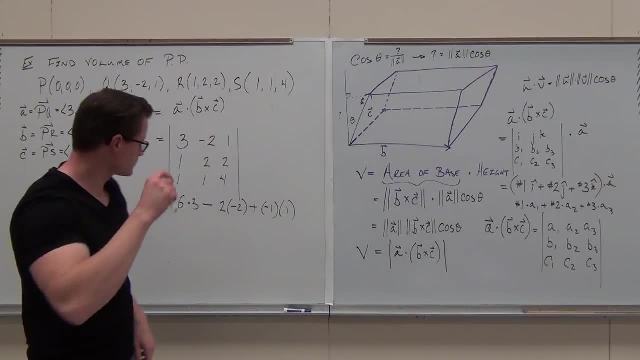 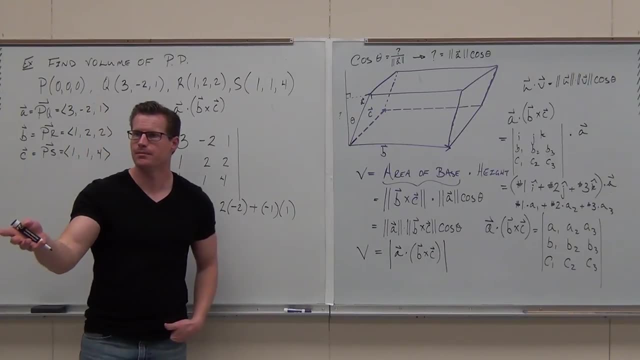 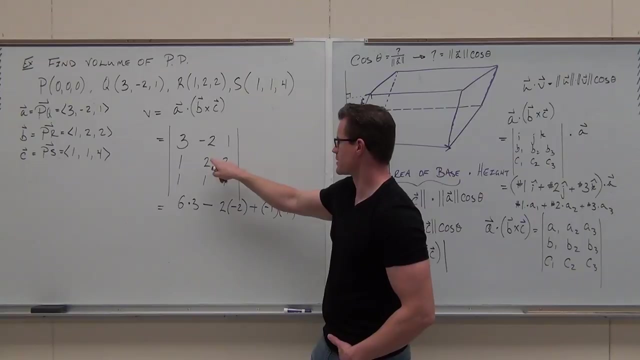 1.. Can you do that? Can you guys do that? Are you going to see where the numbers come from? Do you see how we do determinant 3?? Determinant negative: 2. Make sure the minus is there. Then determinant times 1.. 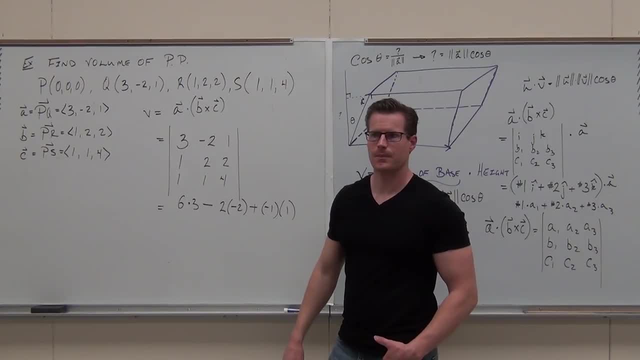 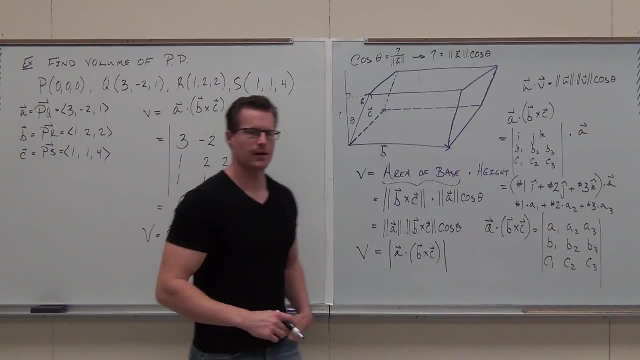 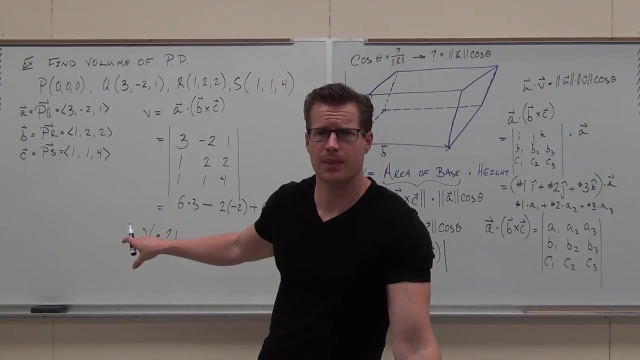 21. 21. 21. 21. 21. 21. 21.. I'm going to ask you, maybe a loaded question: Is this easy, medium or hard for you? The actual doing it? It's not bad. 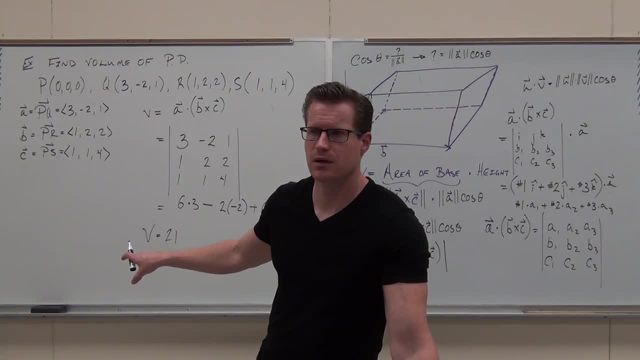 It's medium, Is it okay? Can you do it? Yeah, The understanding of this stuff, man, I've got to be honest. There's a lot that we have done in this class to get to this point. This formula is not that bad. 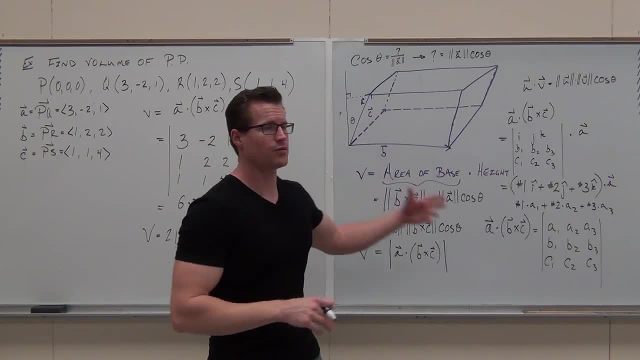 I mean, it's the determinant, But we have covered an awful lot of stuff. I'm going to talk about just a couple of those things right now and then we're going to take our break. okay, The things you need to add. 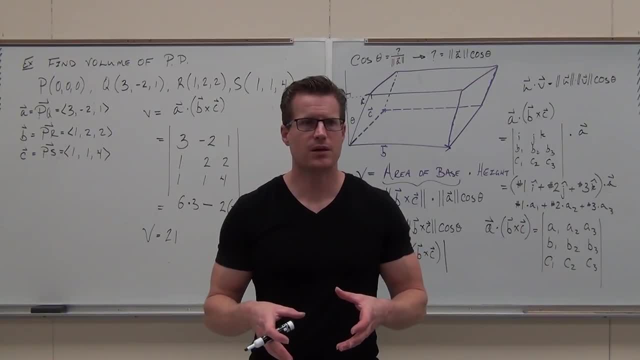 The things you absolutely know in this class at this point are this: You need to know how to find a dot product. You need to know how to find a cross product. You need to know how to find the angle between two vectors, how to find the position vector of practically anything. 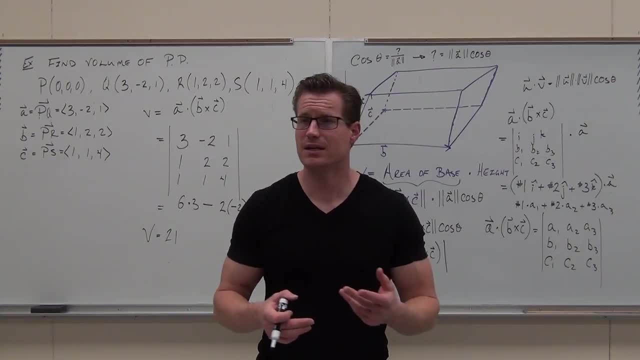 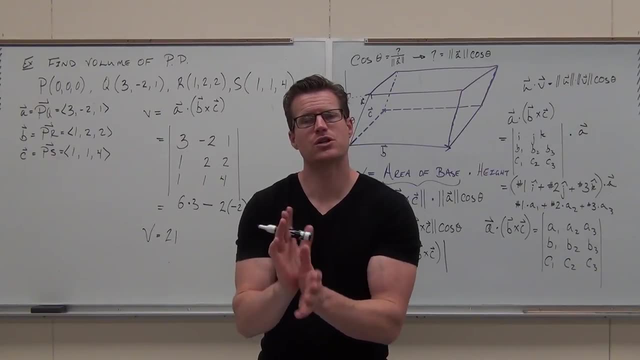 You also need to know how to do some application stuff. If I give you two vectors, you should be able to find the area of the triangle that those things create. If I give you any three vectors, you should be able to find the volume. 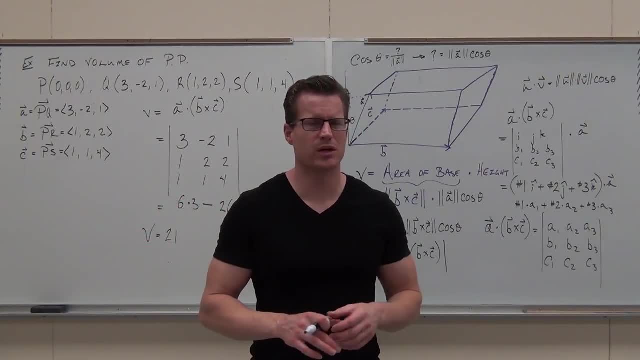 of the parallelepiped that those things create. That's where you should be at this point. Do you feel like you're? You're there And the unit vector? Goodness, you got to find a unit vector. Can you do that? 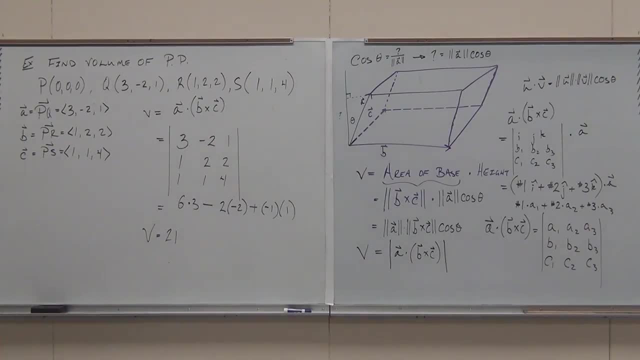 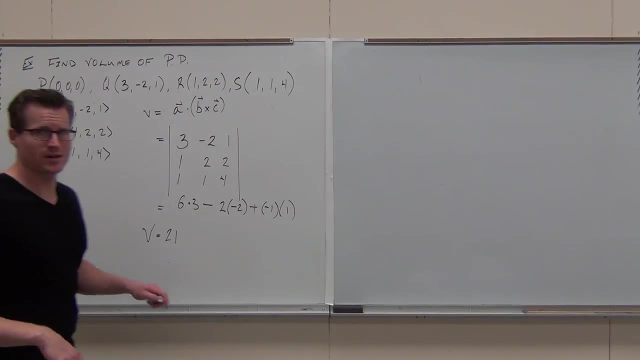 Okay, We're going to take a pause and then we'll come back and do a couple of things. All right, I told you during the break I was going to ask you a question. I want to hear you think. There you go. 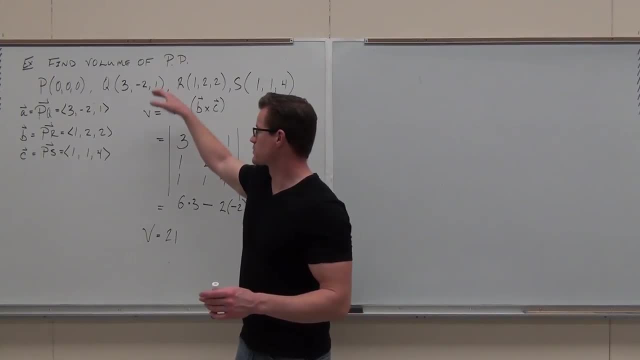 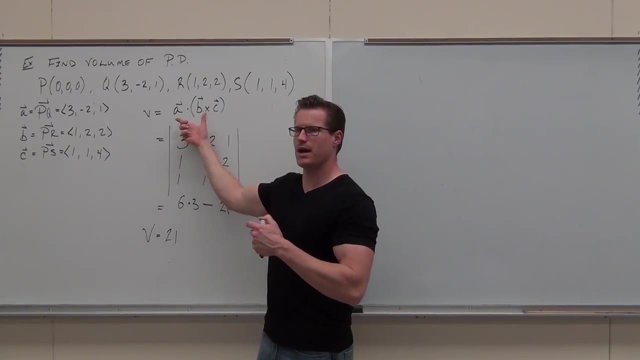 There's a question: What happens if you do all of this work? By the way, do you guys like this Instead of doing cross product and a dot? It's pretty nice. It works only in this situation, though. So if you have a dot on a cross, 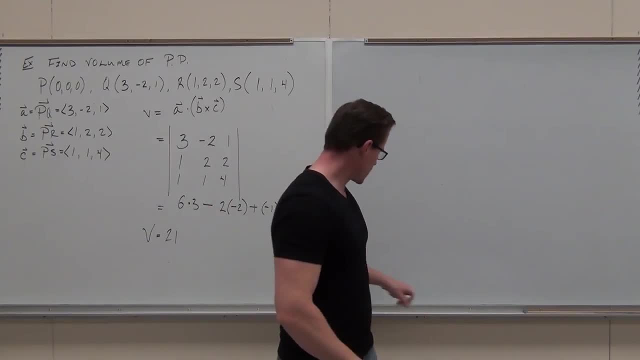 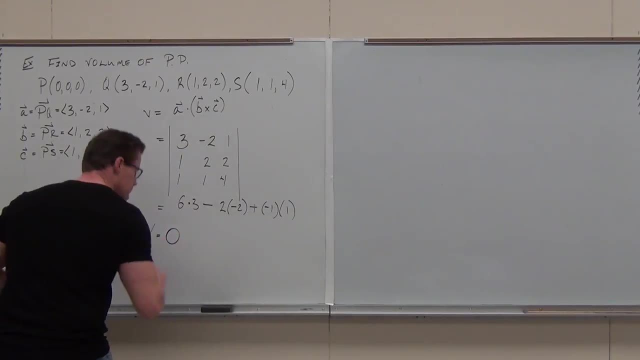 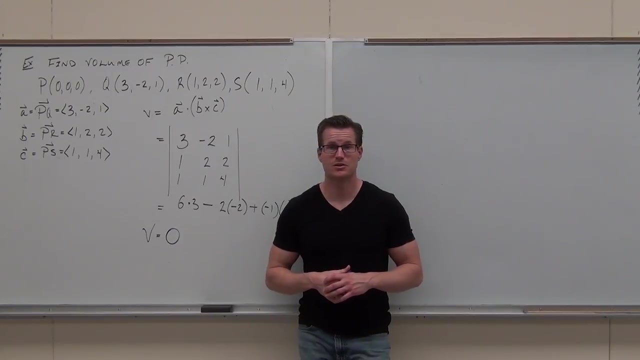 Do that. But what happens if you do all this stuff and you get down to the very end and you get goose egg? What does that mean? You did do something wrong, You did something okay and you're sure you're right. 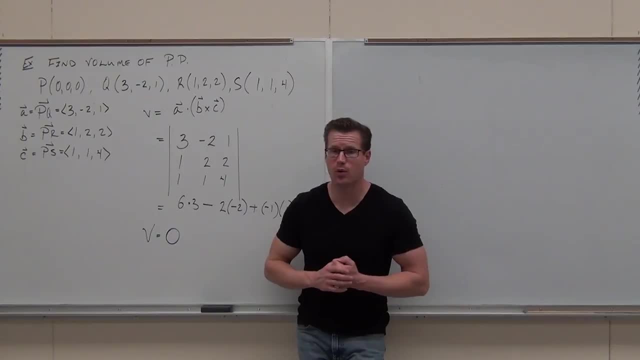 Double check, triple check, and you had your four points that were given and you got zero. Can a parallelepiped have a volume of zero? Yeah, What would it just be How. It would be a plane. It would be a plane. 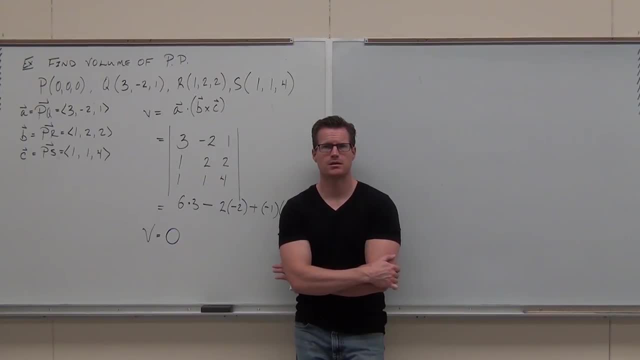 Which means that its height would be zero. Okay, Which means what? If you have four points? If you have four points And you do this thing, where you make this, you know and you get: the volume is zero, which means the height is zero. 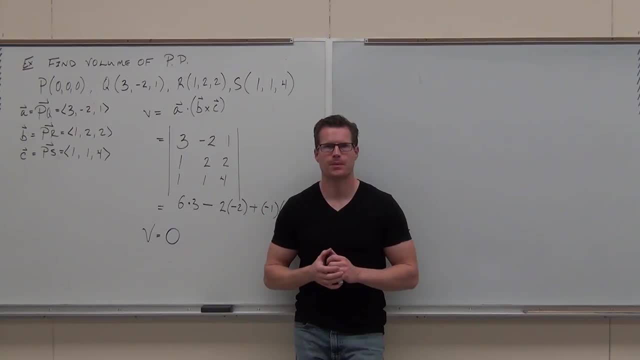 What's it tell you about those four points? They can't be equal. okay, They're obviously different points. They're: If you have a volume of zero, it means that you have no height, which means that that point, that's not. 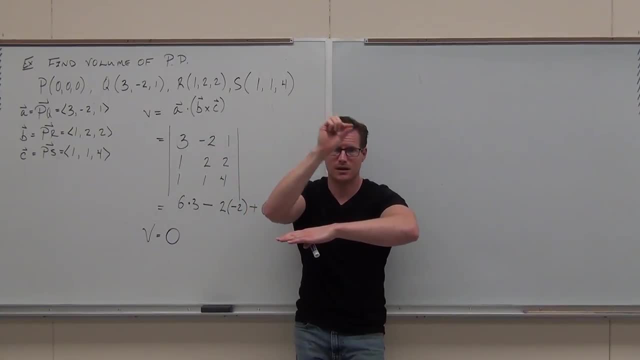 in the other three-point plane. The fourth point plane is in that plane. If your height is zero, it means the fourth point is in the same plane as the other three points. Isn't that kind of cool. It means you have something that's co-planar. 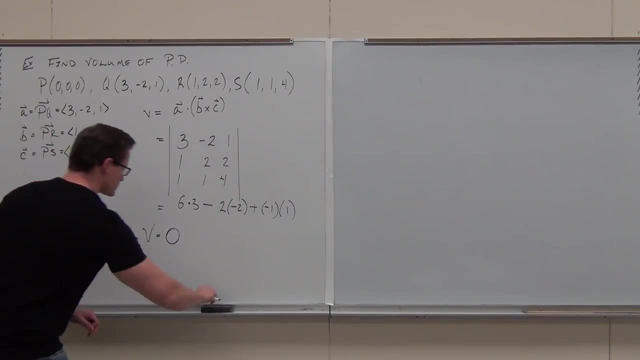 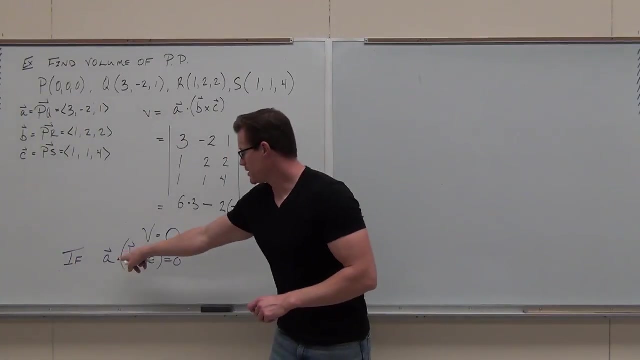 So, if you ever have the situation, If you ever have this situation, if you ever have this situation where you have cross product, dot product and it equals zero, here's what it tells you. It tells you that these three vectors- 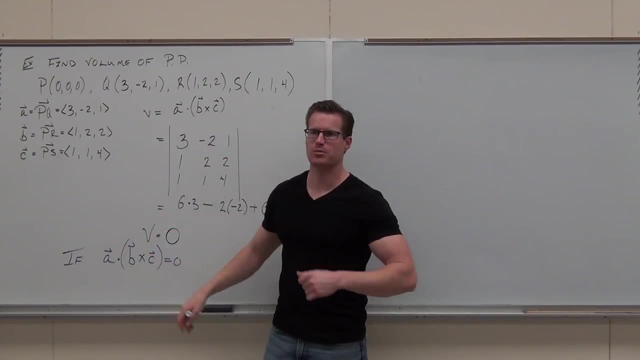 obviously they have the points right. They have all those. these three vectors are co-planar. These vectors are, or all four points. either way, these are co-planar. In fact, that's how you test whether vectors are co-planar. 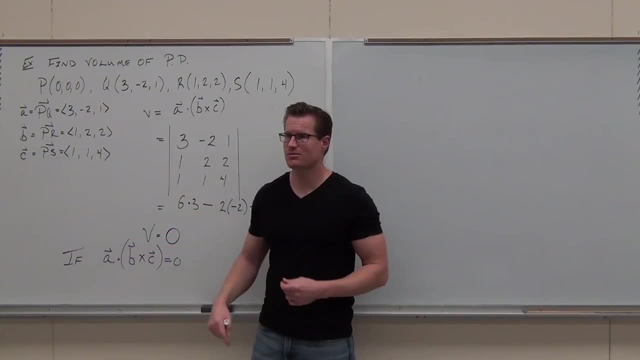 You try to find the volume, guys. If you try to find the volume at zero, it tells you they're co-planar. If you try to find the volume that's not zero, it tells you they're not co-planar. And then you automatically get the volume for free. 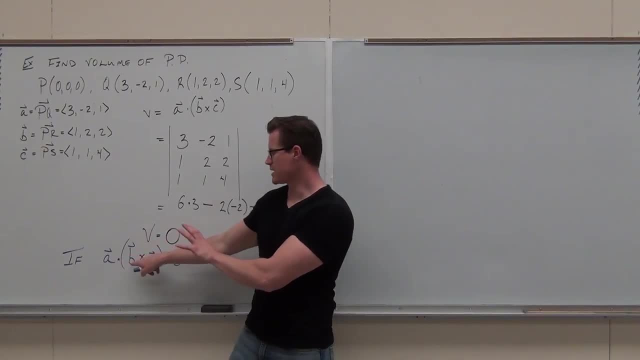 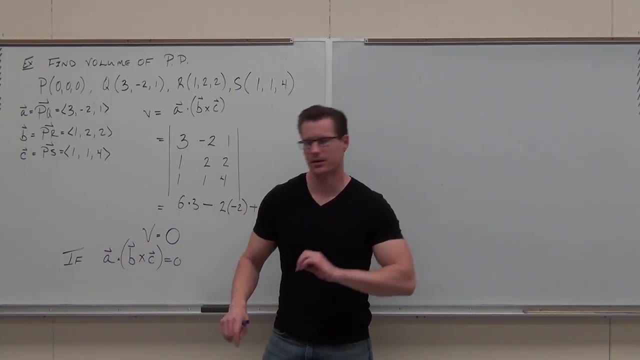 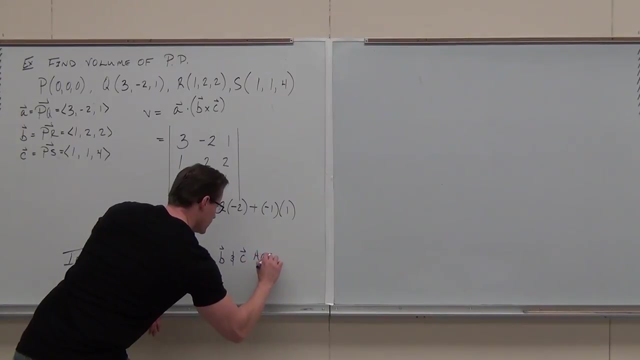 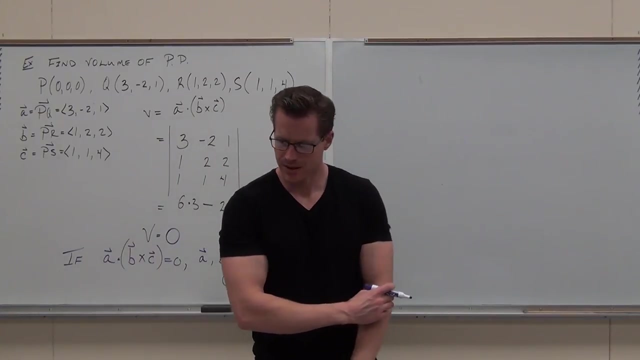 Does that make sense to you? So this is how you test whether these three vectors are co-planar or not. If this happens, A, B and C as vectors are co-planar in the same way. It's kind of neat. 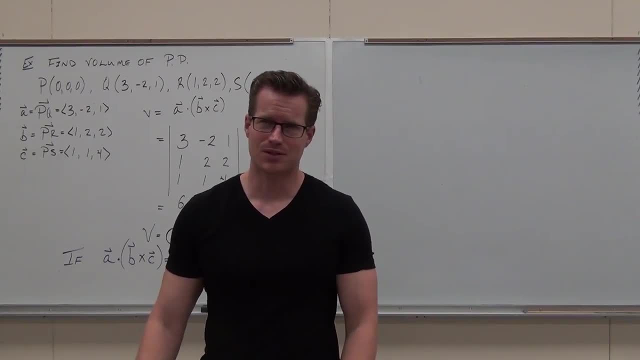 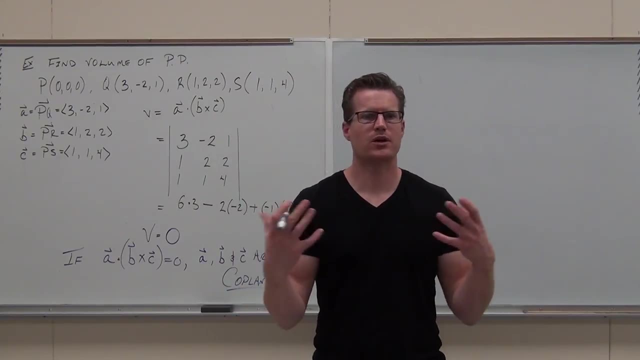 Kind of neat. Now we're going to go back a little bit. I'm going to prove that. one thing I said I was hopefully going to forget about and I didn't, So you're welcome for that one. We're going to prove that when you do a cross product, 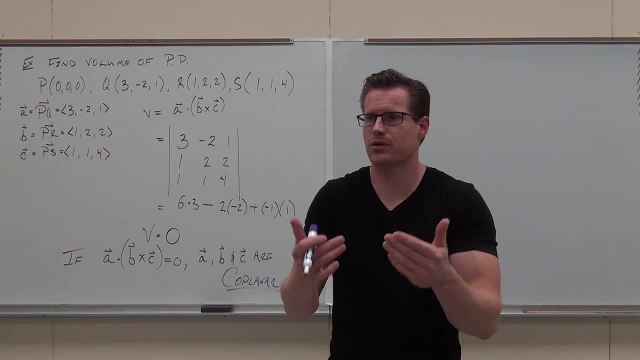 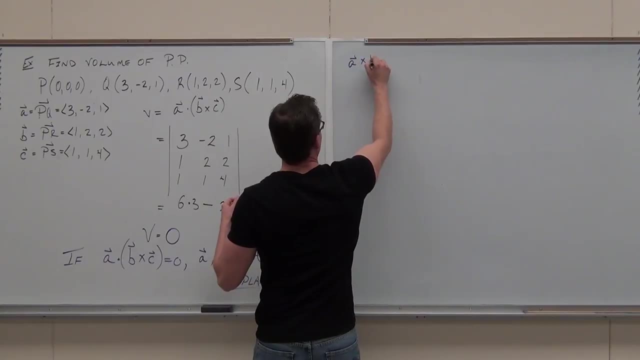 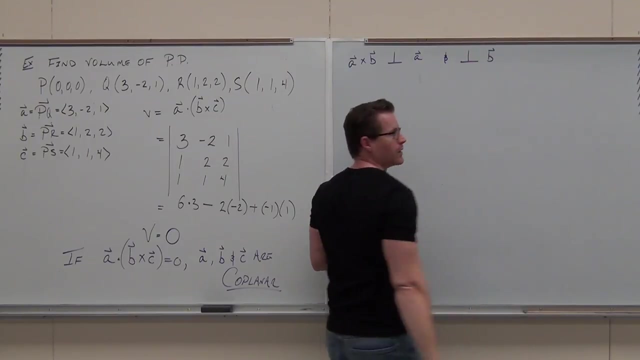 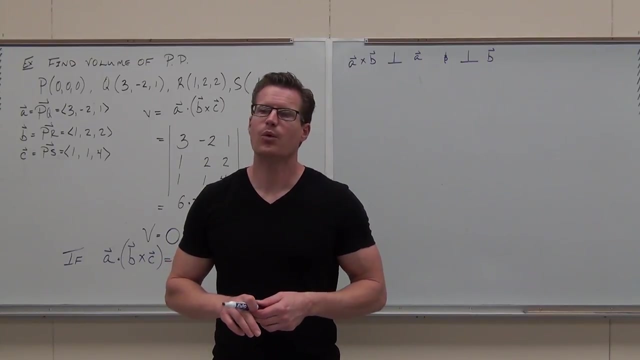 what you get is actually mutually orthogonal. We're going to talk about that. So here's what I've told you. What I've told you is that A cross B is perpendicular to A and it's perpendicular to B. What we're going to do right now. 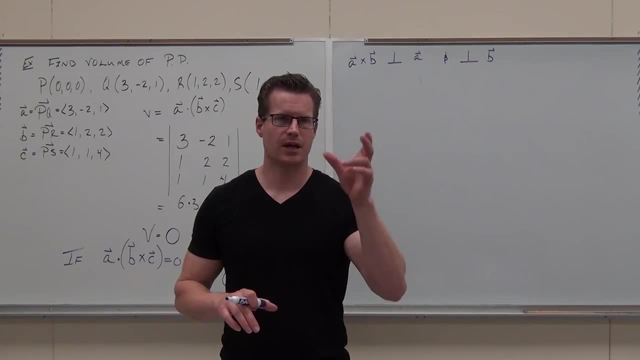 I'm only going to prove one case of this. I'm going to prove that A cross B is perpendicular to A, and you can use the same method to show B, And then you can do B cross A with A, B cross B with B. 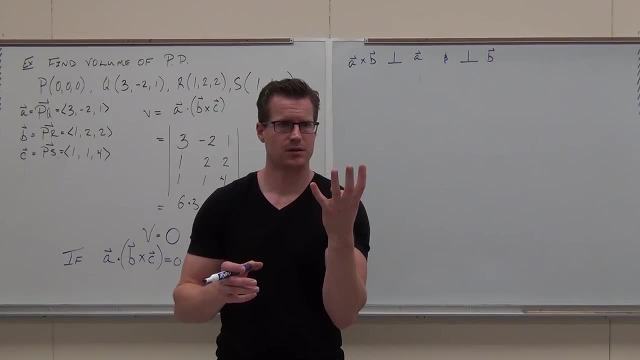 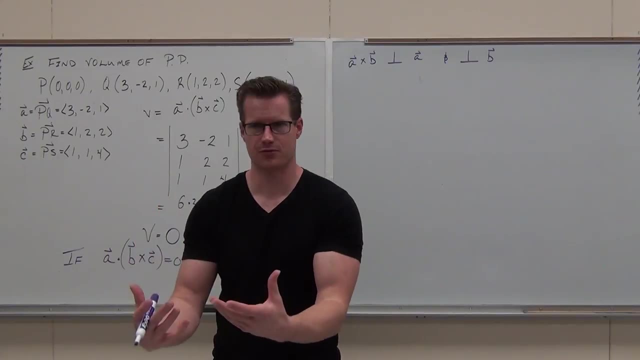 It's a four-case scenario. Does that make sense to you? Are you guys alive? Yeah, So we're going to do just one case and you can extrapolate from there. So let's start proving that this is perpendicular to this. 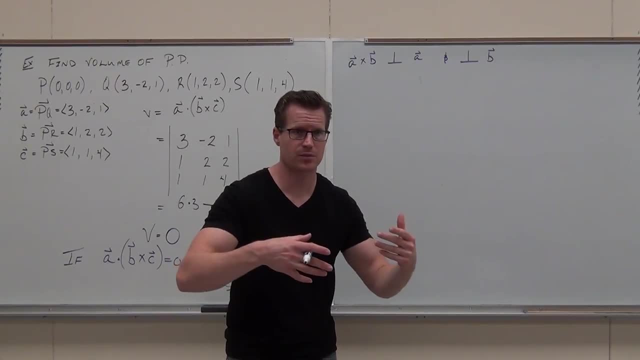 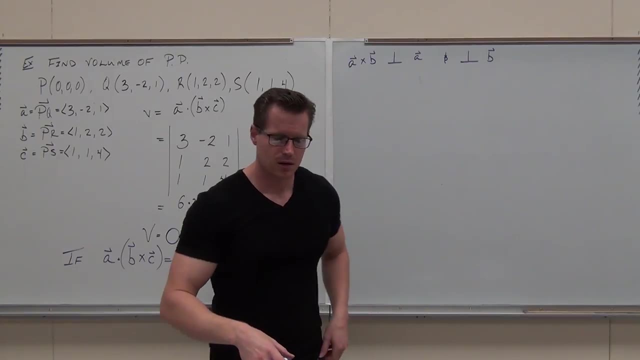 Here's what we know. So, by the way, if you're looking for the proof of cross product does mean orthogonal. this is it. Okay, this is the proof I was talking about. Let's start with this. We talked about it. 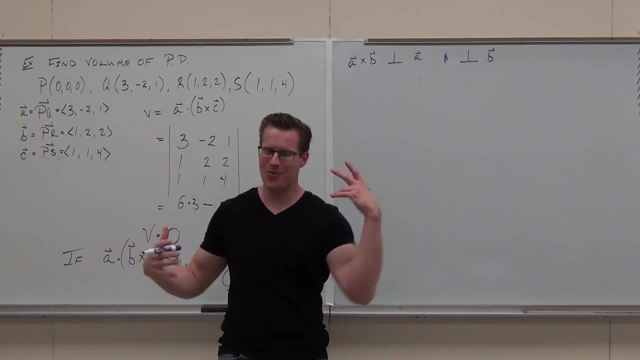 I should know it's going to be there. when I ask you, You're going to yell it at me. I'm going to scream for joy. I'm going to be like whoo. How do you check whether two vectors are orthogonal? 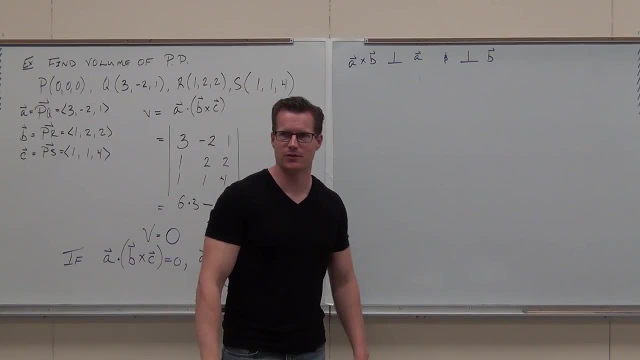 Dot product, Dot product. Whoo, I told you scream for joy. That's my joy face, All right. So hey, is that a vector? Yes, Is that a vector? Yes, If they are orthogonal. if they're orthogonal. 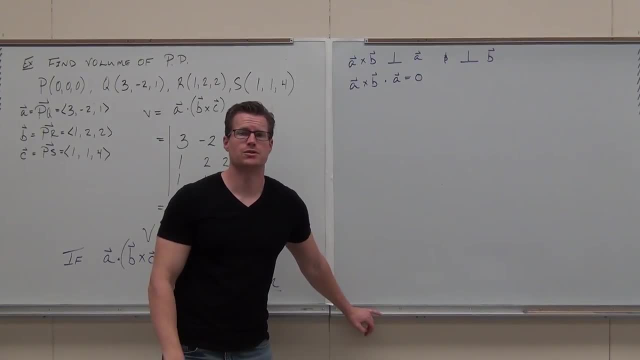 then that has to be the case. That's got to be true. I just thought of a new way to prove this. Can we try it? Oh, this is going to be fun. This is going to be super fun. I'm so glad we did it after this, because I just thought of it. 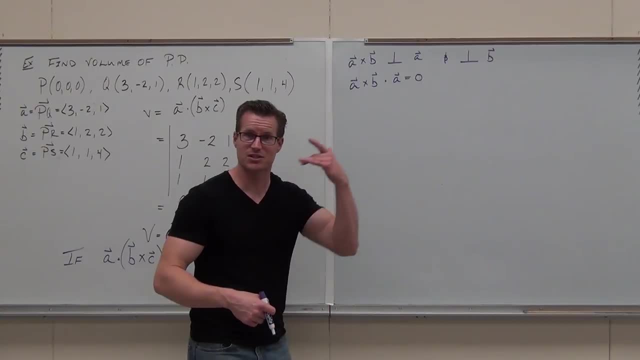 right now for real, like for real. I'm not even lying- I usually lie about stuff like that, But I seriously just thought of it right now. Yeah, we're saying this is going to be awesome, That's got to work right. 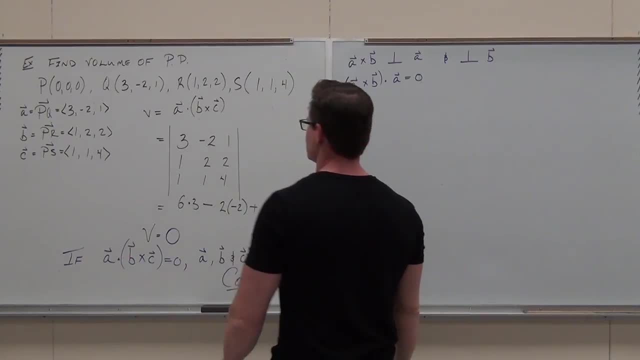 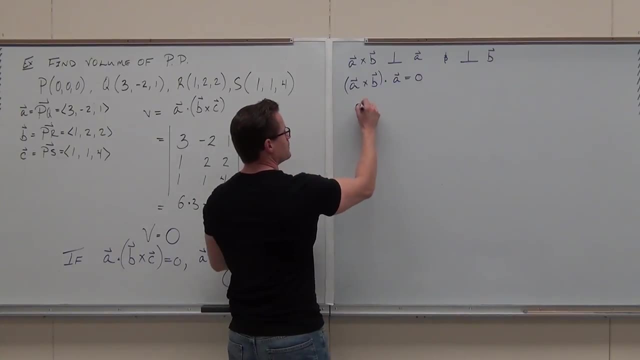 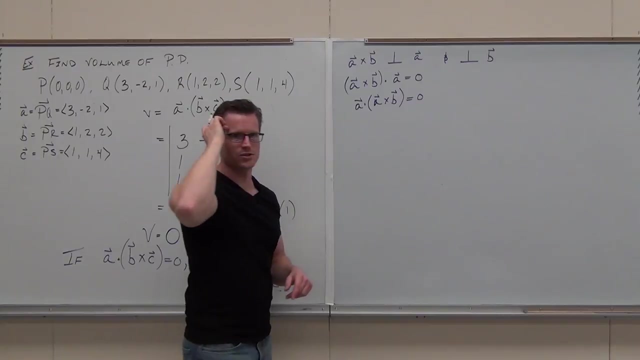 It looks a whole lot like what we did, doesn't it Like a whole lot. I'm just going to reverse them. I'm going unscripted right now to see if it works. I hope it works, If not, I'll just edit it, you know, as an impressor. 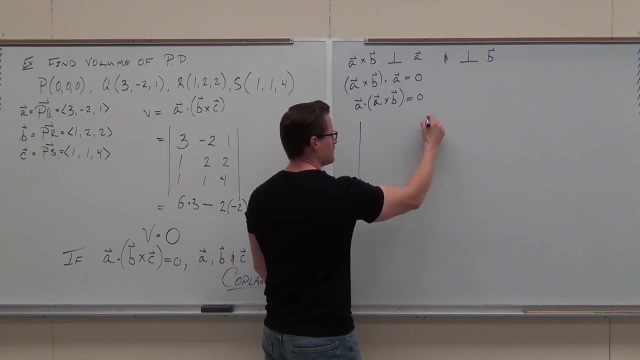 Press the button. I need an editor to freaking work. That's what I needed to do, Stupid editor. Anyhow, let's put it up here. What would go on the top row Would I have I's J's and K's? 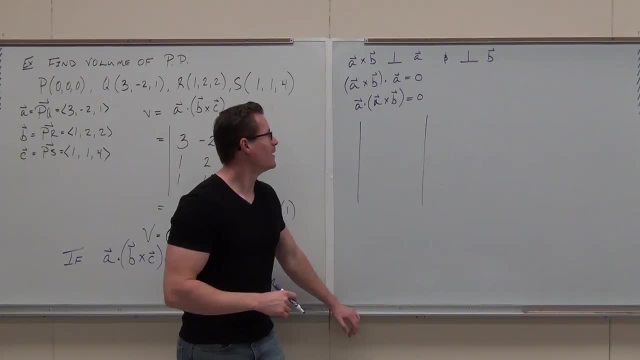 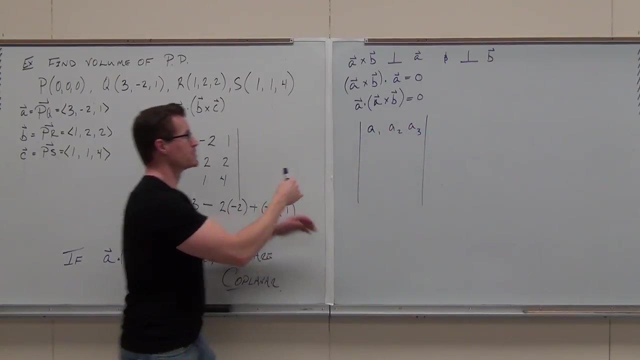 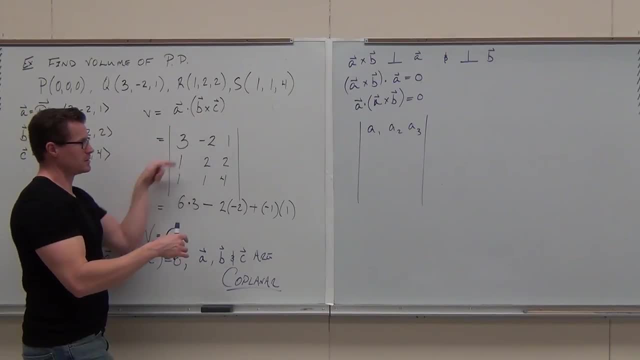 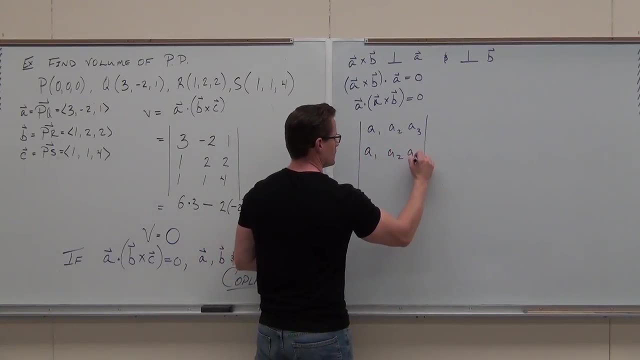 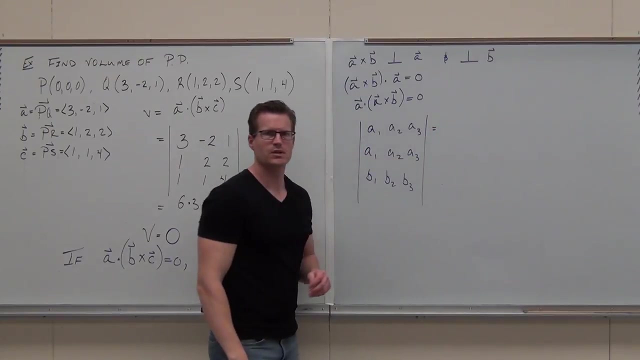 We're saying A B C. Here's A B C. Now we're going A B C, Now we're going A A B. You guys OK with it. Same thing, because they're the same two vectors. 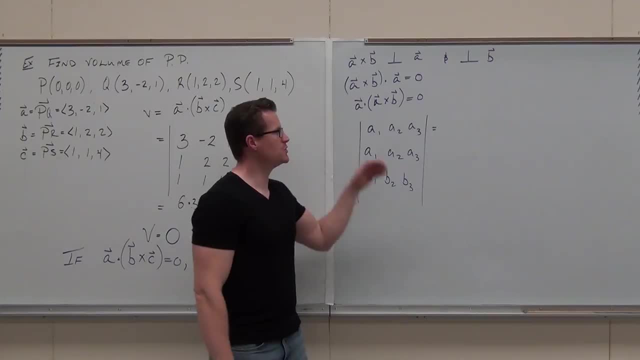 And then B is the only odd node out. follow what i'm talking about. why don't you guys see if you can work through this, as i'm working through it, and we'll see if we get the same thing. okay, so let's do our cover up. this is our last. 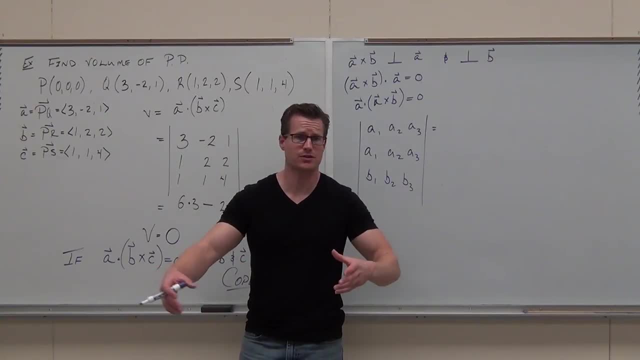 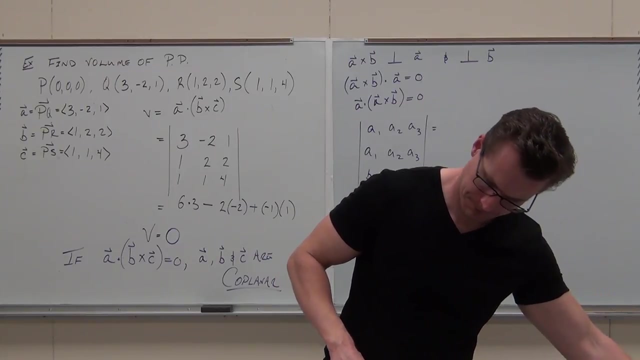 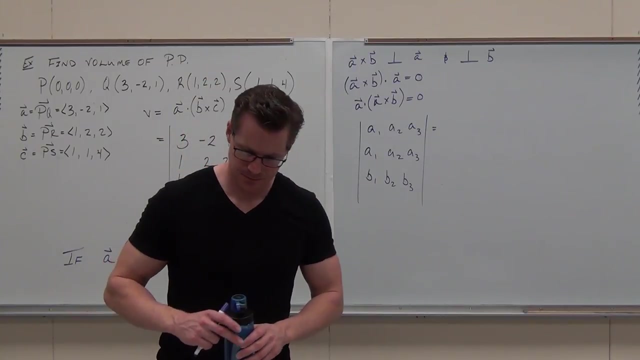 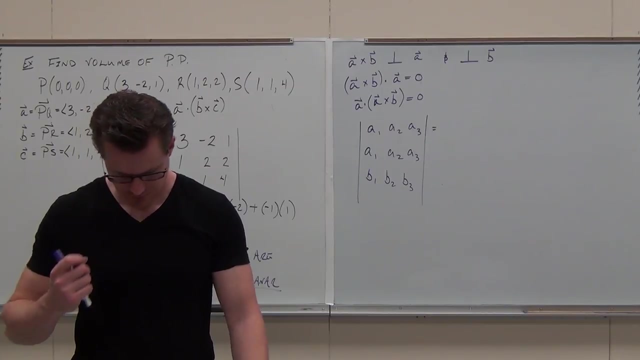 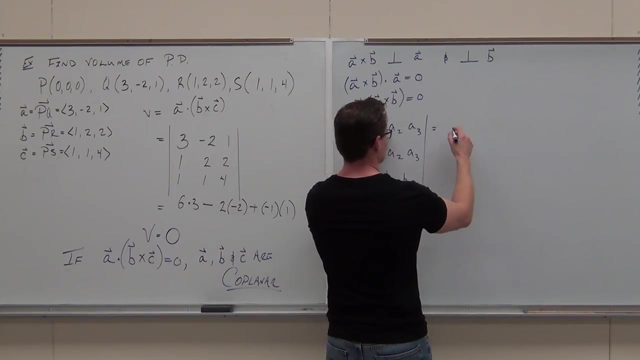 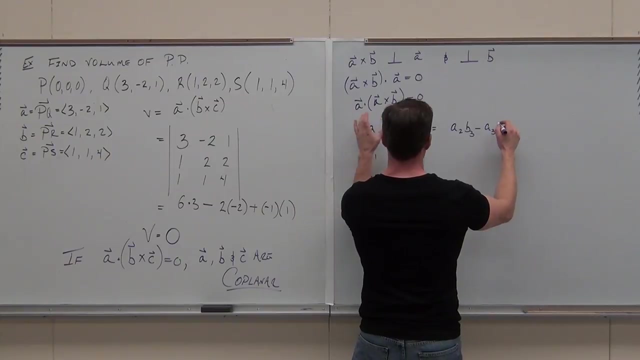 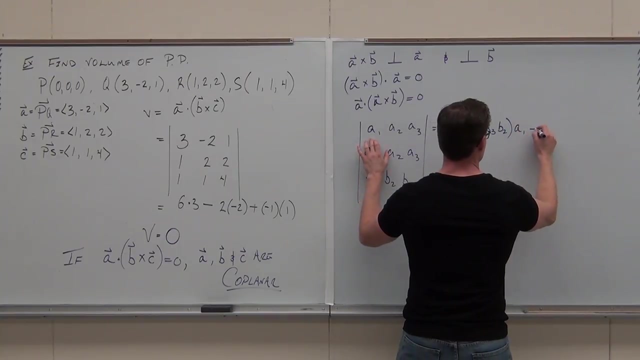 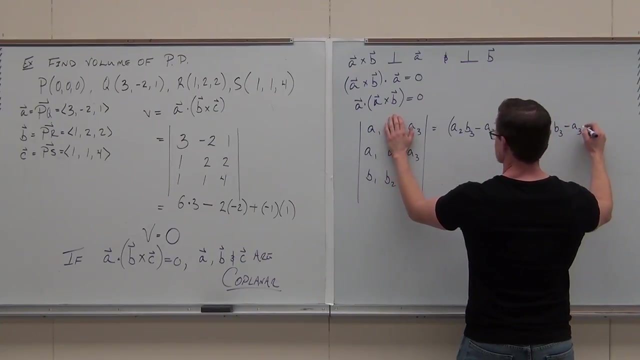 chance to practice the cross product in in this class. really, it is as it applies, just to doing cross product. we'll, of course, use it, but it's our last chance to do the section, so go ahead and practice. so i'm going to double check: got it? 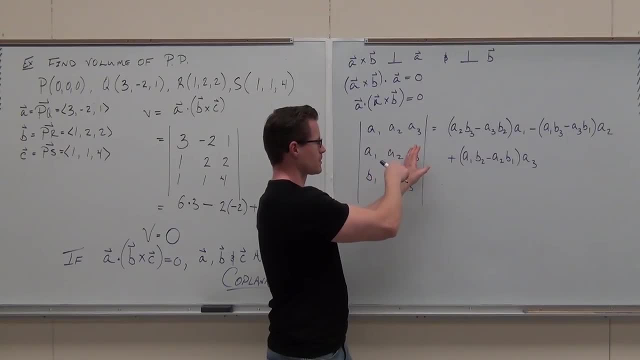 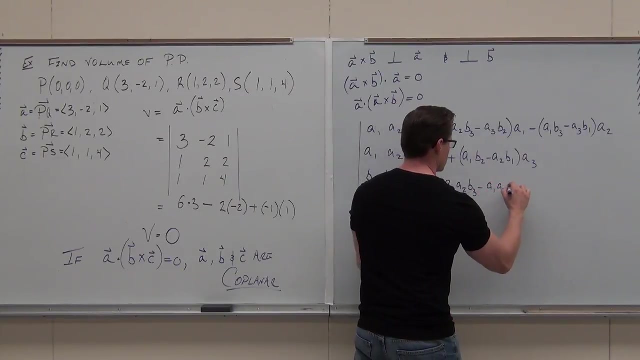 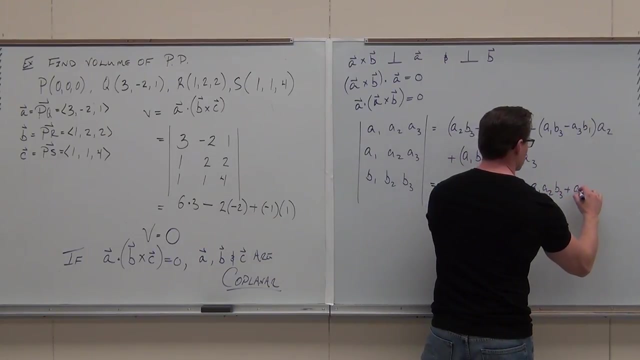 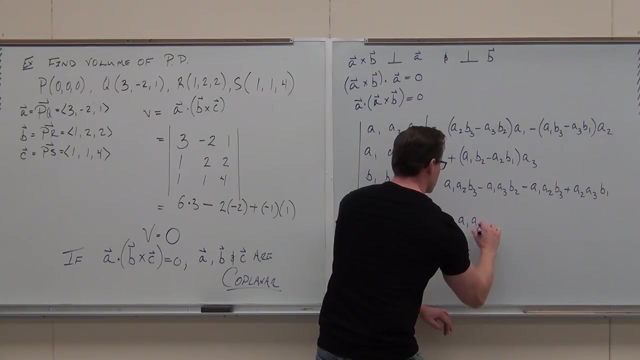 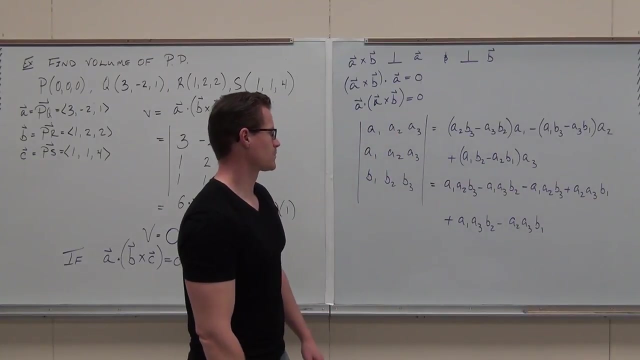 got it, got it. did you get the same thing i got? i want to be all super, super cool, let's distribute this stuff. i want to distribute a1, a2- once you sign, and a3. i want to distribute that. i want to see what happens you. 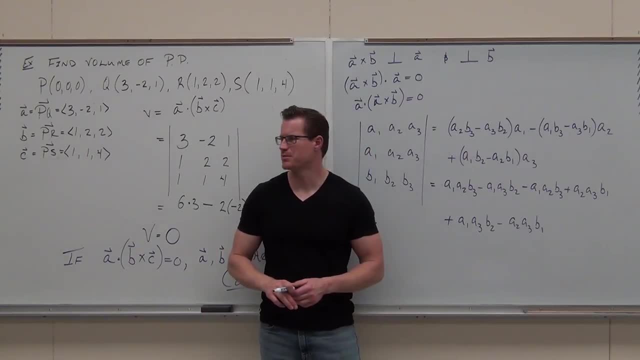 that's what i got when i distributed. you get the same thing that that i got when you distributed. do you see the magic? what happens to all of this stuff? i love that. that's my favorite part of math, by the way. i love crossing stuff out, so i became a math teacher. looks like crossing stuff out. i couldn't really be the terminator. 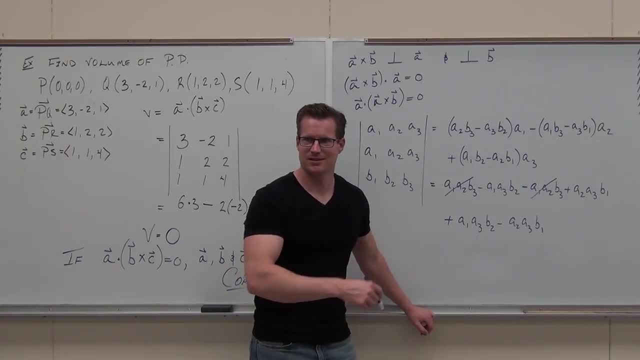 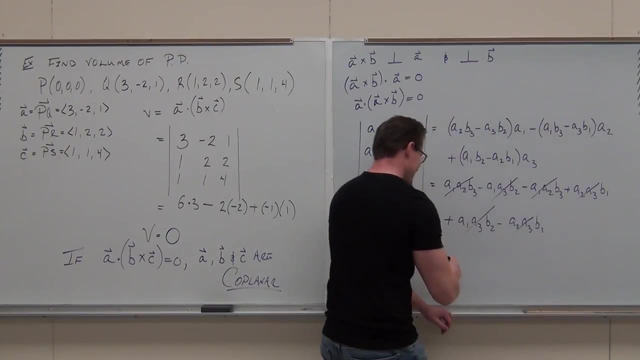 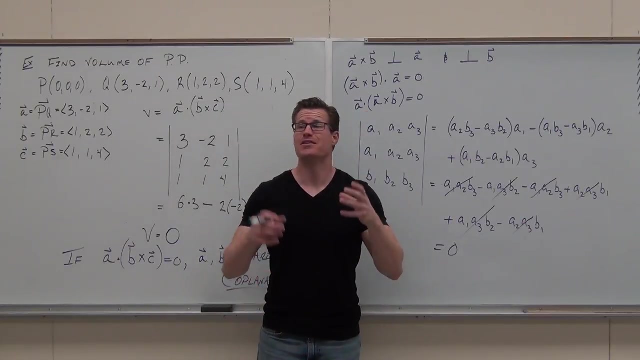 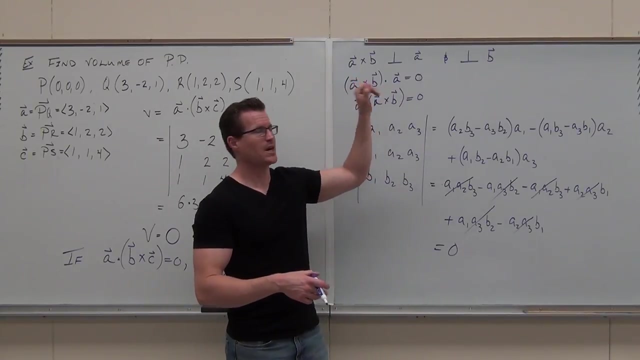 but i could still turn. you know, whatever terminator was, it equal to zero. that's the proof. i just proved that the dot product is zero. if a dot product is zero, then your vectors are perpendicular, they are orthogonal. if you replace this with b, same stuff. if you switch this around, same stuff, replace it with b. 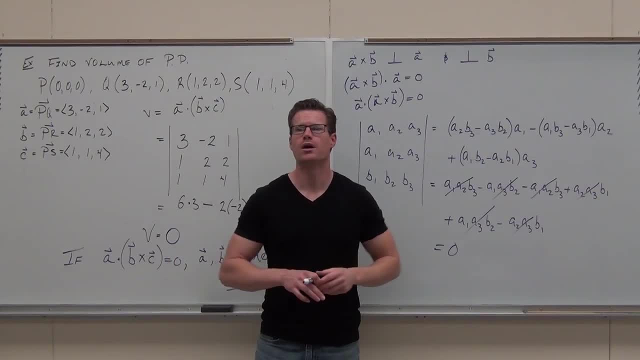 again same stuff. it's always gonna work into zero. and that proves for you that when you're actually the cross product, you are finding a vector that is orthogonal to both a and b, the vectors from whence you where you got that cross product. that that, that's a proof for you. so fans feel okay with. 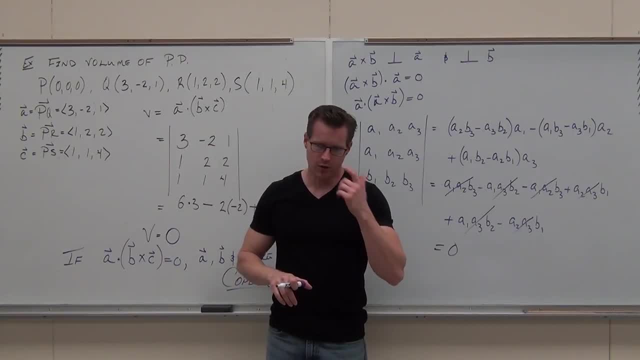 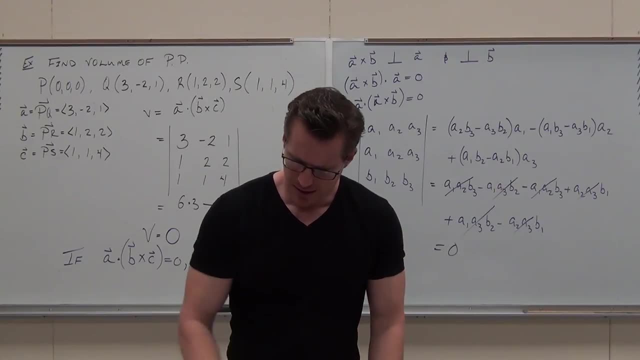 that group one of the easier ones we can do. that's kind of nice. we're going to go one more step. we're going to talk about something really cool, really useful for you physically people. so let's talk about about this thing. you know what we had. 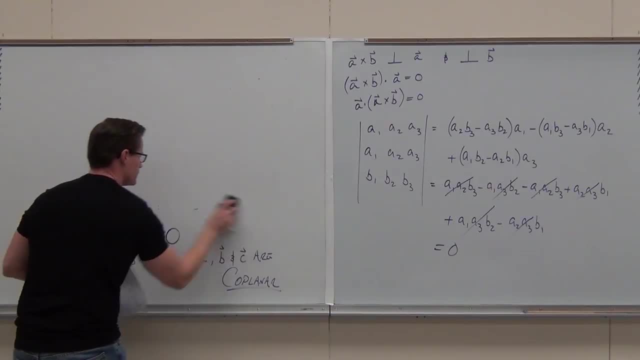 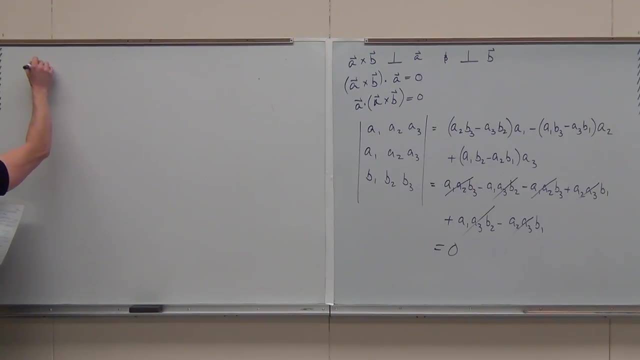 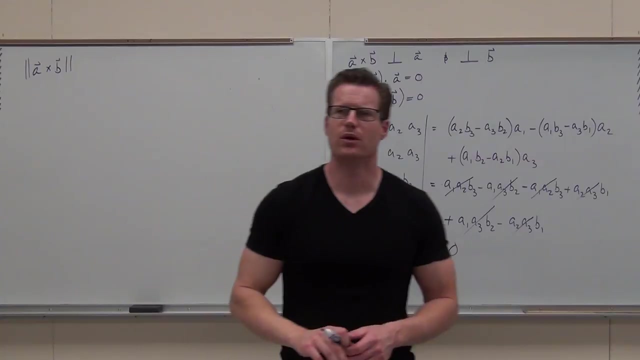 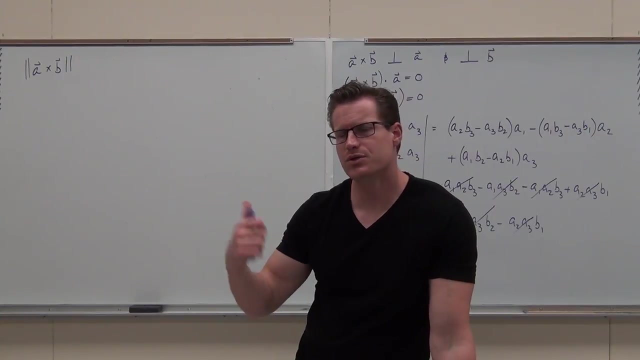 so tell me in your own words how you would describe that to somebody, what i've written on the board. we're at that point. i know you just learned it today, but how would you describe what that represents to somebody who did had no idea what it was? 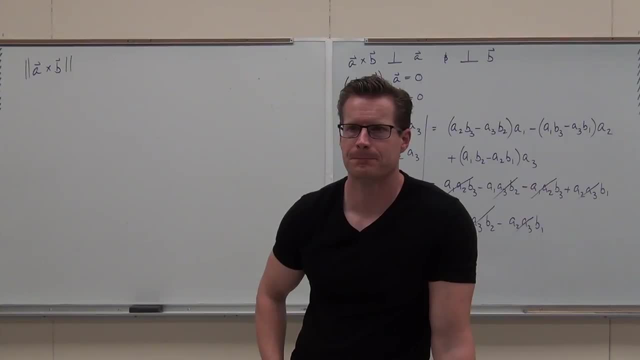 i'm going to wait for you to say something. it's a length of a vector. that's true, because it's a magnitude. what vector? length of a vector? that is what compared to- i just kind of proved it we. it's a length of a vector, that's what two a and n. okay, so if you get a, 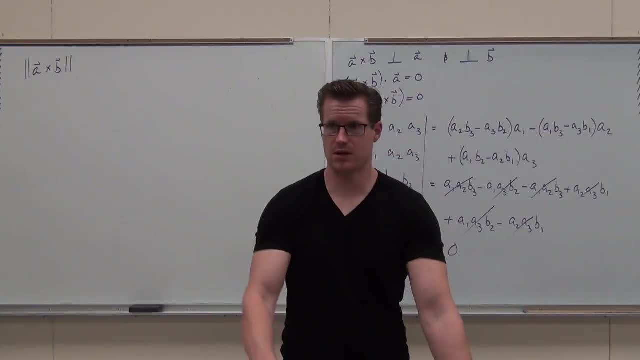 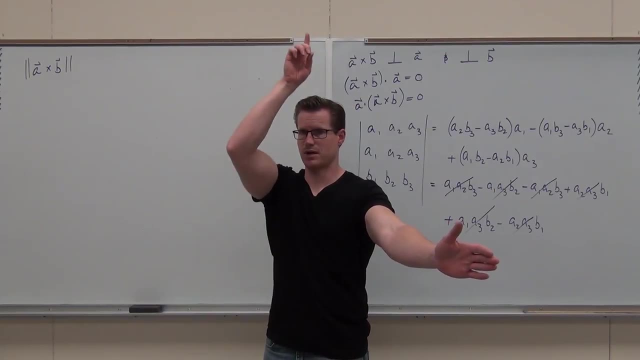 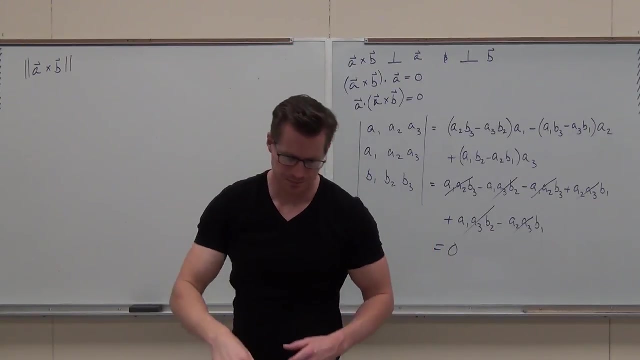 vector length of a and b and you can show it with your hands. could you show it so like? if he's like, hey, here's, here's a and here's b, then a cross, b is this way and it's the length of that vector. that's what's happening. you guys are here with what i'm talking about, if that's true. 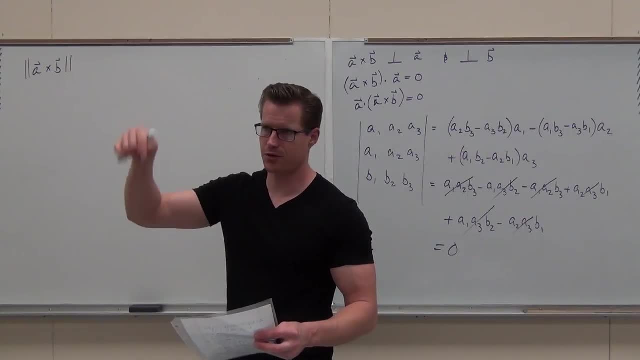 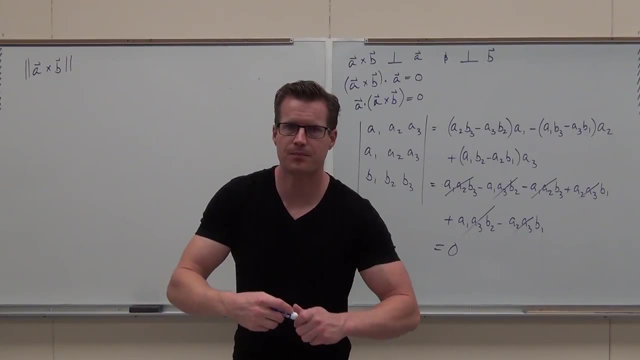 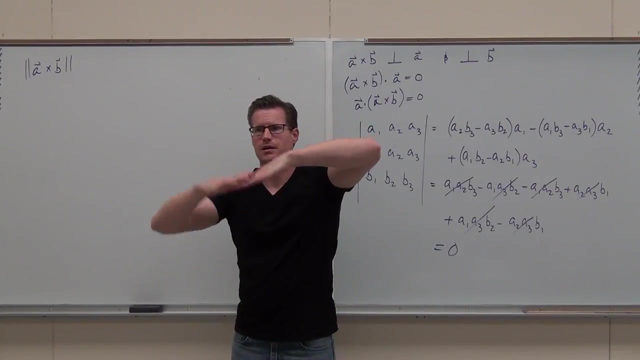 if that's true, if that's the, the magnitude of the vector that's orthogonal to both a and b, then it's just the nice thing to do is to take something and twist it here, yeah, and then you take that to represent torque, because when you have, when you have this lever and you rotate it, what happens to a bolt or? 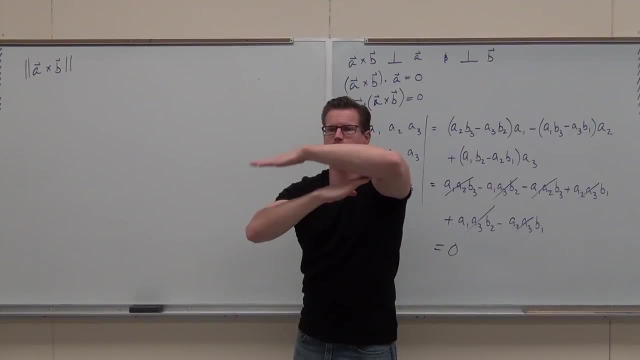 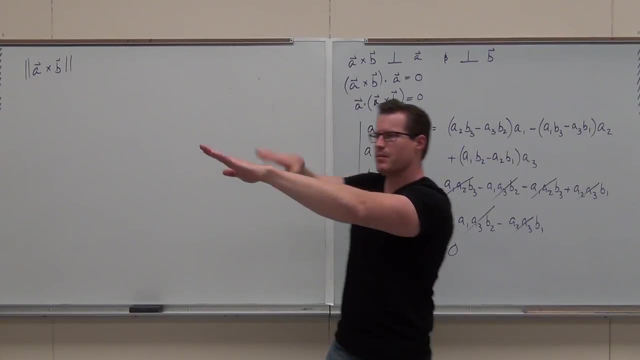 anything that's being twisted, even the right hand rule, guys, when you twist something from here to from here to here- my fifth favorite dance move, what? right behind one of wrex? okay, so anyway, when you- here's my vector, it's closing. this way the torque is going to go clockwise right in. 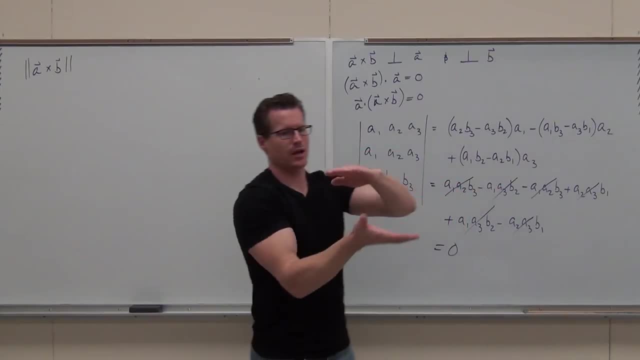 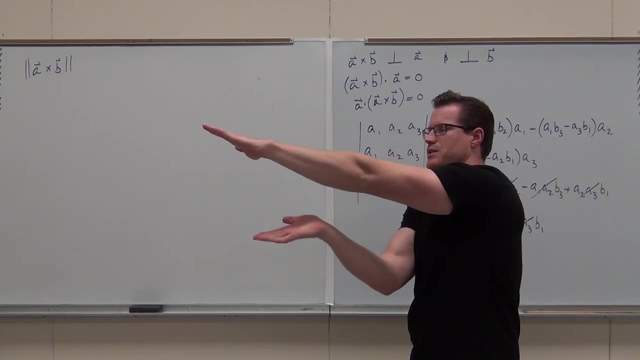 If I do the other way- take it from here to here- untwist it. right-hand rule says I did it wrong. good night, sorry. Right-hand rule says I'm taking this vector and going this way. it's going to twist it this way in. 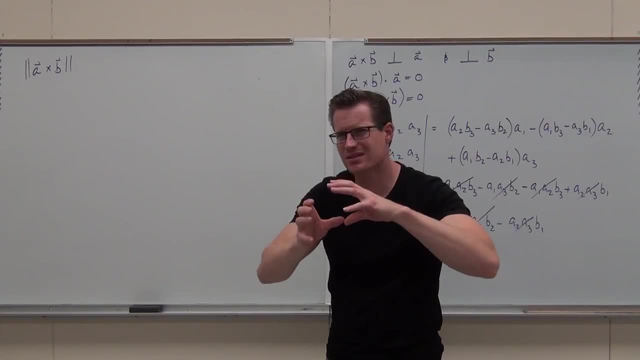 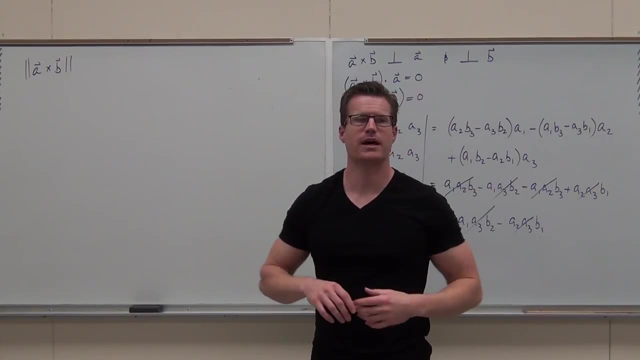 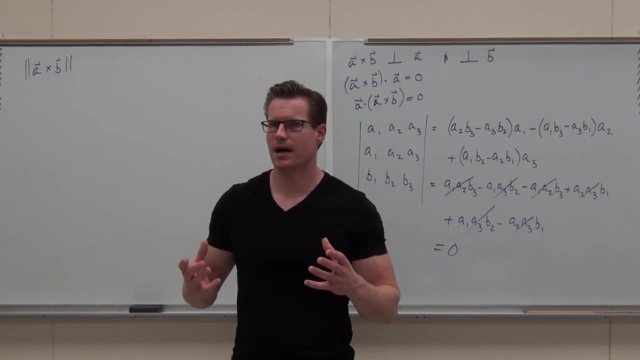 That is torque. So the magnitude of that twist, the magnitude of the vector that's going in, so perpendicular to both A and B, the length of that, is how much torque you actually get. That's how we represent torque. Now, naturally it's kind of nice to represent torque. 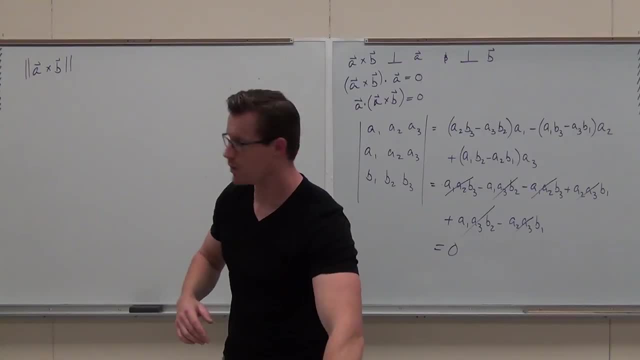 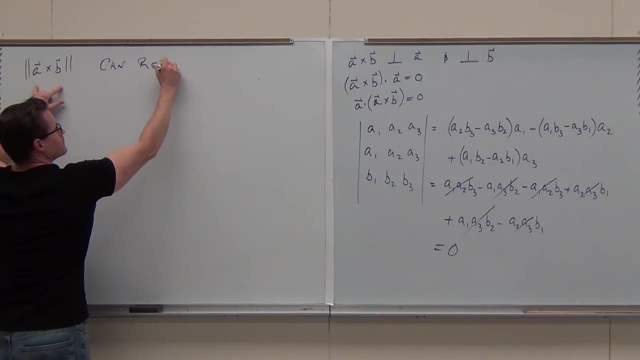 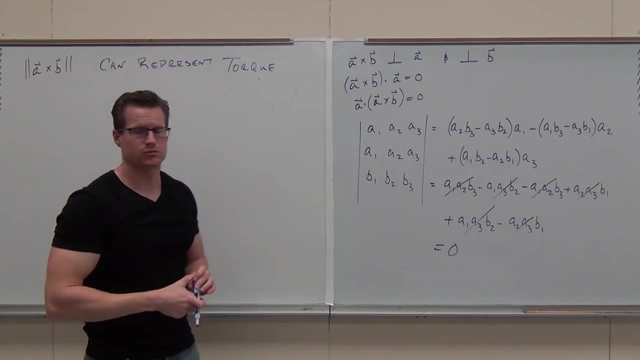 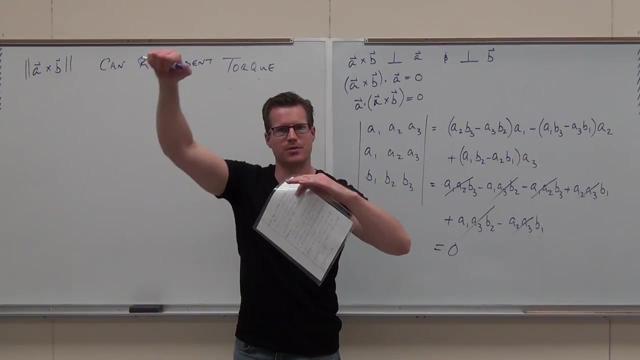 as an angular movement, right? So we're going to choose to say, well, okay, this thing can represent torque true statement, But since we oftentimes rotate around something, we like to do, that right. We like to rotate around a particular bolt. 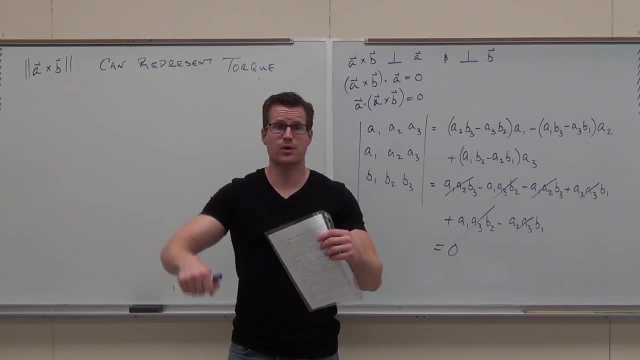 or tighten something down. If you ever torqued your lug nuts on your car, you know that we're rotating and all of a sudden the thing goes click and you go: oh, that's enough, 100 foot-pounds or whatever you're doing. 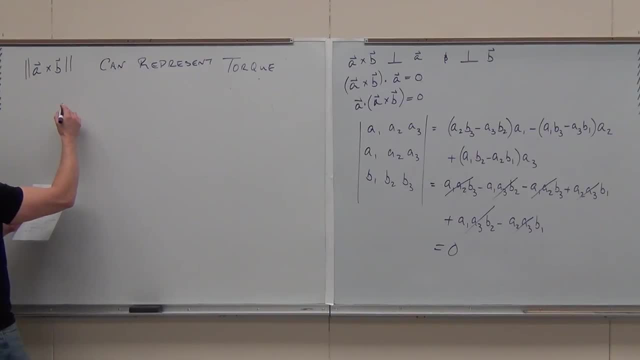 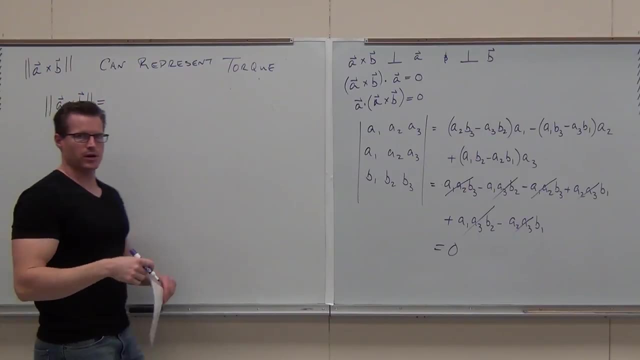 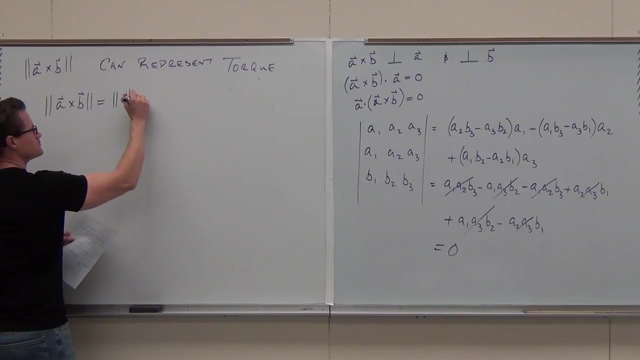 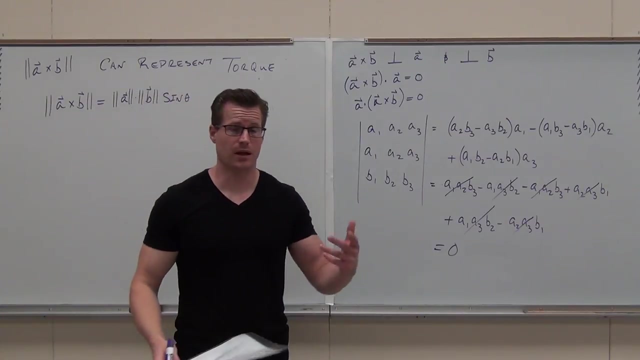 So it can represent torque, but we're going to use this to do it. We're going to say that this, by what I proved in class- another use for it That we proved earlier- spent a lot of time doing it actually. 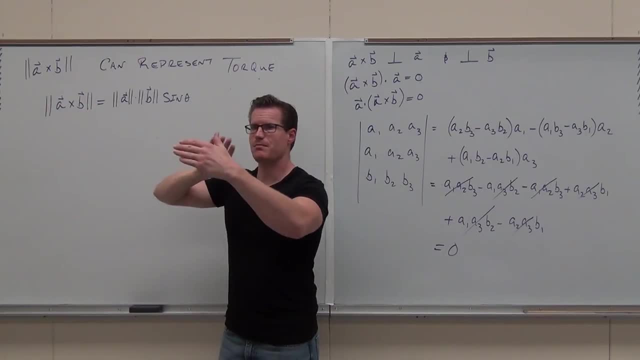 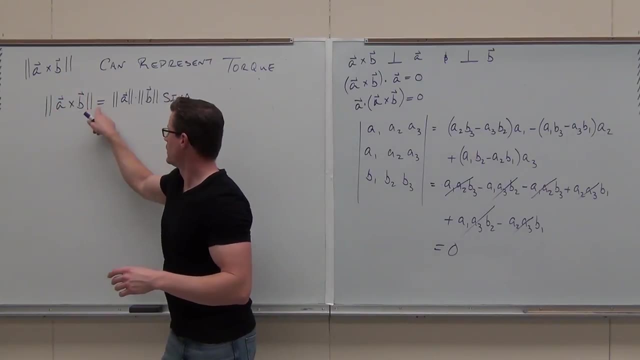 But wait, if this we just said represents the magnitude of that mutually orthogonal vector, we call that torque, if that represents the torque and these are equal, then we can use this to represent the torque as well. So we get this definition for torque that does. 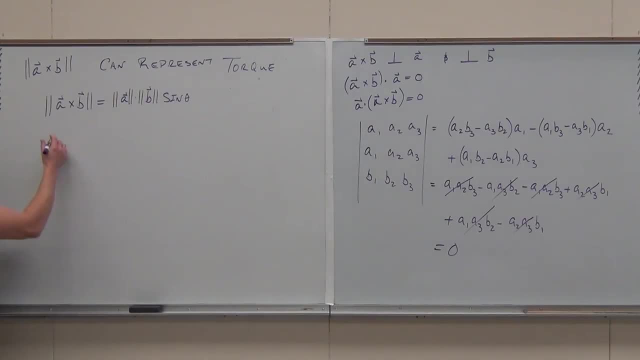 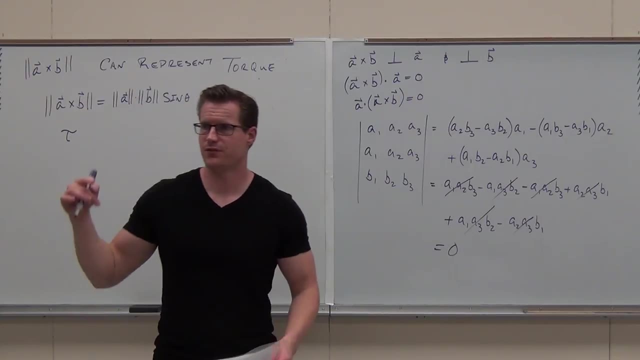 that sort of thing. Now listen, if you've taken physics you might have seen it, but this is where it comes from. It says: if we have torque now, torque can be thought of as a vector also. but we're going to focus. 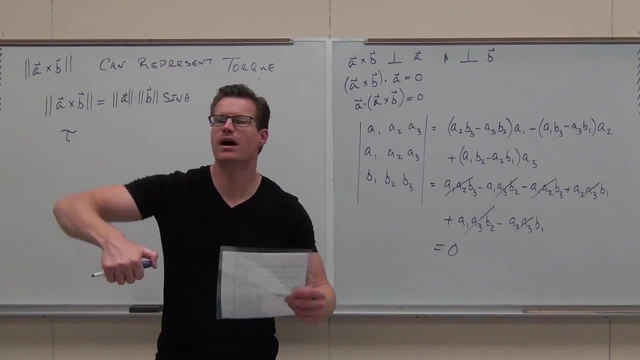 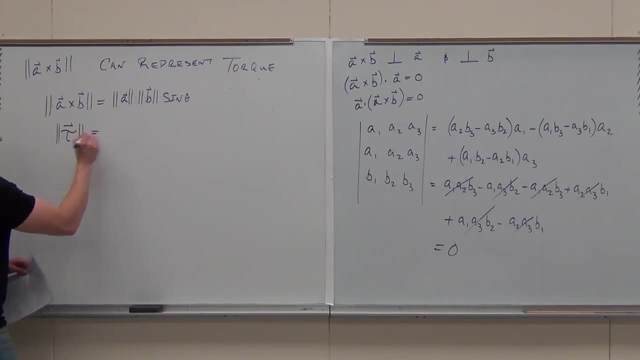 on the magnitude of the torque, what you're actually getting out of it, okay, How much you're torquing that bolt, what you're actually doing. So, when we take that torque vector, okay, well, how can we think about torque? 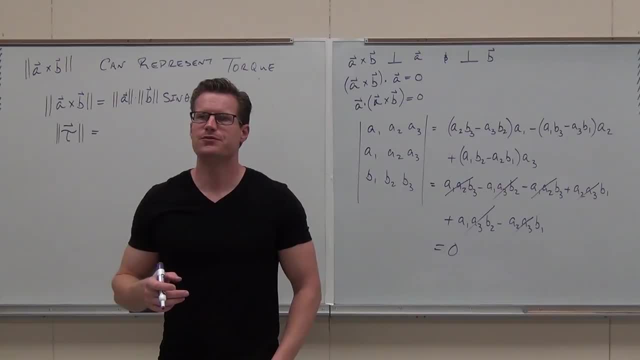 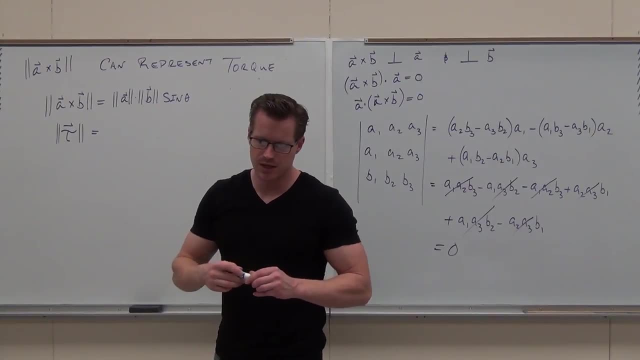 We can think about torque as this: The two vectors you're at actually using. instead of A and B, we're going to use some like real words here. The first one is how far away you are from your point, right? 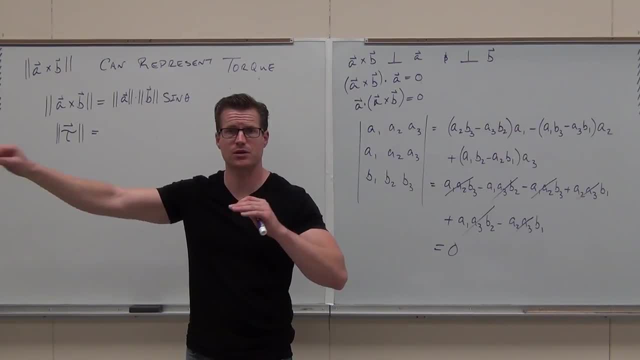 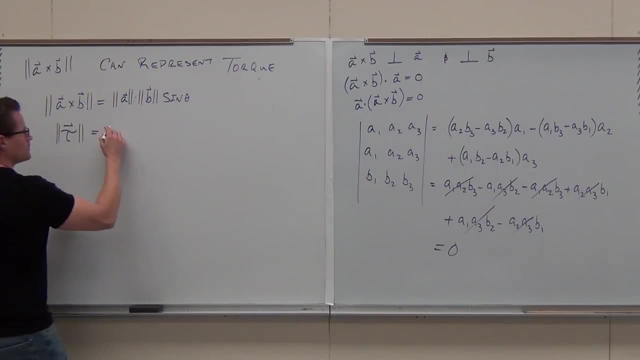 That's called your lever arm and we use R for a radius to represent that. So one vector is- hey how far away you're actually pushing on that. so that's our R, it stands for a vector. So if we use a vector to represent that radius, 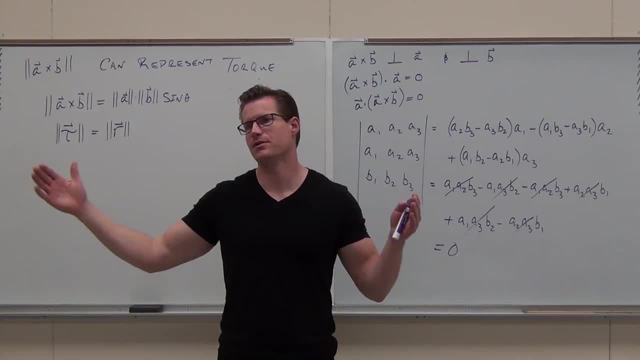 how far away are our lever arm and we take the magnitude. now we literally have the length of our lever, Big enough lever and I can move the world right. So the further away we are with the equal amount of weight. 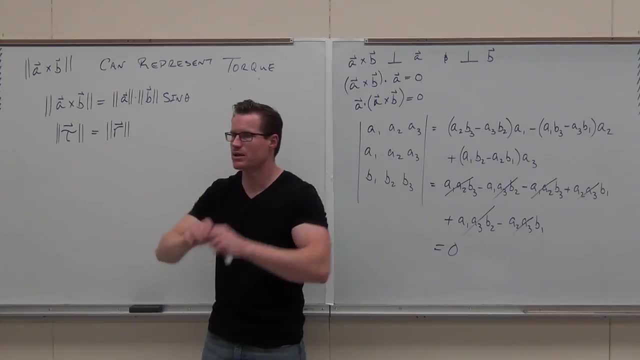 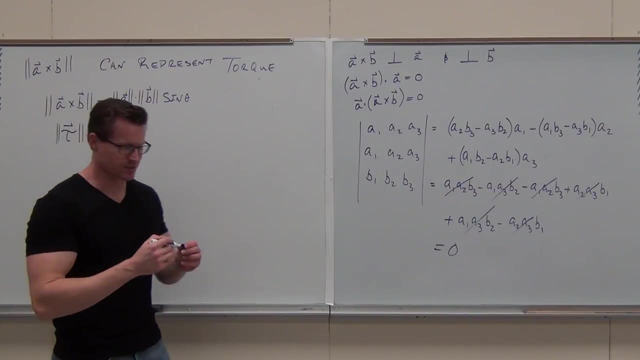 the more torque we're applying, You can see it, The magnitude gets longer, Your torque is more. That's happening, That just happened, And then we go: okay, well, what else? What else is there? Well, at the end of that lever arm, 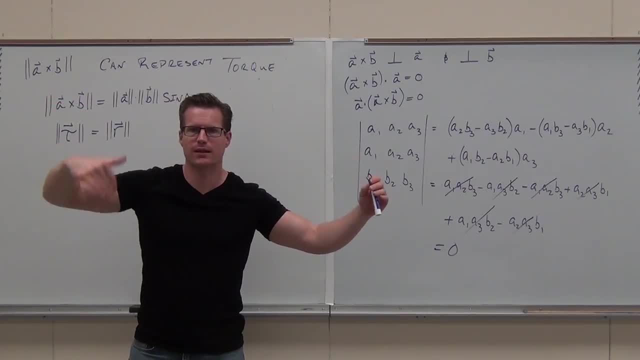 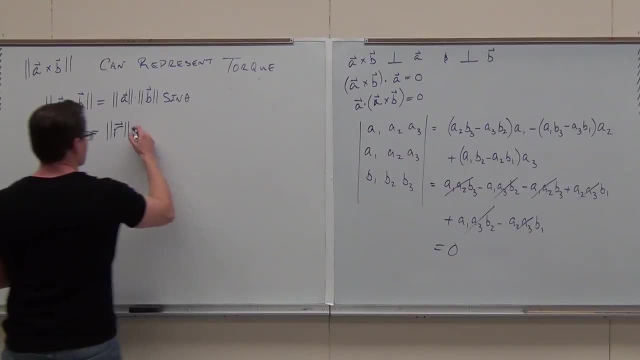 you're going to be applying a force, You're going to be pulling on that lever. Well, that force has a vector and the magnitude of that force is how much you're actually putting on that lever And you're going to be rotating that. so, if I take my lever, 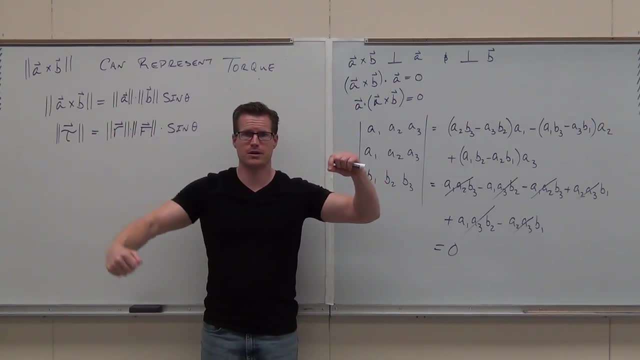 and I put the my force at the end of the lever, I'm going to get some sort of angular motion around a bolt or something real that's turning. So how much we turn, that is how much torque we're actually getting. so the sweeping out of that angle. 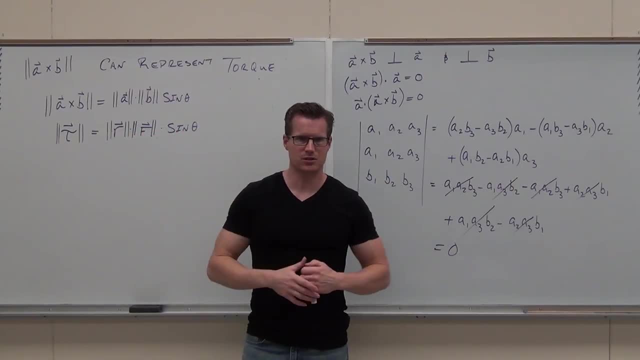 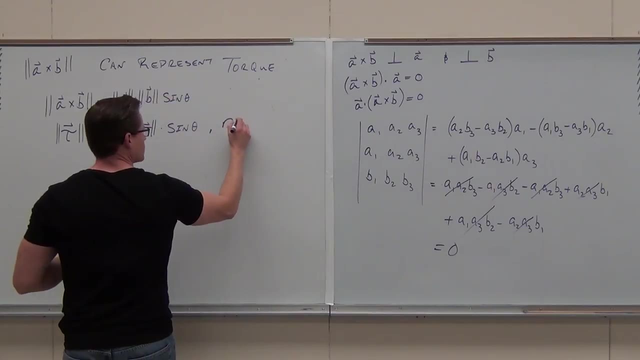 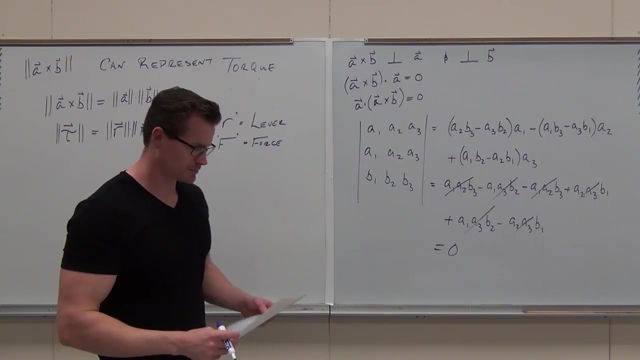 sign of that. times these two magnitudes, That's the magnitude of our torque, It's actually really easy to find R. we say that's our lever, F is our force. if you want definitions, Let me give you one just really quick, quick example. 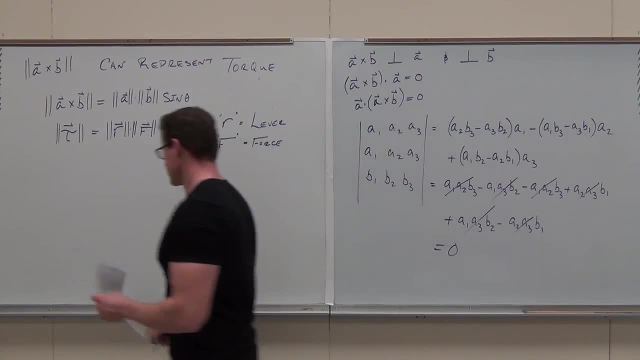 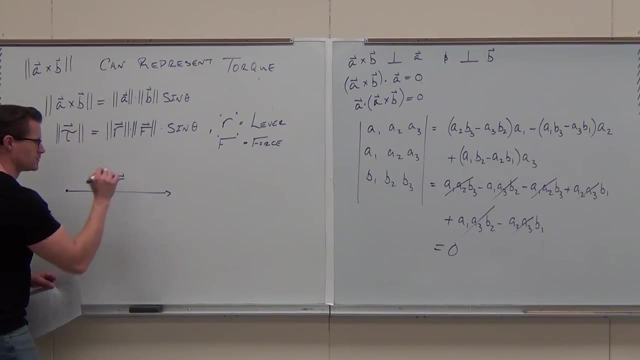 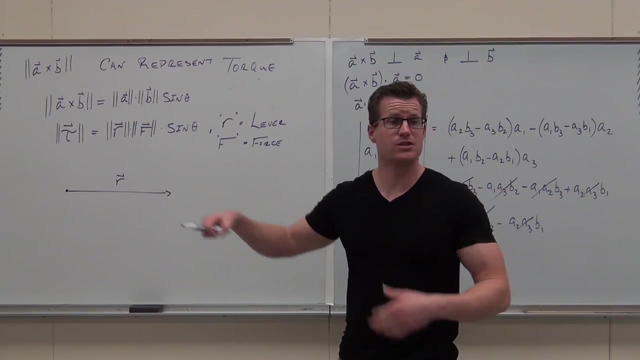 and then we can, we can call it good on our section here. So there's our our what. what's that stand for Lever? So this is the wrench right. So we're, we have a, a bolt right here. 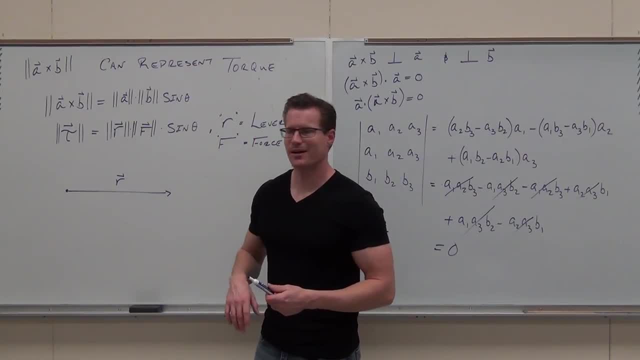 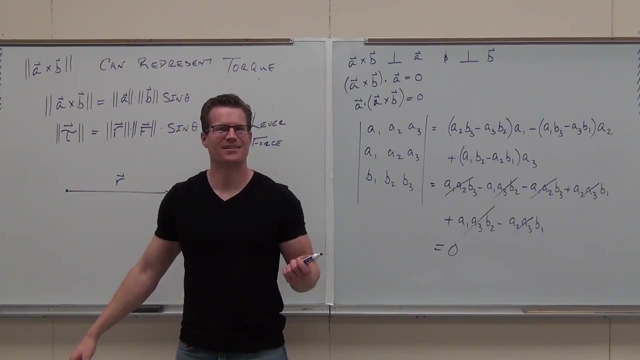 We've got our, our wrench. Now. normally, if you're smart about it, you're going to turn the wrench from right here. It doesn't make any sense Why? Because they're always shortening. They're always shortening. 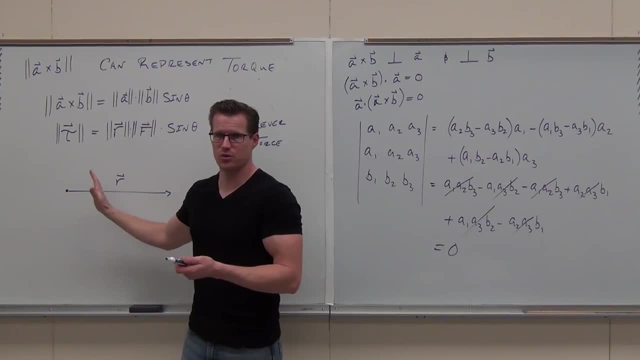 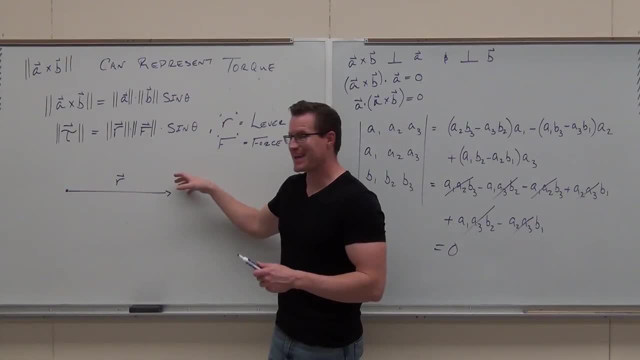 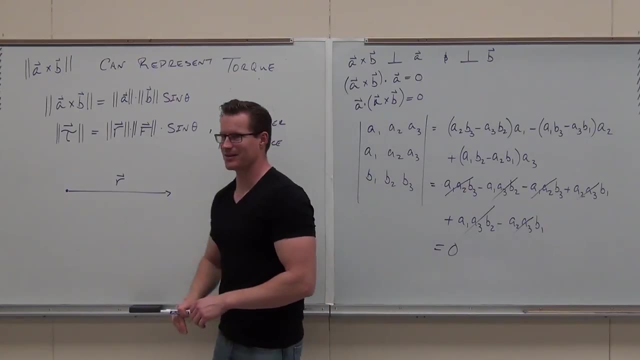 to get the same amount of torque, Which is why we push, logically, at the end of our lever, We go: let's go way out here. Rah, I feel like a man. All right, Anyway, that's how I, that's how I get down. 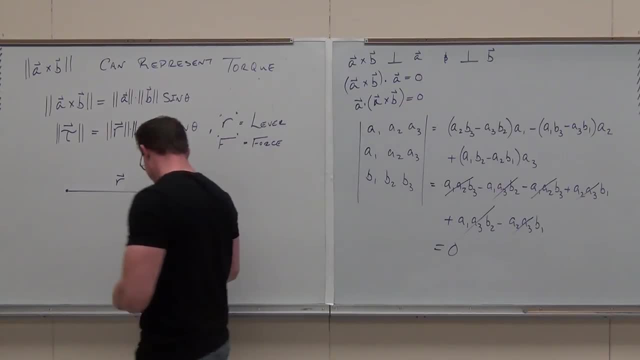 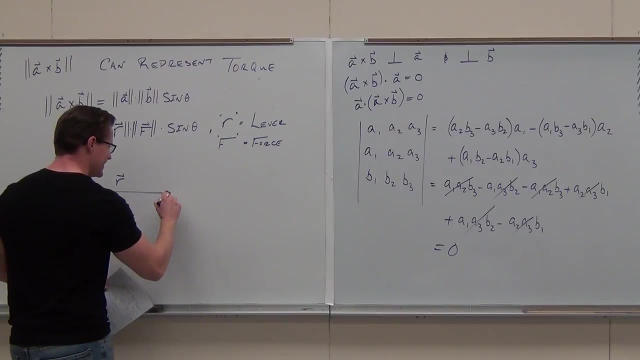 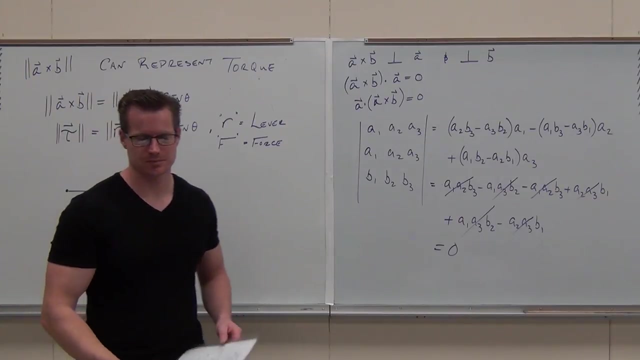 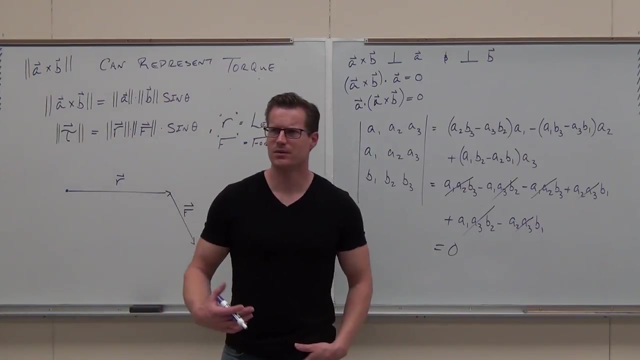 I just torque my lug nuts on my truck And we're going to be, you know, Applying some sort of a force, And you go, wait a minute, this, this doesn't. this doesn't quite look like like our typical torque situation. 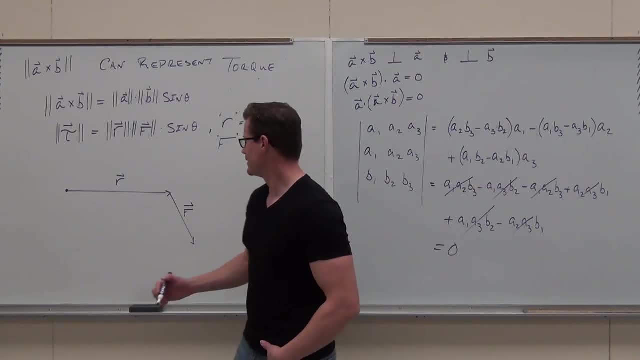 because what we want is a cross product. What we want is this vector to be right there And you go. well, that doesn't. I'm not going to turn it from right here, but by vector addition, by what we can actually do with these things, 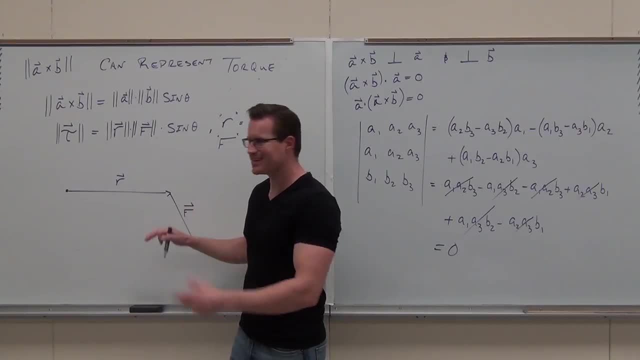 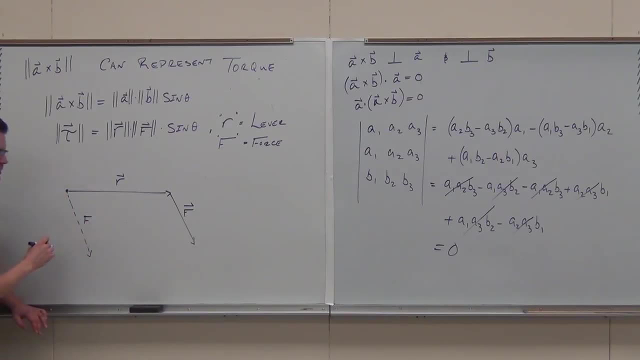 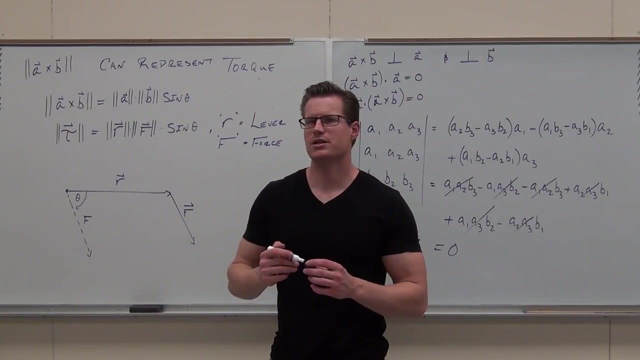 these are all movable Think position vectors. So we go, let's just pretend that our force is right here, And then it really does sweep out an angle. Which way is it going? Which way is that bolt going to turn? Now I know that, logically, all bolts are kind of 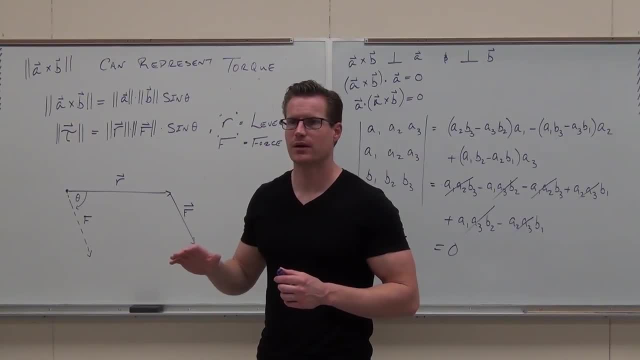 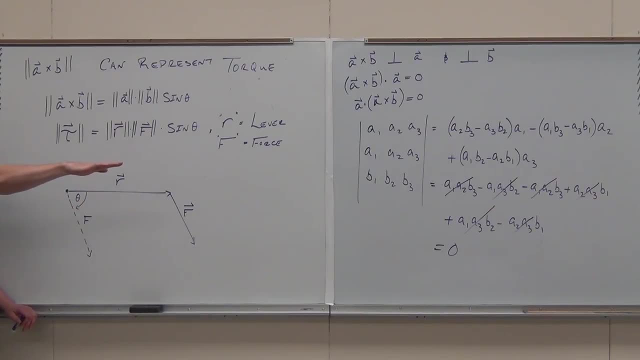 you know clockwise turn. But if you put your hand out and put it on the lever so that your palm opens towards where it's going, We're moving it this way. Where's that bolt going If we, if this was our lever and our force is going this way? 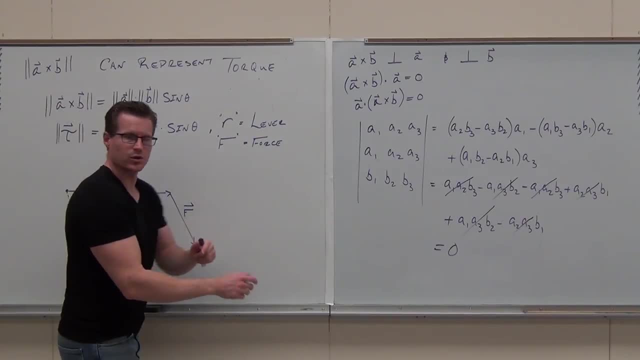 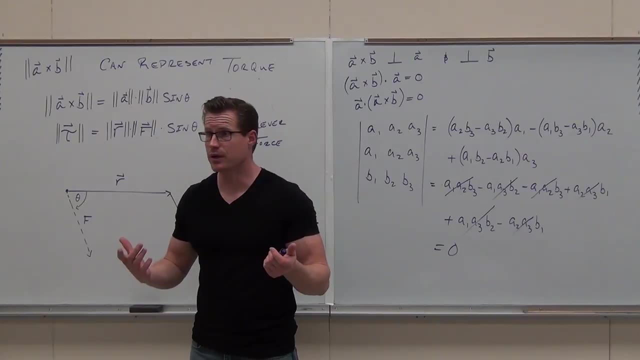 we'd be going out towards you. Does that make sense to you? So we're going to be going in towards the board. In fact, when we think about it, our torque, our torque- is perpendicular to what we're actually doing. Our, our torque doesn't go this way. 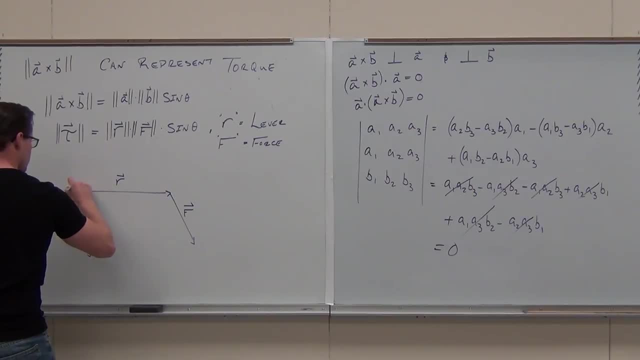 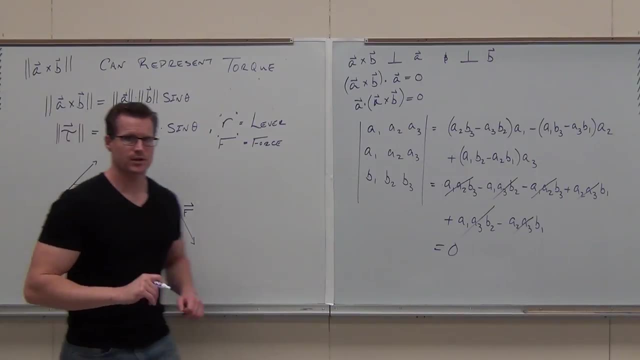 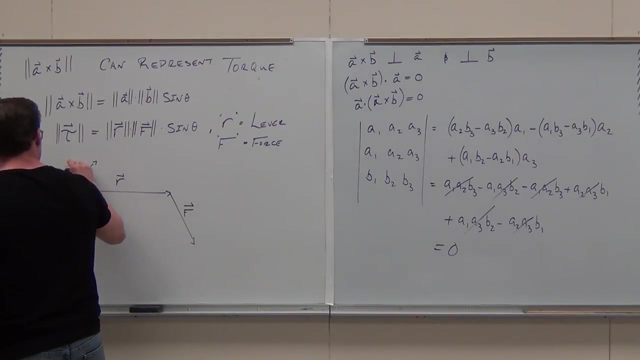 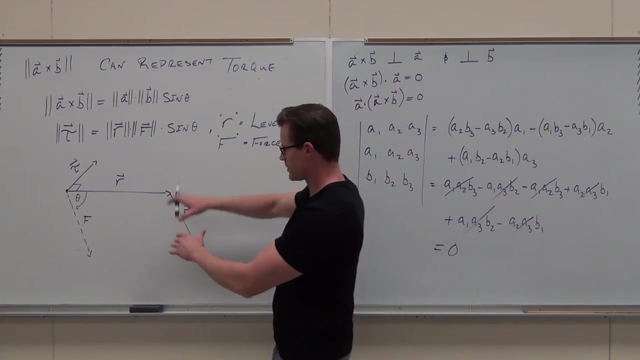 It goes into the board so that it's perpendicular. It's actually mutually perpendicular with that. That's where our torque's headed. It's right in there. If this is on the flat plane, it's going into the board at 90 degrees. 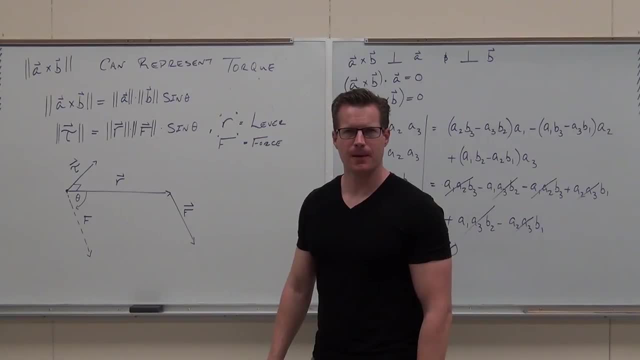 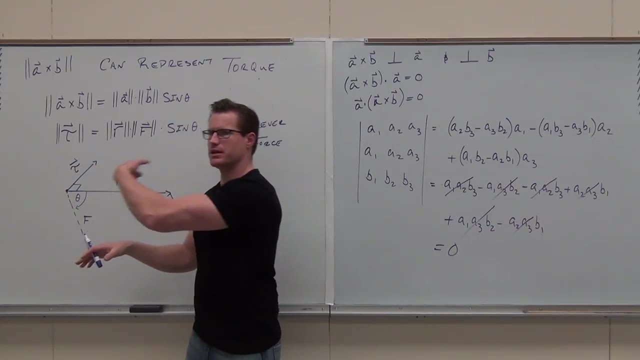 You guys all right with the idea? Do you actually have to move it? Not really. You just have to understand that. that's what's going on. is that we're sweeping out an angle. It's moving into the board. That's, that's the plan. 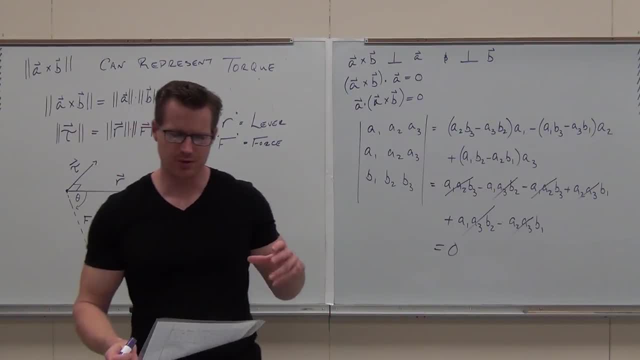 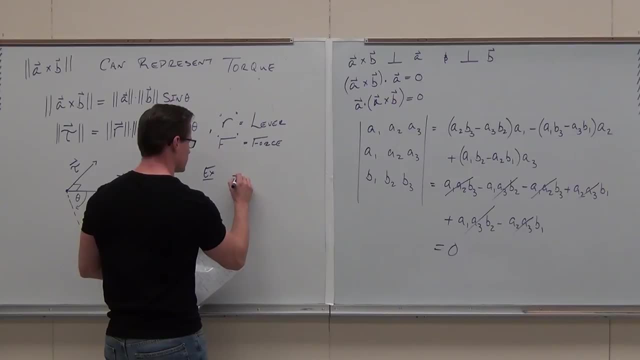 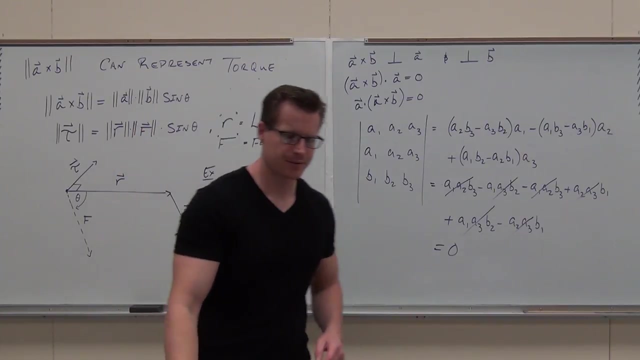 Let's go ahead. Let's do one example. Again, we're focused on the magnitude- how much is actually happening- And we'll call it good on our section. So you got a hex head bolt. We've got a pretty standard, you know: open end wrench. 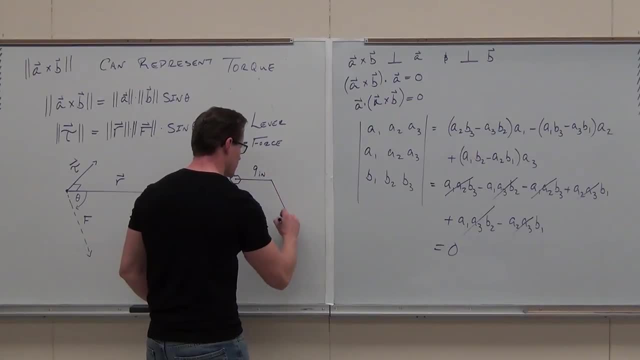 And then we're: we're pulling on this thing, Pulling this thing with 50 pounds, So we're putting some weight on it And I'm guesstimating here, So we're going to be rough estimating, But that's 60 degrees. 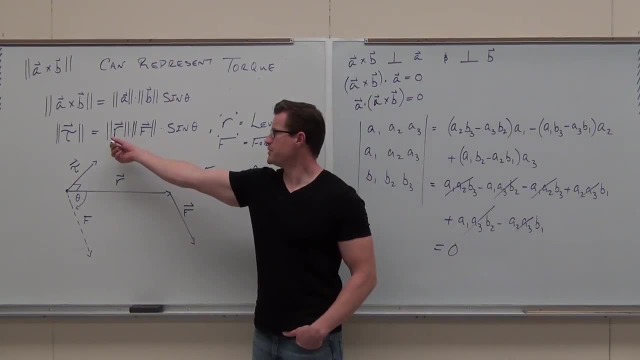 So, again, the way this works is: hey, do you know the magnitude of your? oh, you need some magnitudes. Do you know the magnitude of the lever? Yes, What is it? Nine inches, Nine inches, Inches That matters. 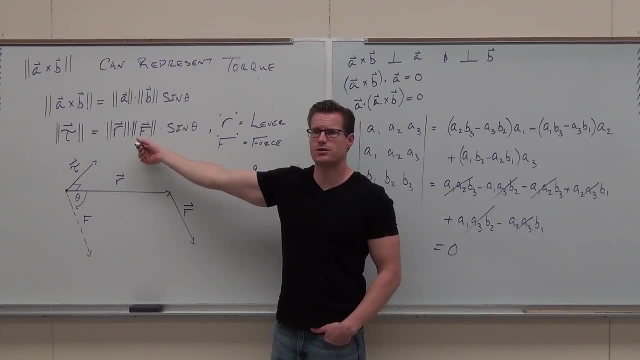 Yeah, That matters. What's the magnitude of your force? Notice, I don't really care about the actual vector, because we're talking about magnitudes here. And then do you know the angle between them, How much we're going to sweep out, is what we're talking about. 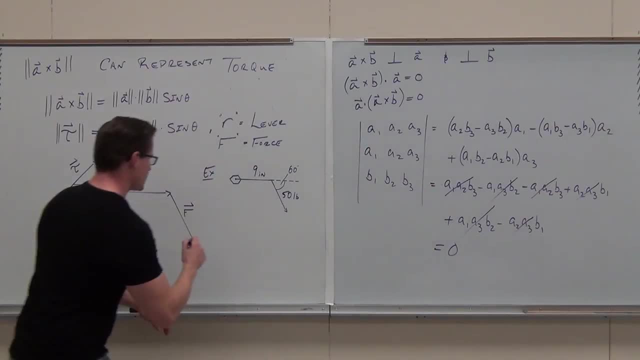 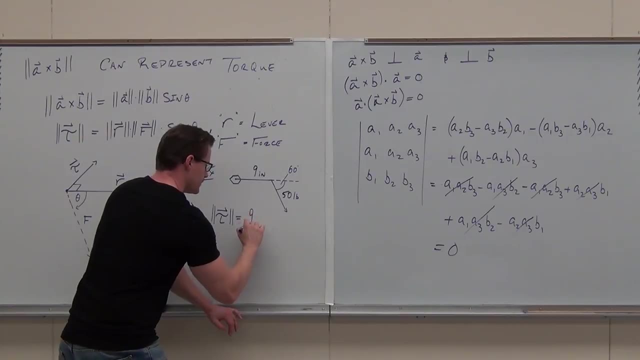 What is that? So, if we want to find the torque in this situation, We got nine inches, because that's the magnitude of our lever. We got 50 pounds, because that's how much force we're putting on it, And it's at the end of our lever. 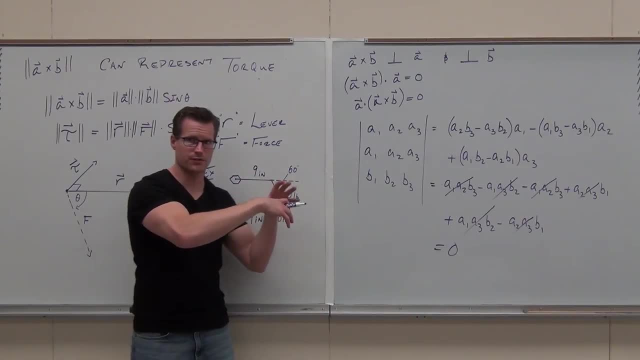 So if your lever was actually longer but you were not holding it at the very end, you'd have to go to where you're actually holding that lever. So if you had a one-foot wrench, but then you're at nine inches, you've lost some of that energy. 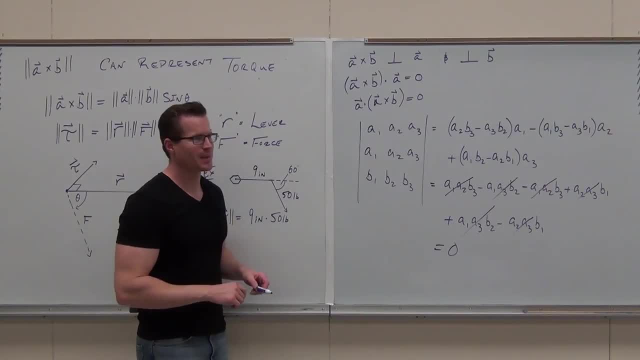 which, yeah, that's typically what happens. right, We don't go: oh, here's my wrench, Hang on Right there. You can't do that Because you can't get enough on it. So you're- I mean you're- grasping it. 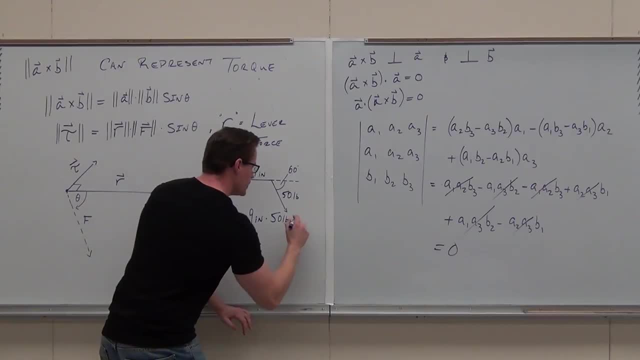 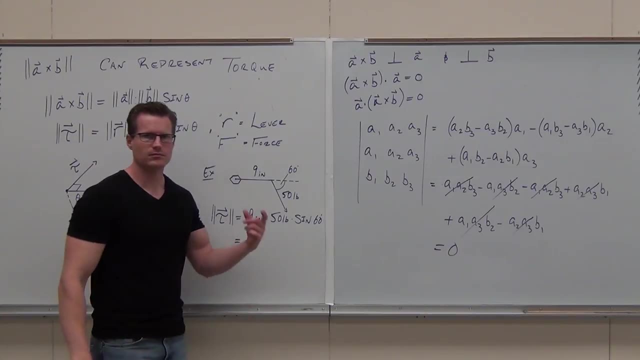 Yeah, So you've got to measure to where you're actually holding that wrench. Sine 60. All right, How much is that? A rough estimate, So you can just give it to me to the 10.. So I know, sine 60 degrees root 3 over 2, but just use the decimal approximation of that. 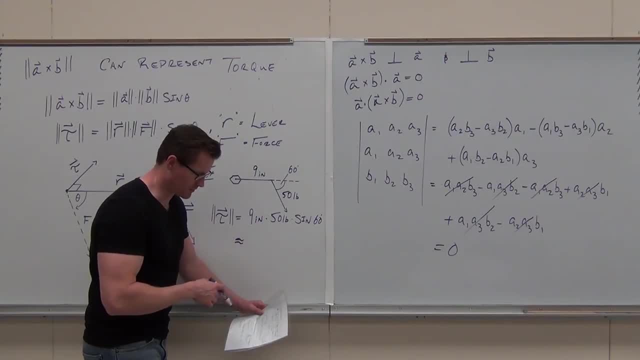 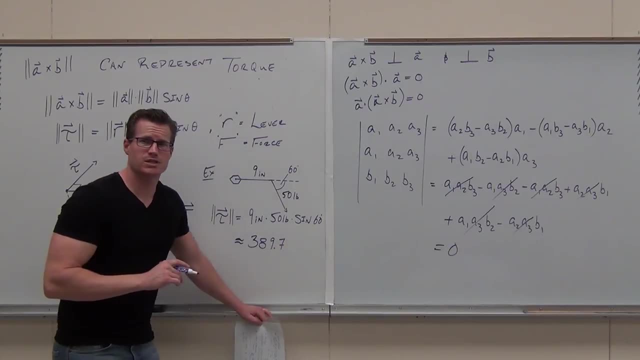 If you would multiply by 50,, multiply by 9, and tell me what you got, It should be All right. It should be like 300-something, 389.7. what Inch pounds Not pounded? 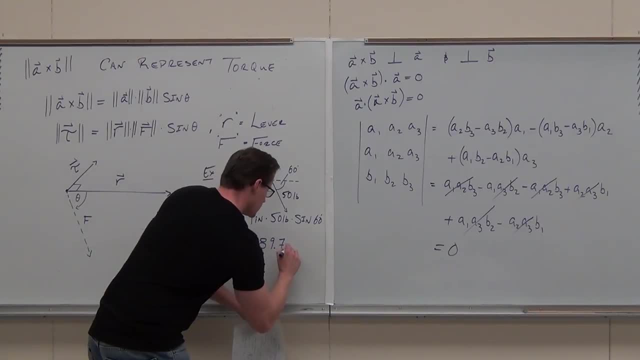 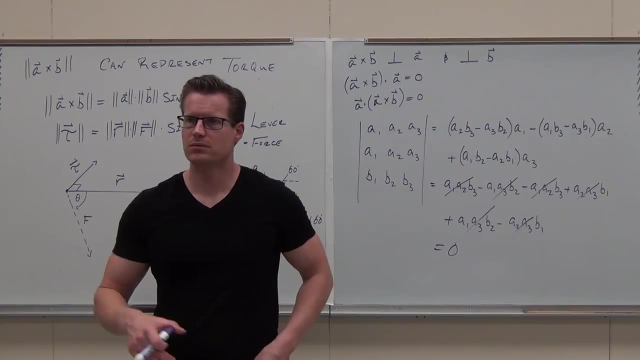 Foot pounds. Inch pounds. Inch pounds- Oh, Could you change it to foot pounds. Yes, Yes, How? Yeah, divide by 12.. Divide by 12.. Yeah, 12 inches in the foot. Divide by 12, and you go. 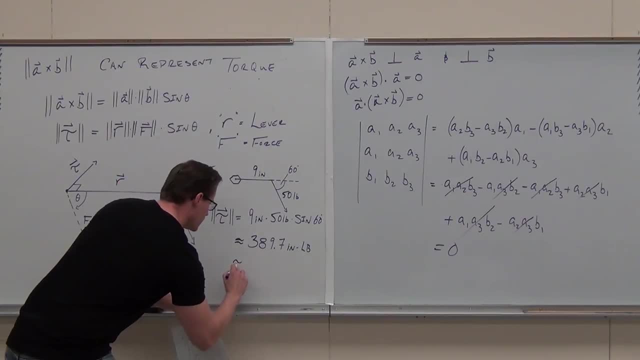 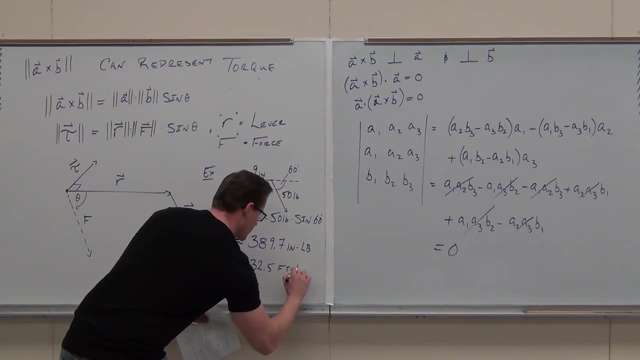 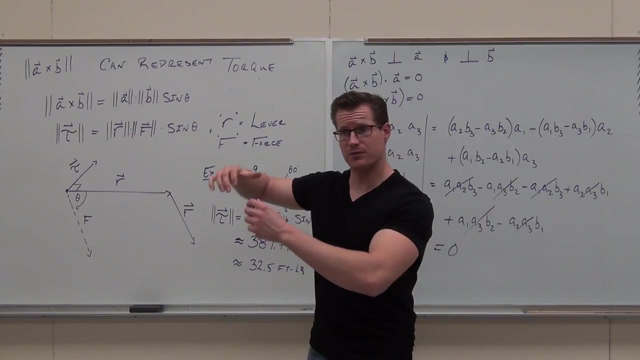 Okay, Well, yeah, You know what My torque wrench is: in foot pounds, About 32.5 foot pounds, which that should make sense, right? You're putting 50 pounds, but not at the end of a foot. 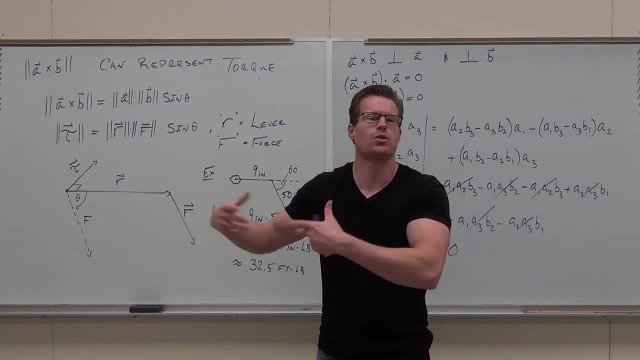 It's something that's shorter than a foot. You're going to lose force on that and you're going to lose torque on that is what I'm talking about. So show of hands, do you feel okay with what we've talked about? 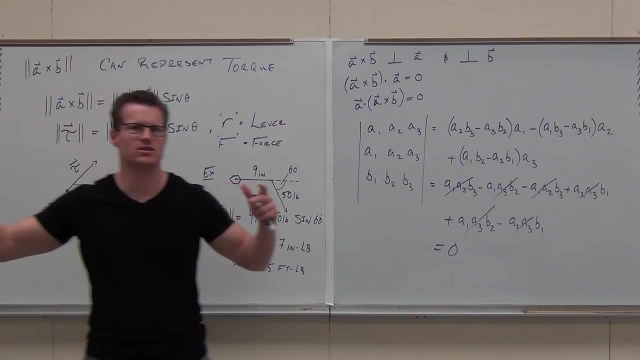 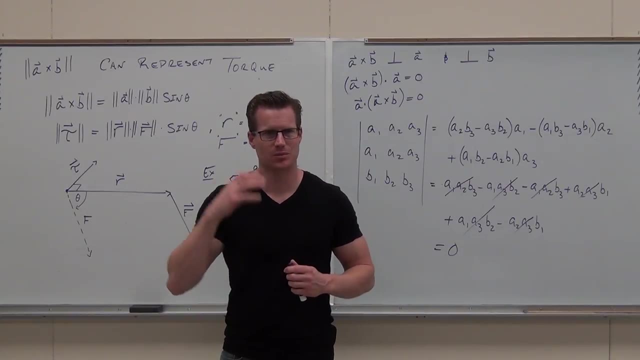 Does this example make sense? Sweet, Any comments? questions like anything about it. Torque thing is pretty cool, right? Something compared to what we've done, maybe even a little bit easier to visualize. That's what I like to do. 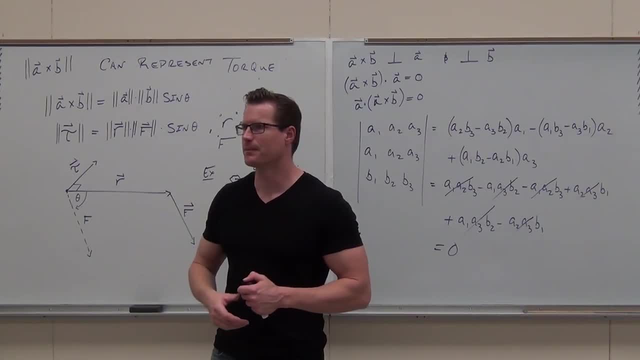 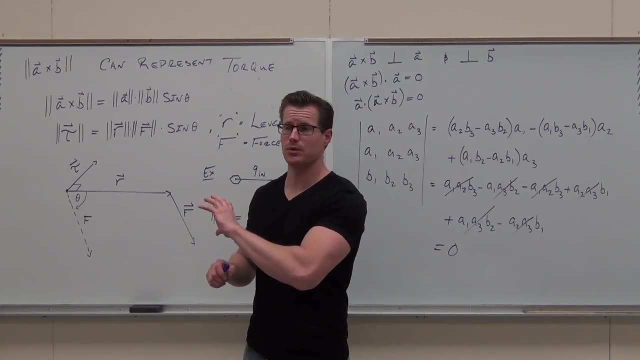 I like to make sure you at least can see something that's visual about it. Is that how the wrench or that you're putting the pounds on? That's how much torque is being applied to that bolt. So you are putting down 50 pounds. 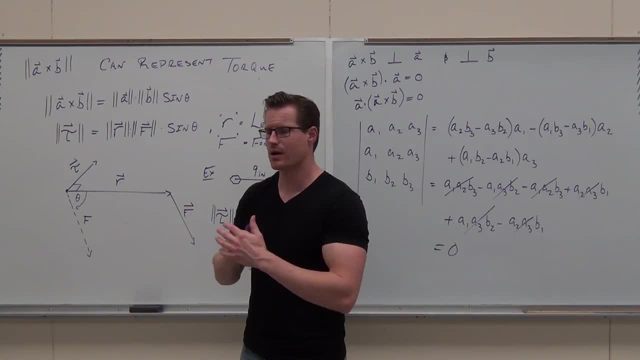 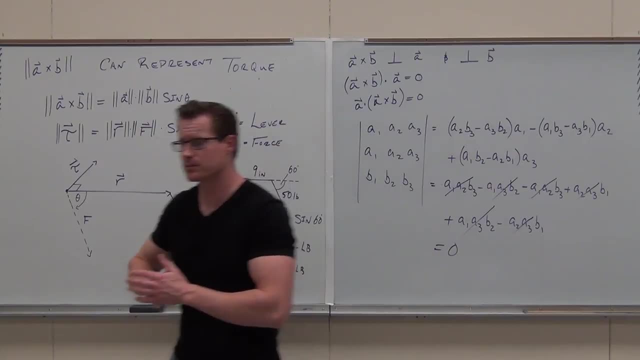 That's staying there. The wrench is nine inches long, so that's staying there, But when we're sweeping out that angle, apply 32.5 foot-pounds of torque on that bolt.